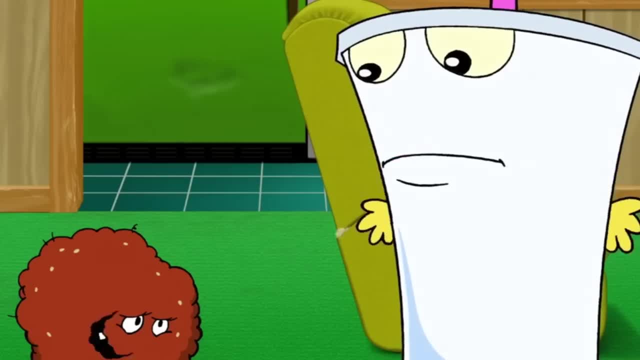 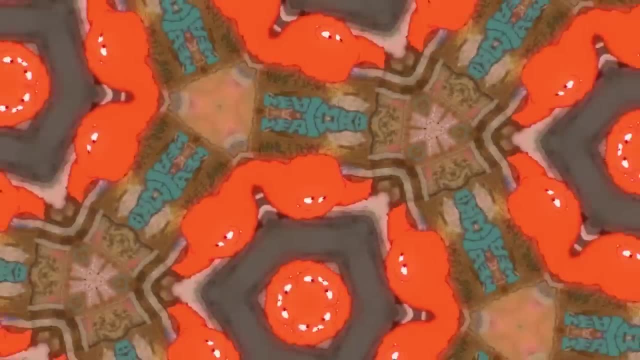 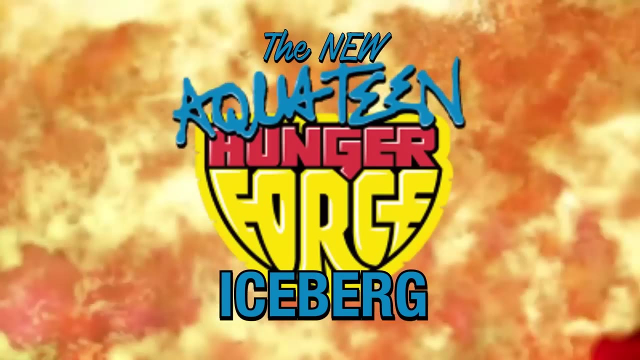 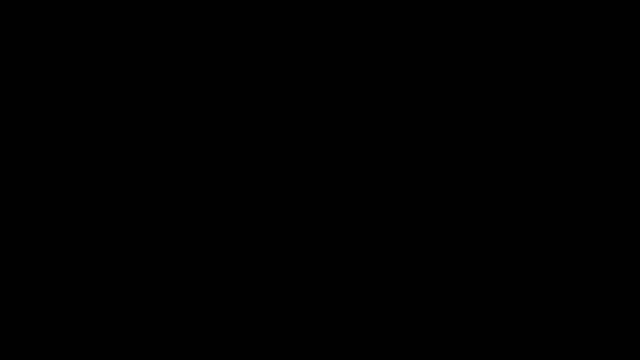 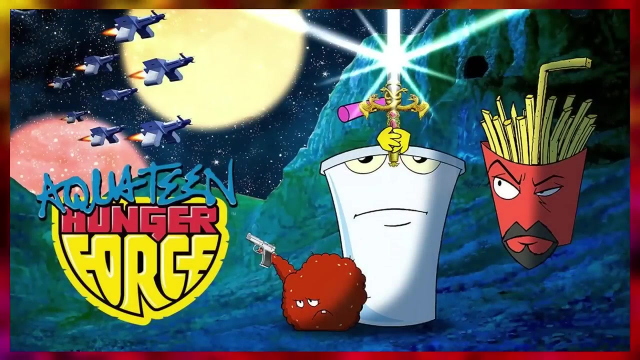 cuddle up with your loved ones and let's dive right into this brand new iceberg. ON DELAY, CONTINUITY IS FORBIDDEN. Okay so canon isn't forbidden, but the series has almost zero continuity, Which is great for new viewers, because they don't have to know anything about season three to. 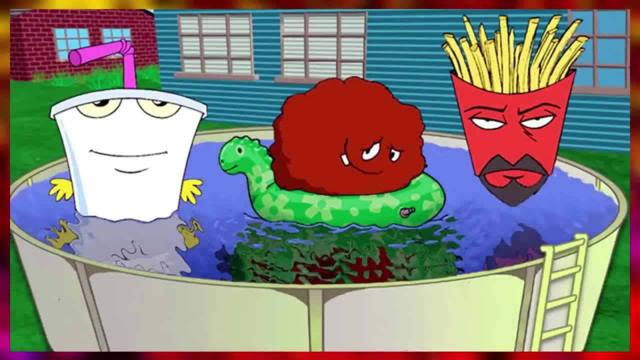 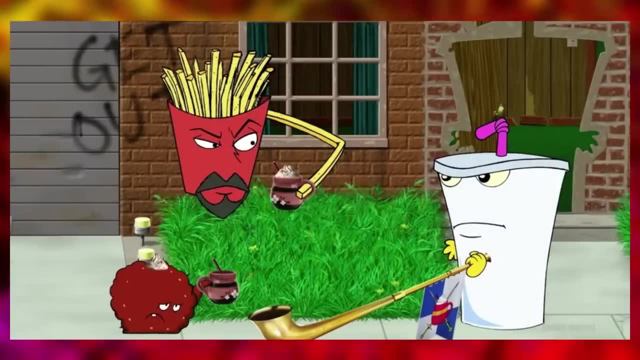 understand and enjoy season nine. for example, Everything from character deaths to blown up houses and TVs and characters becoming disfigured does not matter. in the grand scheme of things, All tragedies and disasters in the world of Aqua Teen just get reset. However, there are some rare 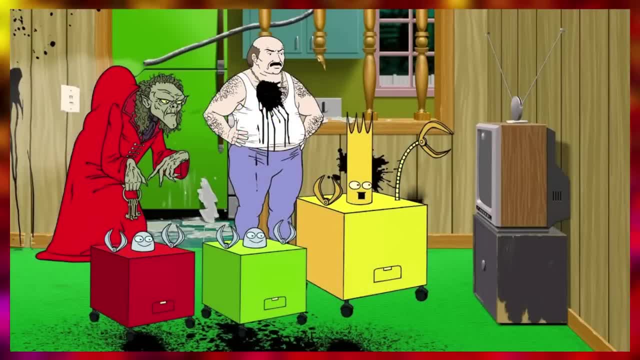 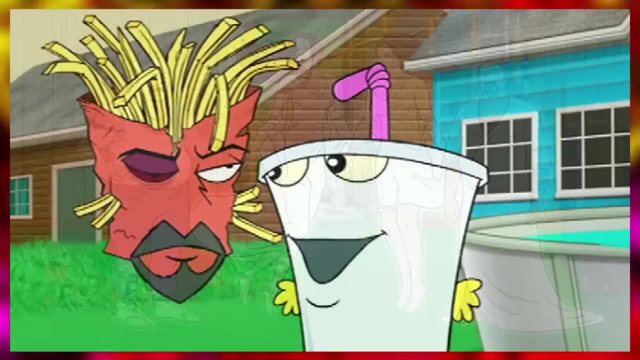 instances of continuity in the series, like characters bringing up past events, and there's also the linkage of the first three episodes of season five. But besides those examples and a couple of others, the show just does whatever it wants and there are never any long-term consequences. 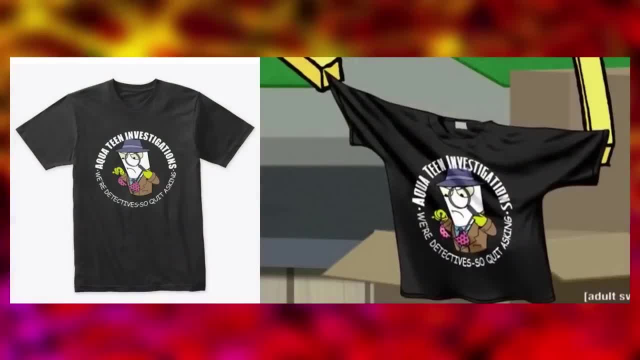 SCRAPPED DETECTIVE IDEA. Briefly, during season one, the Aqua Teens set out to solve crimes under the title Aqua Teen Investigations. However, the detective idea was abandoned just after the first few episodes of the first season, Though the idea was revisited during season eight when the show 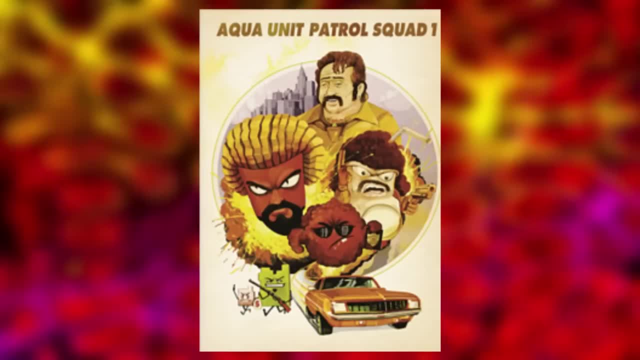 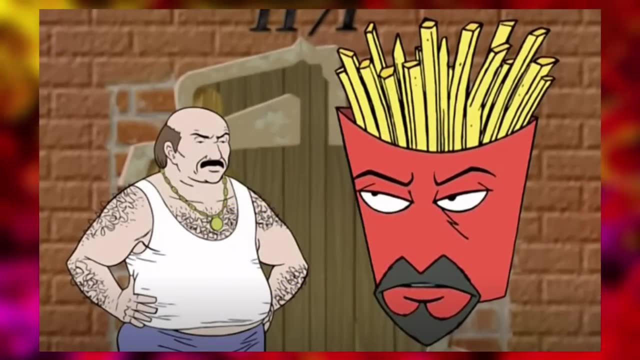 changed its name to Aqua Unit Patrol Squad One. The detective days are sometimes mentioned throughout the series, like in the Aqua Teen episode Kidney Car, where Frylock mentions that they stopped being detectives because the business was not making them a whole lot of money. According. 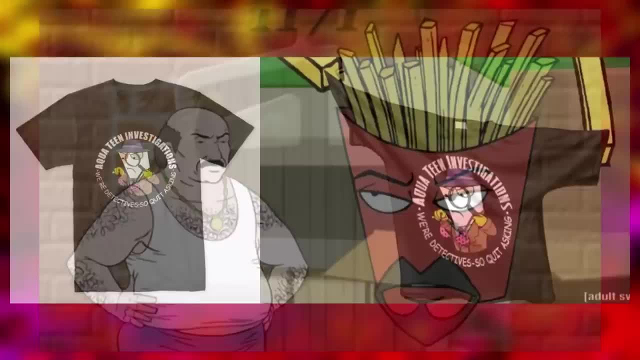 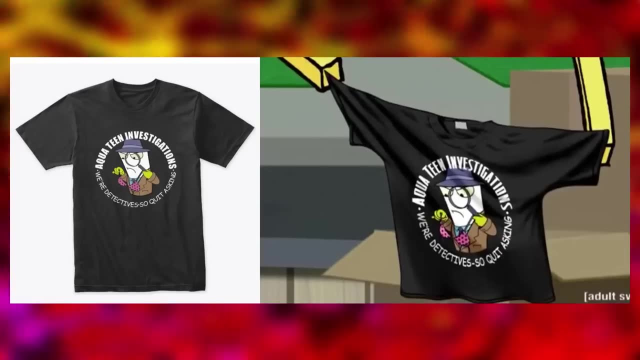 to Dave Willis and Matt Malero. they only made the Aqua Teens detectives because they felt like the network would identify more with that concept instead of just talking food products hanging out. So they disguised the series for a couple of episodes and eventually dropped the whole. 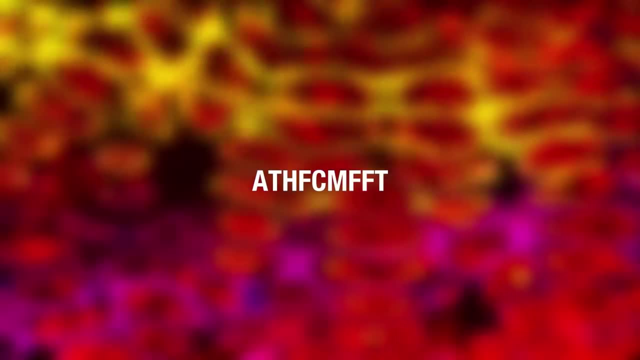 detective bit by episode four. SCRAPPED DETECTIVE IDEA. The series is based on the story of a woman who was tested positive for FSM and she was also on board to get a job at the United States. SCRAPPED DETECTIVE IDEA- Aqua Teen- Hunger Force Movie Film for Theaters. 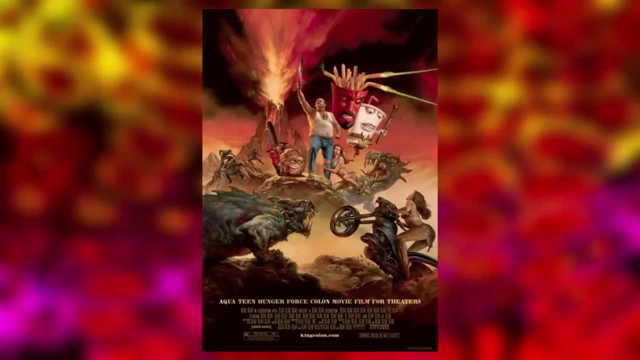 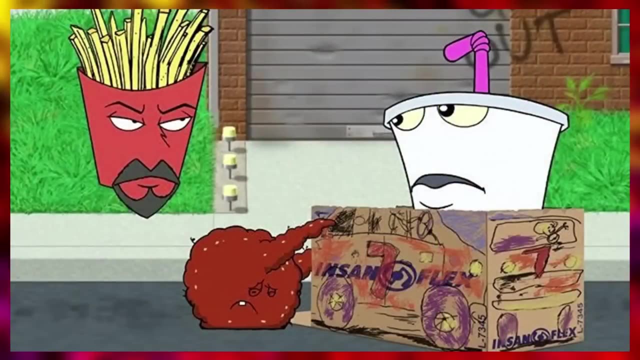 Aqua Teen Hunger Force Movie Film for Theaters was the first full-length Aqua Teen movie and Adult Swim's first theatrical release. The film released on April 10th 2007 and earned a whopping 5.5 million Freedom Dollars in box office sales. GOOD LORT, THAT'S BUSSIN. 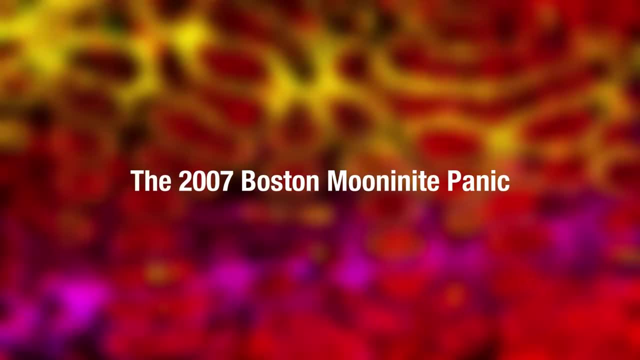 SCRAPPED DETECTIVE IDEA: The 2007 Boston Mooney Night's Panic. In November of 2006, Boston Air and Air was gonna be releasing a series of excellent, exciting romantic and gotten a super big success. The series was a hit, but the social media非常 hit it hard as it wouldn't stressing the 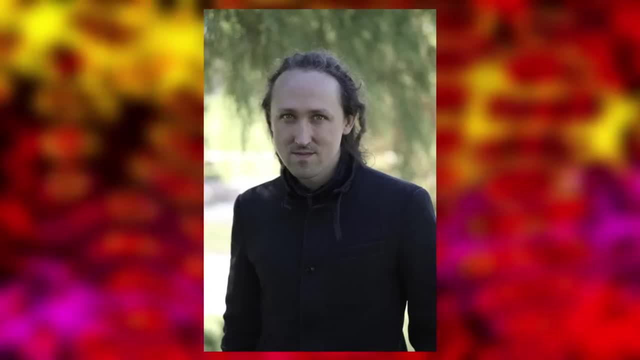 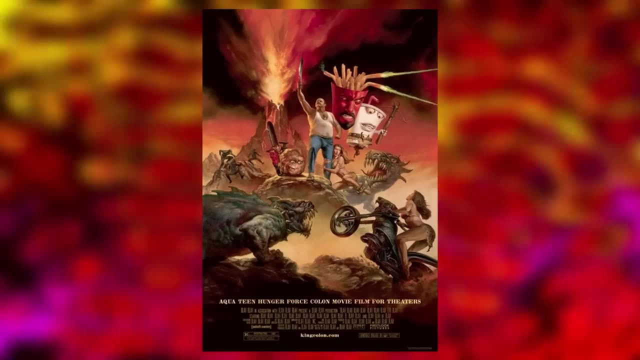 artist Peter Berdovsky, who goes by the pseudonym Zebler, was hired by Interference Inc to work on a promotional project, aka a guerrilla marketing campaign- for the first ever Aqua Teen Hunger Force movie, which was scheduled to release in April of the following year. The project consisted of: 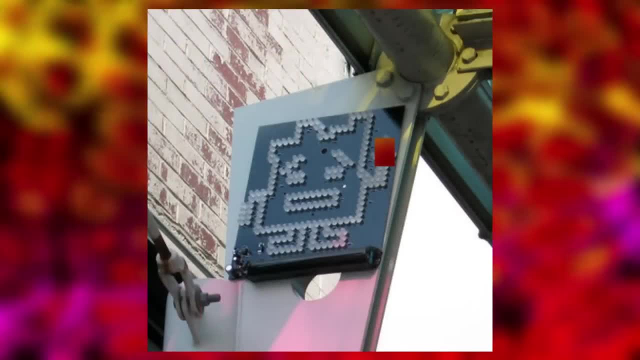 hanging up 40 electronic signs throughout certain areas of Boston. These signs were battery-powered LED light brights depicting the Moonanites Ignignok and Ur flipping the bird. Berdovsky agreed and enlisted his friend Sean Stevens to help, So the company sent the guys 40 signs. 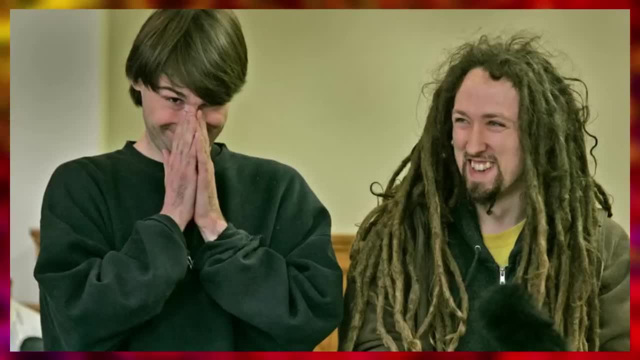 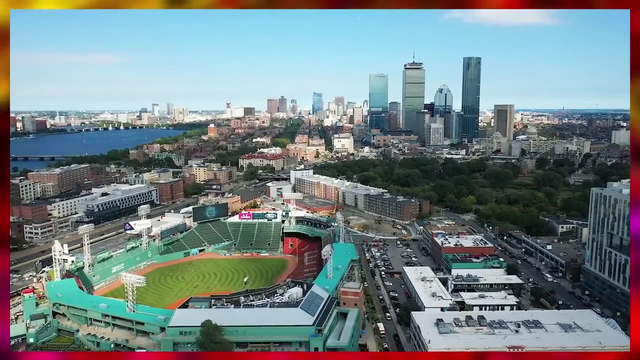 a list of where to place the signs and also some do's and don'ts. The signs were placed throughout Boston in January of the following year and the guys were each paid $300 for their service. The two men also filmed themselves placing each sign throughout the city to prove. 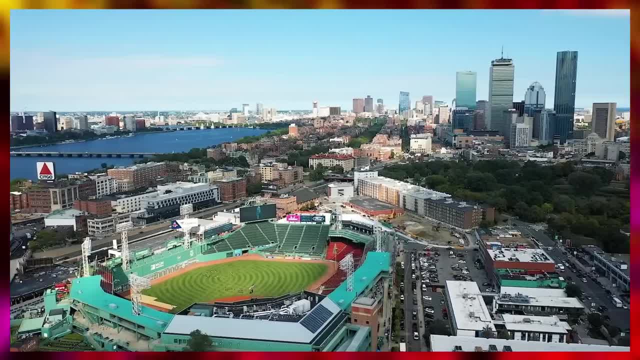 to Interference Inc that they completed their mission. However, on the morning of January 31st 2007,, a person spotted one of the Moonanite signs on a stanchion that supported the Moonanites, Ignignok. The sign said: 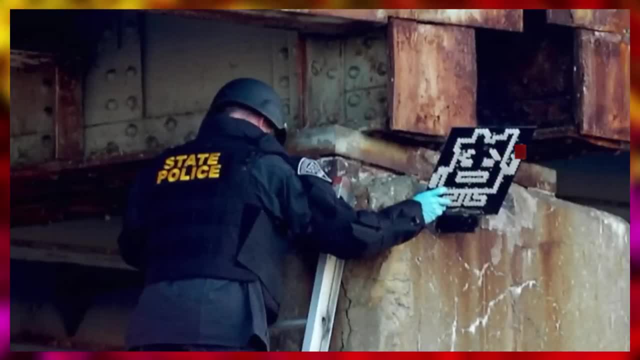 of Interstate 93 above Sullivan Station. Soon afterwards, the Boston Bomb Squad arrived to the scene and ultimately used a small explosive filled with water to destroy the first electronic sign as a precaution. Throughout the rest of the day, the city of Boston was on pause as more and more. 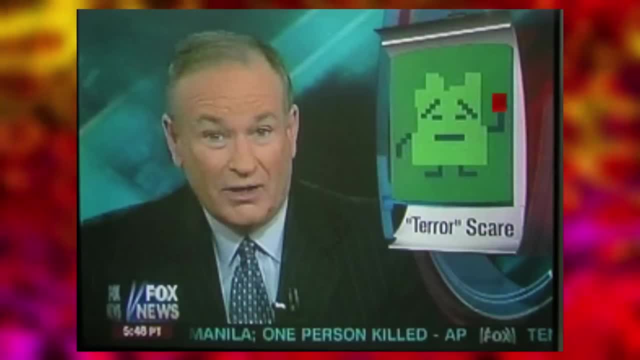 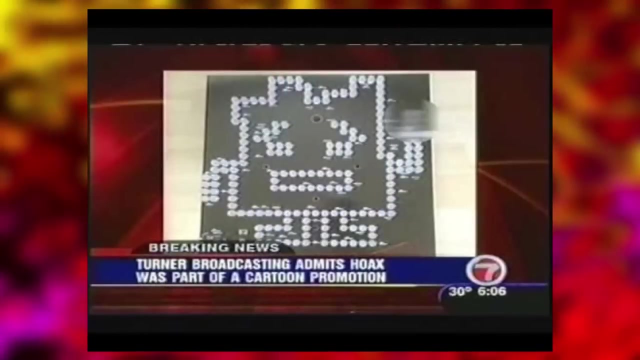 of these signs were discovered. Basically, the Boston Police and Fire Departments mistakenly identified these battery-powered LED signs as improvised explosive devices or IEDs. As it turns out, 10 cities were involved in this marketing campaign, which began two to three weeks before the Boston incident occurred. After about seven 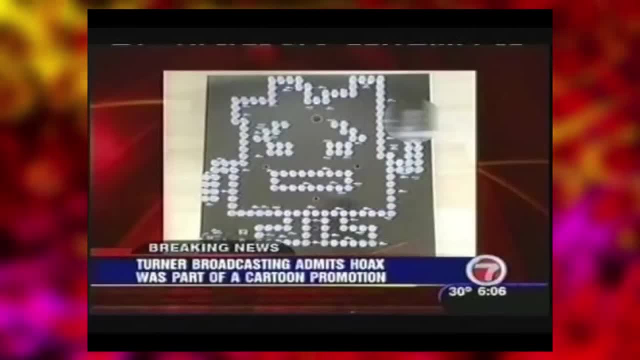 hours, the images on the signs were finally identified as Moonanites and the police concluded that the incident was just a publicity stunt. As a result, Turner Broadcasting had to pay $1 million to the Boston Police Department and another $1 million to the Department of Homeland. 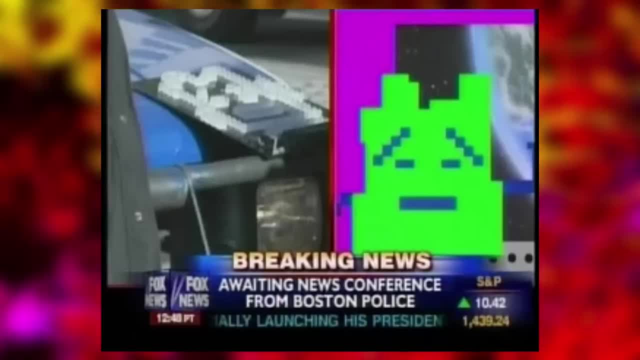 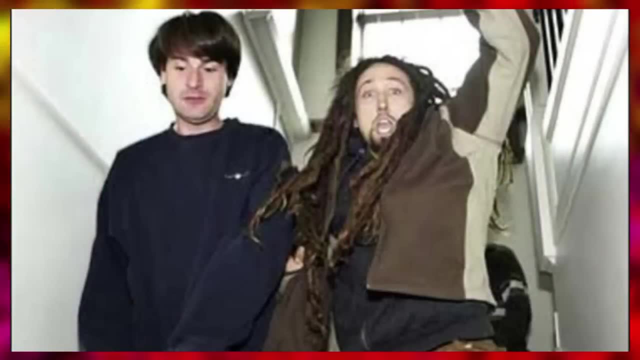 Security. Cartoon Network's general manager and executive vice president, Jim Staples, also resigned from the company. And as for Berdovsky and Stevens, they were also arrested by the Boston Police Department during the evening of the same day for violating Chapter 266, Section 1021.5 of the General Laws of Massachusetts, which states that 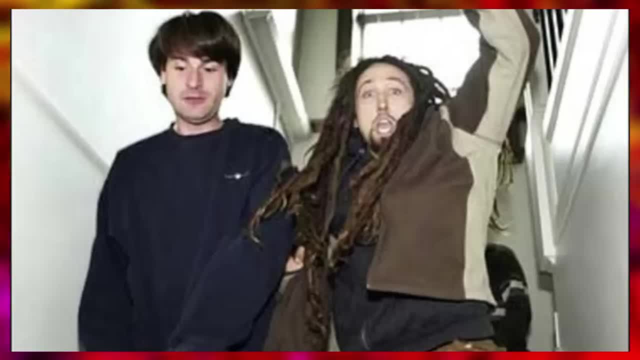 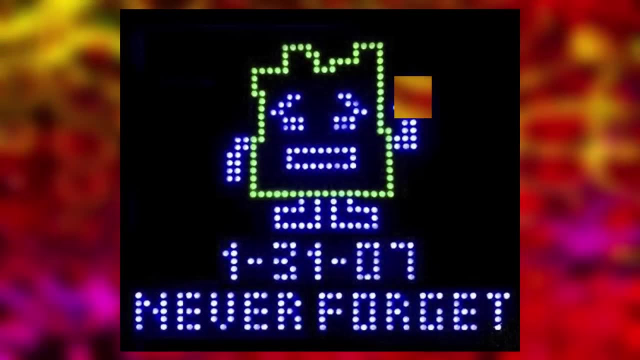 it's illegal to display a hoax device with the motive to cause citizens to feel threatened, unsafe and concerned. They were released on a $2,500 bail the following morning. The two gentlemen ended up completing 80 and 60 hours of community service and made a public. 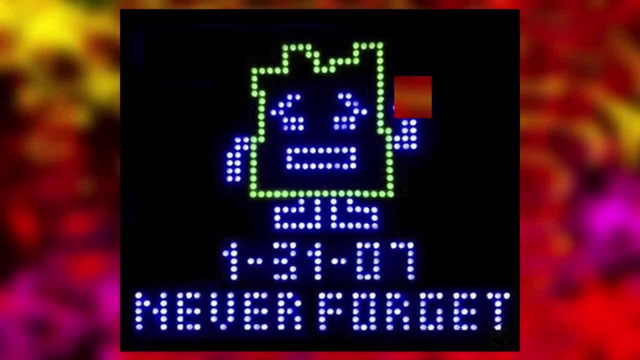 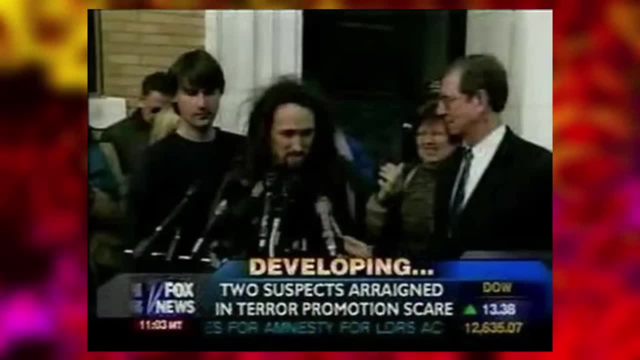 apology And Turner Broadcasting also issued a public apology. One of the most bizarre moments from this entire fiasco was when Berdovsky and Stevens appeared for a press conference and, instead of answering the media's questions about the panic, they refused to answer any questions not related to haircuts from the 70s. As for the rest of the signs located in other major cities around the United States, some fans quickly acquired as many of these LED lights as they could and tried to auction them off on eBay with prices ranging from $500 to $5,000.. So, to answer that question, I'm going to give you a little bit of an idea of what's going on. 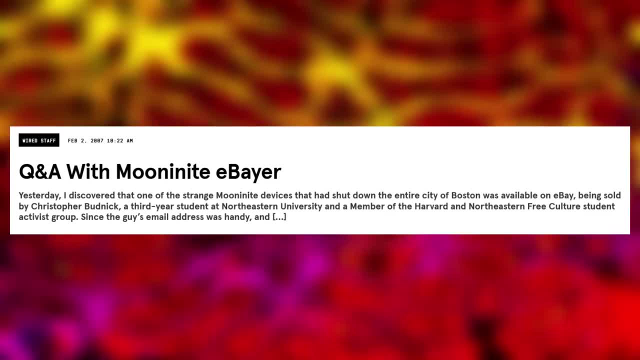 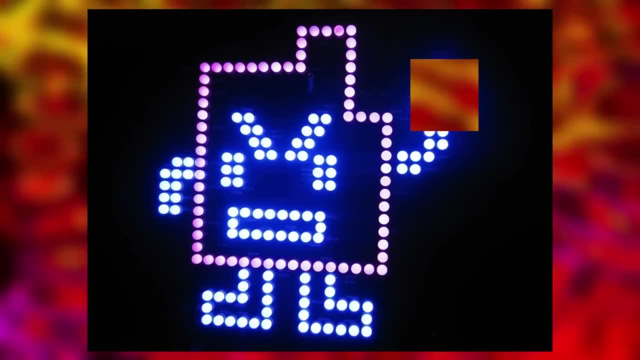 Whoever currently owns one of these authentic signs. I envy you a lot. You are very lucky to have a piece of history in your possession. However, there is still hope for those of you who want one of these LED Moon Knight light up signs based on the 2007 Boston hoax. I did some 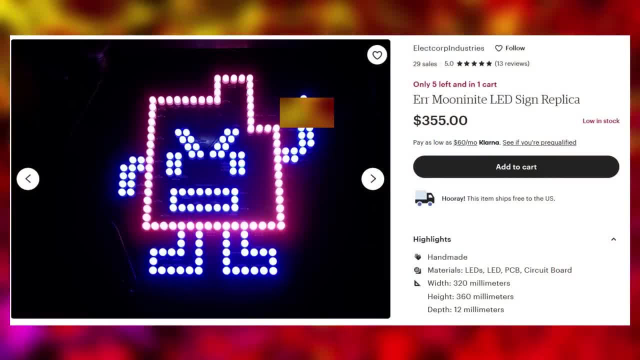 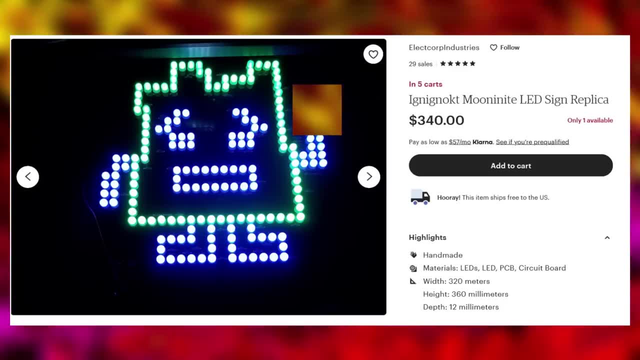 digging and found an Etsy account that makes identical replicas of these signs for like $350.. And you know what? I kind of want to buy one of these signs. I mean sure I could be making more responsible decisions with my money, like paying my tax. 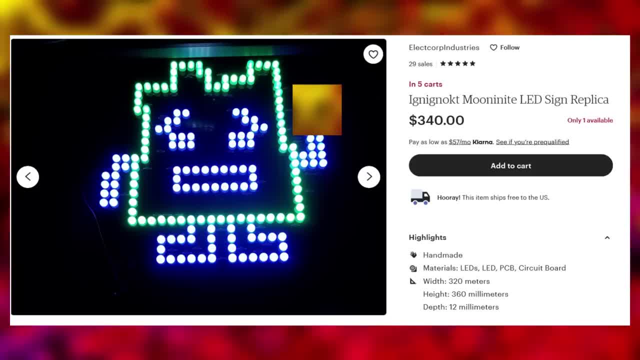 and replacing my brakes and rotors and getting my car inspected. But I mean, come on, guys, which is more important here, Being a responsible taxpayer with a great driving etiquette Or buying a cool LED light for my setup? Yeah, exactly right, You know, it's a good thing. I'm not a 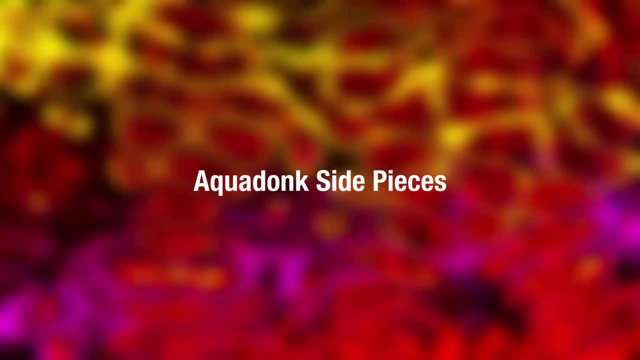 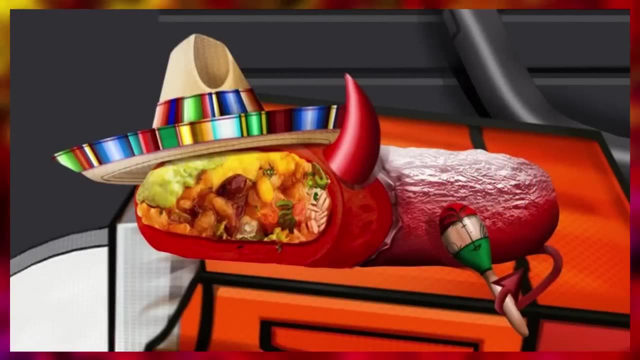 financial advisor. Aquedunk Side Pieces. Aquedunk Side Pieces is an online exclusive Aqua Teen miniseries that puts a focus on some of the most popular villains of the series, like the Plutonians, the Moon Knights and Hand Banana. 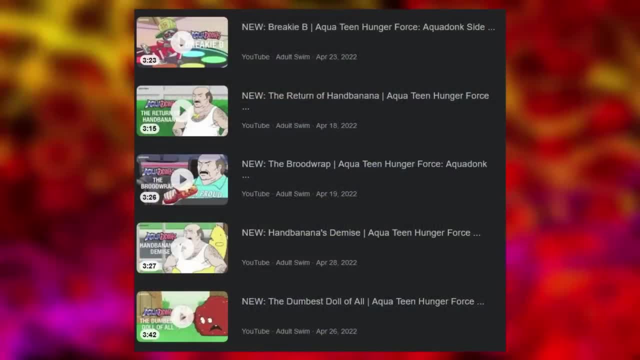 If you search for the name of the series, you'll find a link to it in the description below. If you search up Aquedunk Side Pieces on YouTube, you will find a playlist of 10 short episodes that are sure to make you laugh your pain and sorrows away. 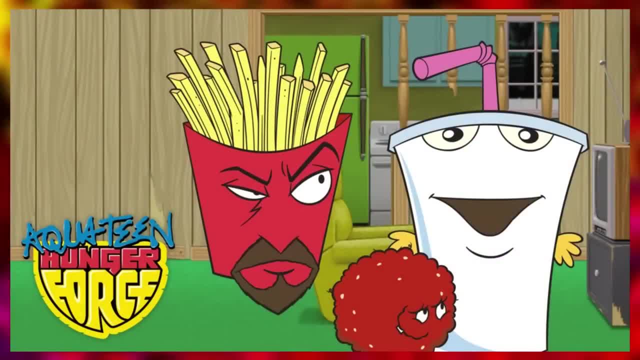 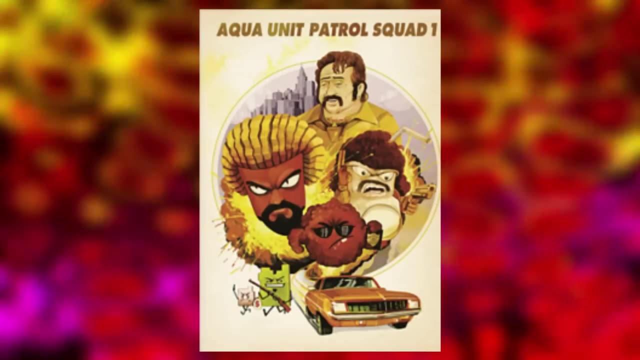 Name Changes. For the first seven seasons, the show's title was Aqua Teen Hunger Force. It wasn't until the introduction of season 8 where we would see Dave and Matt's desire to mix up the formula by renaming the series for each season going forward. So Aqua Teen Hunger Force was changed to Aqua Unit Patrol. 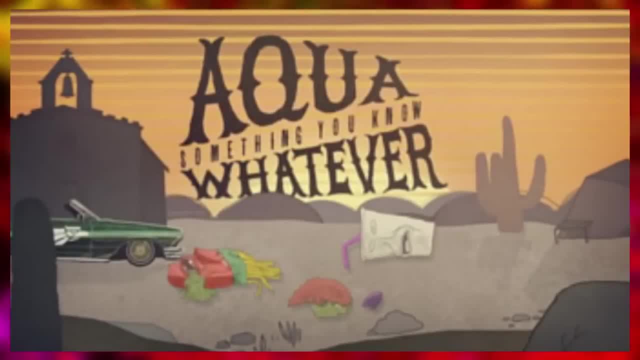 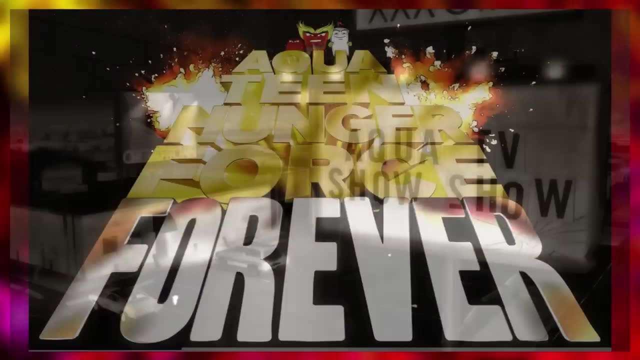 Squad 1 in season 8.. Then it was changed to Aqua Something You Know Whatever for season 9.. Then the title was changed to Aqua TV Show Show in season 10.. And finally the show was renamed one more time to Aqua Teen Hunger Force Forever for season 11.. According to Dave Willis, the reason 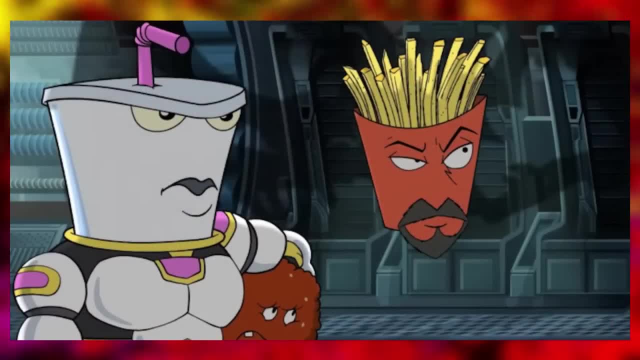 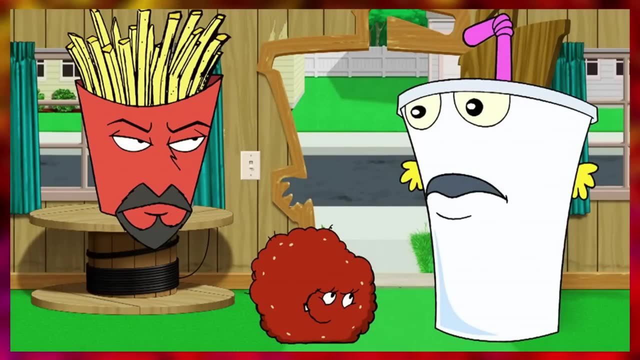 behind the show's many title changes was because he wanted media outlets to write about the show, which kinda worked. Not a Spinoff. Not a Spinoff. Aqua Teen Hunger Force has always been labeled as a spinoff of the classic show Space Ghost Coast to Coast. This is because during the days of Coast to Coast. 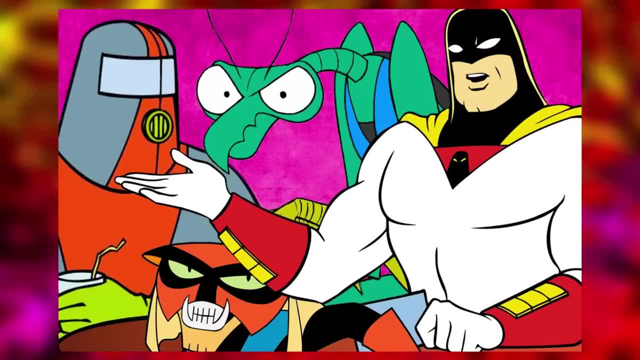 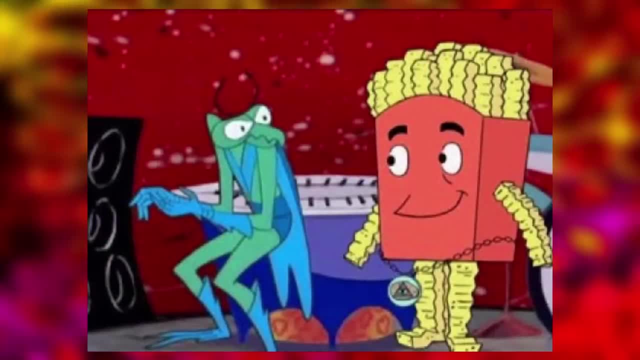 Dave and Matt, the creators of Aqua Teen, wrote an entire episode about Space Ghost not being able to pay a fast food restaurant bill. So the restaurant forced its mascots, the Aqua Teens, onto his show. The executives at the time were not huge fans of the episode idea. 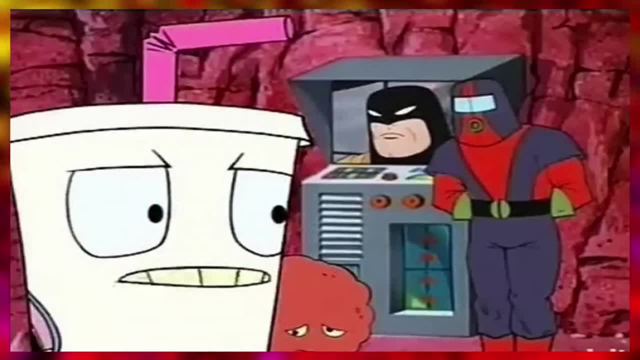 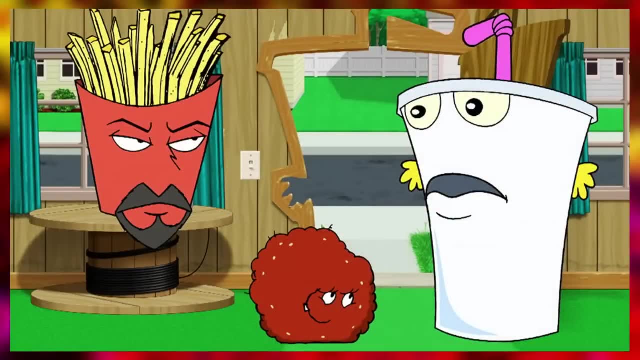 but during a production hiatus of Coast to Coast, Dave and Matt asked the network if they could create a pilot based on the newly created fast food characters. Thus, Aqua Teen Hunger Force was born. Eventually, the Space Ghost episode, Baffler Meal, was finally aired in 2003.. However, Aqua Teen isn't 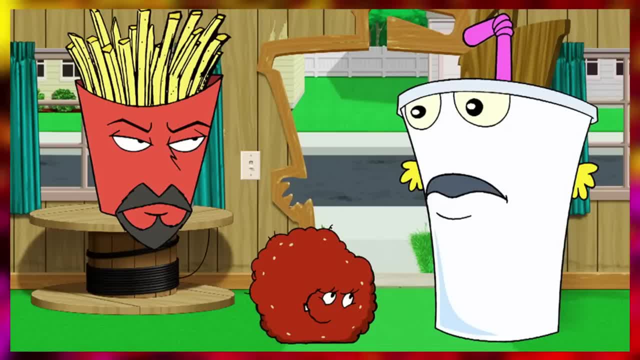 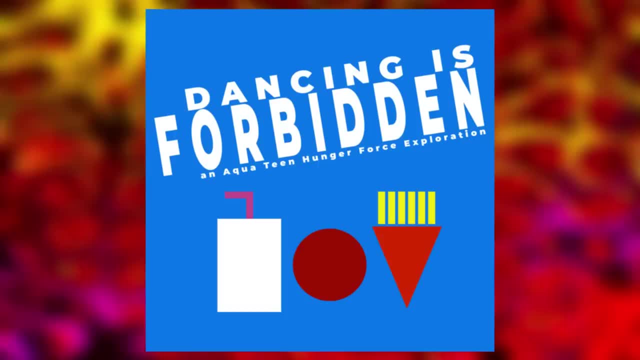 really a spinoff of Coast to Coast. I personally used to always consider Aqua Teen a spinoff, but after hearing Matt Malero and Ronnie, the host of the Dancing is Forbidden podcast, discuss why the series isn't, in fact, a real spinoff, I now understand why it isn't. 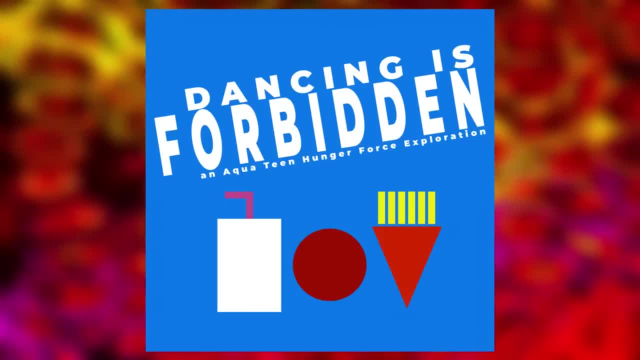 Credit to Ronnie for letting me use his podcast audio. by the way, I will probably refer to this episode of the Dancing is Forbidden podcast for a few enticing moments. reason this video. so shout out again to the amazing ronnie and his awesome podcast, which. 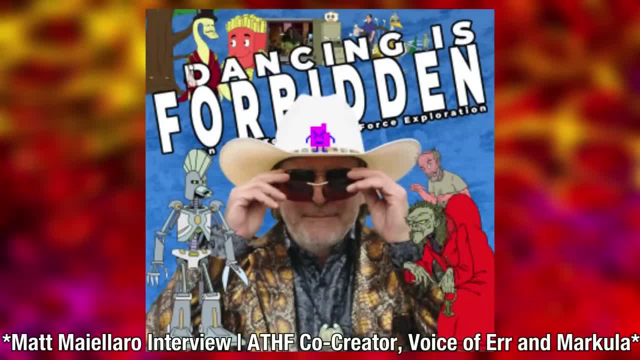 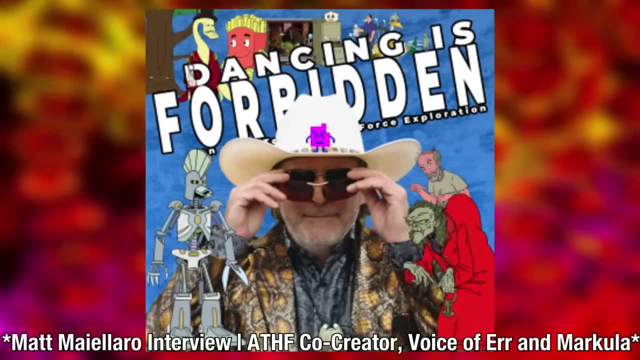 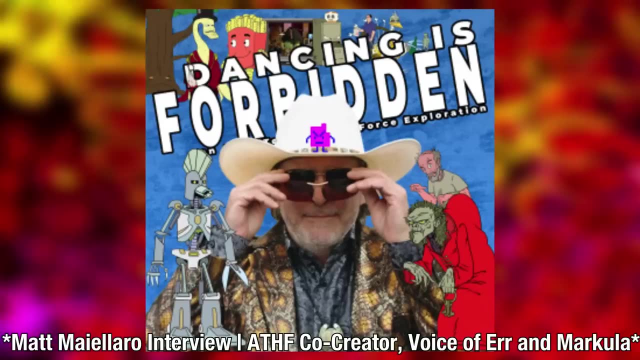 you should 100% check out. i don't know if you've heard this rumor, but i'd like to nip this one of the bud. but aqua team is not a spinoff from space ghost. right right, it never was, and i've seen it reported that way and it's totally its own thing. so right, yeah, yeah, it's like a spinoff from a. 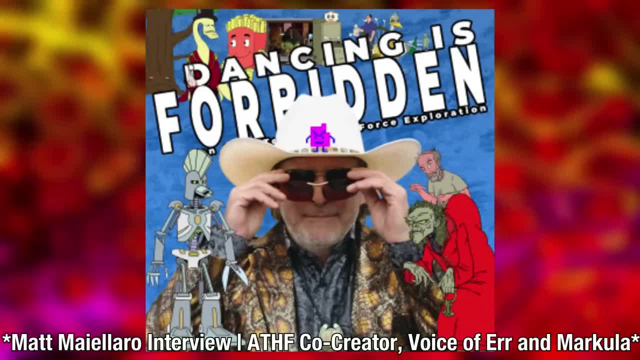 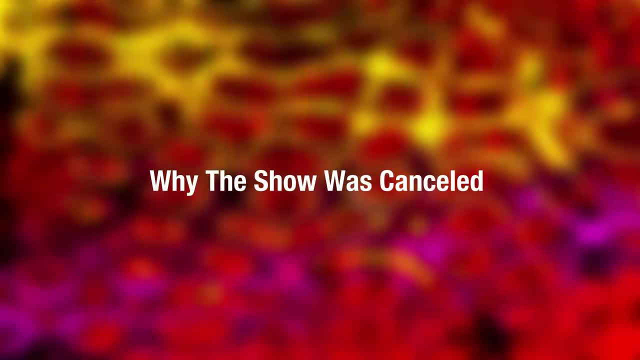 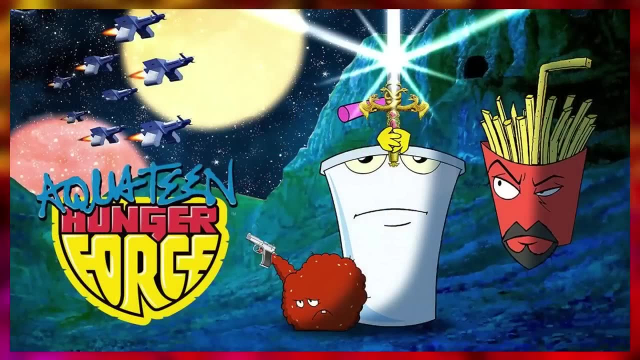 from a script that got rejected, but it's not like a real spinoff, something like the brack show where, like the characters were actually in space. yeah, right, why the show was canceled against the creators wishes. the series ended after season 11. the news broke midway through the production of 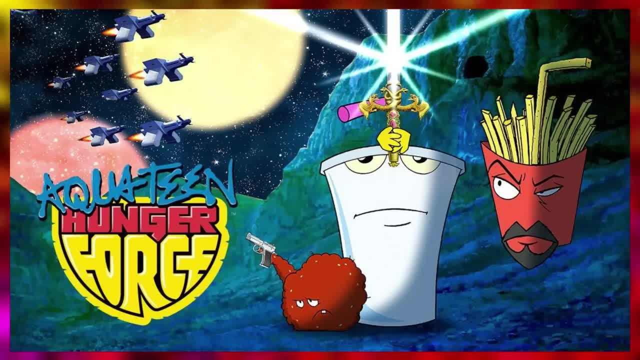 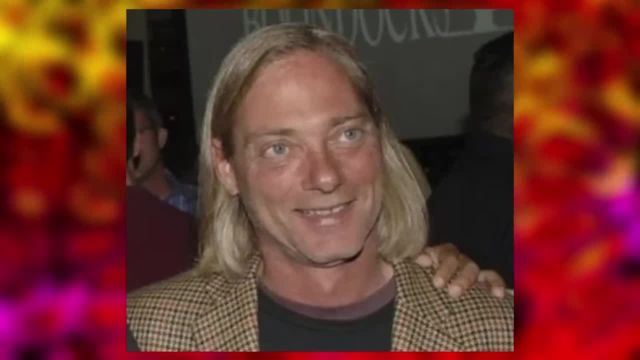 season 11, which, according to the creators, gave them enough time to create a proper finale. dave willis stated that former president of adult swim, mike lazzo, made the decision to end the series because he was ready to move on from it, even though the series had positive reception. it was. 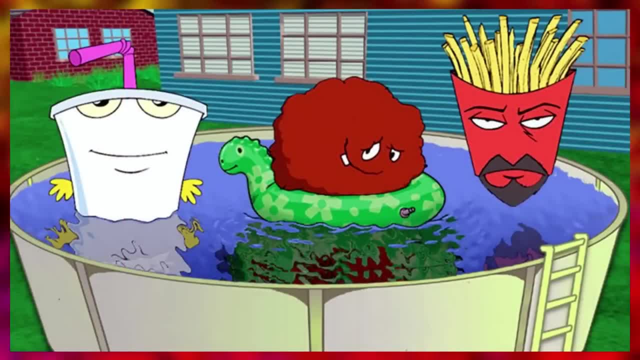 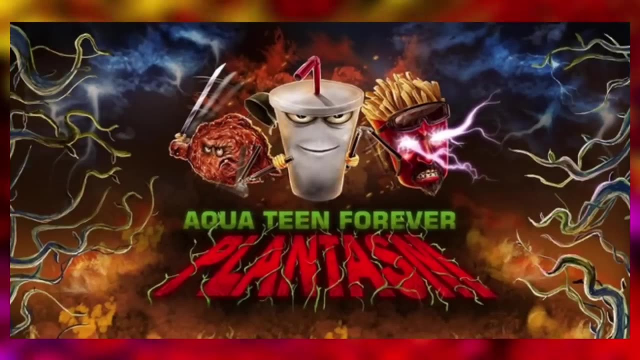 cheeky to make and generated a lot of freedom dollars. Mike Lazo was interested in giving new shows a chance on the network and did not want to continue making episodes of old shows. Plantasm, Aquatine Forever. Plantasm is the second full-length Aquatine Hunger Force movie, which 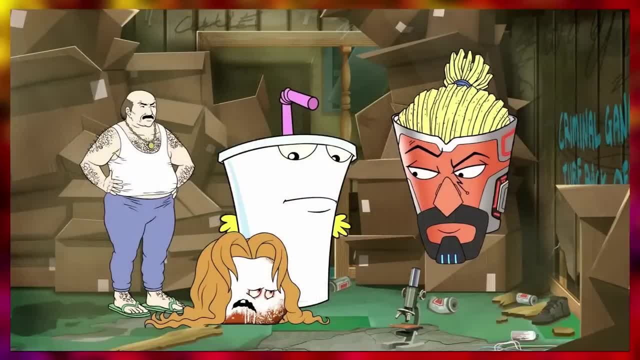 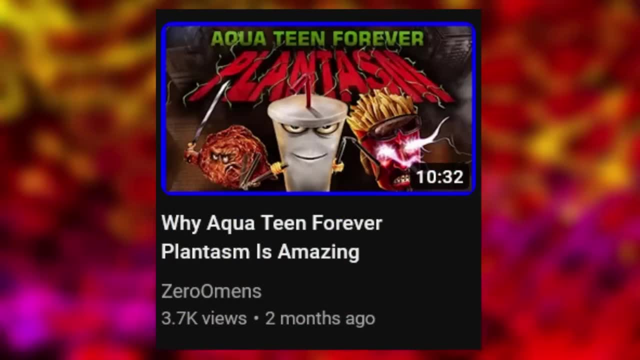 released on Blu-ray 4K and digital on November 8th 2022.. If you want to learn more about Plantasm and my personal thoughts on the film, then check out my Plantasm review video. I will try my. 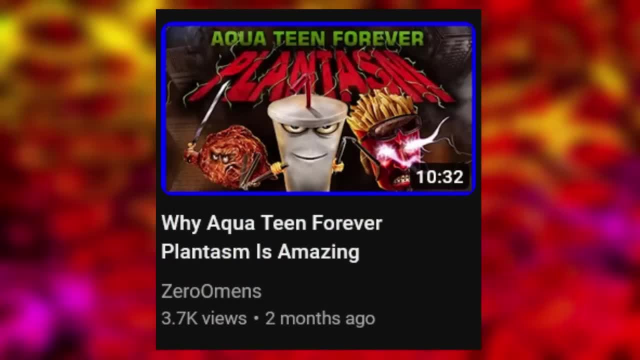 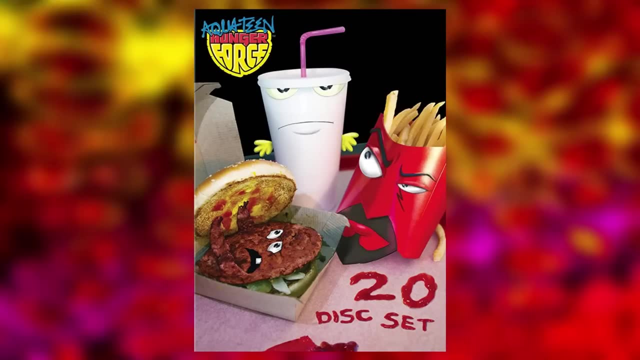 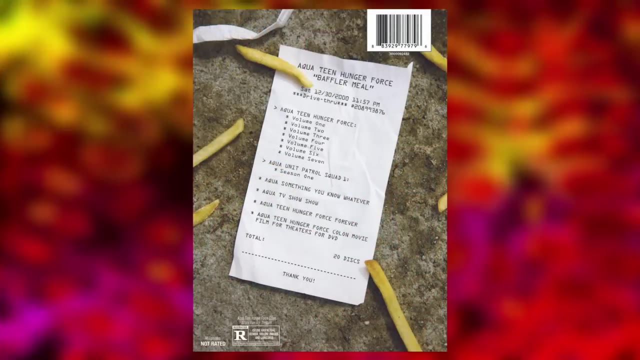 hardest to remember to leave a link to the video in the bio Baffler Meal Collection: Aquatine Hunger Force. The Baffler Meal Complete Collection is a giant 20-disc set containing almost every single Aquatine episode, loads of special features and even Aquatine Hunger Force colon movie film. 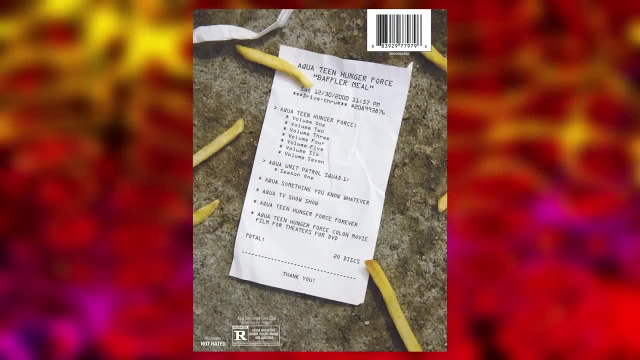 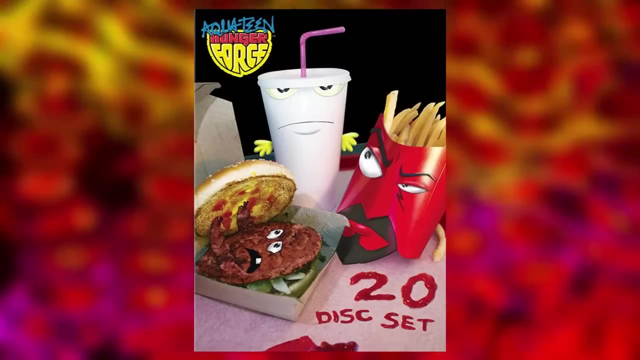 for theaters. The box set was released on September 20th 2022, and you, my friends, can play the role of Plantasm in the film. If you want to see more of the film, then purchase this massive piece of history for 82 Freedom Dollars, You know, unless Amazon decides. 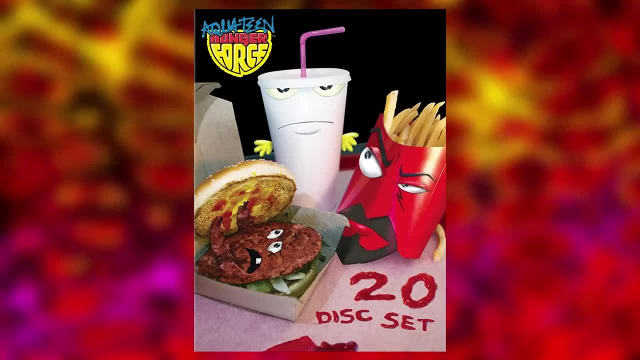 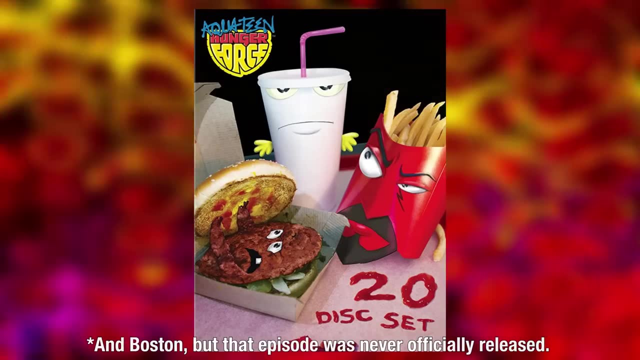 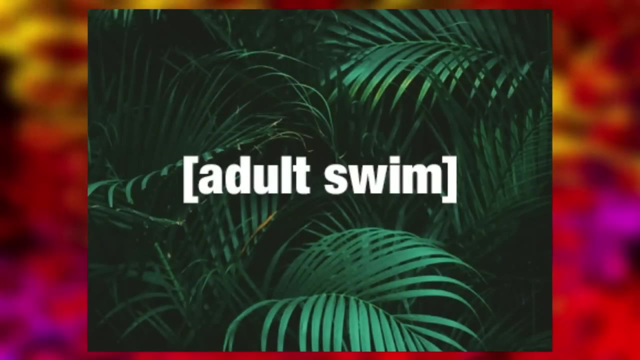 to update the price before the video releases, which is totally possible. The only episode not present in the box set is Shake Like Me, which we will discuss later on in the video April Fool's 2007.. On April 1st 2007,, Adult Swim promised to air the first Aquatine Hunger. 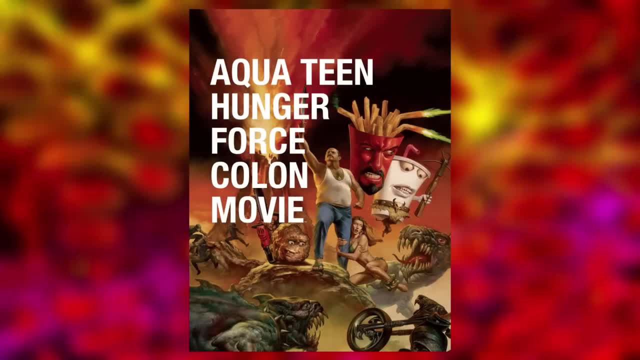 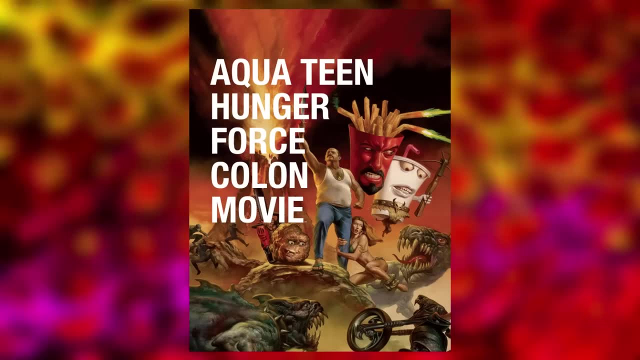 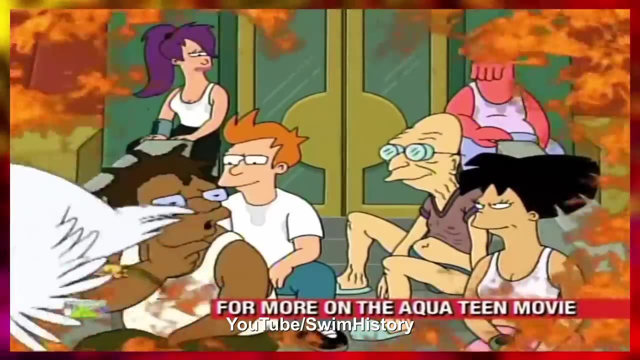 Force movie in its entirety before its theatrical release and, to everyone's surprise, Adult Swim stuck to their promise. They did play the entire movie but, uh, the first two minutes of the film played in full screen before the rest of the film was aired in a tiny one-by-one box in. 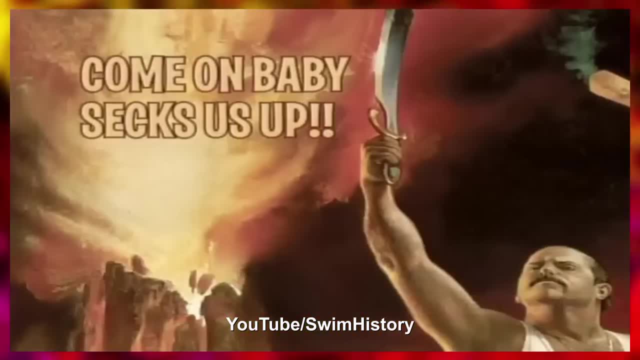 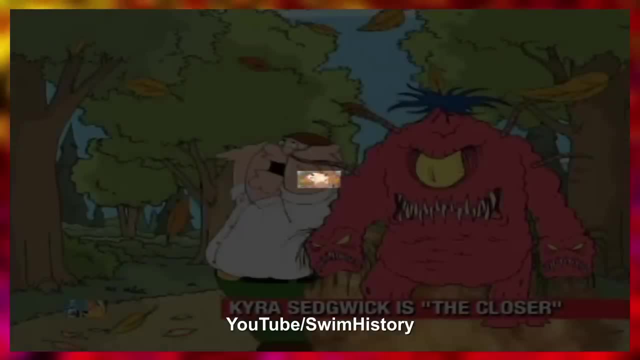 the bottom corner of the screen while the normal Adult Swim block played. So again, Adult Swim stuck to their promise of airing the entire movie. You just needed a f***ing magnifying glass to see the film. And let me tell you guys something: Seven-year-old me wasn't super happy after. 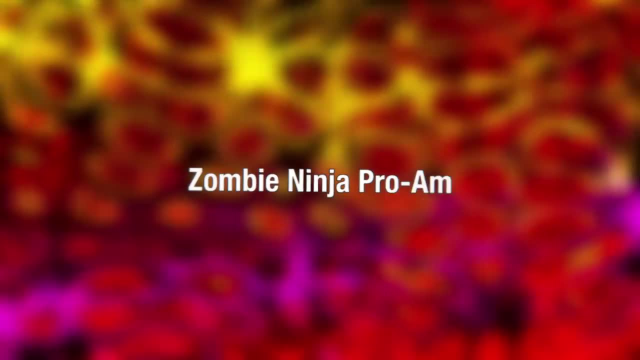 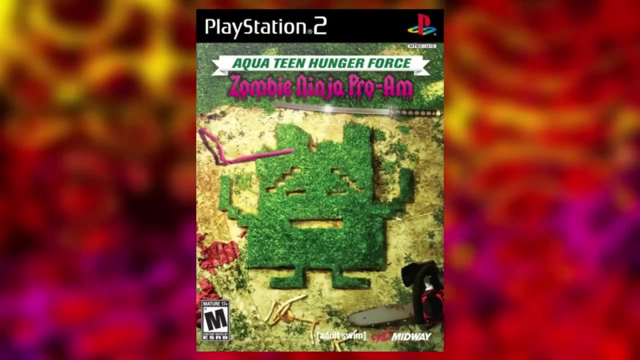 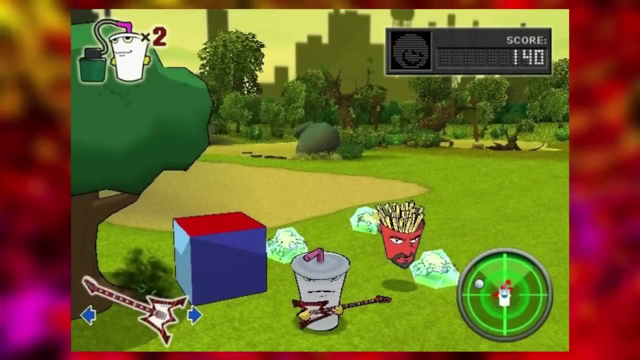 staying up late just to get punked. Zombie Ninja Pro-Am- Aquatine Hunger Force- Zombie Ninja Pro-Am is a PlayStation 2 exclusive video game titled, based on the Adult Swim series. It's a hybrid kart racing, fighting golf game that takes place across several New Jersey courses. The game released in North America on November 5th 2007,. 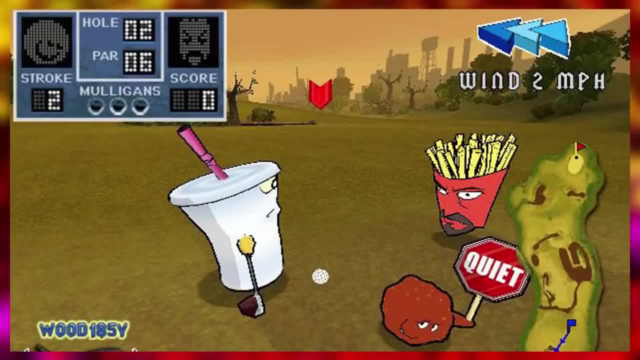 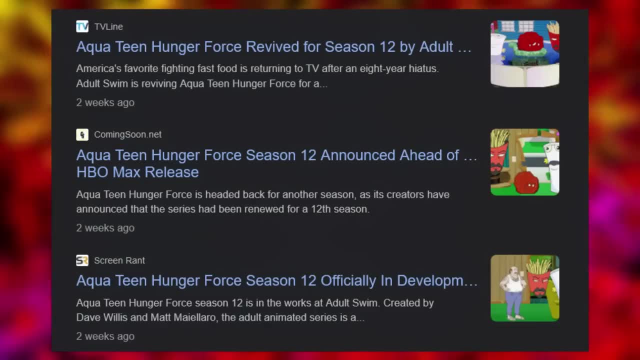 in Australia on November 15th and in Europe on November 16th, Season 12.. Recently, it had been announced that Aquatine Hunger Force, the series, would be resurrected for a 12th season consisting of five episodes. Yes, that's right, You heard me. 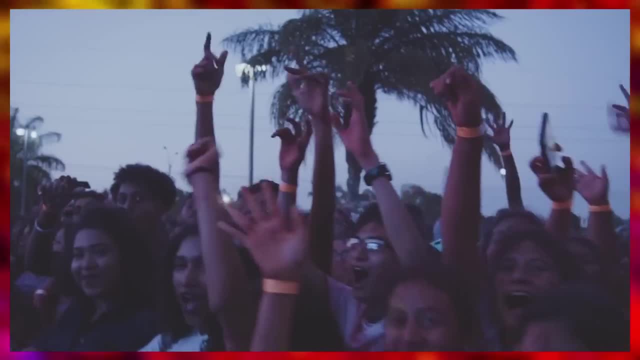 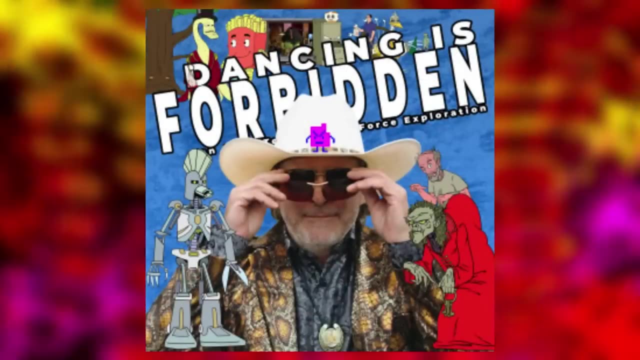 correctly. You may clap, You may clap. You may cheer, You may cry. However, this news isn't exactly new. information On the Dancing is Forbidden. podcast episode featuring Matt Malero: it was revealed that five new Aquatines were ordered. 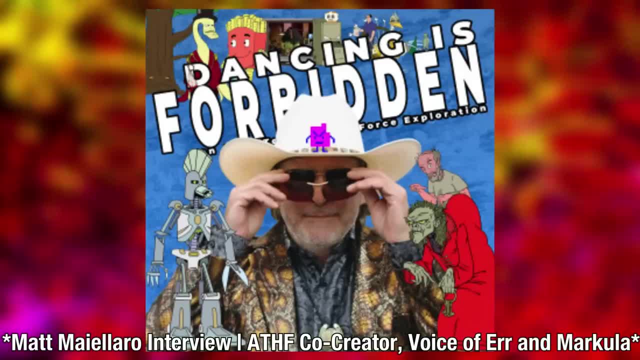 Well, did you know? we're doing five new ones right now? Five new ones, Yeah. Five new Aquatines, Yeah, And so we almost brought it back. No, you're not. You're f***ing wrong With me. 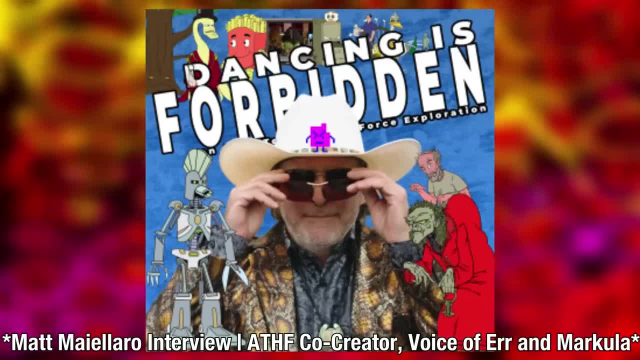 I'm not man. In fact, as soon as I'm done with you, I'm getting back on with Dave. We're wrapping up the first script. so Oh, wow, Yeah, I'm serious. They ordered five more. 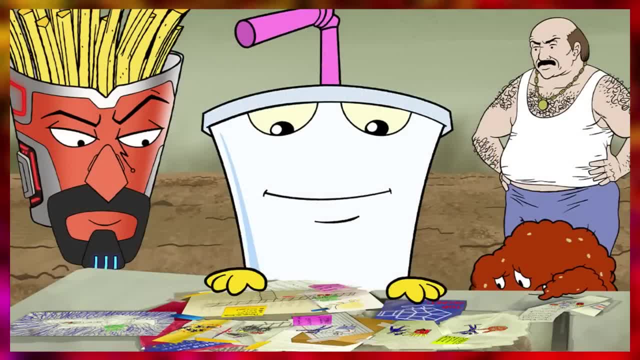 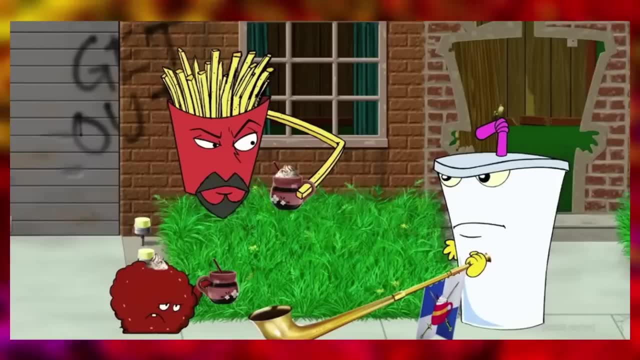 Now there is no word on when exactly we will receive season 12 of Aquatine, but if I had to make an educated guess, I would say towards the end of 2023, probably in the fall, but we'll see what happens. Either way, let us rejoice. 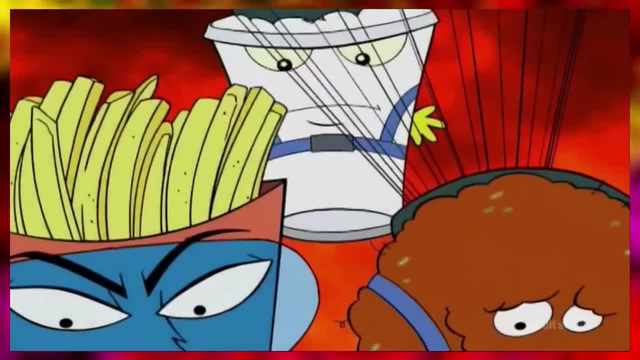 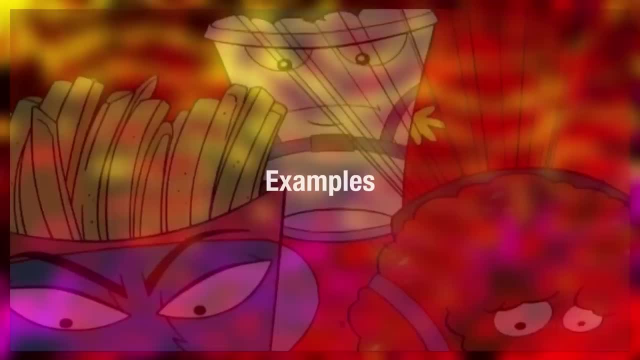 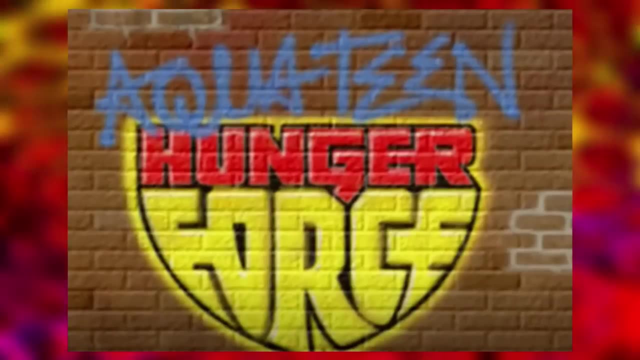 Opening intro sound effect. In most episodes of Aquatine between seasons one and seven, there is a little sound effect that plays right at the end of the opening credits, before the episode starts. Well, as it turns out, Matt Dave and sometimes their sound designer would pick out funny sound. 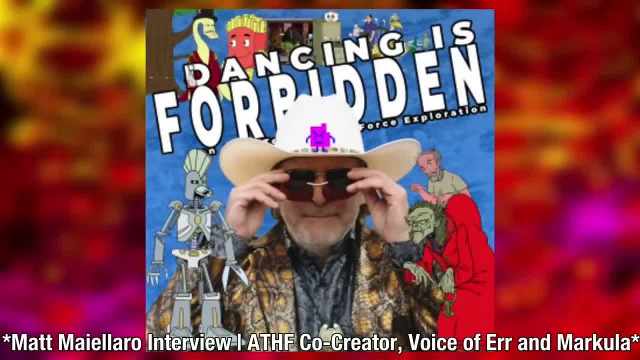 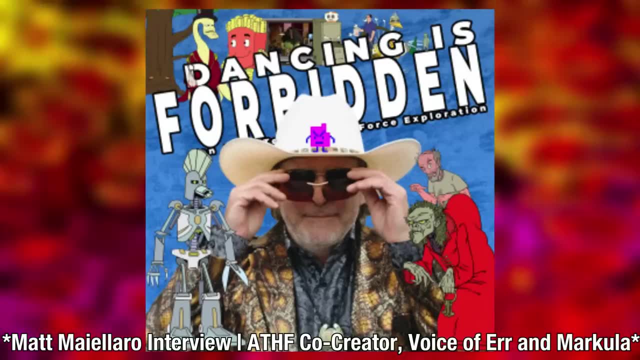 effects and add it to the end of the opening credits. Sometimes I would say, what if it were this? And then we'd agree, And sometimes it was just, you know, different. It was either me or Dave, And then we would just agree on what it should be. 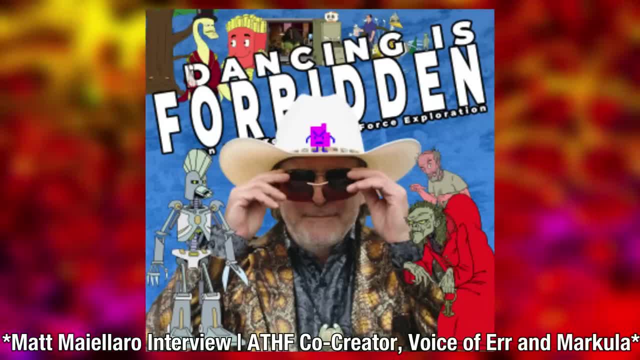 Sometimes it was our sound designer. What if you know? I was like: yeah, that's funny, And Dave was like: yeah, I like it too, So it would stay Again. shout out to Ronnie for allowing me permission to use. 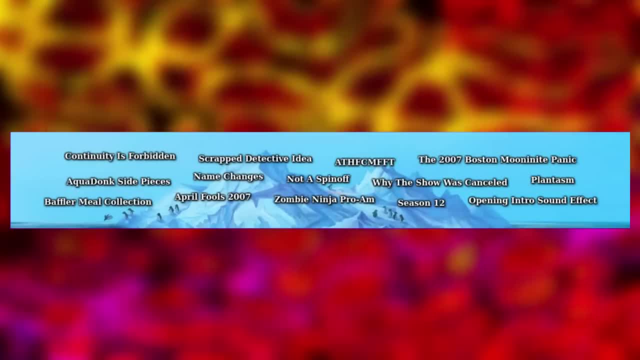 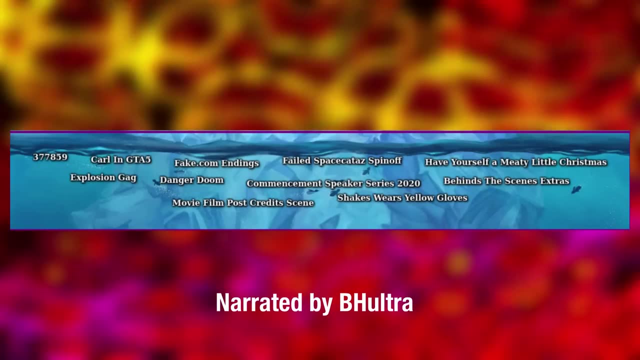 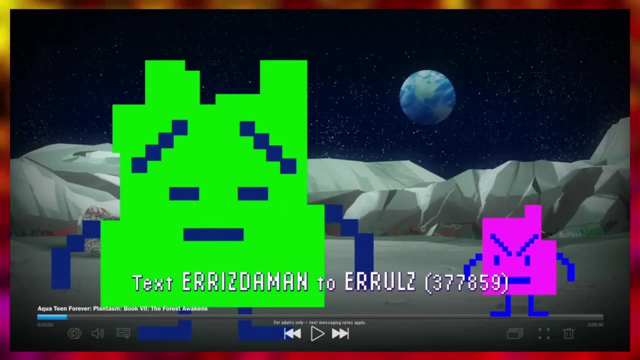 some audio from his episode with Matt Malero. And that, my friends, was the first layer of the iceberg, Layer two: 377859.. During the Fruits Moonanite segment of the newest Aquatine movie, Aquatine Forever, Plantasm, Ignig, Nott and Ur appear on screen threatening to destroy the film. 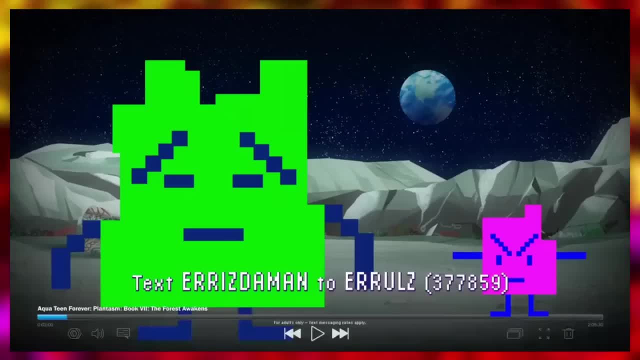 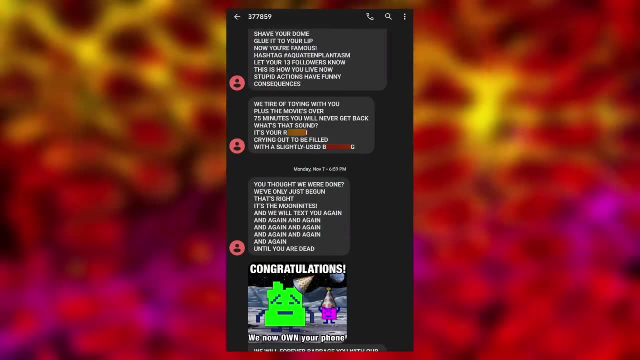 unless the viewer texts: ur is demand to ur rules 377859.. If you do try and text this number, you will be bombarded with spam messages from the Moonanites themselves. Participants receive messages filled with memes, threats and even spoiling the ending of the film. 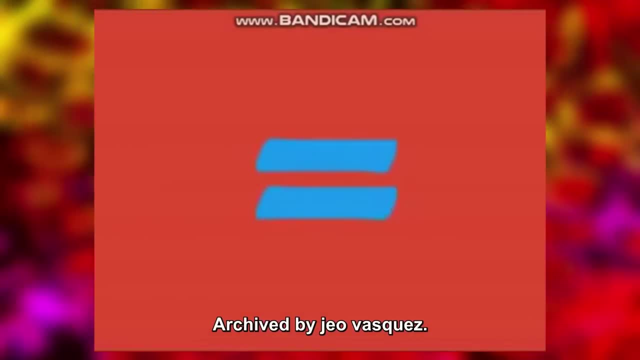 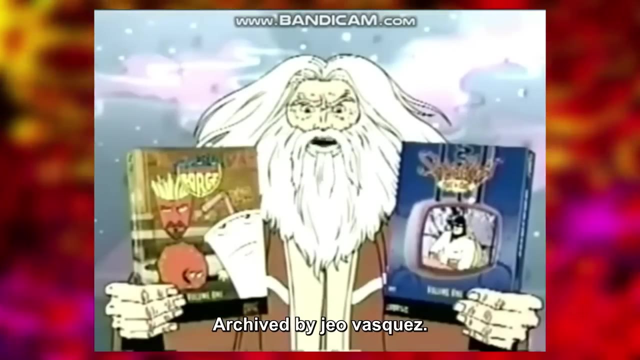 Bumpers. It wouldn't be an Adult Swim related iceberg without mentioning the endless amounts of bumpers, promos and commercials displayed on the block throughout the years. However, due to my state-sanctioned parole, I'm only allowed here for a certain amount of time. 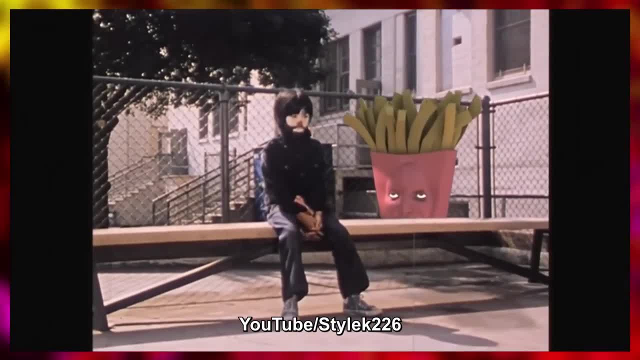 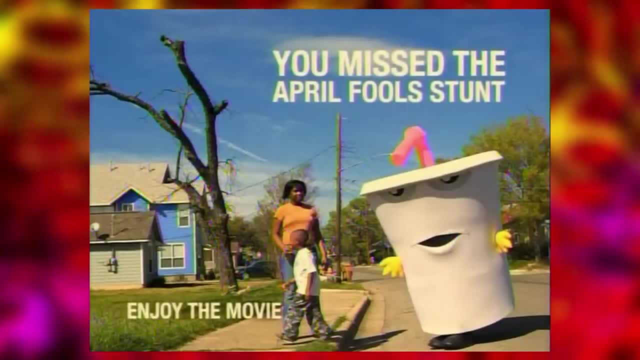 so we'll just cover the important ones for now. Plus, there's a chance that some Aquatine bumps were never properly archived and are now forever lost to the endless void. But it wouldn't hurt to mention some very notable bumps from the history that are archived: The La Samba de Saint. 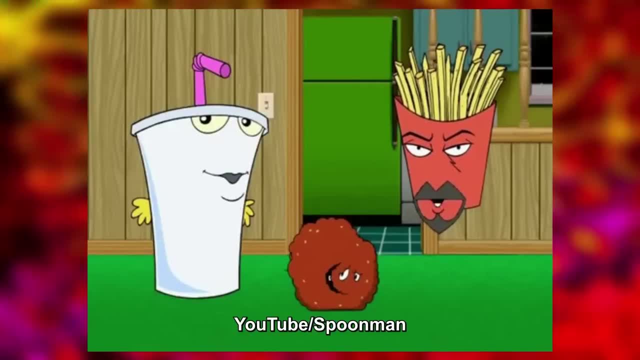 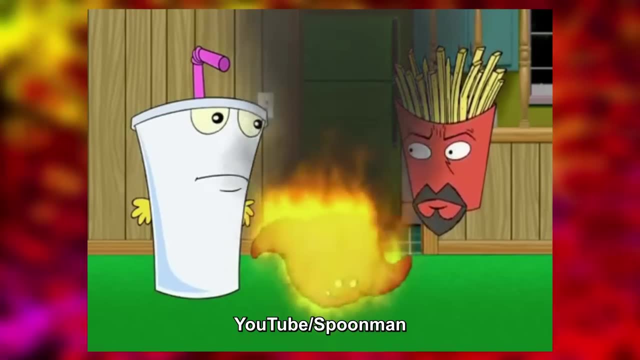 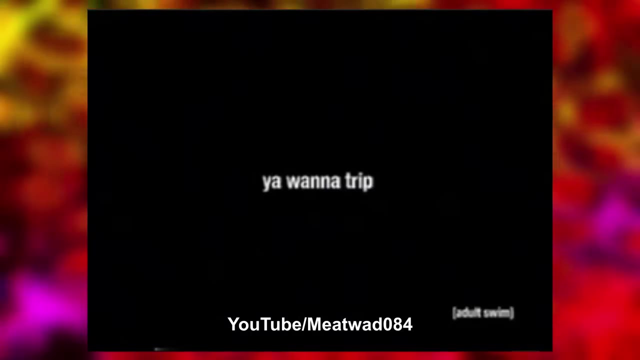 Germain bump which features the Aquatines lip-syncing to the La Samba song as Meatwad spontaneously bursts into flames. The Adult Swim Aquatine Hunger Force theme lyric bump which, just like it sounds, is the official lyrics to the theme song used in the first. 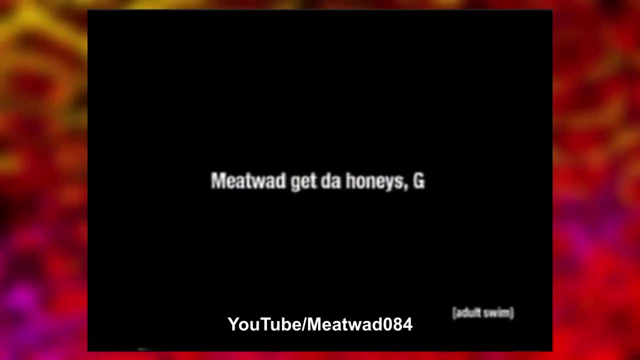 seven seasons of the show performed by Schoolie D And I'm glad this exists because, honestly, for years I thought the line was ice on my fingers and my toes and on my toys, because Meatwad is a little kid and plays with toys a lot in the series, whether they be made of trash or not. 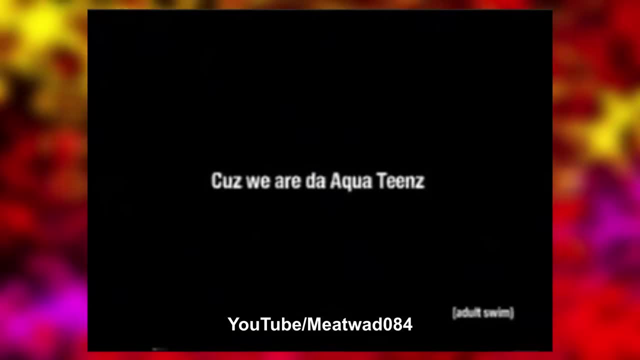 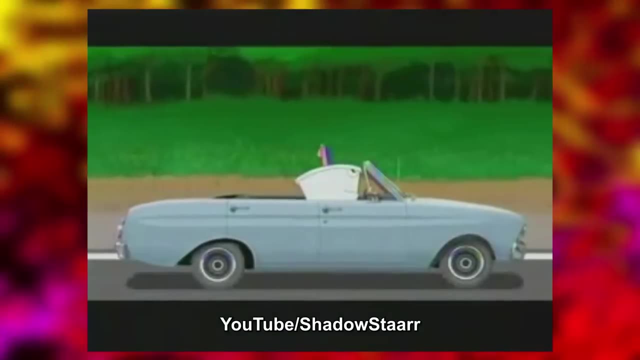 But the line is actually ice on my fingers and my toes and I'm a Taurus because Schoolie D did not know anything about the show show before they had him do this theme, The Aqua Teen Hunger Force, is cancelled. commercials which shows Frylock, Meatwad and Shake individually. drive a convertible into a. 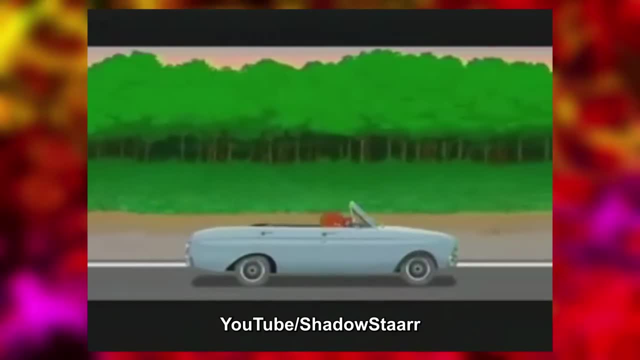 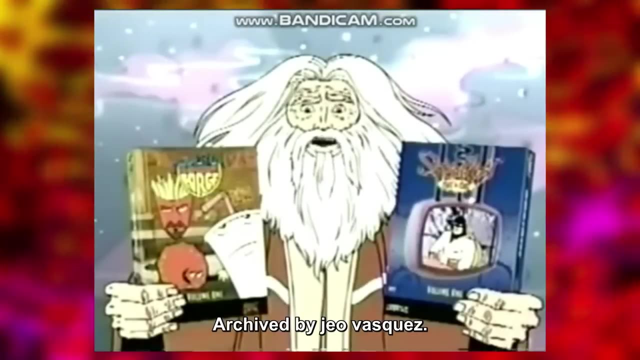 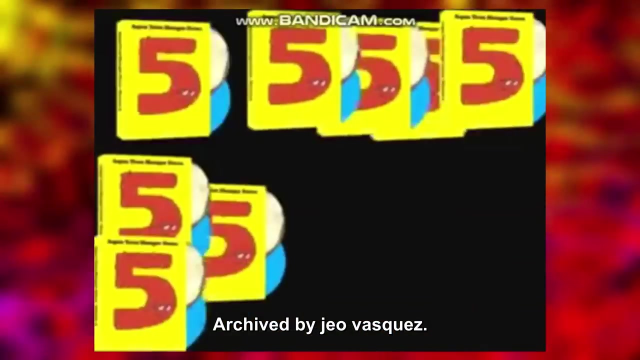 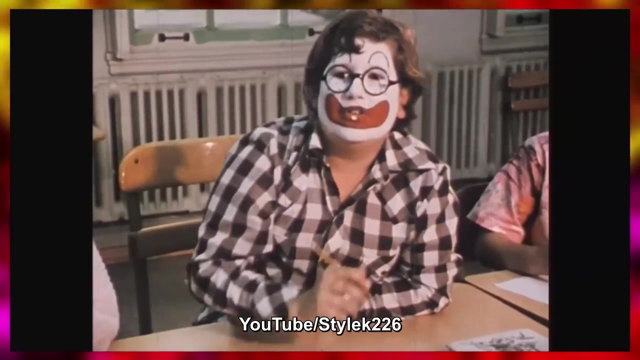 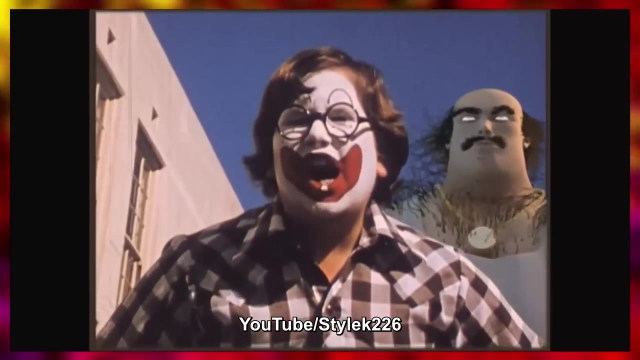 tractor trailer and explode, with Carl ending the bump by saying- and now there is one- before exploding himself. The Aqua Teen DVD commercials, which there are many of: The Clown Kid Bumps featuring 3D animated Aqua Teen characters. If you don't know, The Clown Kid Bumps were clips taken from the 1976 film If Mirrors Could Speak. 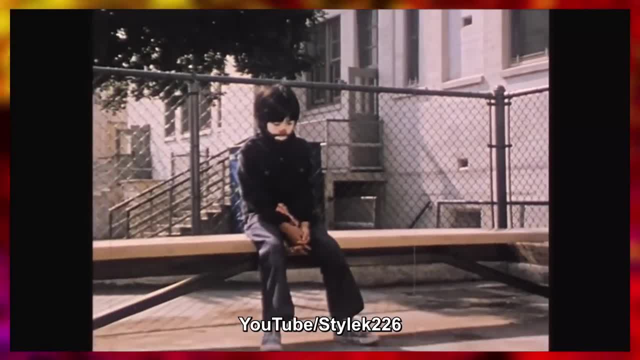 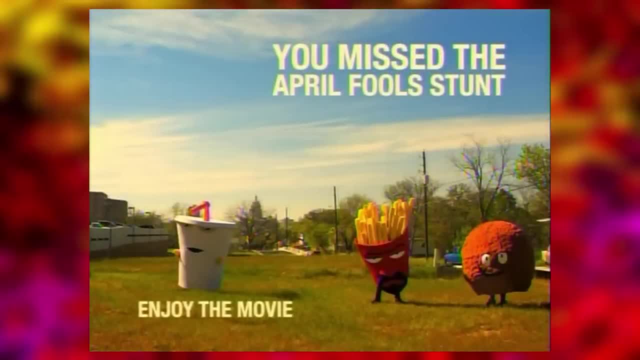 with eerie music and nightmare fuel 3D models of various Adult Swim characters that would air from time to time. They didn't make these Clown Kids. this is actually what the movie is. There are also a colossal ton of movie film for theater bumpers and 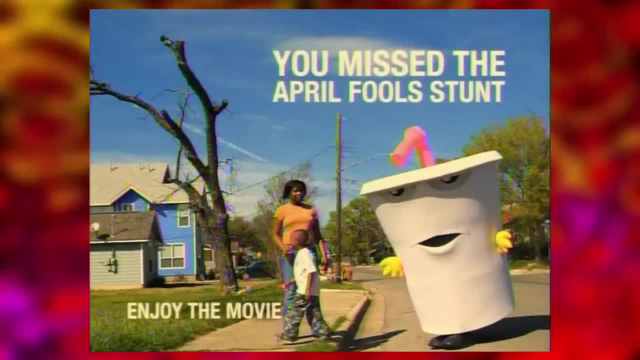 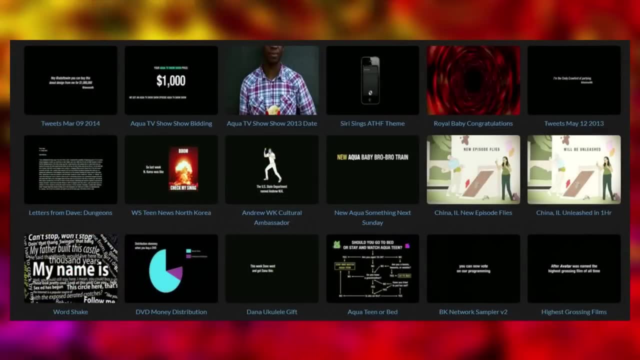 promos as well. But if you're curious and want to watch more Aqua Teen bumpers, commercials and promos for yourself, then check out Bumpworthycom, as they have an incredible catalog of archived bumpers not just from Aqua Teen, but a ton of other Adult Swim. 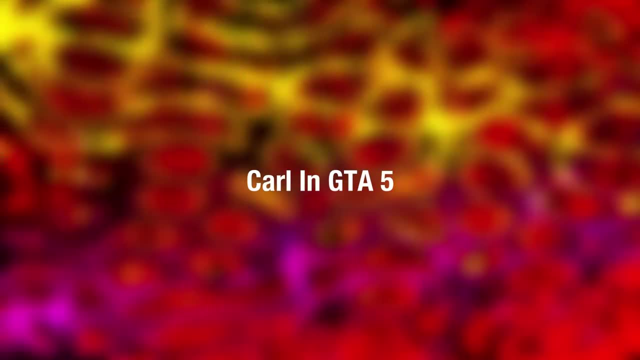 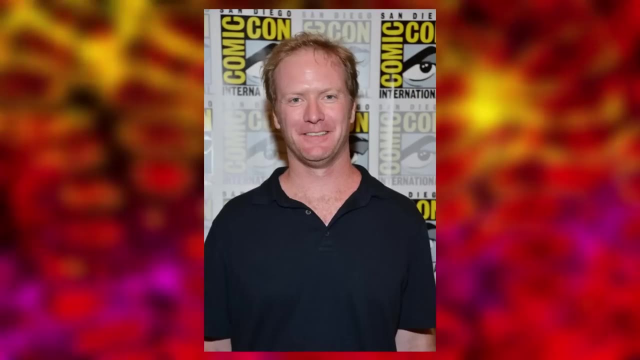 properties Carl in GTA 5. In Grand Theft Auto V, Dave Willis, the voice of Carl from Aqua Teen, makes a small voice cameo on the Fly Low FM radio station in the Carl voice, using the same cadence to imply that it is Carl. 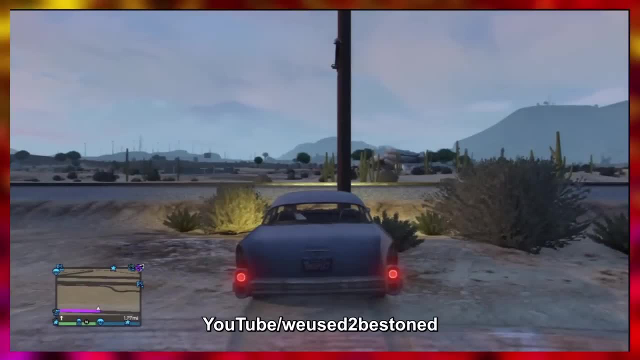 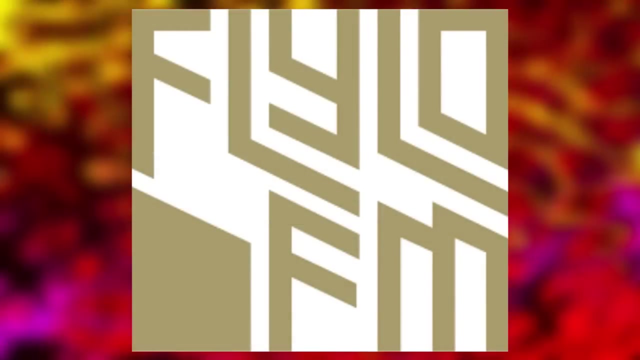 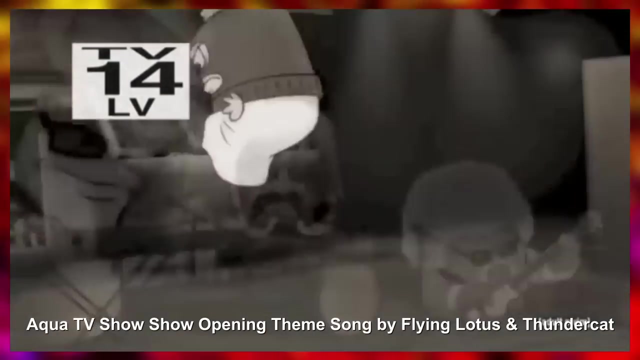 himself. It's worth noting that the station he calls into Fly Low FM is hosted by the artist Flying Lotus, who has collaborated with Adult Swim multiple times in the past. Seriously, if you look up some classic Adult Swim bumps right now, a good portion of them have beats produced by Flying Lotus playing. in them, most famously during the game. If you're interested in learning more about the game, check out Bumpworthycom, as they have an incredible catalog of archived bumpers, commercials and promos for yourself, including a ton of other Adult Swim properties. 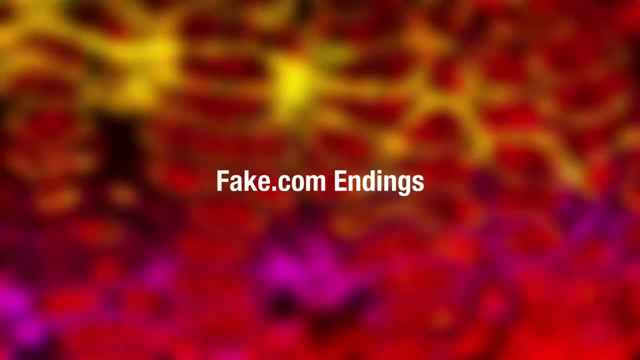 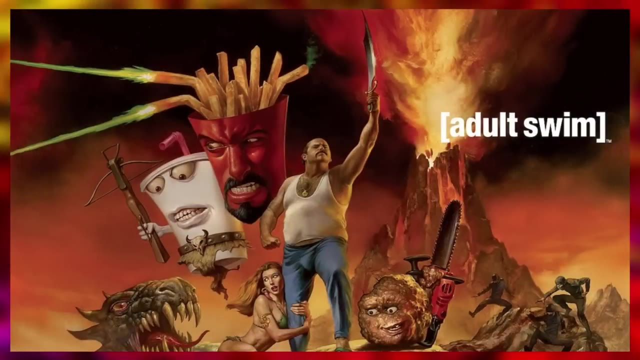 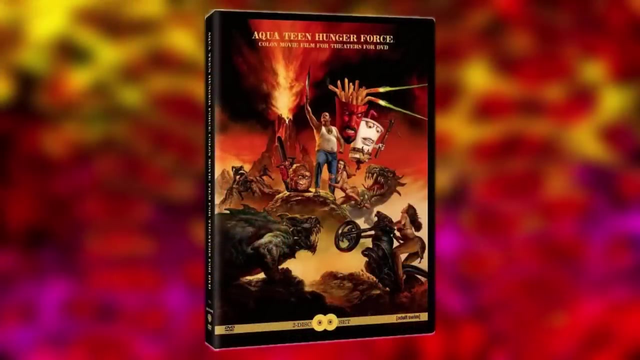 Fakecom Endings. During the promotional period for Aqua Teen, Hunger Force- Colon Movie Film for Theaters, the creators and network released 10 fake movie endings on different websites and some hidden at the end of Flash Games as a reward. These fakecom endings are also available in their entirety on the second disc of the film's DVD. 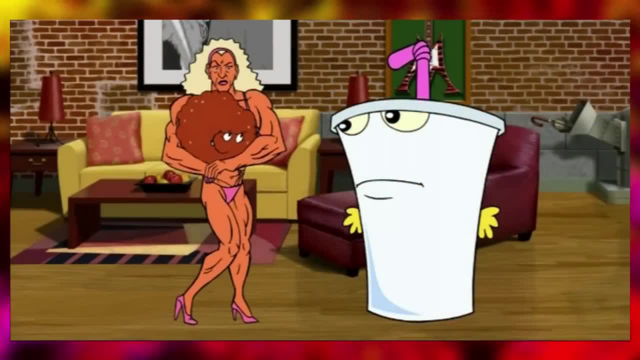 And we're going to cover some of those endings. Dr Zod- Ending This ending- starts mid-conversation with Meatwad explaining to Shake that because he was created by the evil Dr Zod, he isn't programmed to feel emotions. Shake reminds. 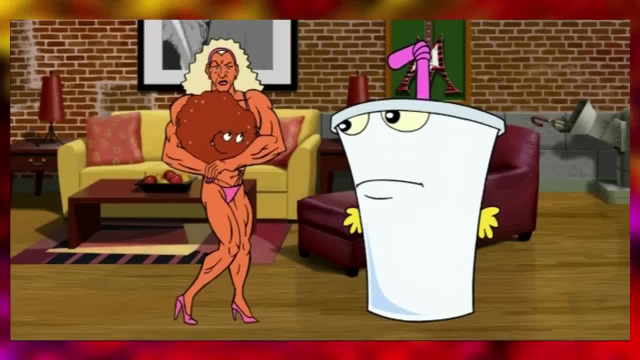 him that he's marrying the woman he's being held by, Linda, or Dr Weird, in disguise from the movie Meatwad, proclaims that he doesn't care and loves her anyway, but also that now he's gots to kill her as he pulls out a gun. 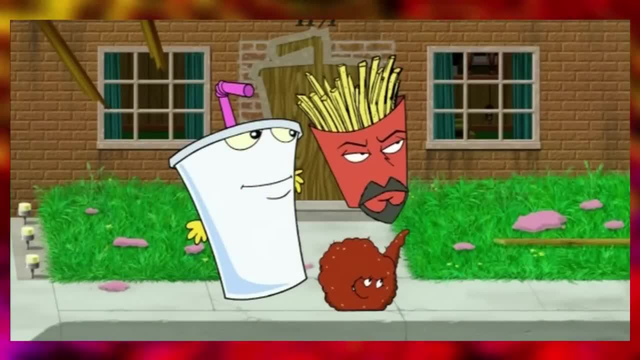 The Wonder Man Ending. This ending shows Shake, Frylock and Meatwad waving goodbye to a faceless hero named Wonder Man after he saves the planet. However, the Aqua Teens would never see or hear from him again because, according to narrator George Lowe, Wonder Man was arrested for m***ing a child in another galaxy. 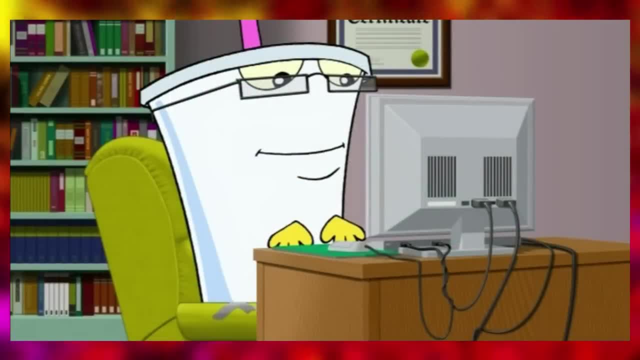 Blood Mountain Ending. The Blood Mountain Ending is a parody of the ending of the movie Stand By Me. It shows Shake typing on Frylock's computer about his visit to Blood Mountain, where four people named Gordo, BJ, Doogie and The Blimp all lost their 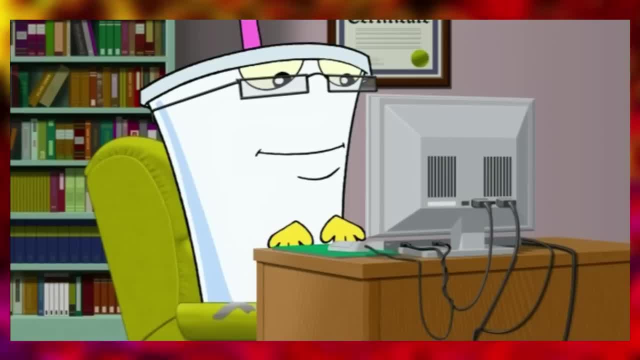 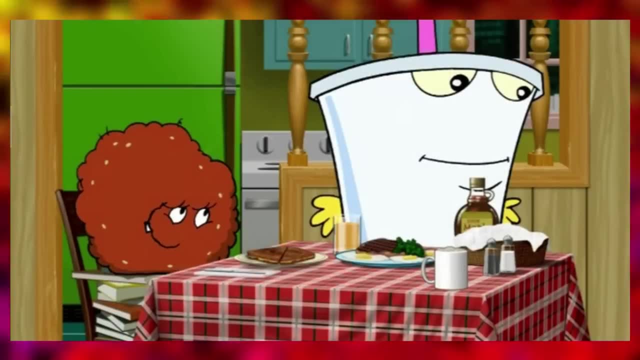 virginities that summer, only to be eaten by DC Comics' Swamp Thing, who just so happened to be filming their s***ful intercourse with a new photosynthetic camera. Sandwich Ending In the Sandwich Ending Shake enters the living room with some sandwiches and Meatwad says: 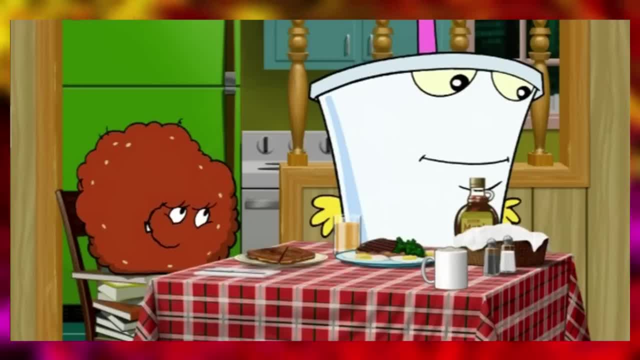 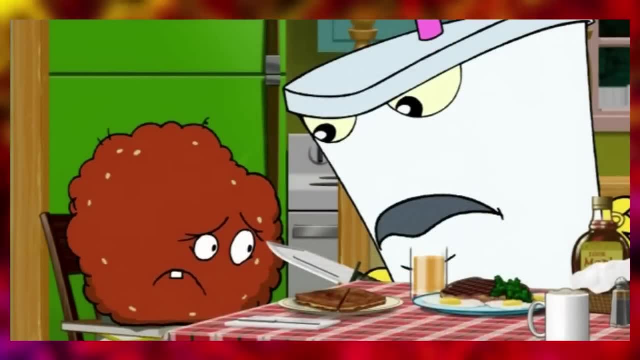 God bless- I can't do the voice. God bless us everyone. as the music swells and the movie fades out: Sandwich Jewels Ending. The Sandwich Jewels Ending follows the same path as the original Sandwich Ending. However, after Meatwad says God bless us everyone, he proclaims that he is allergic to bologna. 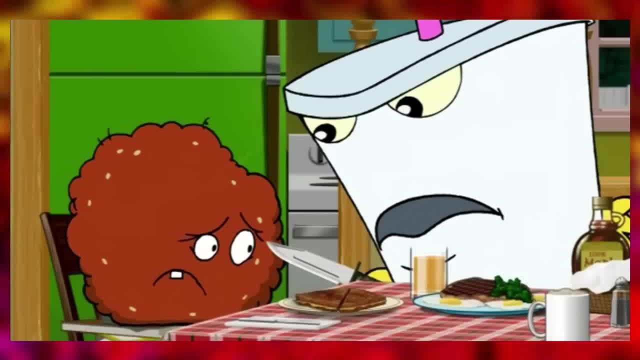 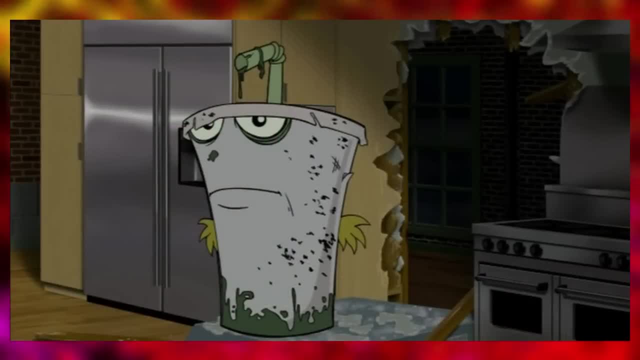 and calls out Shake for it. Shake then holds a knife directly at Meatwad and commands him to give up the jewels. Zombie Shake Ending In this ending after shooting a horde of off-screen zombies: Freilach and Meatwad question. 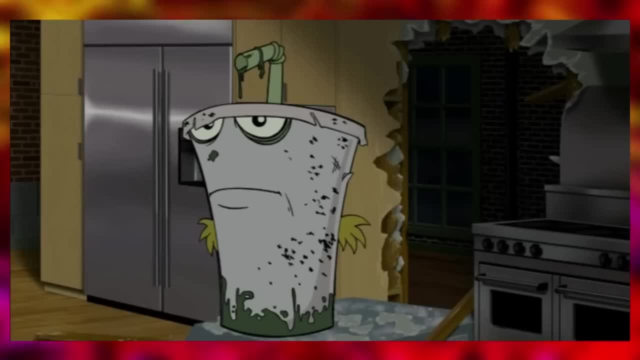 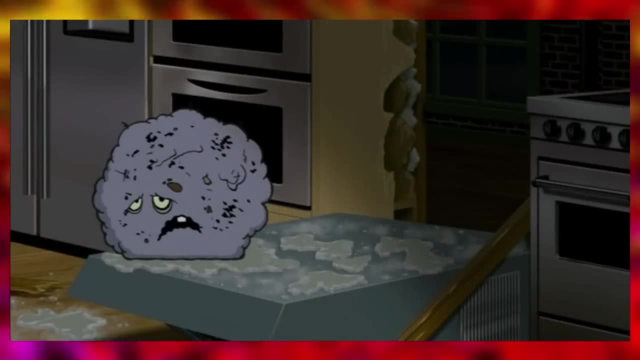 the whereabouts of Shake. In a shocking twist, Shake enters the room from the right as a zombie Zombie Meatwad Ending. This ending is pretty much the same as the Zombie Shake Ending. however, Shake and Meatwad's roles are flipped. Meatwad also sings Twinkle Twinkle Little Star before. 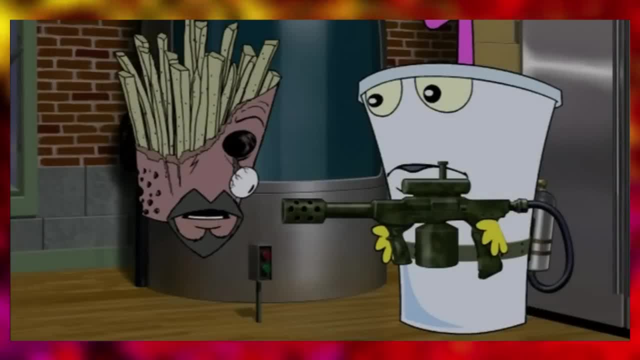 letting out a horrifying growl: Zombie Freilach Ending. Once again, Shake and Freilach are slaying a bunch of off-screen zombies. Once the fight is over, Shake congratulates Freilach who, in another shocking twist, is actually a zombie. 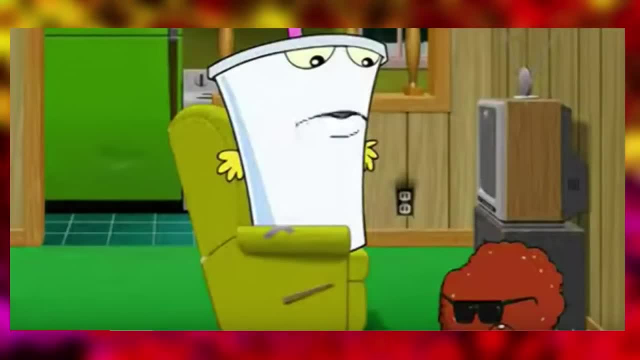 Determinator Ending In this ending. Shake is watching television in the living room until Meatwad teleports into the room demanding a motorcycle, boots and clothes. When Shake explains that he doesn't own any of those items, he gets shot in the face, If it wasn't obvious enough already. 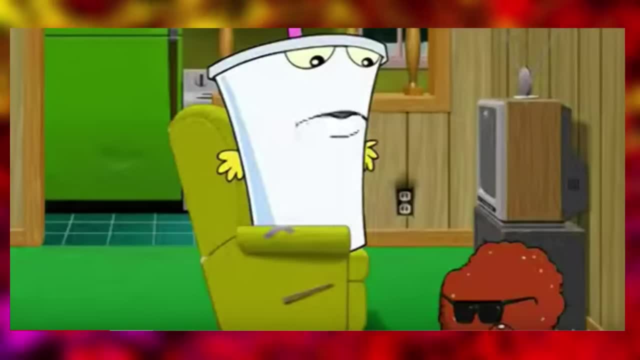 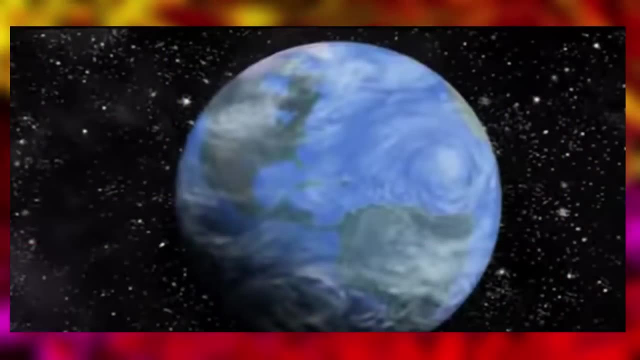 the Determinator Ending is supposed to be a parody of the Terminator franchise Earth Ending. This last fake ending shows Earth with Shake narrating off-screen about how the planet's resources are so precious to humanity and that we're running out The ending. 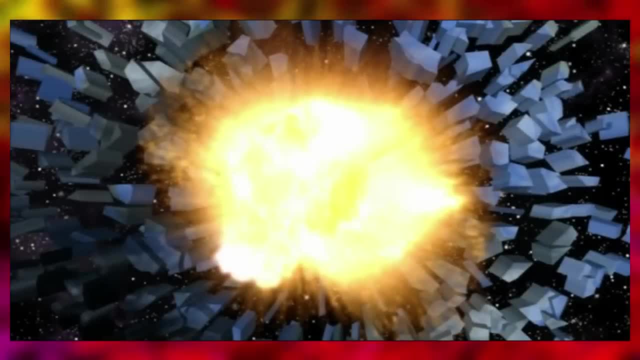 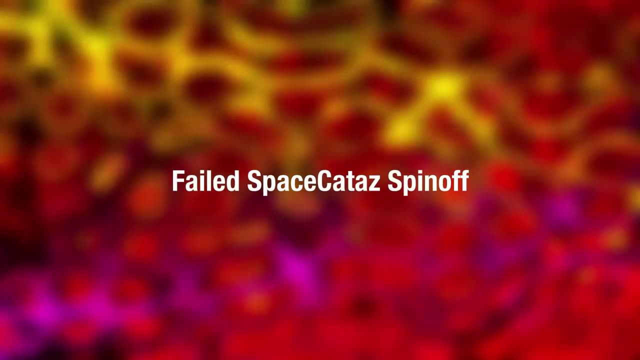 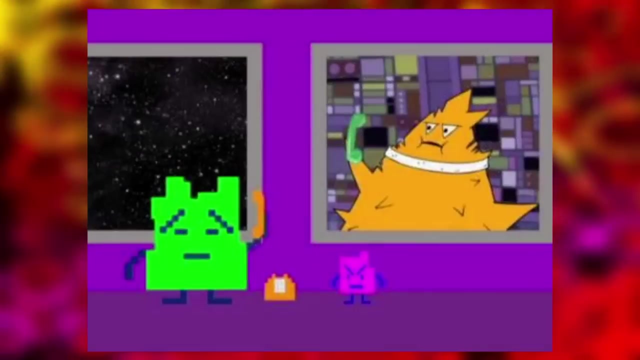 concludes with Shake commanding the viewers that the next time they fill up their car's gas tank, just don't. It's that simple. Followed by the Earth exploding. Failed Space Cataz Spinoff. Space Cataz is a failed spinoff of Aqua Teen Hunger Force, centered around an ongoing feud between the Moonenites and Plutonians. 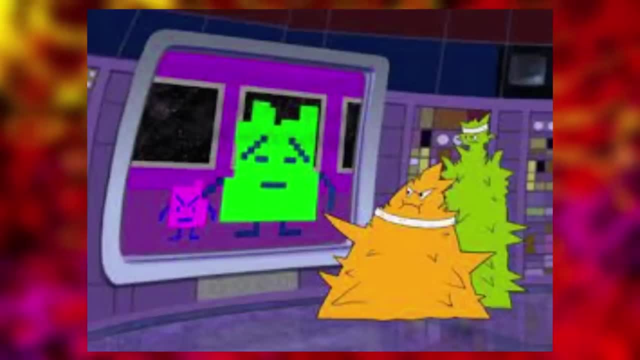 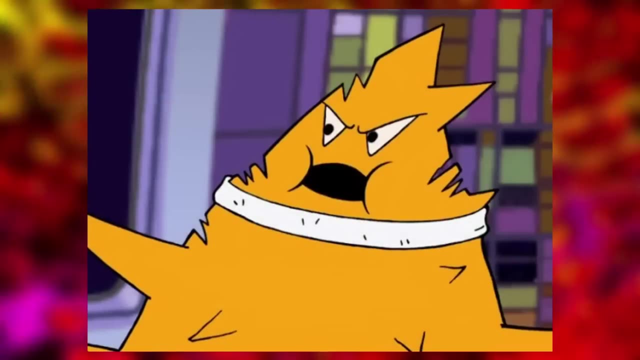 The project was cancelled because Adult Swim felt there was little, if anything, that could be done with the characters. So, instead of becoming its own series, the failed 10-minute pilot for the show was split up and included at the beginning of every episode of Season 3 of Aqua Teen, replacing the Dr Weird and Steve cult openings from the 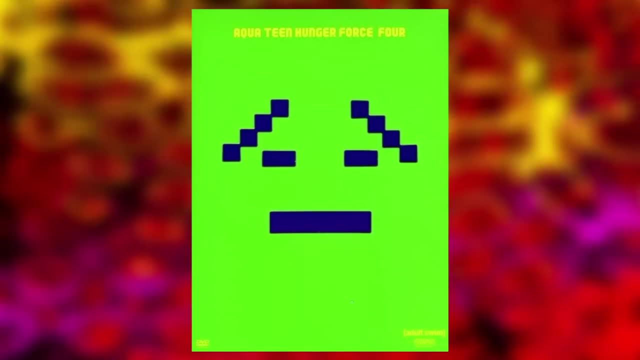 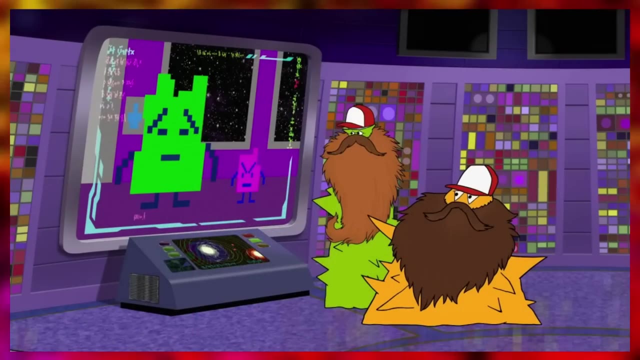 seasons prior. The full episode is available as an extra on Disc 2 of the Volume 4 DVD box set and the Baffler Meal set as well. It's worth mentioning that, although Space Caduce is not part of that spinoff, it was created in spirit of that idea. 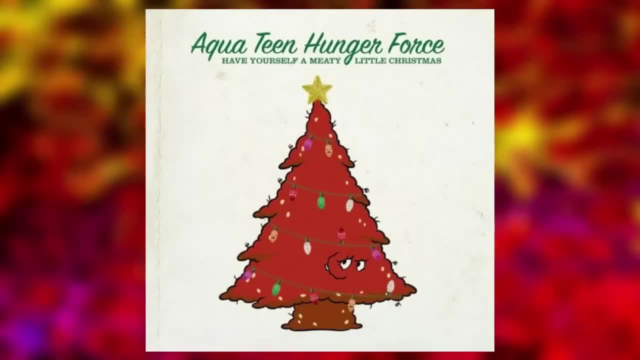 Have Yourself a Meaty Little Christmas. Have Yourself a Meaty Little Christmas is an Aqua Teen Christmas album, which released in the late 90s and early 90s. It's an album that's been released on November 3rd 2009, and features such classics as Feliz Navidad, Hark, The Herald. 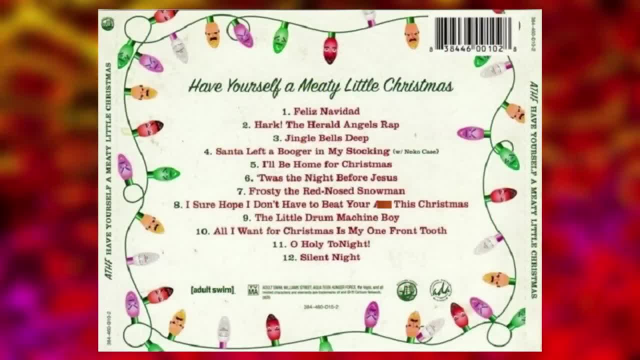 Angels Rap, Jingle Bells. Deep Santa Left a Booger in My Stocking. I'll Be Home for Christmas. Twas the Night Before Jesus Frosty the Red Nosed Snowman. I Sure Hope I Don't Have to Beat Your Ass This Christmas. The Little Drum Machine Boy, All I Want for Christmas is My One. 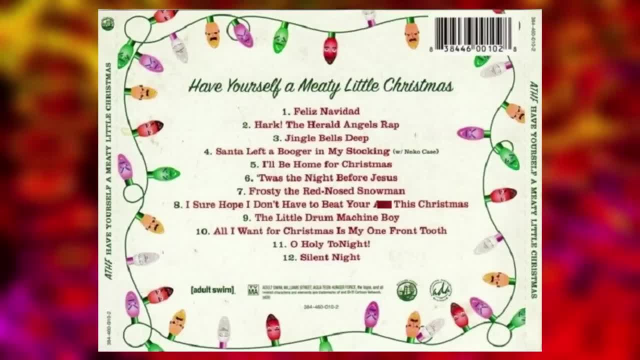 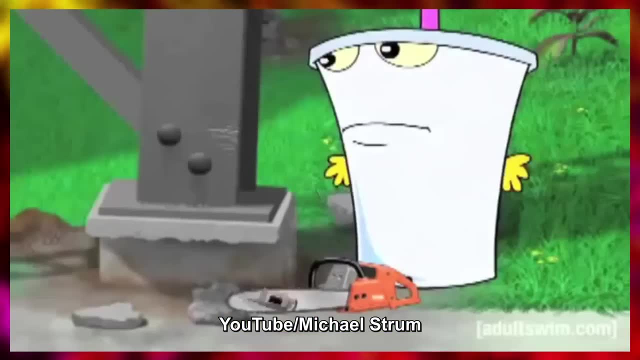 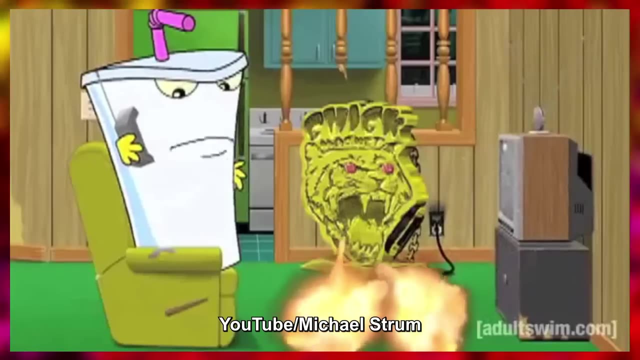 Front Tooth. Oh Holy, Tonight, Silent Night, and I'll Be Home the Day After Christmas. Explosion Gag. The Explosion Gag refers to how items like a TV remote randomly explode whenever a character throws them to the ground. Despite the lack of continuity in the series, some fans believe that 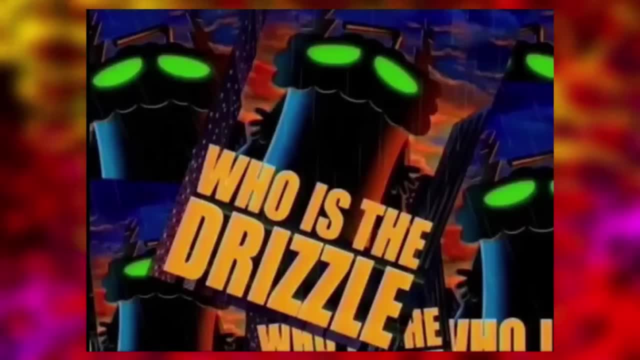 because the Explosion Gag was introduced after the episode's superhero. objects explode because either Shake is still full of radiation and toxic waste or the floor itself is radioactive, or perhaps Shake has an unconfirmed superpower. However, like stated before, there is questionable. 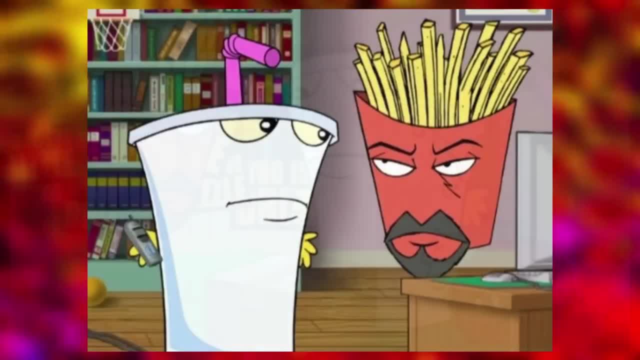 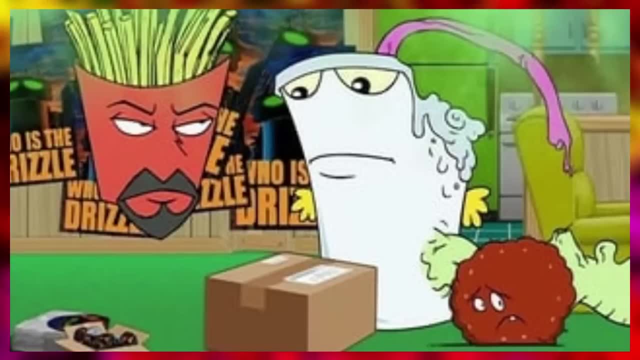 canonicity and the episode, like most, ends with Shake being disfigured, which does not stay to later episodes. Another rumor in regards to the Explosion Gag is that, allegedly, the animators blew up objects on purpose so they didn't have to keep them in the same frame. It's worth noting that 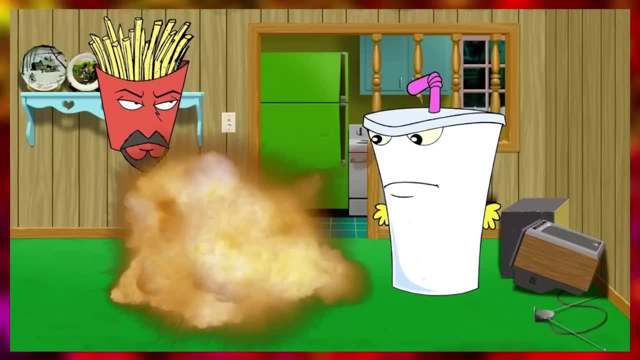 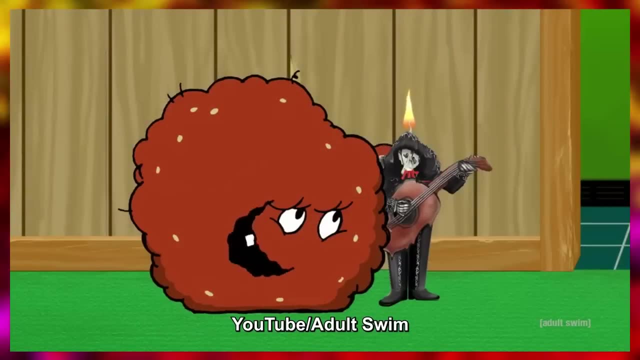 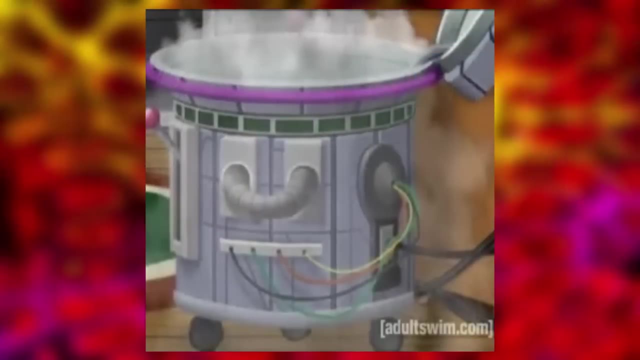 the Explosion Gag was finally addressed by the characters in the Aquadonk episode of The Dumbest Doll of All, but still with no answers. I've heard another rumor that there was an old adult swim bumper explaining that Frylock would clone the household objects so often that they became 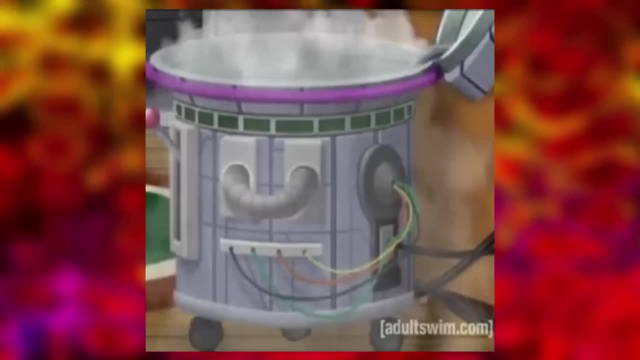 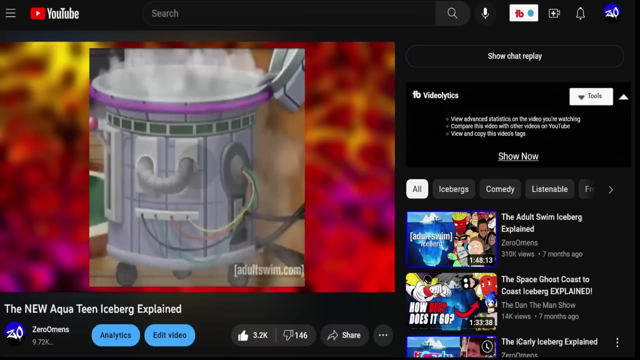 molecularly unstable, but this rumor has no backing, as no bump like that has surfaced as of yet. Buenos dias, everyone, it's your boy. Listen. I don't mean to interrupt this part of the video, but I want to take a second of your time to address the bumper rumor. So I received a 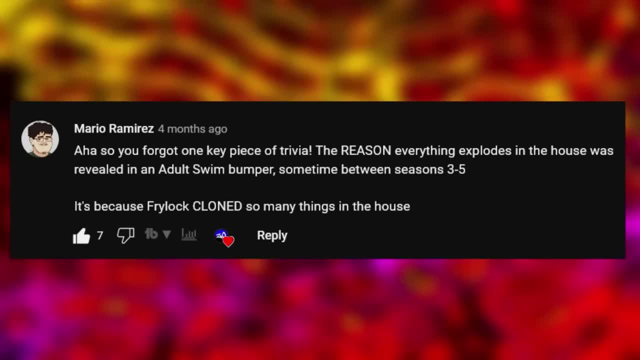 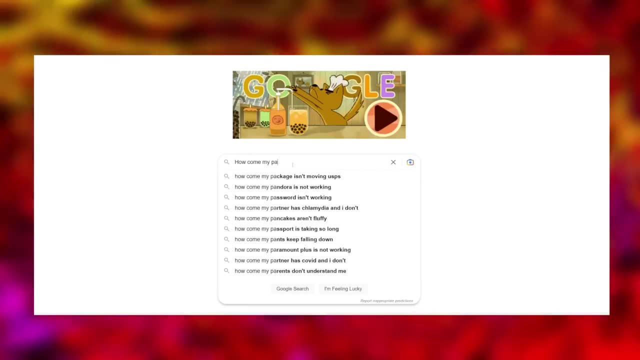 comment on my previous Aqua Teen video informing me of this Explosion Gag bumper, and so I knew, going into this brand new, updated video, that I had to look into the whereabouts of this bumper. So I searched across the internet far and wide. I checked out Archiveorg and Bumpworthy and that one website, your mom. 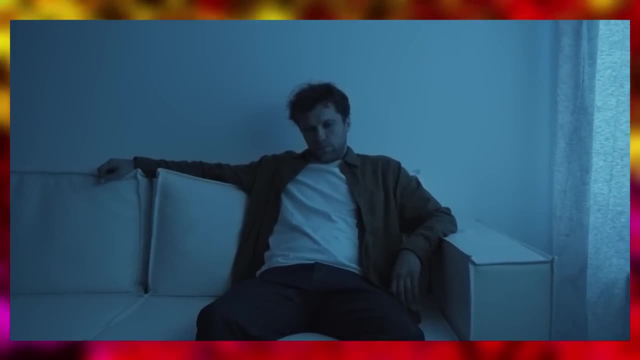 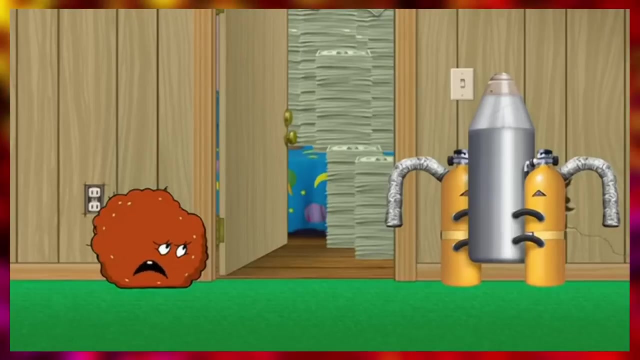 posts photos on. but sadly I could not find the bumper. So then I started to wonder if there was just a bumper promoting the Aqua Teen episode, The Cloning. but from the sound of it it seems like this Explosion Gag bumper is its own separate thing, So I decided to reach out to the only. 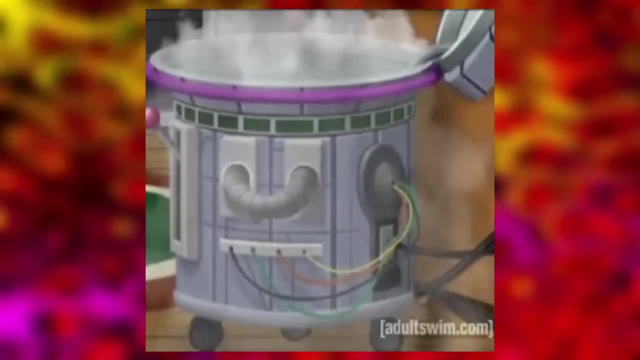 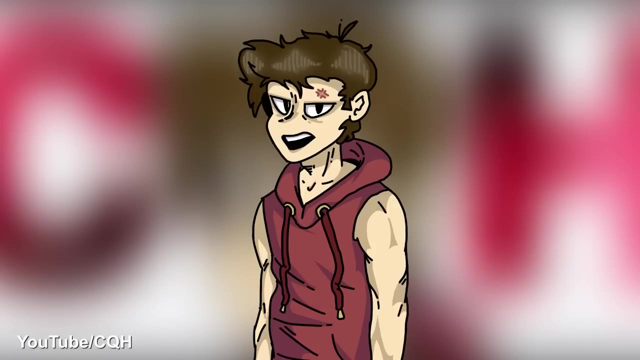 other person that I know who is an expert in Aqua Teen lore and might have an answer as to where the hell this bumper is. Why are you asking me that man, Better yet, what the fuck even is Aqua Teen? Cause like I ain't here to talk about wet teenagers, okay, Never contact me again. 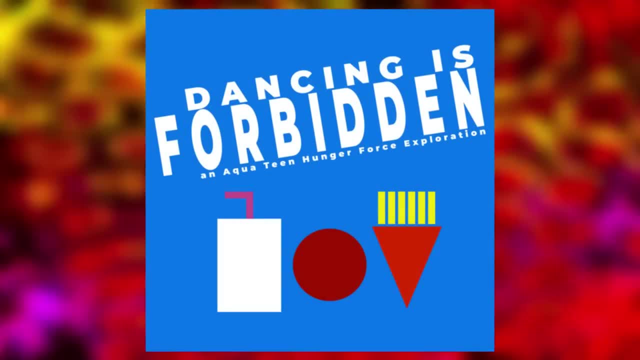 Well, that was a bust. I mean, I guess I could contact Ronnie and see if he knows anything. Okay, so, all jokes aside, I reached out to Ronnie about this and although he didn't have any information about the bumper, he recommended that I contact SwimWiki on Twitter about it. 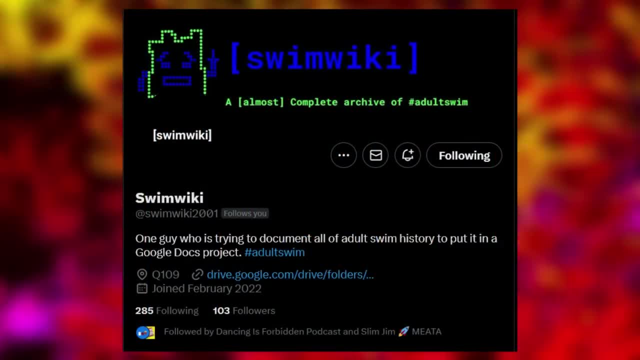 Now SwimWiki- for those of you who don't know- is one man's attempt to document and archive all of Adult Swim's history in a Google Doc. By the way, you should totally give him a follow on Twitter and tell him I sent ya. Anyways, I trusted Ronnie and reached. 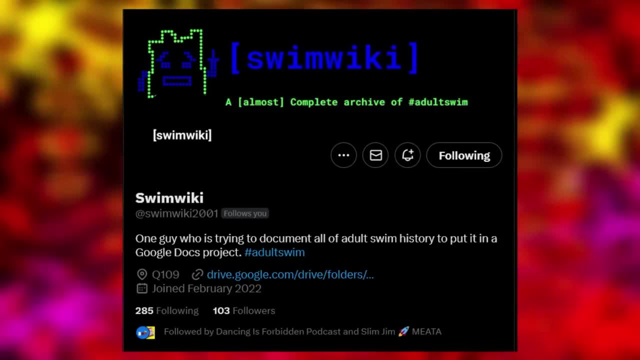 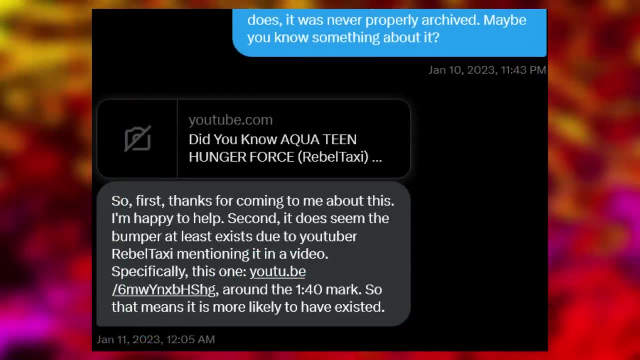 out to him about the bumper and he told me that the bumper was the bumper that SwimWiki had. I just asked him if he knew anything about the bumper and, sure enough, I received a message right back And, first off, he was very happy to help me And, second off, he sent me a YouTube. 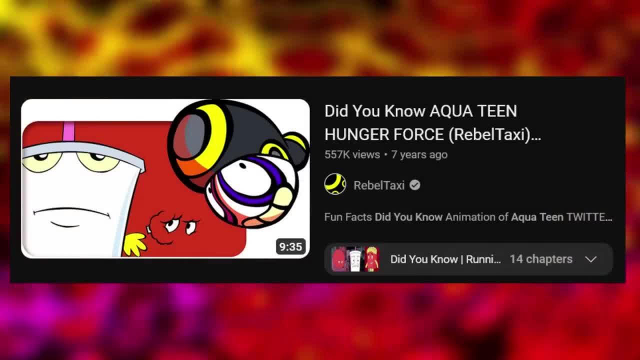 link to Rebel Taxi's. Did You Know Aqua Teen Hunger Force video. And right around the 1.40 mark of the video, Rebel Taxi states that he saw the rumored explosion gag bumper a long long time ago Now. although Rebel Taxi's words isn't exactly solid proof of the bumper's, 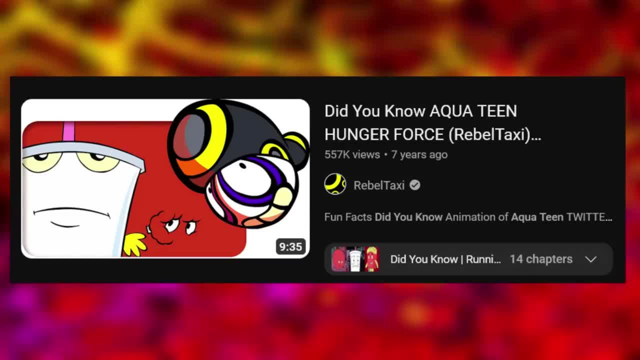 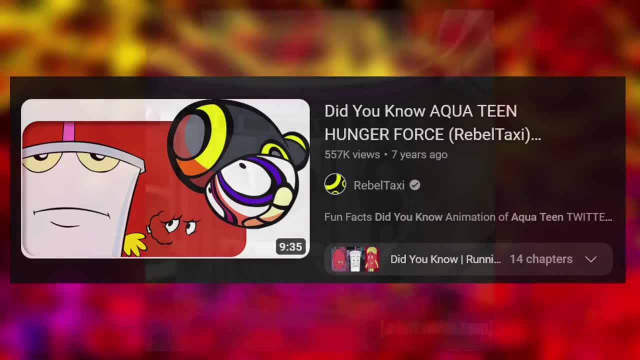 existence. the fact that there's more than one person claiming to have saw this bump leaves me to believe that it did exist at one point, but it just wasn't archived. So that's where I leave it to you guys If any of you watching up until this point know of any information surrounding this. 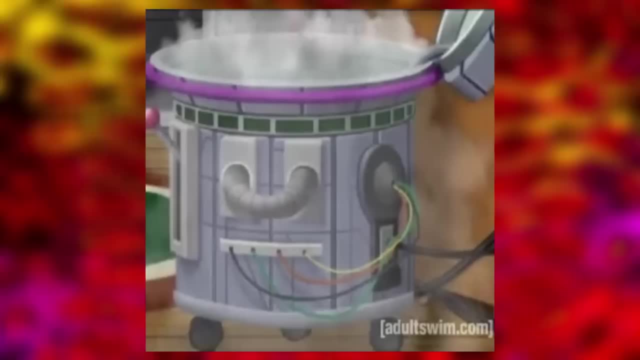 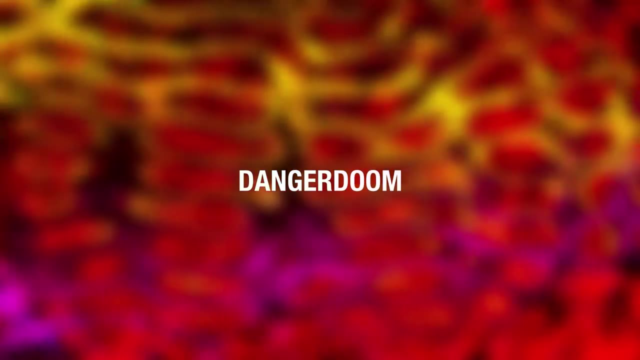 rumored lost Aqua Teen explosion gag bumper. let us know in the comments. Thank you for coming to my TED Talk. Now let's get back into the iceberg: Danger Doom. Danger Doom was a hip-hop collaboration project featuring artists Danger Mouse and the late. 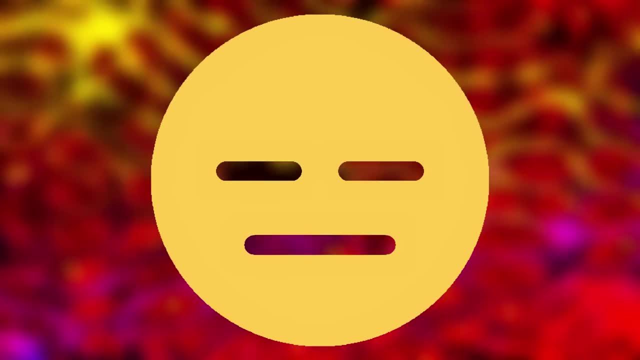 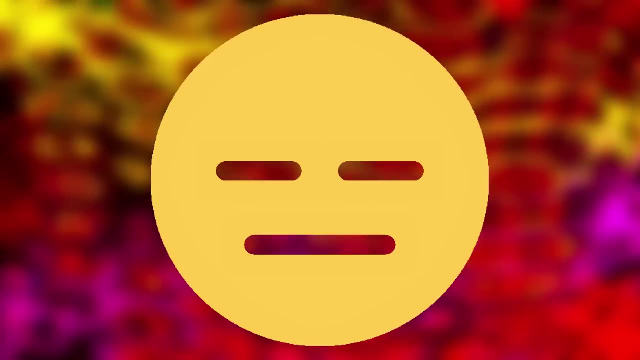 great MF Doom, Hey Zero. uh, couldn't help but notice that in the bullet points he gave me, MF Doom's name is not in all caps. That's gonna, that's gonna dock you some points. Tsk, tsk. 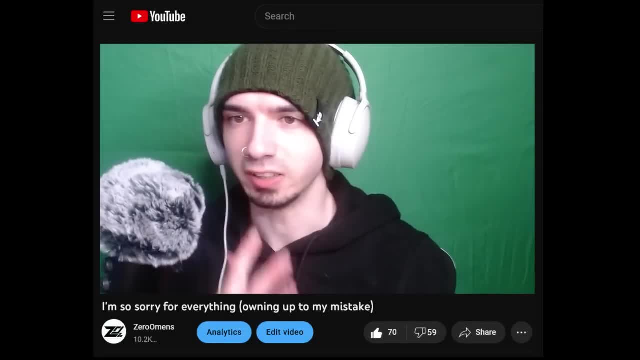 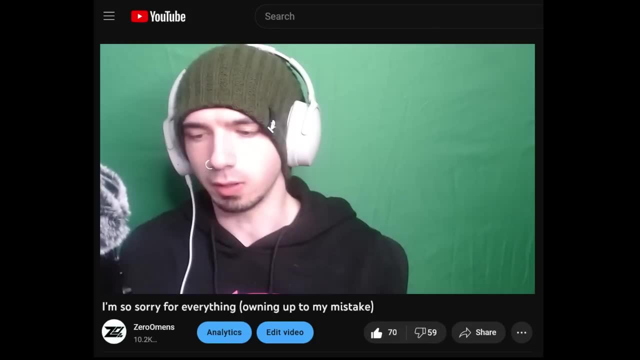 Uh, let's see. I made a severe and continuous lapse in my judgment and I don't expect to be forgiven. I'm simply here to apologize. I blame my keyboard. Their album The Mouse and the Mask features tons of references and characters from Adult. 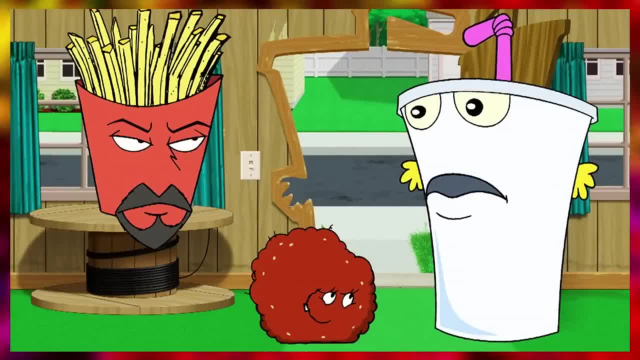 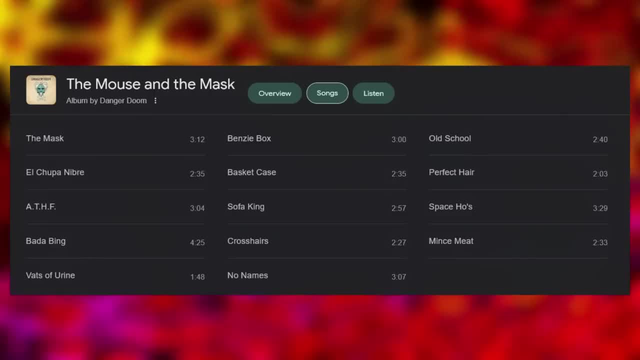 Swim programs like Harvey, Birdman and, of course, Aqua Teen. In fact, Shake, Frylock, Meatwad, Carl and the Moonenites all make appearances on this album. Listen to it if you haven't already. there's a song on the album just called ATHF for Aqua Teen- Hunger Force, and I absolutely love it. 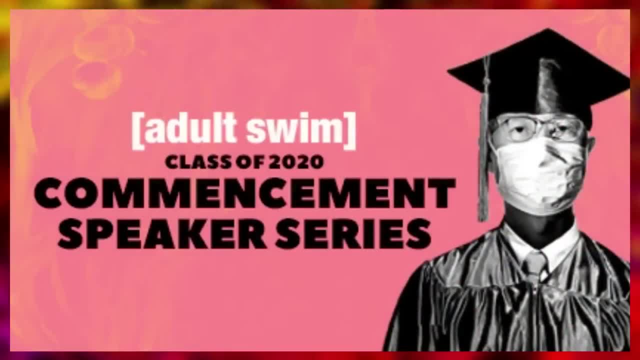 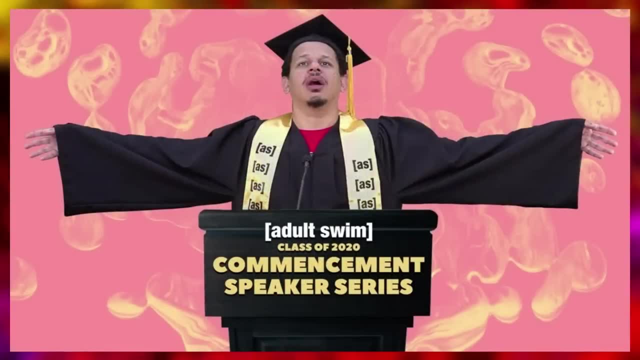 Commencement Speaker Series 2020. The Class of 2020 Commencement Speaker Series was an Adult Swim livestream show Every Monday, Wednesday and Friday of the 2020 graduation season. various real famous people like Eric Andre and Killer Mike. 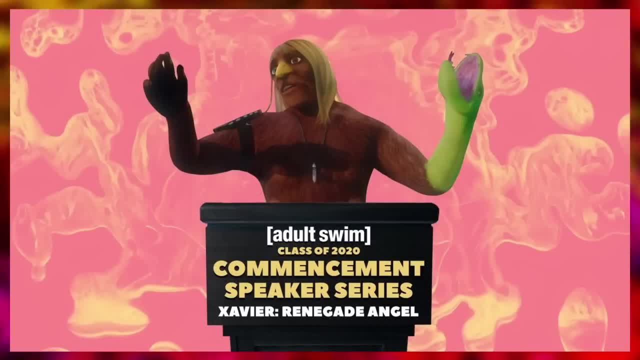 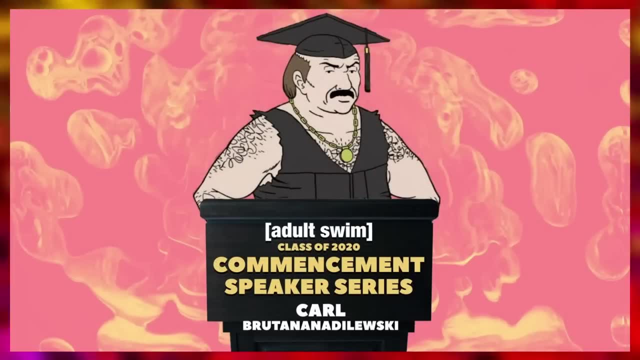 as well as Adult Swim characters like the triumphant return of Xavier, Renegade, Angel, Carl, Brittana and Analuski from Aqua Teen delivered commencement speeches to the graduating class of 2020.. DVD Bonuses: Let's just cut right to the chase. There are a. 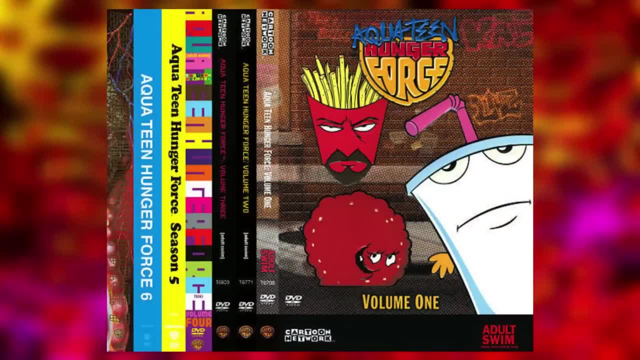 lot of behind-the-scenes extras, bloopers and bonuses for Aqua Teen, and, although it would be awesome to talk about each individual piece of bonus content from the show in-depth, this video will be like four hours long, which is not unheard of for me personally. 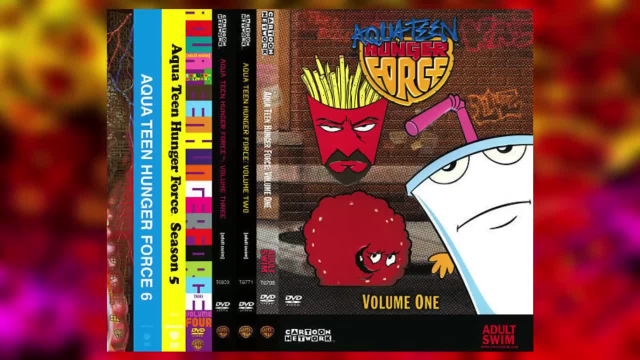 but when I'm in other people's places I gotta be respectful. So for our sanity and your precious time, here's a list of most of, if not all of, the Aqua Teen DVD bonuses, If you ever find some free time away from whatever it is you do when you're not watching Iceberg. 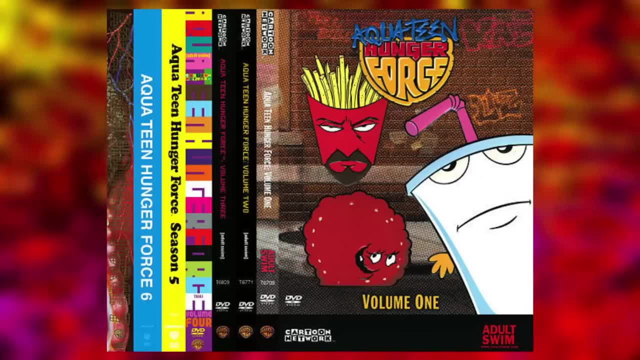 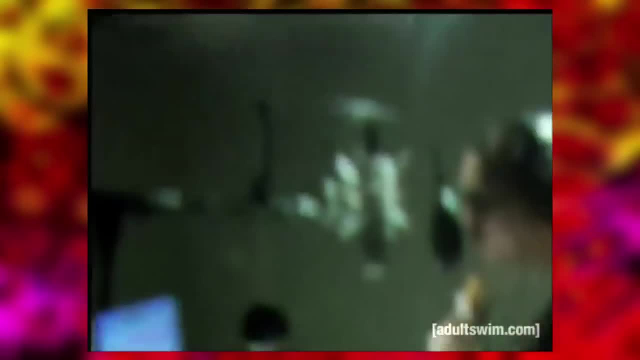 videos and you want to watch hours of bonus Aqua Teen content, then buy the Baffler Meal collection and check the footage out. The bonus features are also available on Archiveorg for free. Tara Patrick Eats a Hot Dog, which is just footage of adult actress Tara Patrick in a. 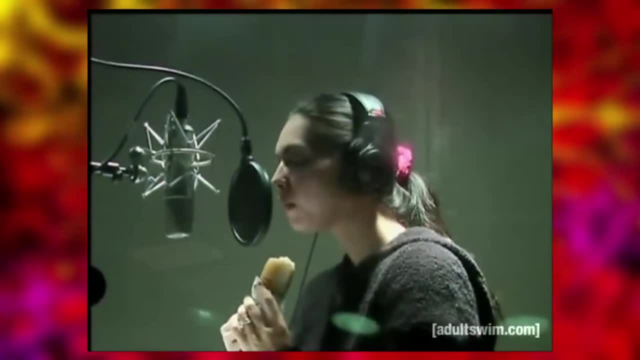 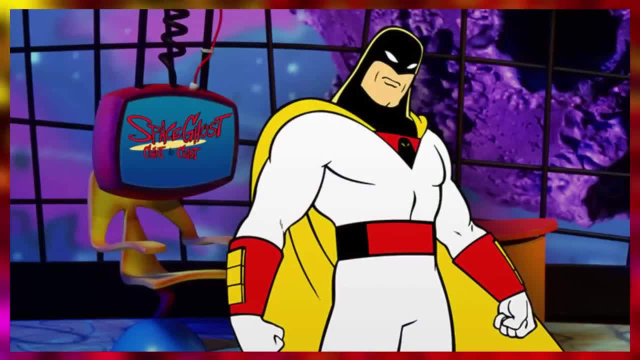 The Space Coast, Coast to Coast episodes Shambrina and Baffler Meal. I know I said I would go through these quickly, but this one requires some more explaining. You see, the Aqua Teens were originally penned to be one-off side characters in an episode of the animated talk show Space Coast, Coast to 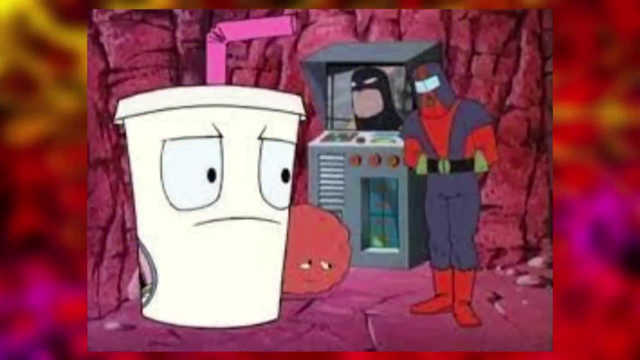 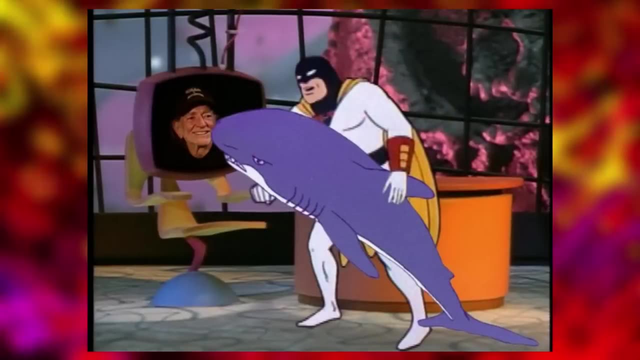 Coast, but it was rejected because it initially focused too much on the Aqua Teens, so it was then rewritten to the episode that made it to air Kentucky Nightmare. Baffler Meal is the version of the episode that was initially rejected because of the amount of Aqua Teen screen time, but after the 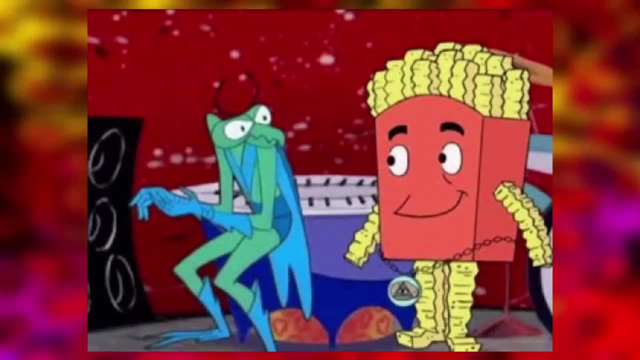 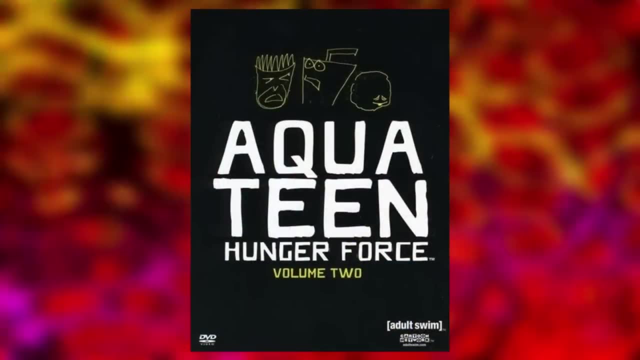 Aqua Teen series had come out already and proved to be a success. they aired the episode as part of the Adult Swim New Year's Eve Marathon on January 1st 2003,, and then the episode was featured on the Volume 2 box set. Granny Takes Her Top Off, which is footage of Dave Willis' real grandmother. 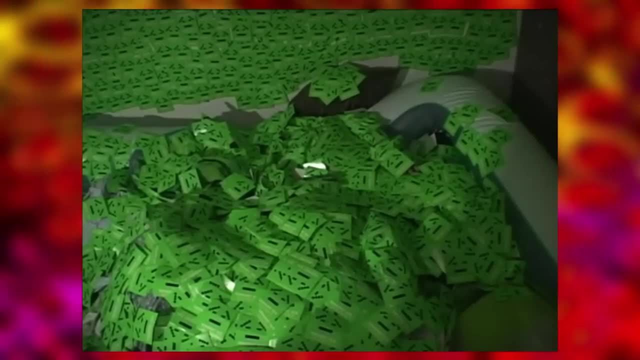 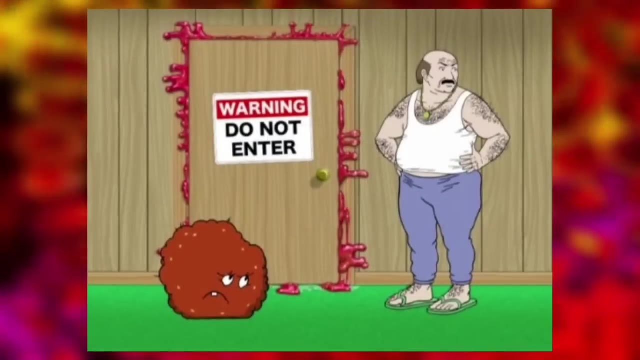 voicing her character in the episode Dirt Foot, The Moon and Nightmare. Easter Egg Short. the Zombie Ninja Pro-Am Trailer. the I Like Your Booty music video. the uncensored version of Dickasode, the Colon Movie world premiere hosted by Space Ghost. the Send Us Money for This Movie. 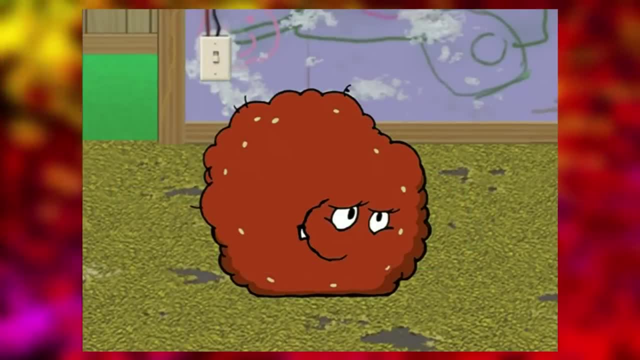 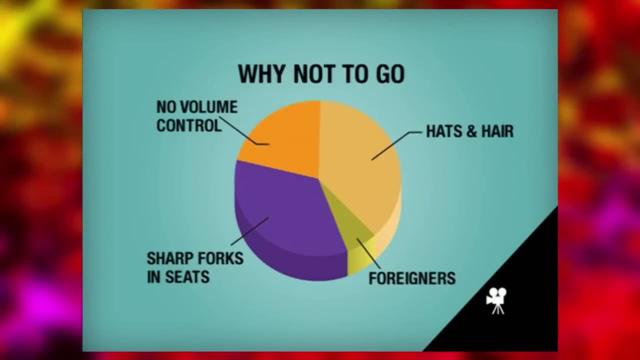 Teaser: various promos and bumps, like the Funny Pete Stuff promos. the Aqua Teen Responds to the Critics promos- 11 additional Aqua Teen bumpers. 2. San Diego Comic-Con promos. Overhead Projector Presentation promos. Dana Man on the Street promos and the Baffler Meal Hunger Imagery Short. 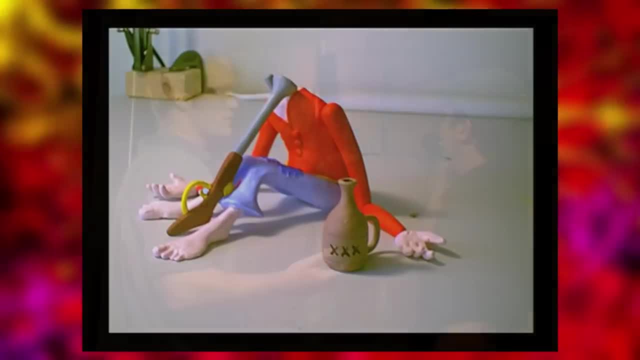 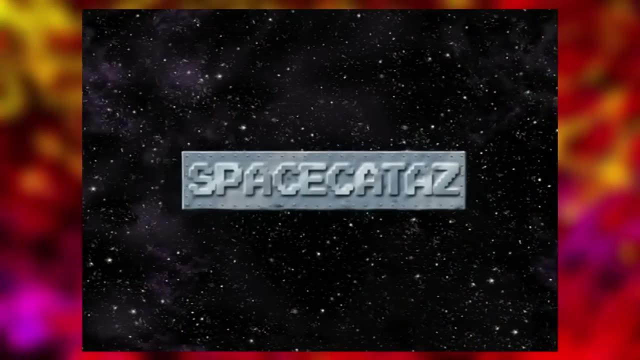 F-Art, which is just fan art. it may be pictured here. Radon, which is a live-action 11-minute short starring Dave Willis and Matt Malero, creators of the show The Fool Space Cataz episode Three. lyric videos for the song Spirit Journey Formation. 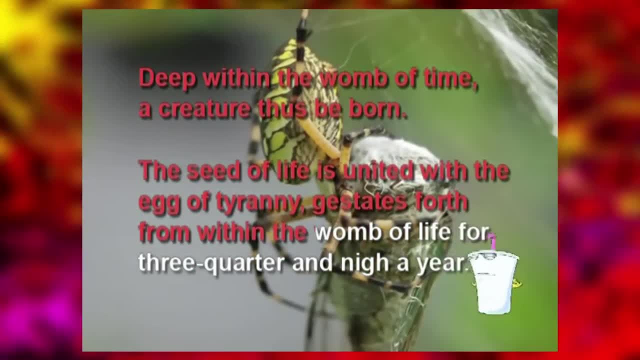 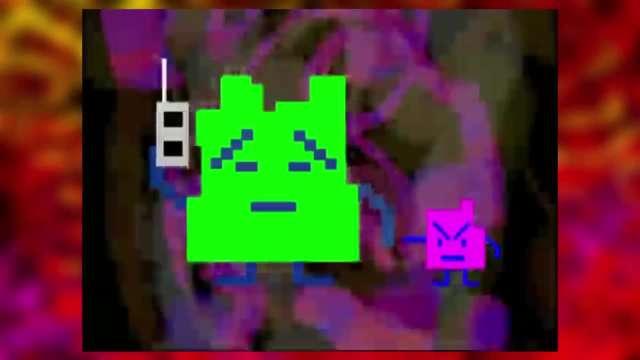 1 version performed by Zach Wilde, 1 performed by Dana Snyder and a karaoke version. Voicemail audio recordings from Shake, Meatwad, Frylock, Carl and the Moonanites, The On Loan from the private collection of Vishal Al Rony, which displayed tons of concept art from: 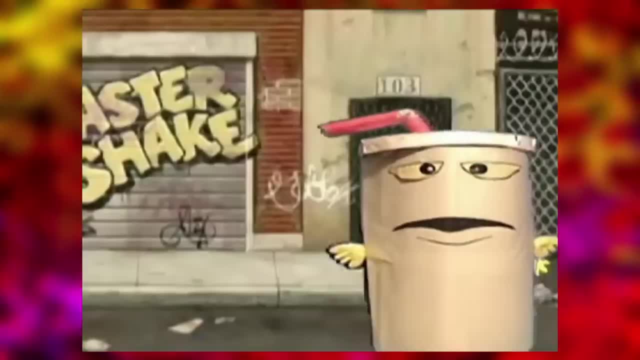 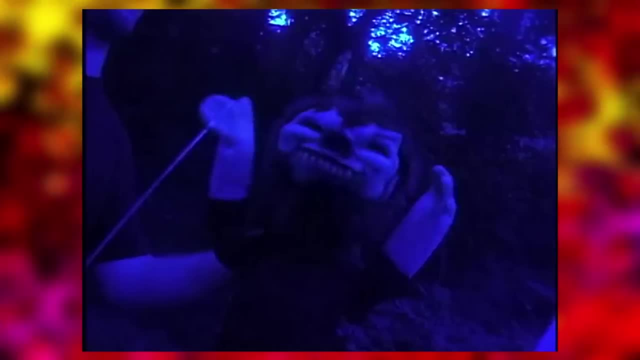 Season 2. A live-action Aqua Teen intro. Lots of short live-action films that were featured in the series as TV shows that the Aqua Teens watched, like Bowling Puppet Show, Horror Puppet Show, Vegetable Man, Teaching Puppet Show, Assisted Living Dracula Witch. 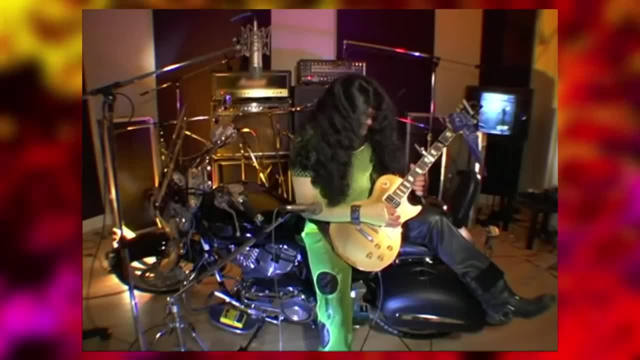 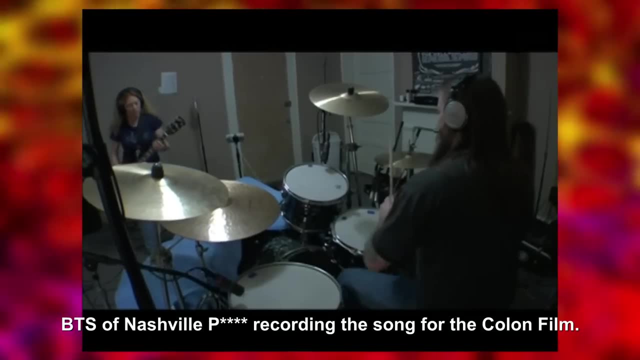 to Be Fair, Does Seem a Little Slow and Learned a Shred Like the Master Shake performing the song Omelette Face with ice caps and the late Neil Peart under the name Nashville. Deleted or unfinished scenes from the episodes: Bart Oates, Grim Reaper. 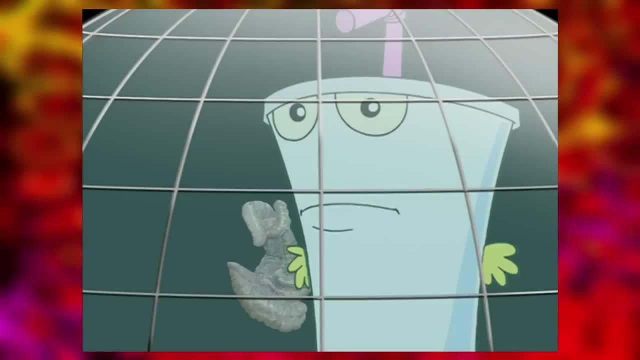 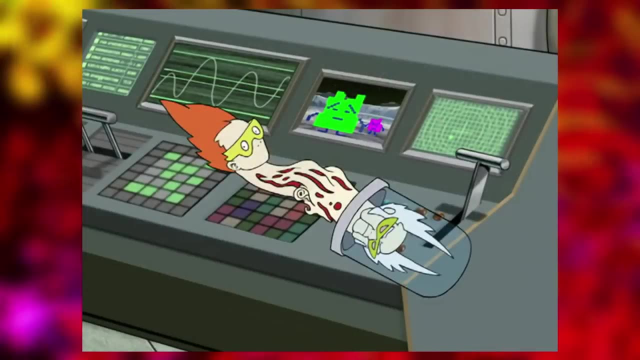 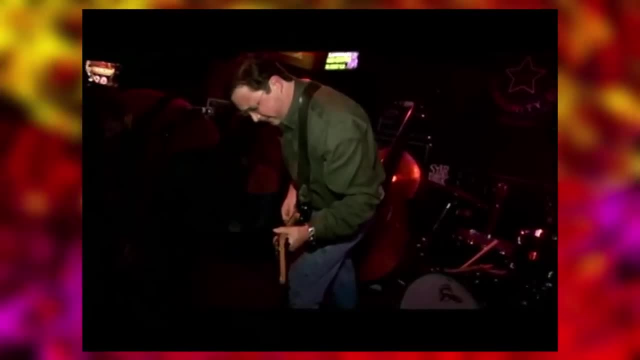 The original cut of Rabot, which was used as the pilot for this episode. The original cut of Rabot, which was used as the pilot for this episode. Tons of live musical performances from Dana Matt and Dave Unearth performing The Chosen. 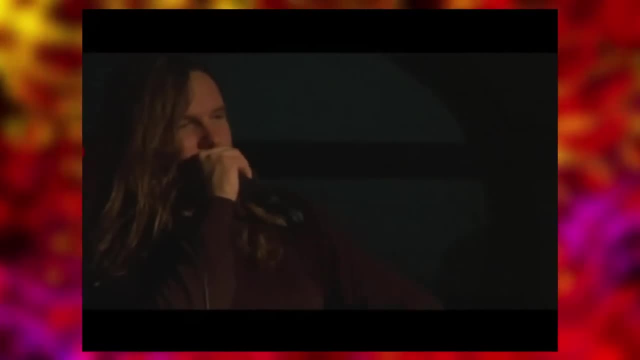 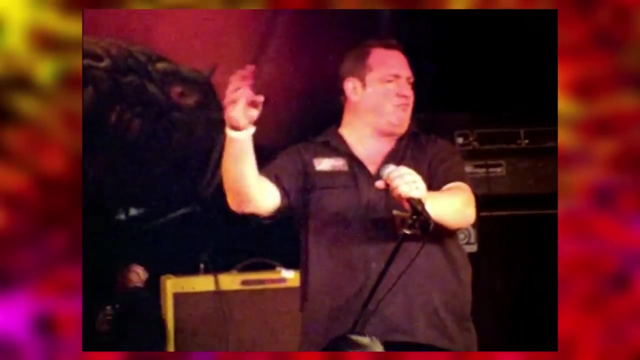 which was a track featured in the Cullen movie film for theaters: The Baffler Meal performance, the Aqua Teen theme song live rock version and Nine Pound Hammer performing Carl's theme. There was also footage of Dana Snyder performing live with a kazoo. 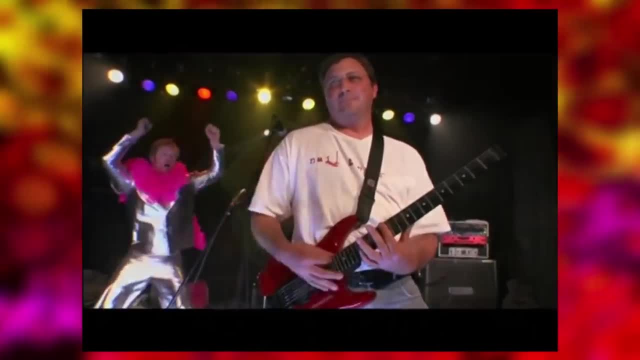 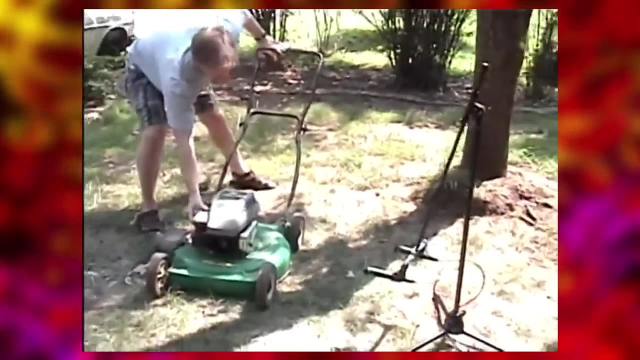 a segment called Favorite Episode Week Promos and Brass Castle Bookwork Resin. Live Capturing lawnmower audio, which shows Dave Willis recording audio of his lawnmower at his house. The Cullen movie theatrical alternative and sizzle reel trailers. The Dana, Snyder and Bob. 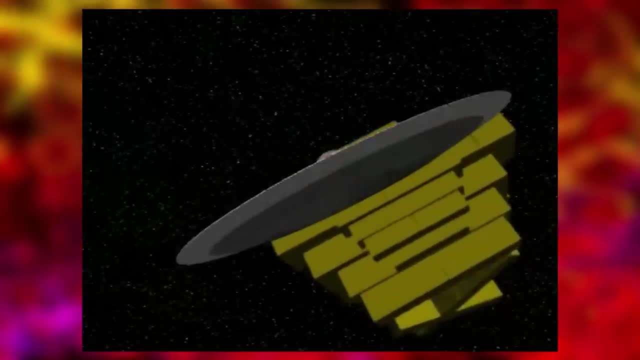 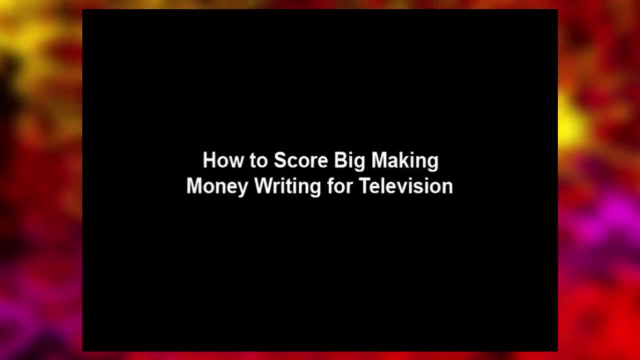 Odenkirk interview. John Schnepp's Cullen movie 3D disc menu. art video Behind the scenes. shorts like Future Wolf, Future Wolf 2, Never Cry Wolf, Future Wolf 3 had a score big, making money writing for television. The thing we shot Wednesday night and the faces in front of the throats that make 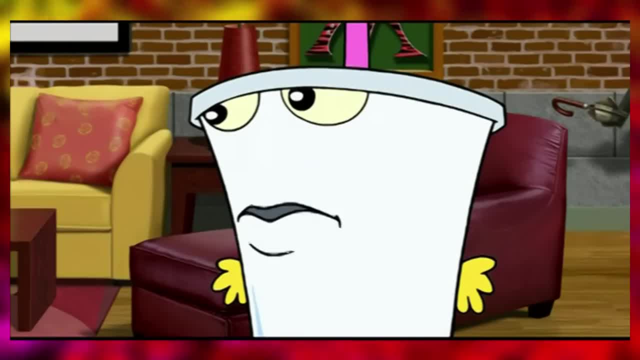 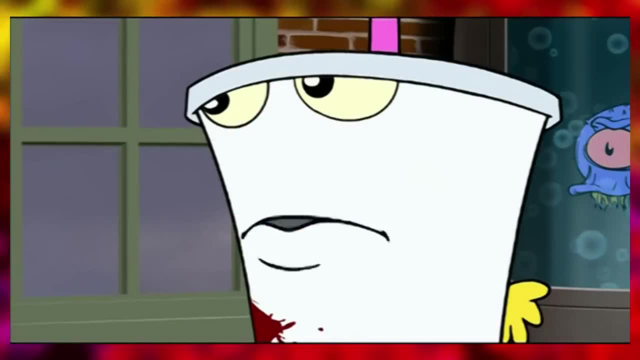 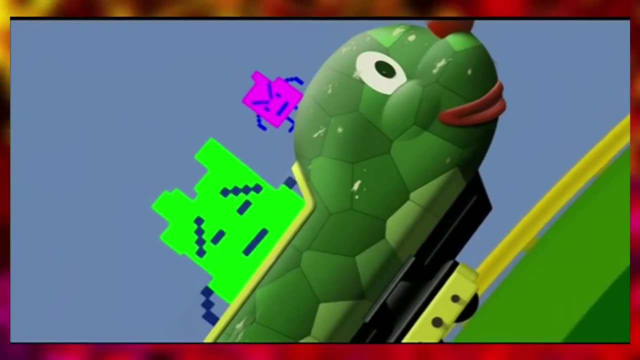 the voices that speak into the microphone. The 10 fake dot com endings that we discussed earlier. The Cullen movie art and music gallery Extended scenes for the Cullen movie. like Shake, Who Created Us, I'm the One Pushing Insanoflex Box Phone Answering Machine. Fight Moonanites and Plutonians on Rollercoaster. 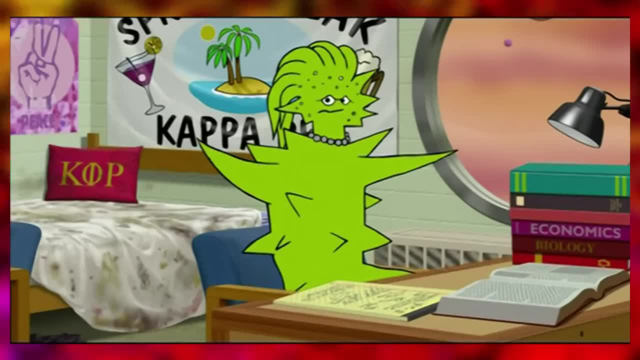 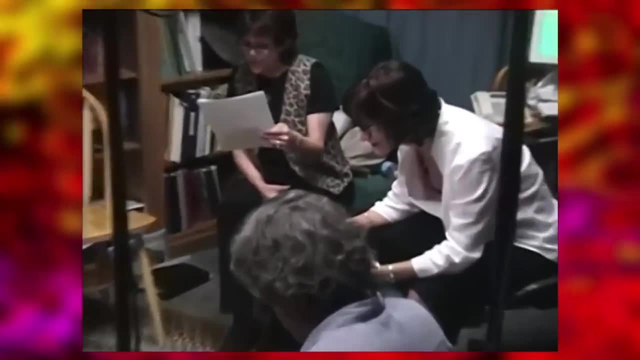 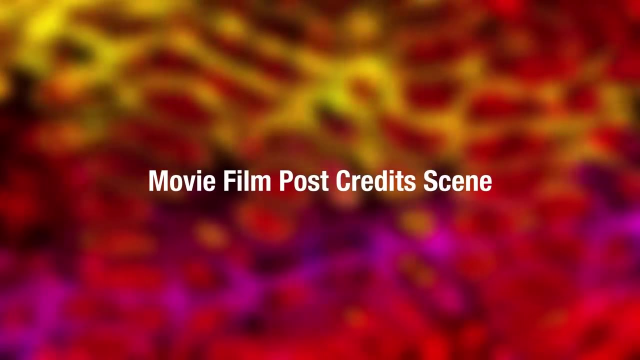 Meatwad Concert, The Dorm Room, and a deleted scene featuring American funk band Cameo. Behind the scenes, footage of Cameo Macedon and the Lobby Singers recording their tracks And finally, the deleted movie Movie film post credit scene. 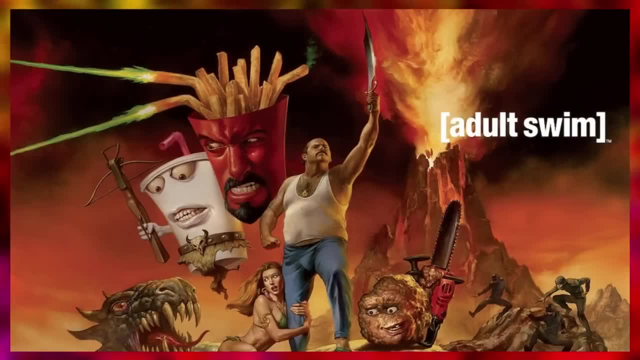 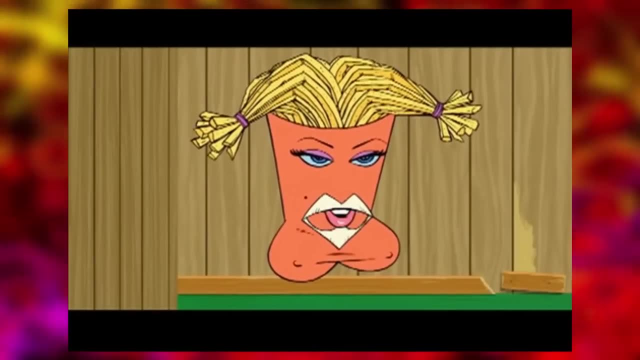 After the credits of the movie film, we are gifted with a lovely post credit scene featuring the cybernetic ghost humping the Aqua Teen's television in the living room, before female Frylock appears on screen to tell him that it's time for bed. in Frylock's voice, Shake wears yellow gloves. 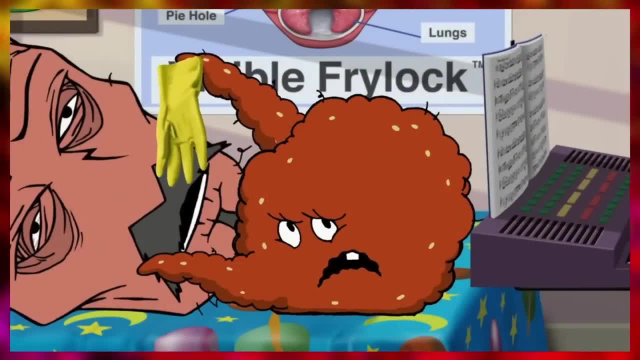 It is revealed in The Last One, Forever and Ever, For Real- This Time We F***ing Mean It- that Shake's yellow hands are nothing more than yellow dish washing gloves. This moment could very well be a callback to the episode- The Last One, Forever and Ever- where Shake's 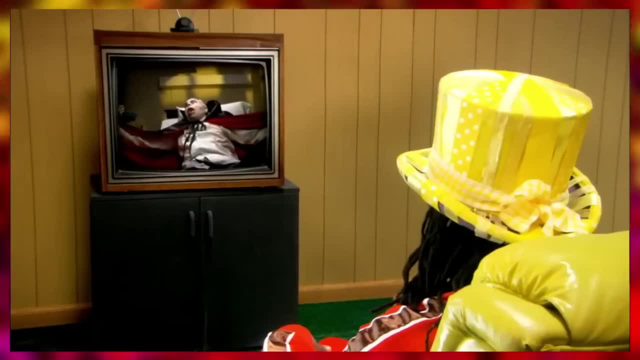 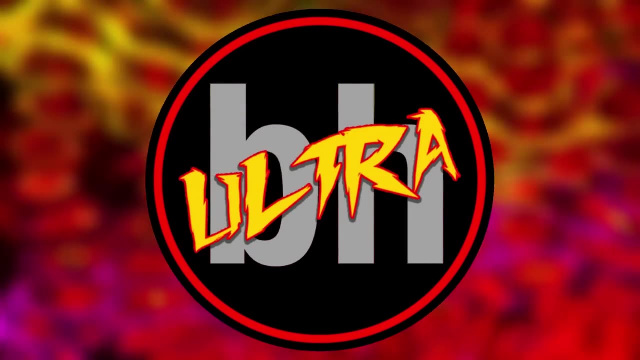 action counterpart wears yellow gloves and is shown washing a dish, something the real Shake would never do. I've been BH Ultra here because I love Aqua Teen and I've always wanted to be a part of an Iceberg video on to Layer 3.. Buenos dias everyone. I just want to shout out Lucian and Dustin from the Weekly Geekly for having me on a recent episode of their podcast to discuss the ins and outs of their series Death Cast, which is a podcast set inside the world of Metalocalypse. The guys were great. 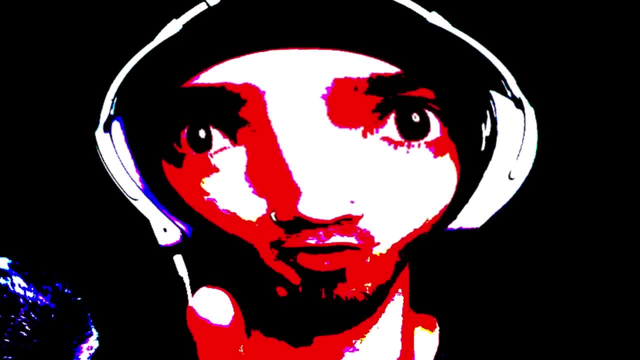 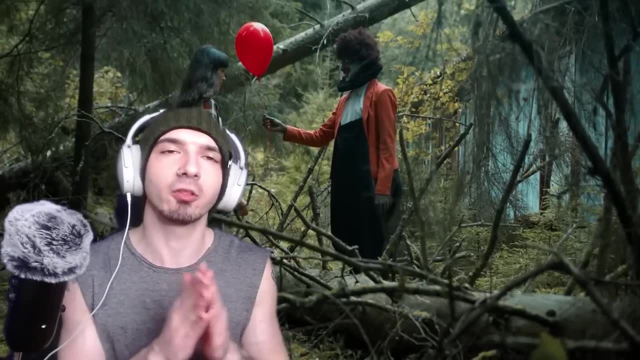 And we were even joined by a very special guest. No spoilers, though, But check out the brand new episode. It's available on Spotify and YouTube. Let the guys know that I sent you, Give them some love And, without further ado, let's dive back into the iceberg. 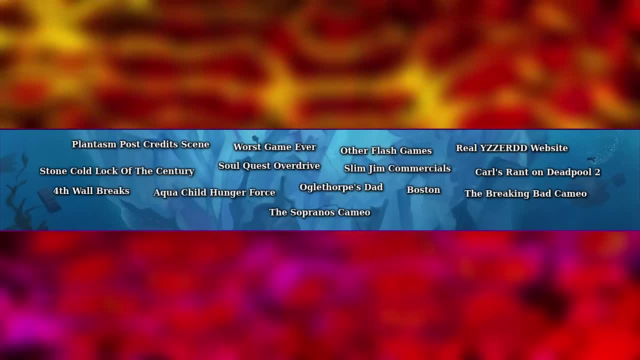 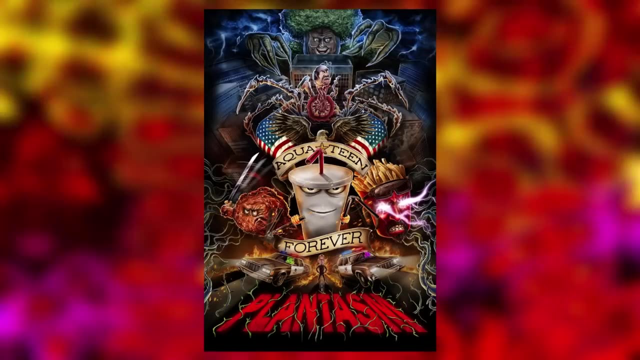 This is the Bibble. You question the words of the mighty Jimmy. No, Plantasm post-credit scene. Hey, spoiler alert: If you haven't seen Plantasm, then skip over the entry. At the end of the Plantasm ending credits, we are gifted with a scene. 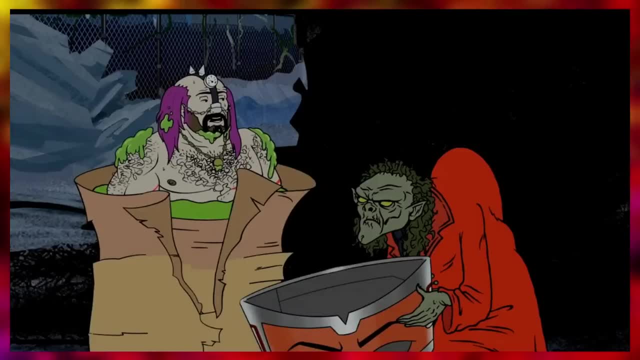 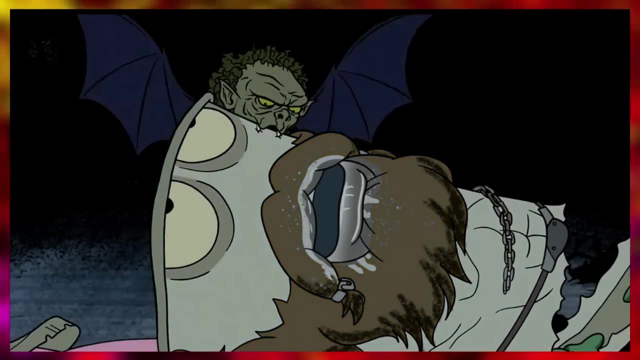 that features Jake, Freilich and Meatwad being eaten alive by the Fraptaculans, the Japongoloids Carl and Markula. Markula then takes a bite out of Jake, which causes him to be reanimated as a vampire. 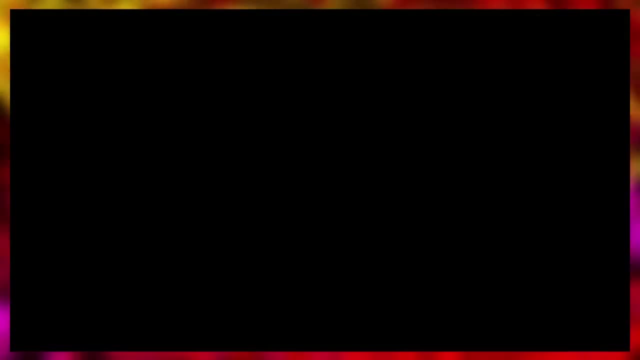 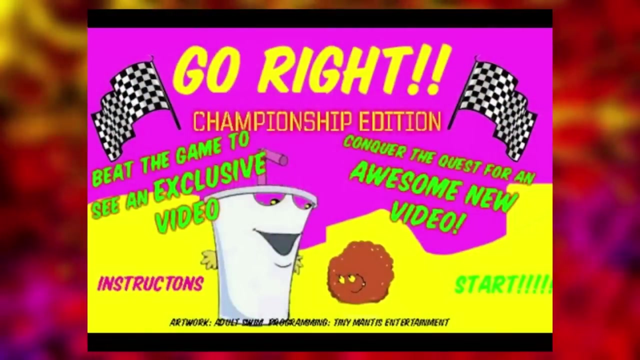 Jake ends the scene by uttering the line. I smell a sequel before flying into the camera. So Plantasm 2 confirmed Worst game ever. The worst game ever was a flash game available on AdultSwimcom Now, while the game isn't playable on the website anymore. 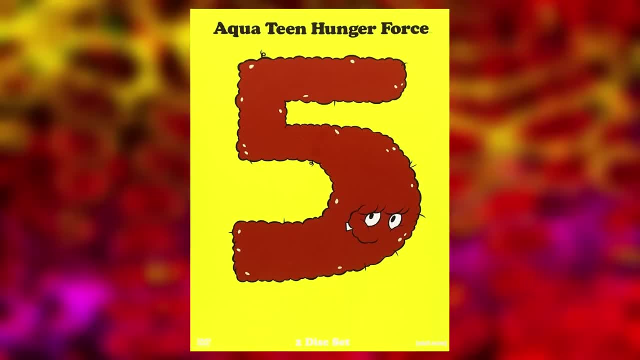 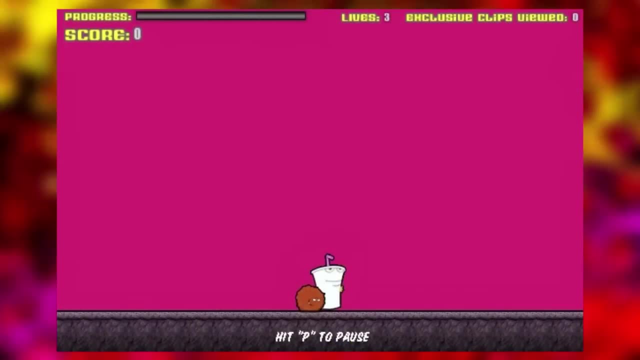 you are. You're able to play it if you own the Volume 5 DVD. Basically, the goal of the whole game is to get Jake and Meatwad to the end of the map by going right, while sometimes jumping over obstacles. I remember playing this game with my nephew when we were younger. 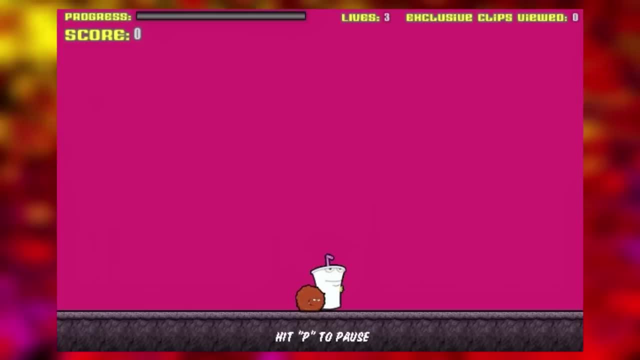 Him and I were very much obsessed with Aqua Teen and we heard a rumor that if we beat the game we would see an exclusive clip from the first Aqua Teen movie. So we grabbed my mom's laptop and tried to beat the game, but it took forever. 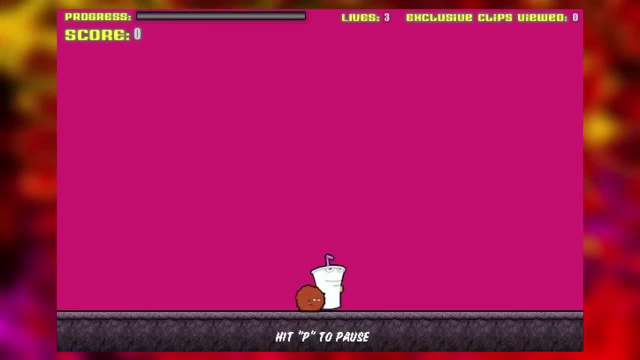 Our tiny attention span. I couldn't handle sitting down in the living room for more than 5 minutes playing the game. Luckily for us, there wasn't really a movie clip featured at the end of the game, at least on the AdultSwim website version. 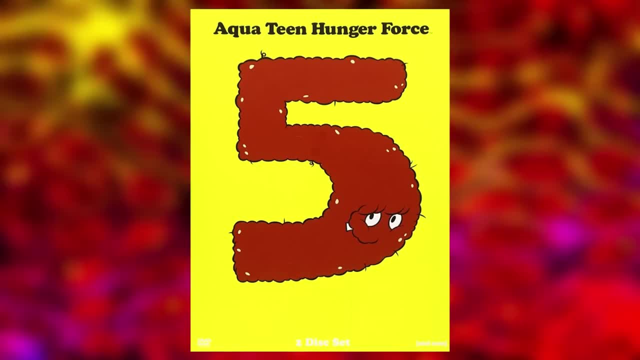 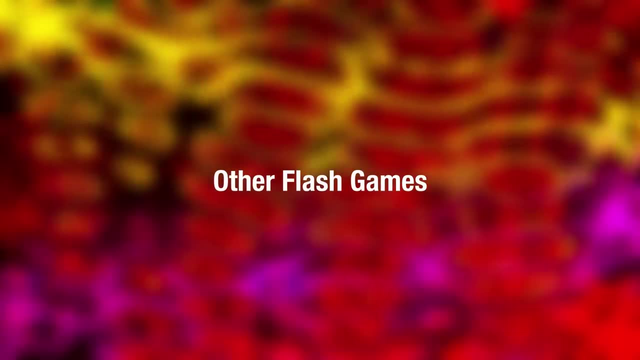 However, if you own the Volume 5 DVD and you play the game and you beat it, a 30 second clip from the deleted movie will play Other flash games Besides the worst game ever, Aqua Teen has had a pretty big selection of official flash. 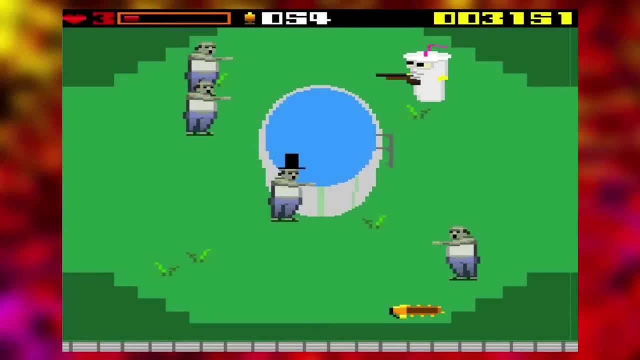 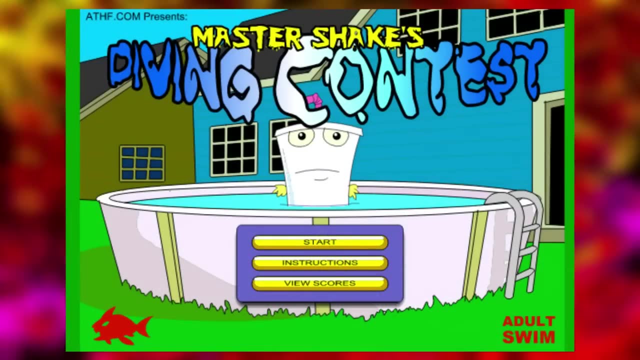 games created, including Dead Evil, Which is an 8.5 hour game, 8-Bit Zombie Game, Head Games, Moon and Night Marauders, which I do vividly remember playing. There was also a game called Master Shake's Diving Contest, Carl's Frickin' Strip Poker. 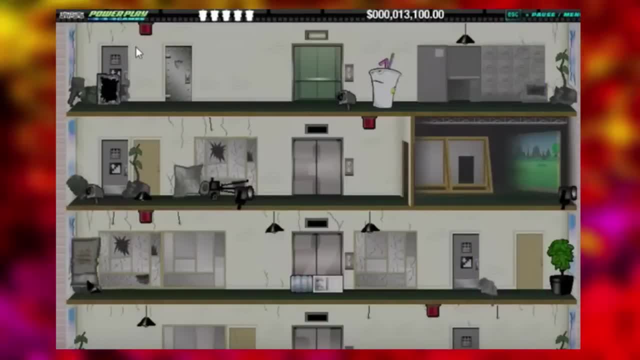 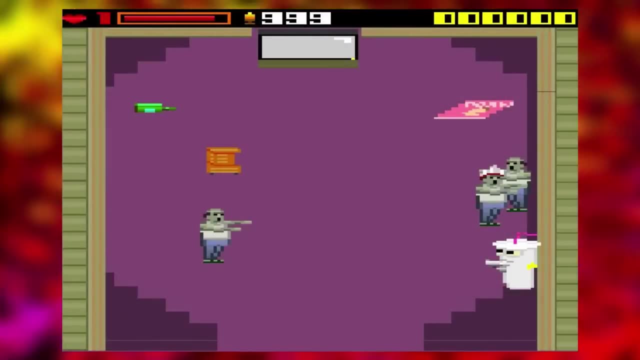 and Studio Shakedown, which was considered a lost piece of media for the longest time. A couple of these games have been archived on Archiveorg if you want to check them out. There were probably a few other Aqua Teen Flash games that existed at one point. 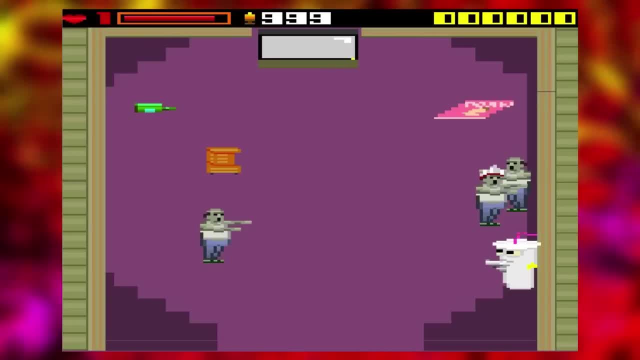 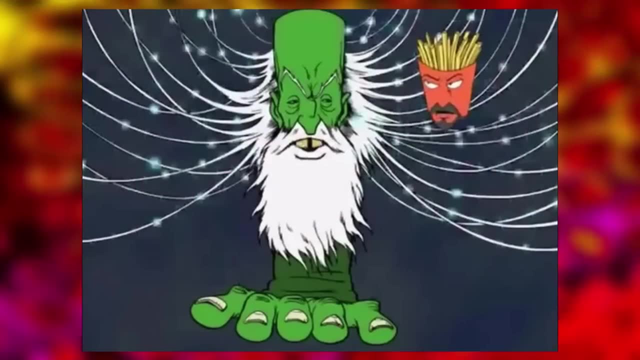 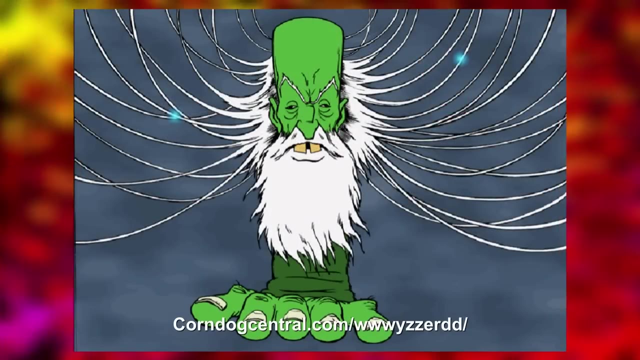 but I believe the games I just listed are the ones people remember the most. Real YZZERDD Website- The wwwyzzerdd website- was a real site created as a tribute to the episode Interfection. Users who went onto the website were bombarded with a bunch of joke pop-up ads that reportedly 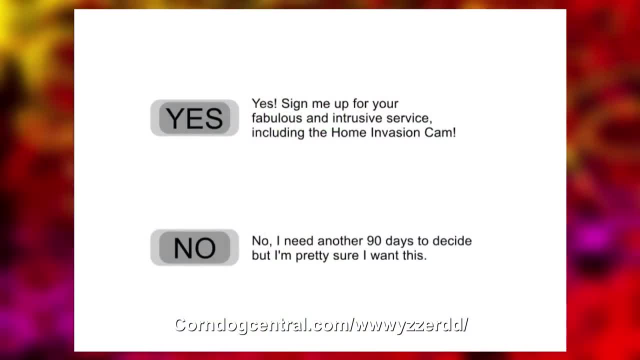 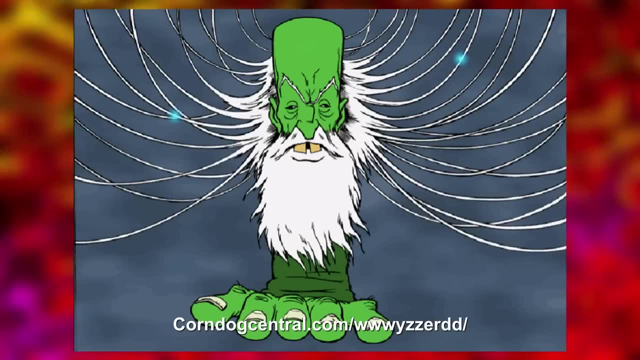 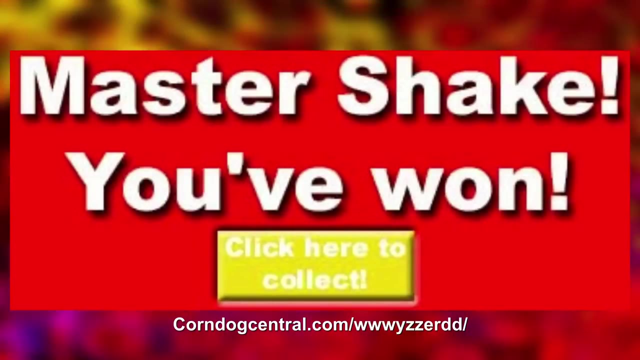 crashed a lot of people's hard drives. Now, sadly, the website URL only redirects users to the Aqua Teen Watch page on the Adult Swim website, which means the YZZERDD website no longer exists. However, the site was archived on corndogcentralcom. slash wwwyzzerdd. 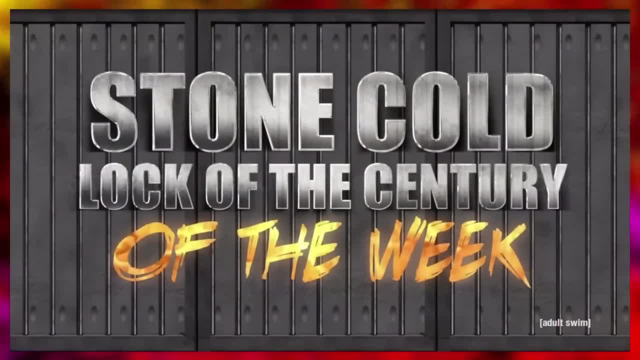 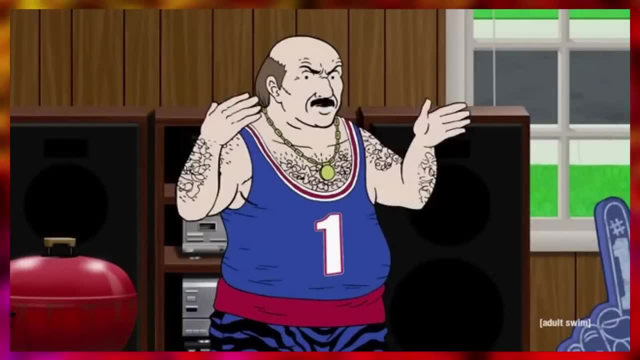 Stone Cold Lock of the Century of the Week. Carl's Stone Cold Lock of the Century of the Week, formerly known as Carl's P*** and Just Carl, and I believe Carl's Lock was an online series on Adult Swim's website starring our favorite. 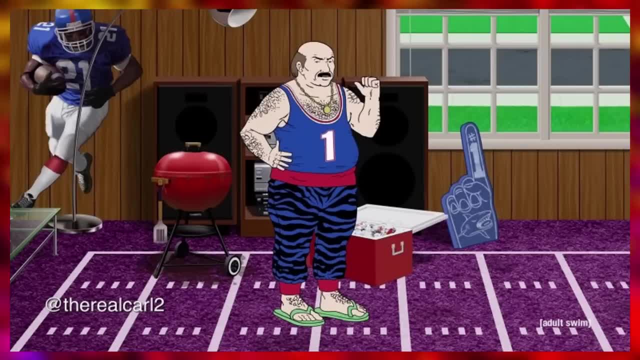 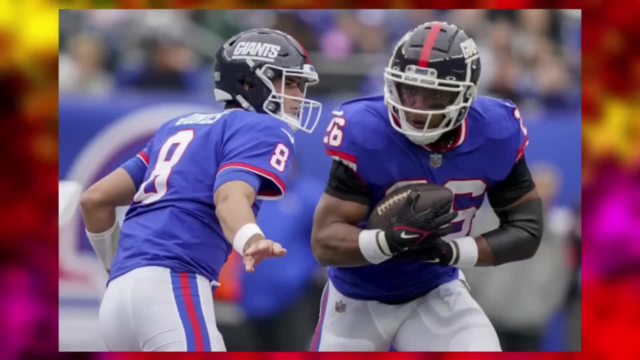 neighbor Carl. The whole premise is essentially about Carl standing in his living room mostly ranting about sports like the current football season, while repping merchandise from the greatest football team in the history of football, the New York Giants. Yeah, you can. 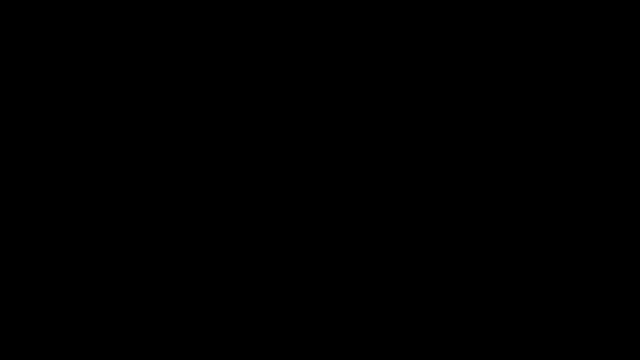 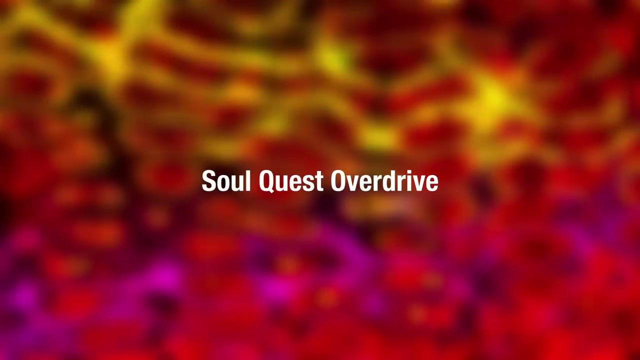 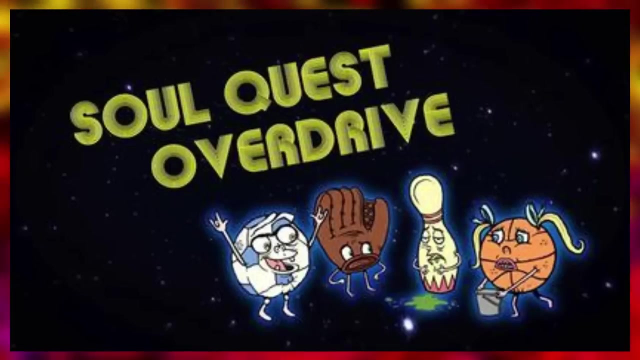 fight me in the comments all you want. We had a great season this year and you can't even deny it. The series started in 2007 and continued until 2016.. Soul Quest Overdrive. Soul Quest Overdrive was a short-lived spinoff of the Aqua Teen series created by Matt Malero. 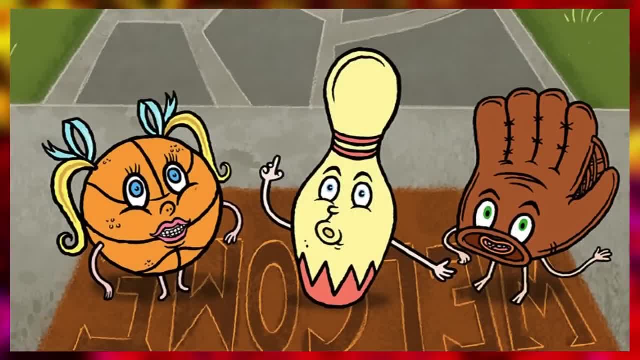 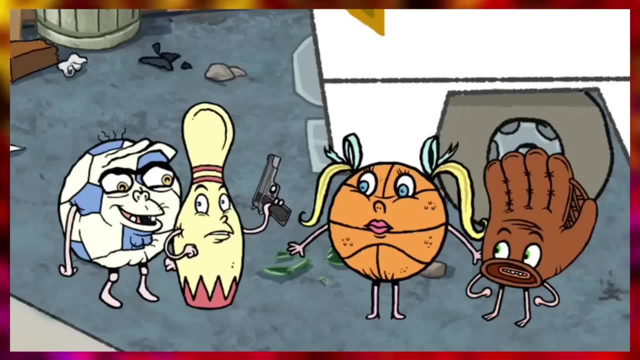 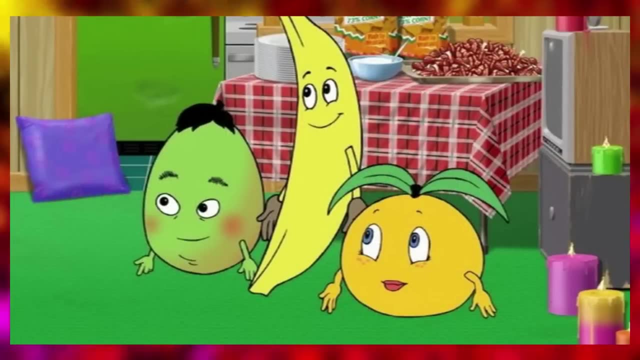 and Dave Willis. Six episodes were ordered, but only four of them were released. The show revolved around Tammy, Mortimer, Burt and Nick. four pieces of athletic equipment, three of which being based off of the Bible: fruit from the Aqua Teen episode of the same name, where Frylock makes friends with talking Christian fruit. 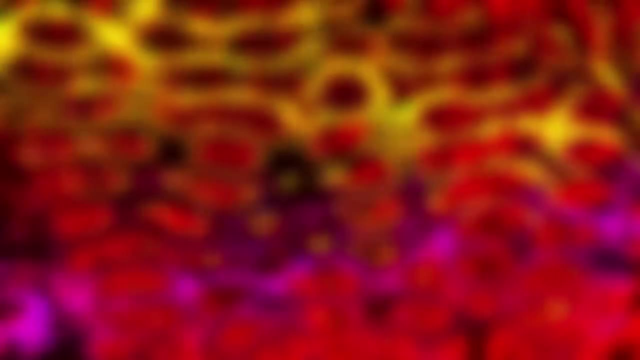 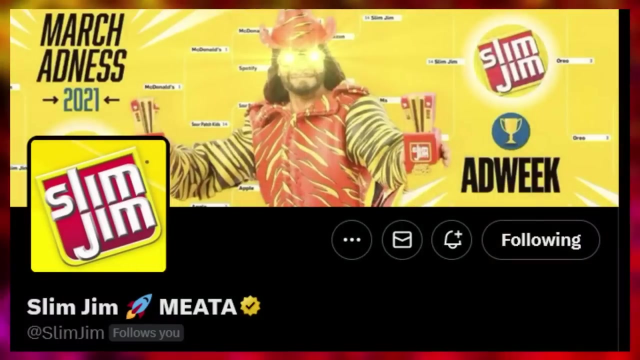 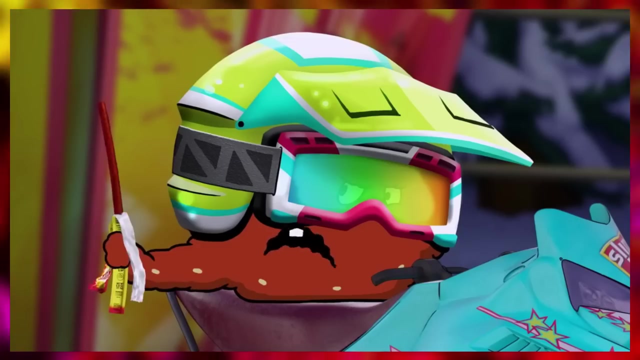 who are hooked on sex, drugs and violence. baby Slim Jim Commercials. The Aqua Teens were featured in three advertisements for Slim Jim. You know the meat guys who follow me on Twitter. They are you better. The first commercial features a fluent animation of Meatwad on a snowmobile. 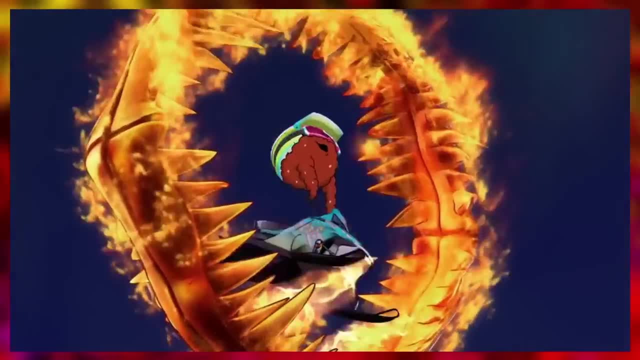 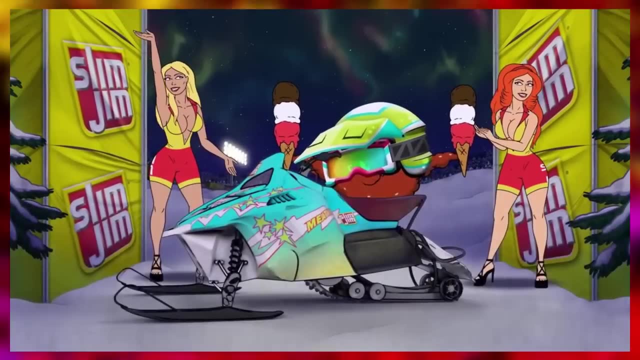 flying through rings of fire, entering the pits of a snake and dodging sharks And holy moly guacamole. The animation in this advertisement is fluent, baby. Not as fluent as Plantasm's animation, but damn, this is a close second. The second Slim Jim advertisement features. 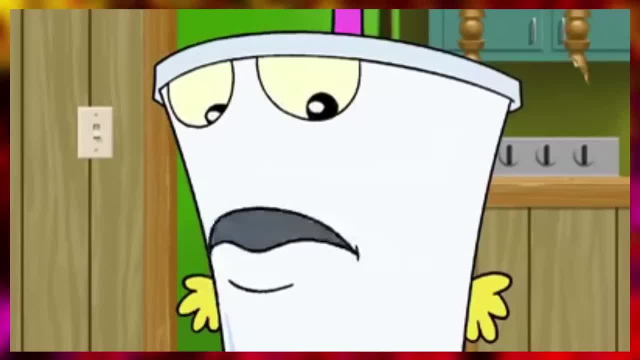 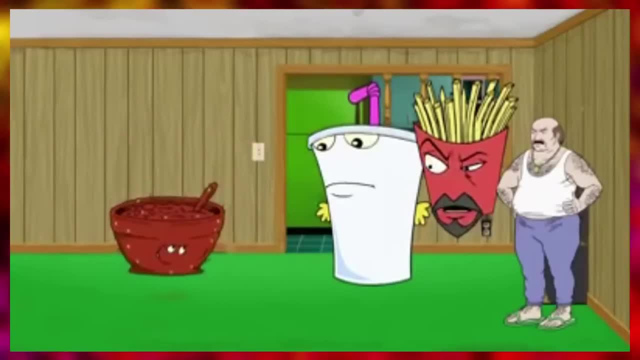 Shake Frylock and Carl playing a game of charades with Meatwad as he transforms into different flavors of Slim Jim sticks like chili, nachos and some other forms, like a cow- the word's famous phrase- and even a Slim Jim And the final Slim Jim advertisement. 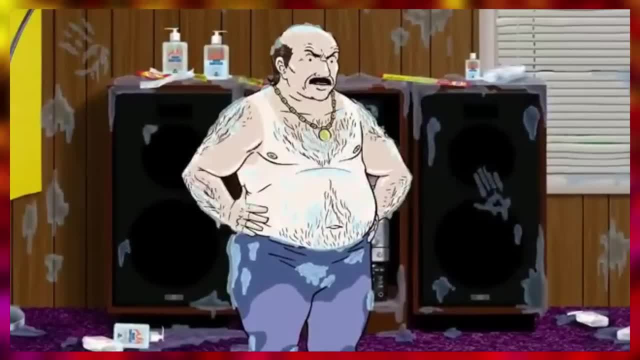 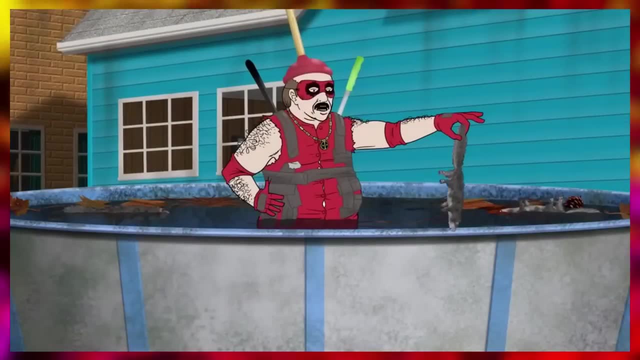 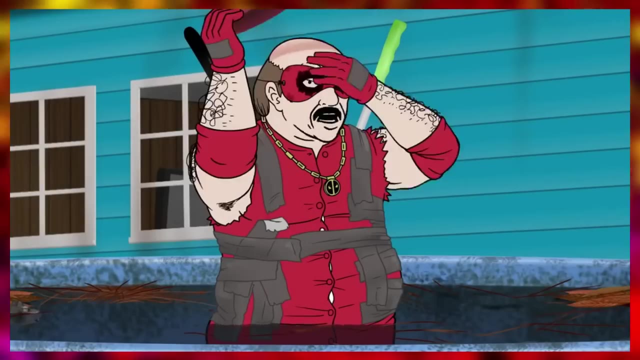 features Carl lighting himself on fire in order to portray a hot and spicy human Slim. Jim Carl's Rant on Deadpool 2. During the promotional period of Deadpool 2, Adult Swim and the Aqua Teen creators put together a promotional video featuring Carl dressed up as Deadpool and Meatwad hitting him with a flamethrower. Because why not? 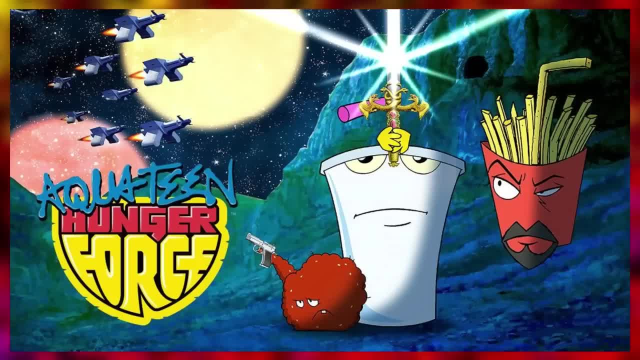 The fourth wall breaks. Wall breaks are pretty common in Aqua Teen. The fourth wall, for those of you who don't know, is the imaginary wall between us, the viewers, and the characters of the series. While it would be easier for me to just list, 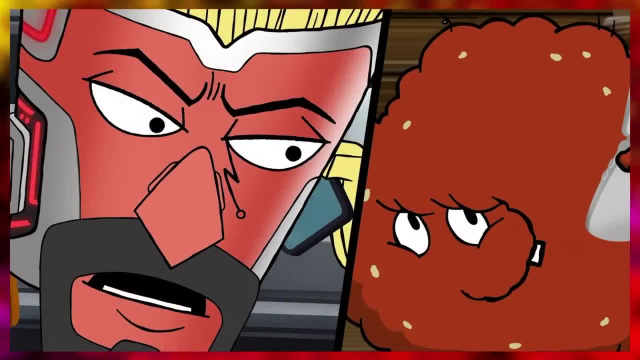 like one or two examples of fourth wall breaks in Aqua Teen. I believe in education, so here are most of the fourth wall breaks in Aqua Teen. If I missed any examples, then drop them in the comments below. At the end of the season one episode Interfection: Shake Frylock. 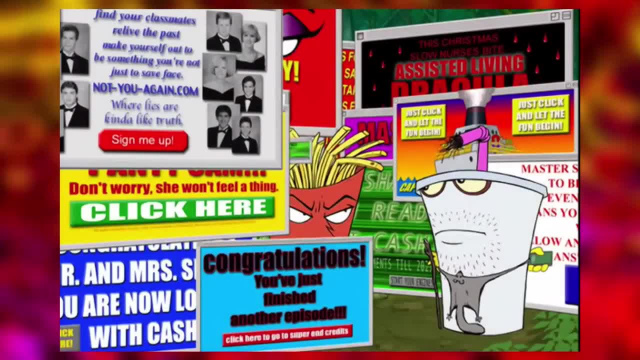 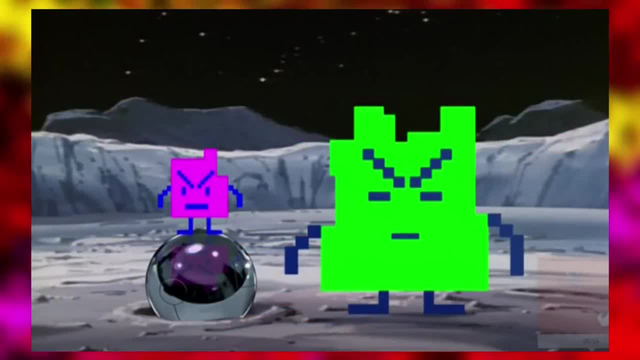 Click. clicks on a pop-up ad that says Congratulations, You just finished another episode. Click here to start the super end credits. At the end of the season two episode, Supercomputer Icknicknock looks at the camera and says: Try having omelets now, Denver. Then jumps. 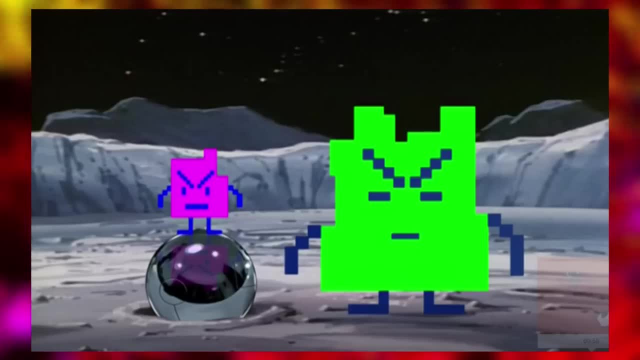 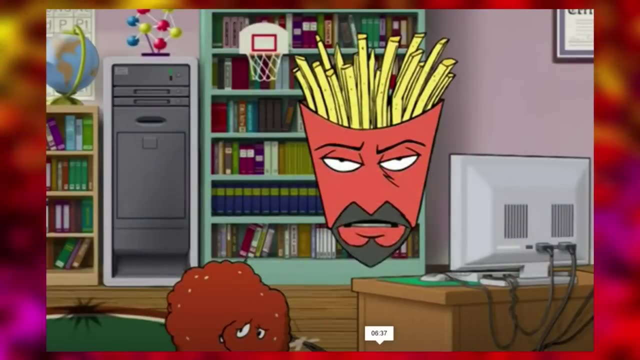 to the camera and asks: Did you hear what I said, Denver, Or should I turn it up for you? While flipping off the camera, The fourth wall is broken several times throughout the season three episode: Gee Whiz. After Meatwad asks Frylock about standards and practices. 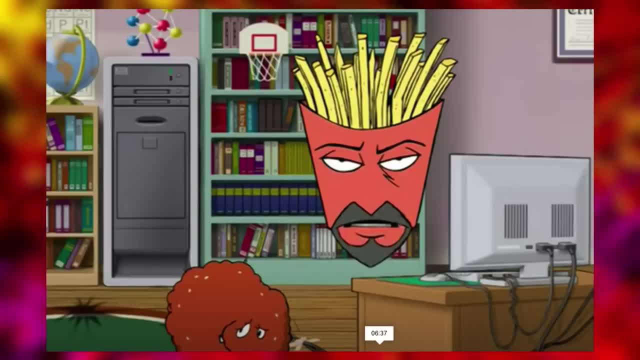 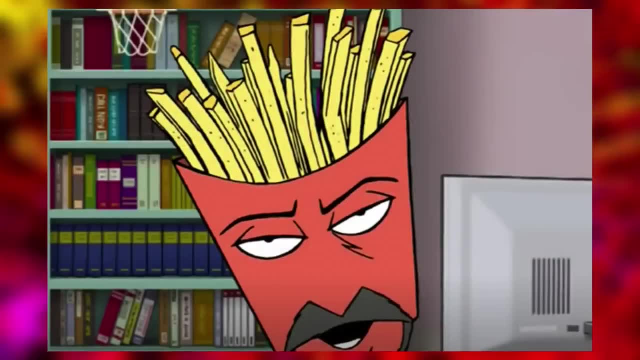 the camera before the standards and practices. video begins to play, An X sign will appear on screen throughout the episode. whenever a word is censored After, Meatwad states that he doesn't understand any of that shit, Frylock responds with: That's okay, Meatwad, No one. 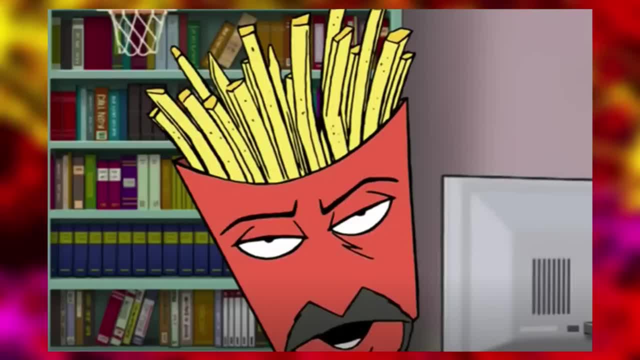 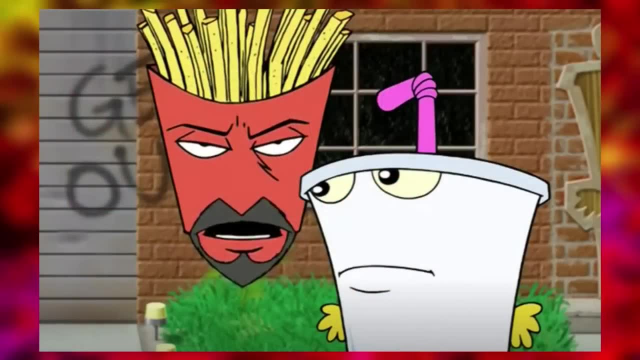 else will either. Then he smiles towards the camera And at the end of the episode Frylock breaks the fourth wall once again by saying: Well, I'm sure- glad that isn't blood- Before he turns to the camera and says I would have been offended out of my Shake also. 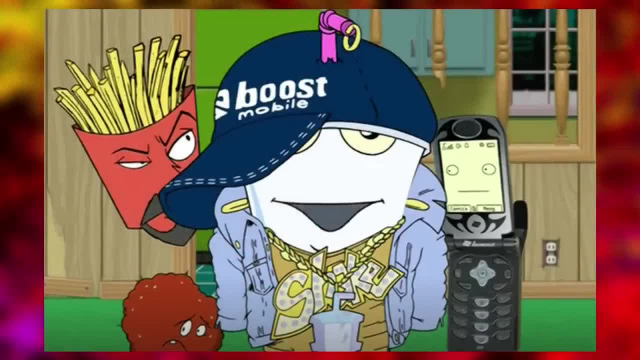 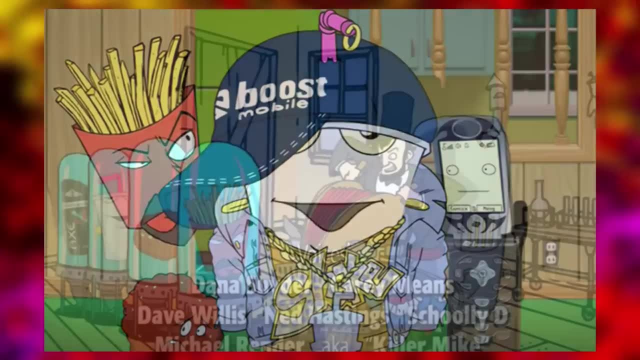 says Me too you. Shake spends a good portion of the season four episode Boost Mobile, looking at the camera and advertising the Boost Mobile phone. The X body spray appears in the ending credits of Boost Mobile as well. Shake and Meatwad show deleted scenes of the. 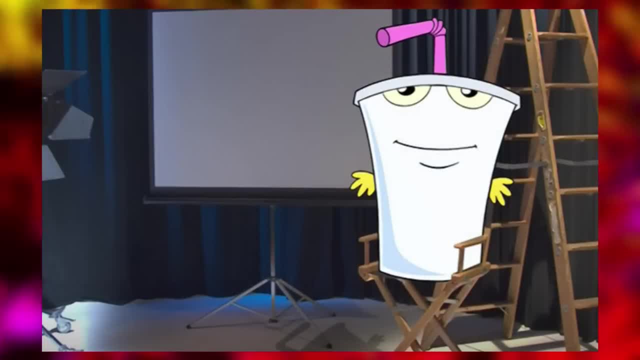 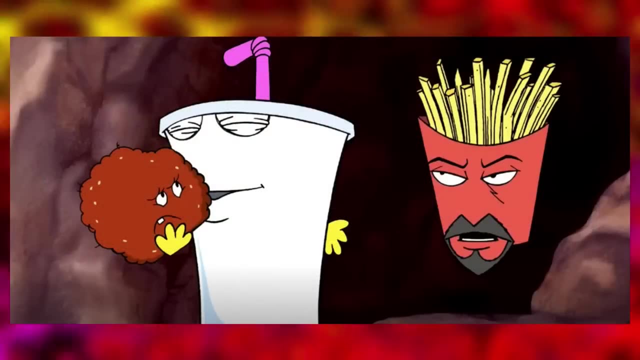 Cullen movie film. in the episode Deleted Scenes And in the season four episode, Global Grilling, Shake looks at the camera and tells the audience to eat their boogers. In the season five episode, The Marines. when Shake and Meatwad kiss in the cave, Frylock states that the kiss is 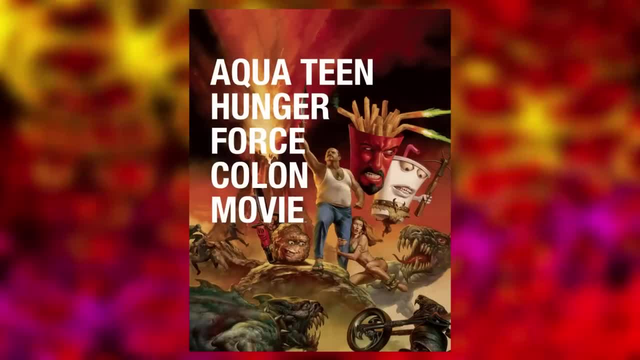 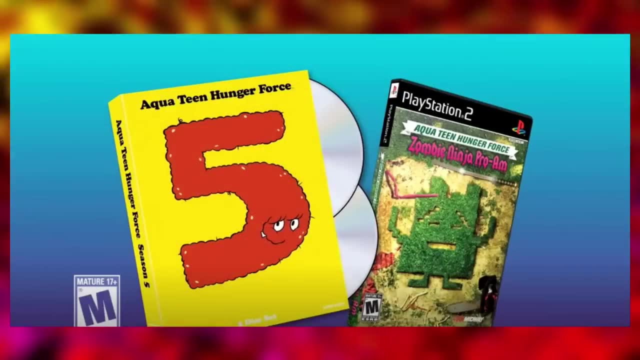 the same joke from the movie, which is referring to Cullen movie film. Then the advertisement for the Cullen movie film DVD pops up on screen, along with the volume five DVD and the Zombie Ninja Pro-Am game And, I'll be honest, this is probably my favorite fourth wall break. 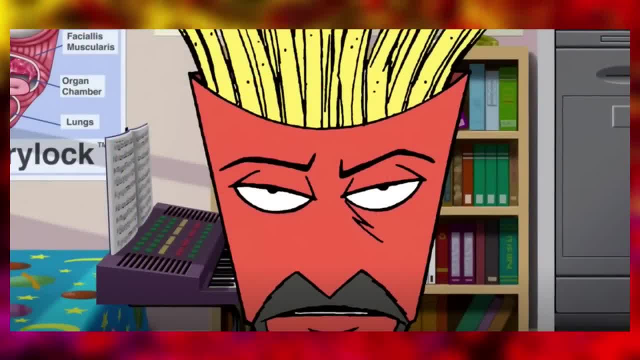 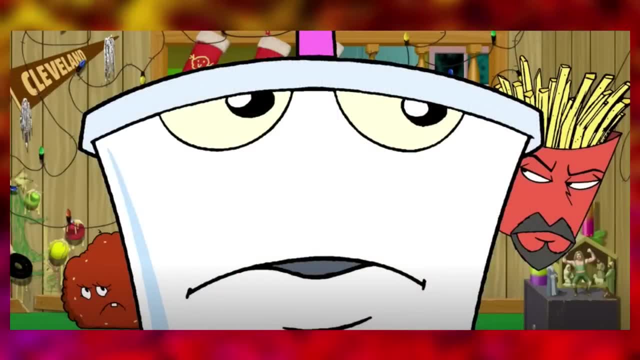 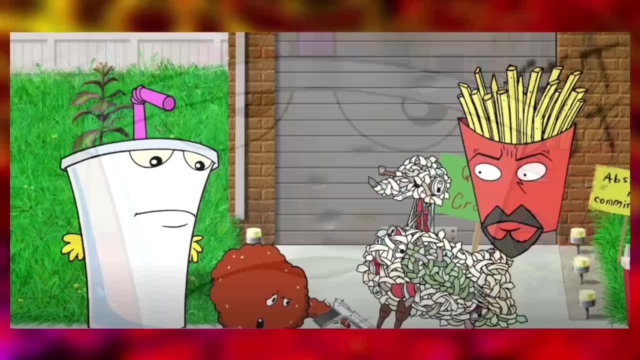 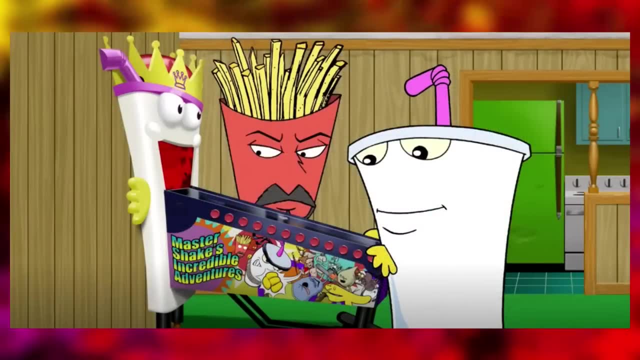 talking about? I don't know what you're talking about. I don't know what you're talking about. And talks about how something changed him at the church service. In the episode Rubberman Meatwad mentions how he wants Samuel L Jackson to appear on the show. In the episode Eggball. 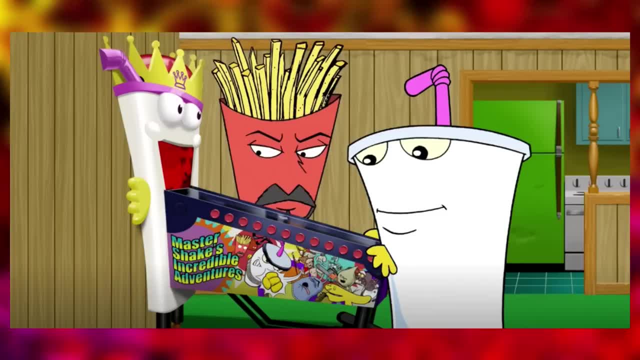 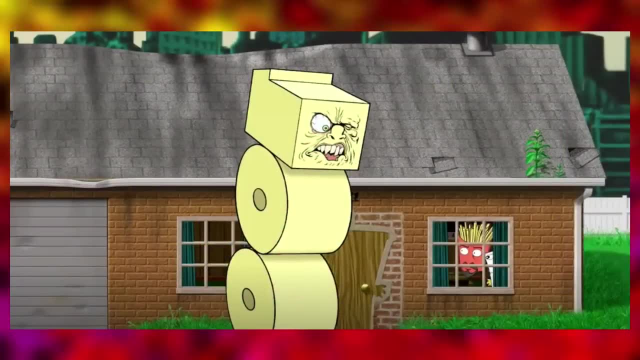 Shake mentions that Family Guy had a pinball machine and then questioned why he didn't have one. There are several fourth wall breaks throughout the 100th episode, like the 100 monster trying to tell Frylock about the 100th episode of Aqua Teen Hunger Force, And when Shake 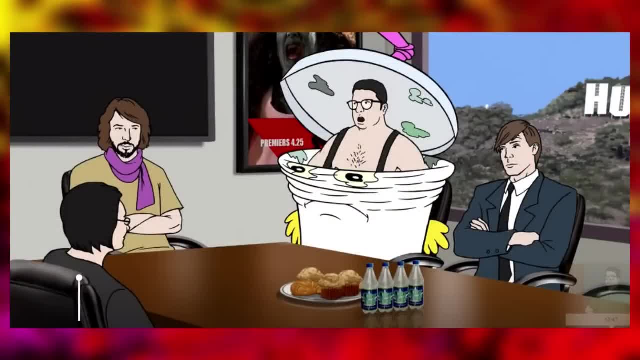 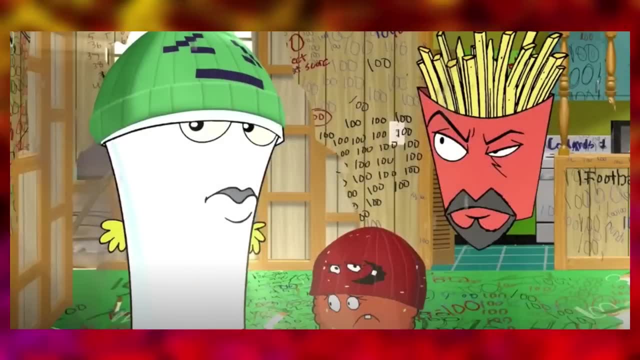 takes a flight to Century City, California- Shake says- I don't know what you're talking about- to confront the Adult Swim executives. in which Dana Snyder, the voice actor for Shake, pops out of Shake's body and confronts the executives about being underpaid for years. 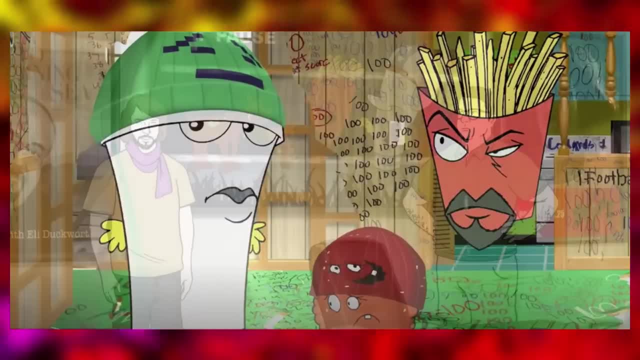 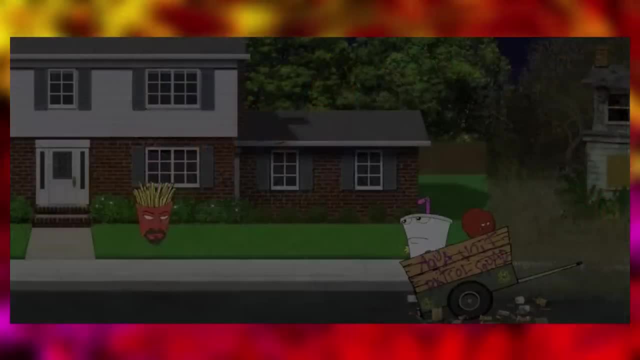 And during the end credits when Dana Snyder shows the Aqua Unit Patrol Squad episode to the Adult Swim executives, which they don't enjoy because of some of the jokes going too far. In the episode, Alan Parts 1, Frylock and Shake briefly discuss the state of the old and new series. At the end, 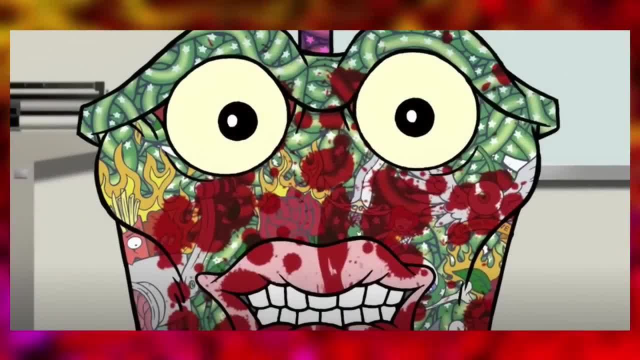 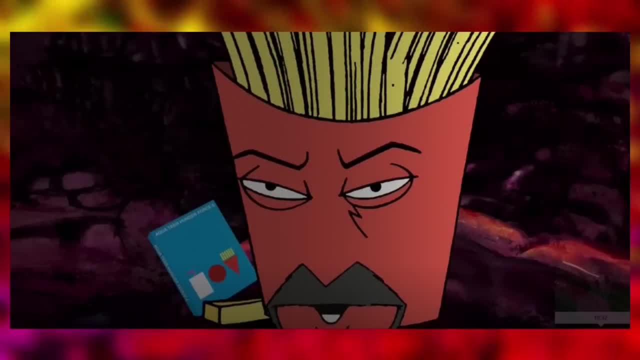 of the episode Freedom, Cobra Shake states that no one can tell that he's sad before looking at the camera and says after I've eaten them. In the episode Vampirous, Frylock pulls out the volume 6 DVD but mistakenly calls it season 8.. In the episode Lasagna, Lance advertises his 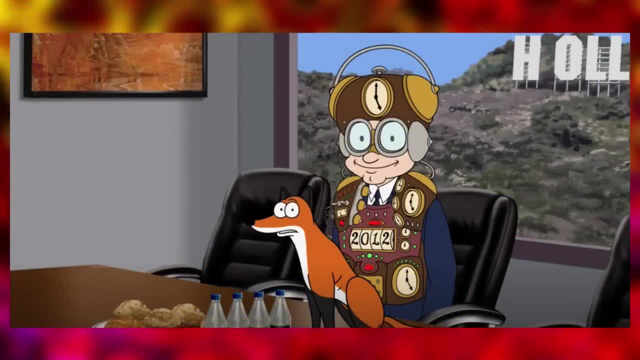 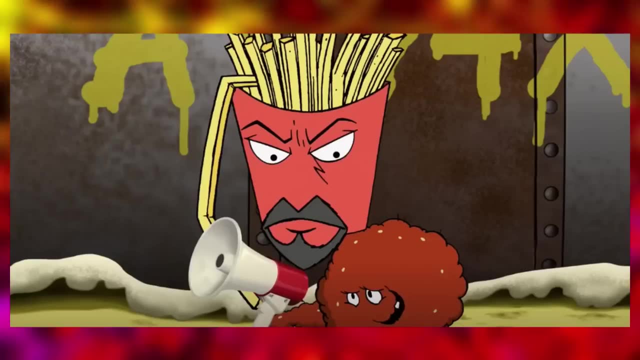 products from ScamWow. In the season 9 episode, The Granite Family, The Fox looks at the viewers and says Sunday's at 9.. In the episode Banana Planet, after Frylock introduces themselves to the monkeys, Meatwad sings the Aqua Teen Hunger Force theme song. In the episode Working Stiffs: 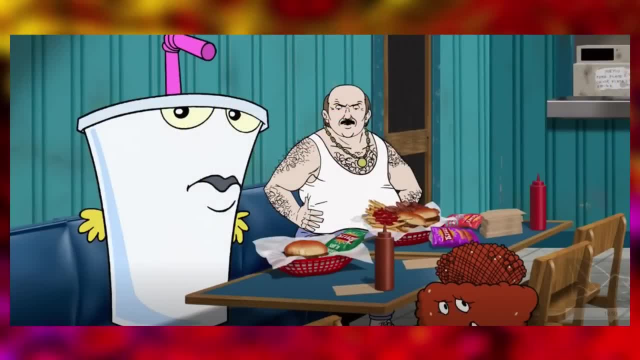 when Carl, Meatwad and Shake are discussing the assassination plan and Meatwad explains that he's going to buy all the cable TV he wants after getting his cut. Carl asks Meatwad if he's out of his mind for paying for cable TV. And then all three of the characters look at the camera and 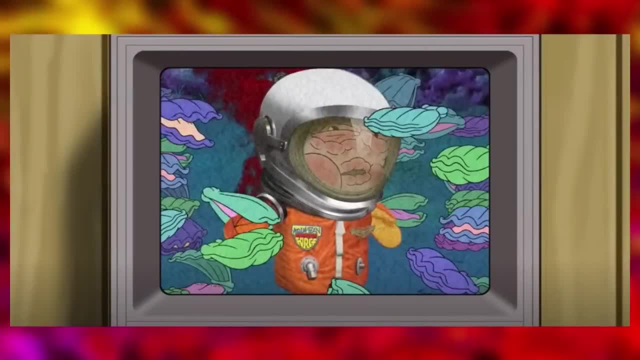 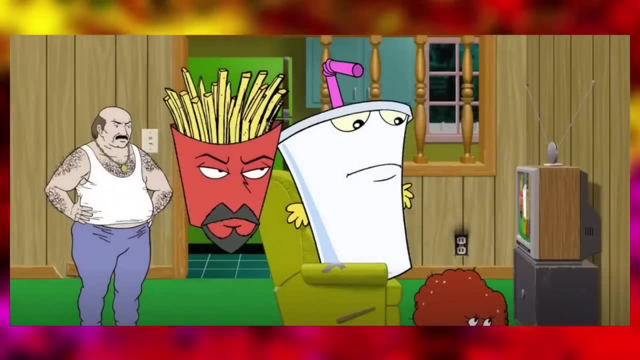 say you're stupid. And finally, in the season 11 episode, The Greatest Story Ever Told, Shake and Meatwad are seen watching the previous week's episode And in the post-credits scene for the episode, the Aqua Teens and Carl mention the end of the series. 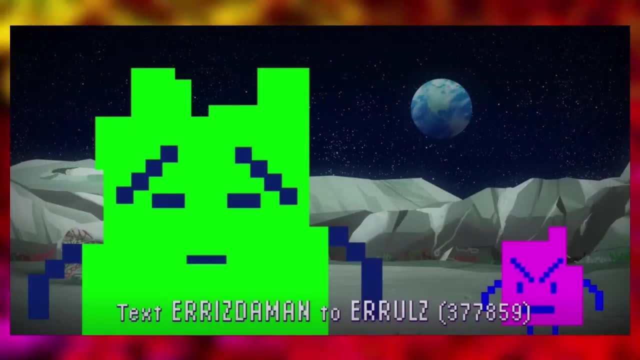 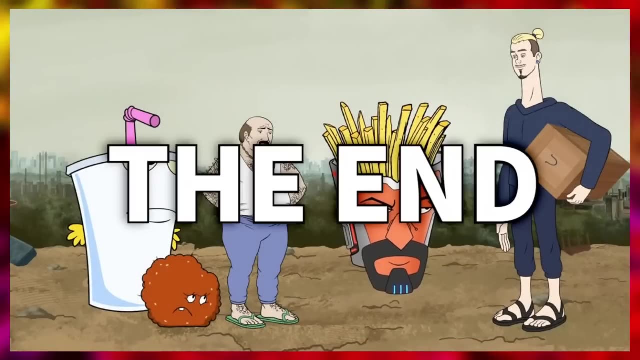 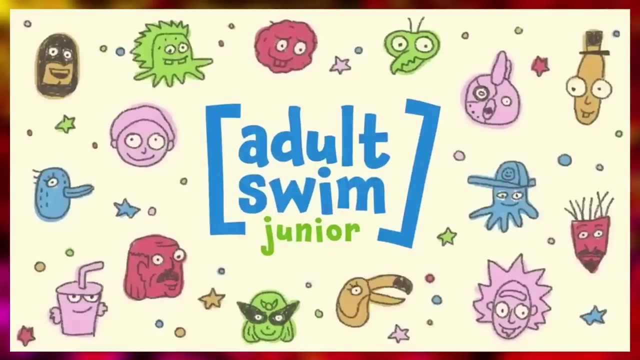 Aqua Child Hunger Force. On April Fool's 2021, Adult Swim became Adult Swim Junior, A kids block which possibly spoofed the then-upcoming preschool. Cartoon Network block Cartoonito Shows and bumpers were dubbed over using children's voice. 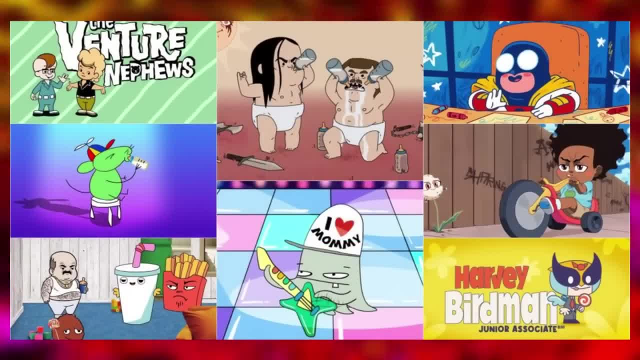 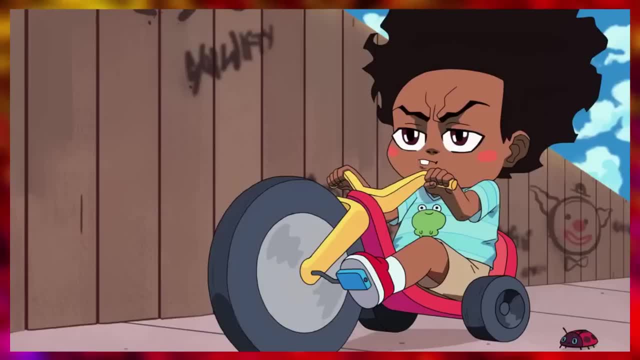 With some adult language replaced with more child-friendly terms. Basically what we're forced to do here on YouTube now. Thanks a lot, you corpos. Many Adult Swim properties were reanimated in a child-like style for the bumpers that premiered that night, Like Space Ghost, which 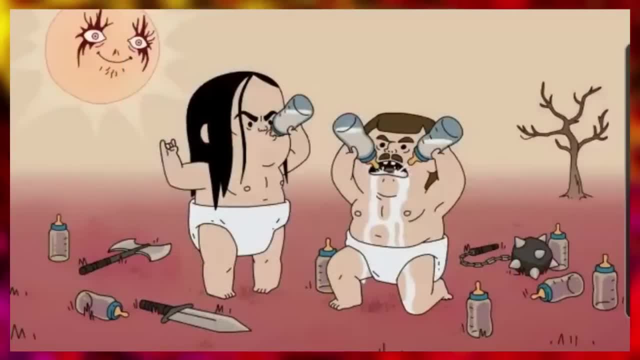 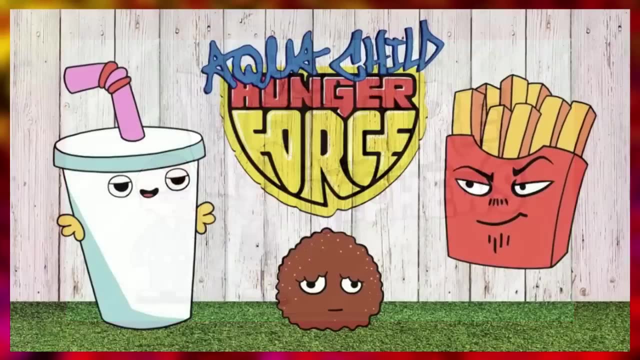 became Space Kid. Crib to Crib. Metalocalypse, which became Metalocalypse Babies, The Venger Bros, which turned into The Venger Nephews, And, of course, Aqua Teen Hunger Force, which was turned into Aqua Child Hunger Force. Only two shows that. 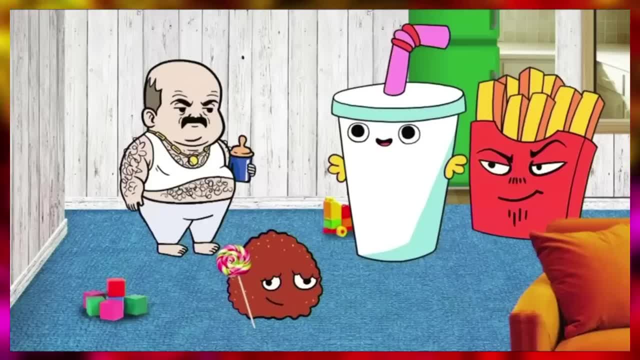 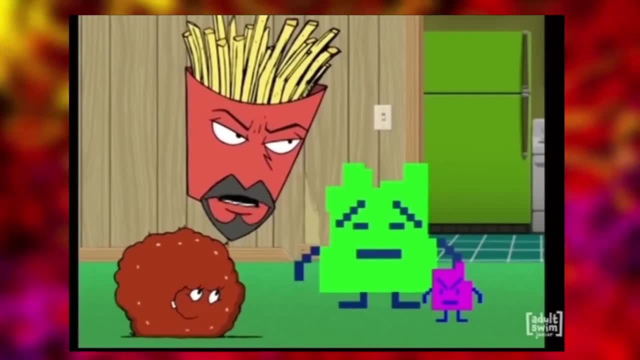 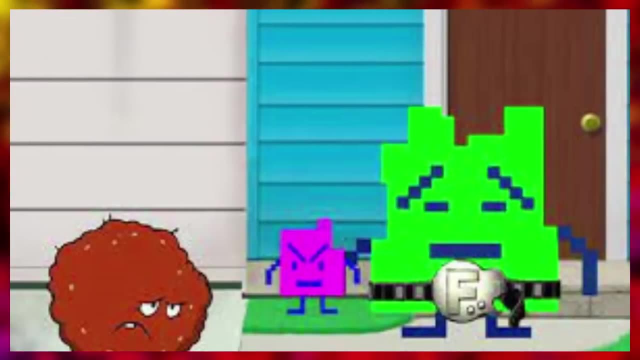 Moonanites received the Adult Swim Junior treatment, Rick and Morty and Aqua Teen, Specifically the episode Revenge of the Moonanites. The episode was fully dubbed over using child voice actors And, yes, that includes the intro and outro. The full dubbed over episode can be found on Archiveorg and I totally recommend. 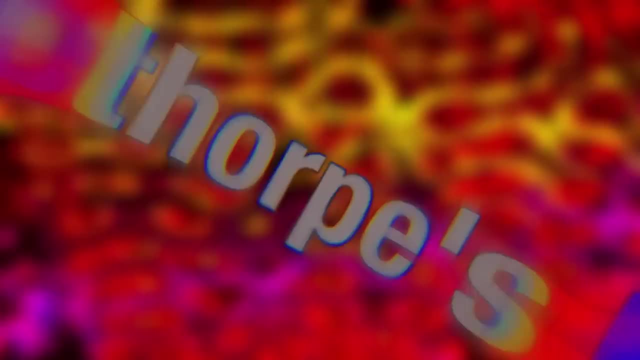 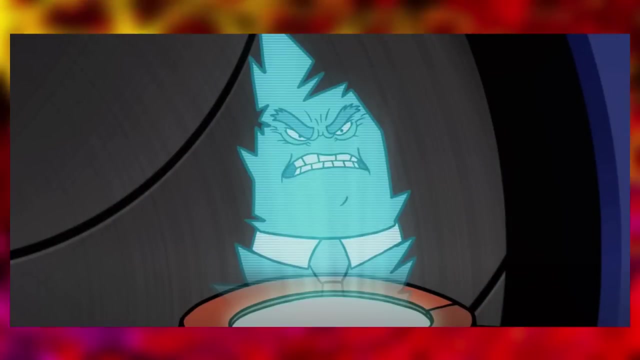 checking it out because it's just hilarious. Oglethorpe's Dad. Oglethorpe's Dad. The episode Space Caduce, to my knowledge, is the first and only time in the series where we get to see a new Plutonian character. Prior to the episode, Oglethorpe and Emery are the 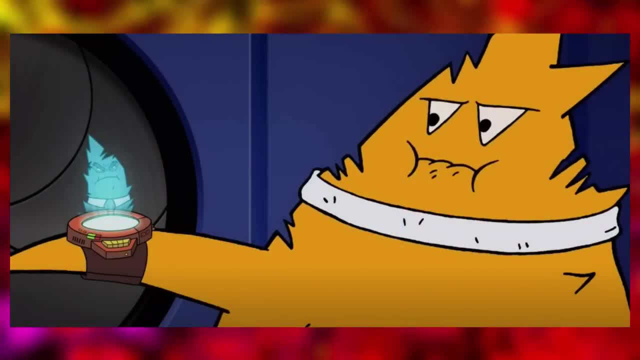 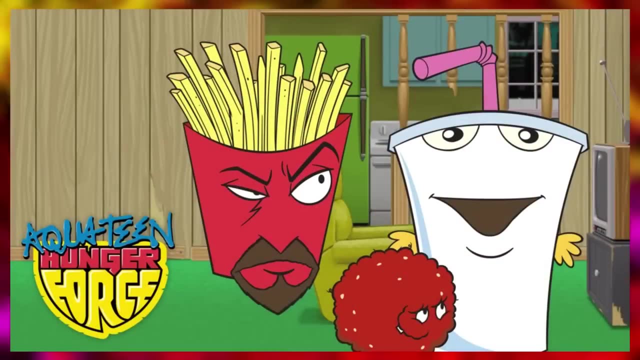 only two Plutonians shown in the series, But at the end of the episode we are introduced to Oglethorpe's dad, Boston. Boston is an episode of Aqua Teen Hunger Force that parodies the 2007 Boston Scare. It was. 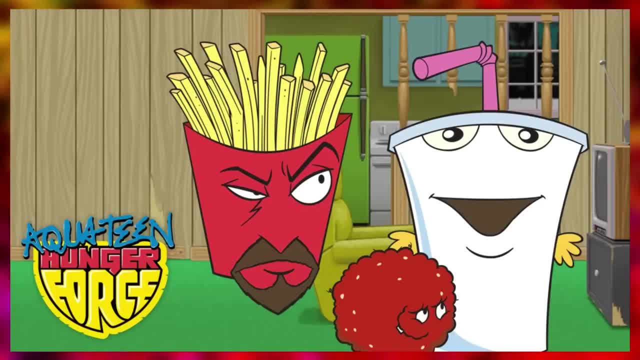 supposed to be the first episode of season 5,, but was pulled out of production. Boston is the first episode of season 5,, but was pulled by Turner Legal to avoid further controversy surrounding the incident and was never formally released. The episode had allegedly went through. 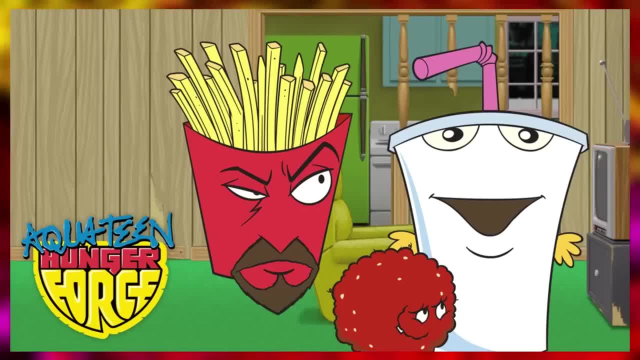 several rewrites and edits due to the network, who were concerned about the episode, which resulted in three different versions of Boston, all of which were ultimately rejected. However, an unfinished version of Boston leaked online in January of 2015,, eight years after the. Boston incident. The leaked Boston episode was uploaded to the internet in January of 2015,, eight years after the Boston incident. The leaked Boston episode was uploaded to the internet in January of 2015,, eight years after the Boston incident, The leaked Boston episode. 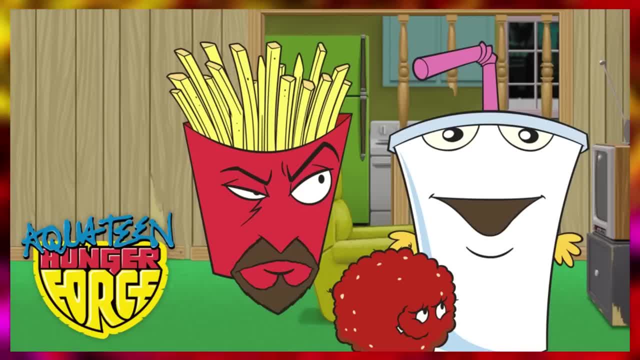 was uploaded to YouTube and went virtually undetected until news outlets and websites began to report on the incident. While the original upload was removed from YouTube, people have saved and reuploaded the episode onto other websites like archiveorg, which you can check out if you want to get a taste of Boston for yourself- Not the city just. 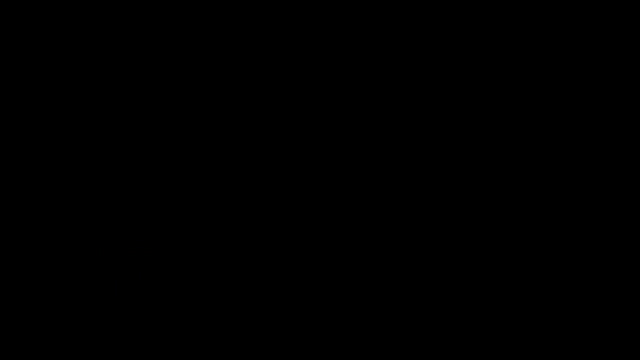 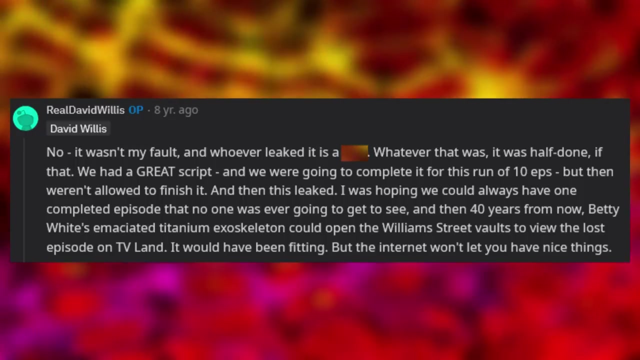 the episode. Stay far away from Boston, Unless you like to get yelled at. According to a statement from Dave Willis in regards to the leaked episode he mentioned was going to be completed for the current run of the show they were working on at the time. 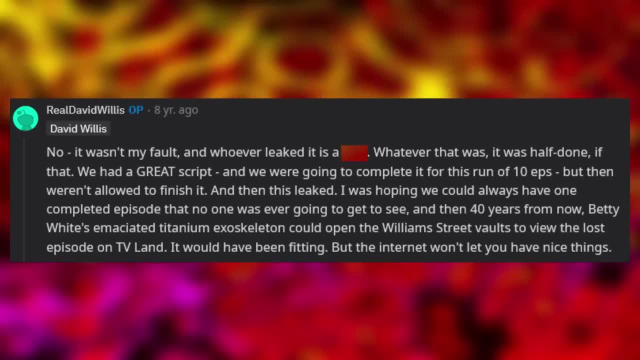 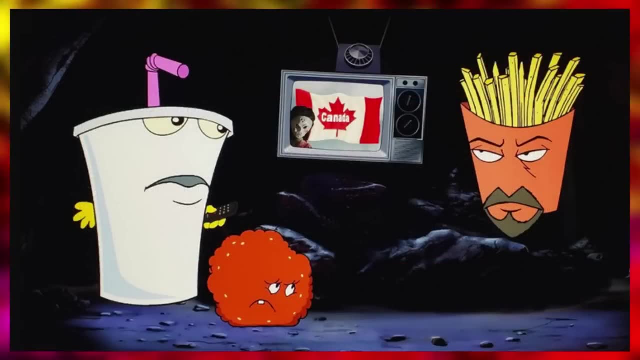 but then they were not allowed to finish it, and then the episode leaked, And whoever leaked it is a giant jerk. However, the Boston assets did not go to waste. Towards the end of the leaked Boston episode, the Moonenites are seen in a dark cave wearing beards and turbans and standing in. 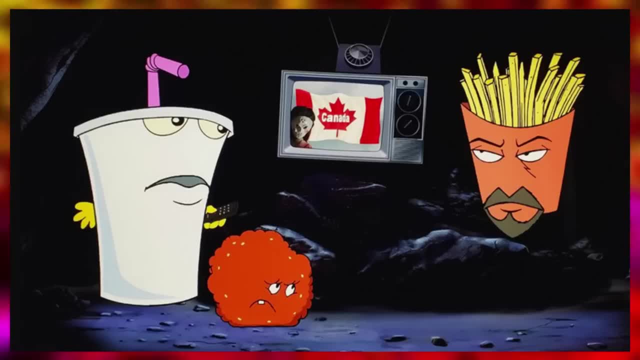 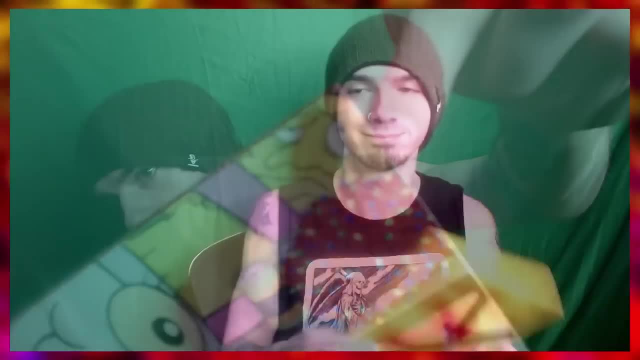 front of a TV. That same exact cave was repurposed for the episode The Marines. Not only that, but the art of Ignignok and Ur dressed up with turbans and beards, and even Meatwad wired up, can be seen on the artwork for the Volume 5 DVD box set And elements of Meatwad dressed up as a 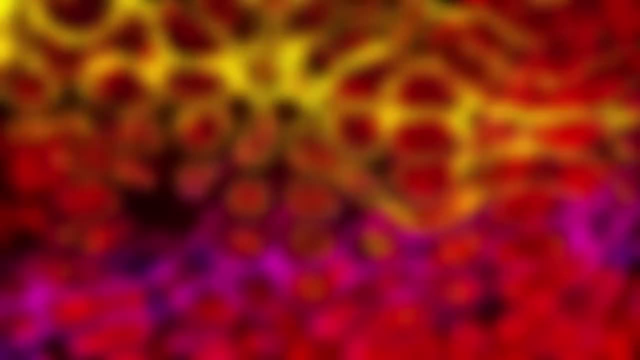 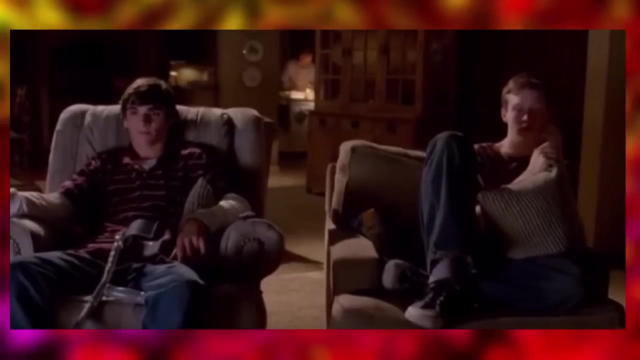 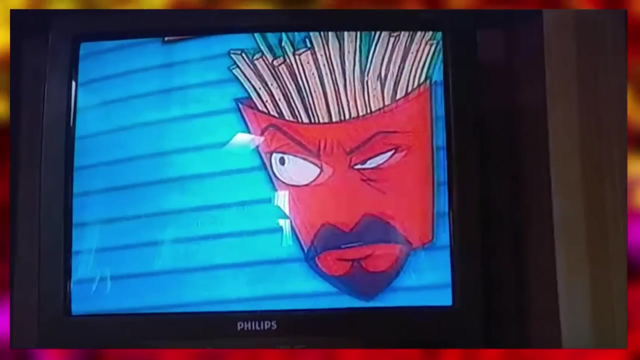 rapper, were reused in the episode Bookie. The Breaking Bad Cameo. In the Breaking Bad episode IFT we can clearly see Walt Jr watching the Aqua Teen episode. Chick Magnet. The Sopranos Cameo. In the Sopranos episode Johnny. 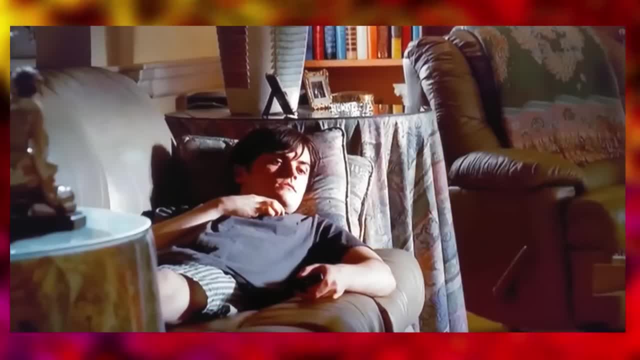 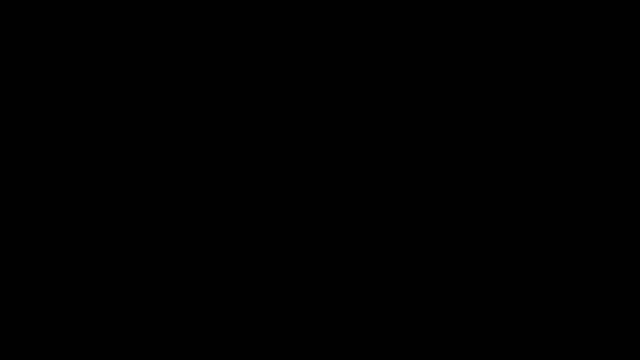 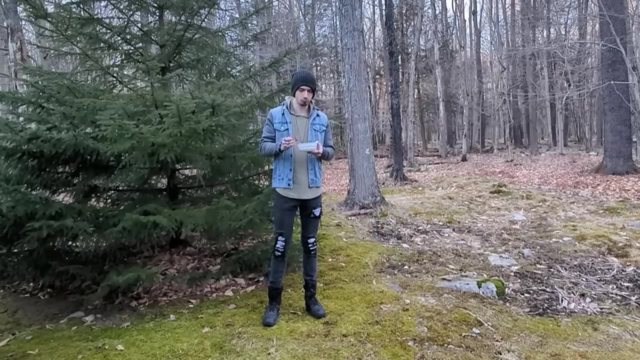 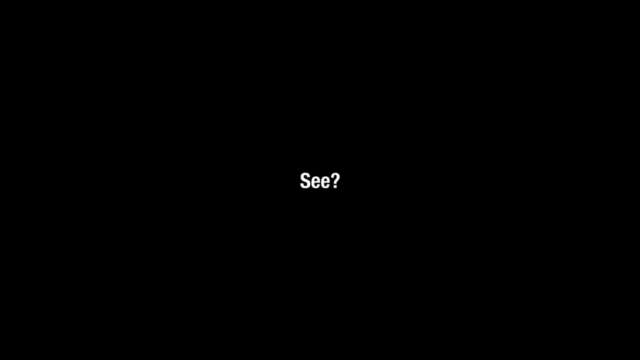 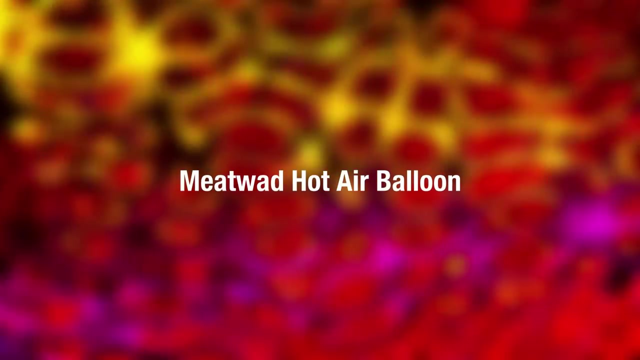 Cakes AJ is seen on the couch watching the Aqua Teen episode Escape from Leprechaunpolis. And that, my friends, was the third layer of the iceberg. I found a perfectly good hot dog in the trash Meatwad Hot Air Balloon. In the wonderful year of 2010,, the Adult Swim Shop offered two 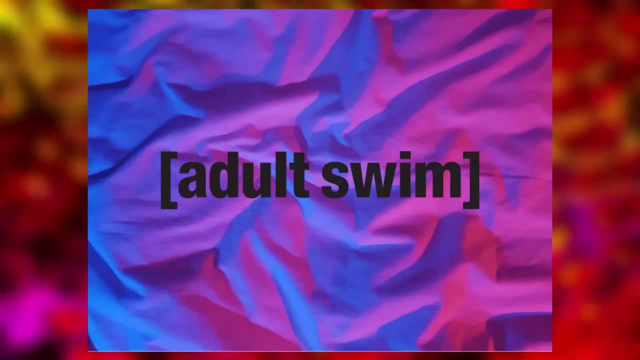 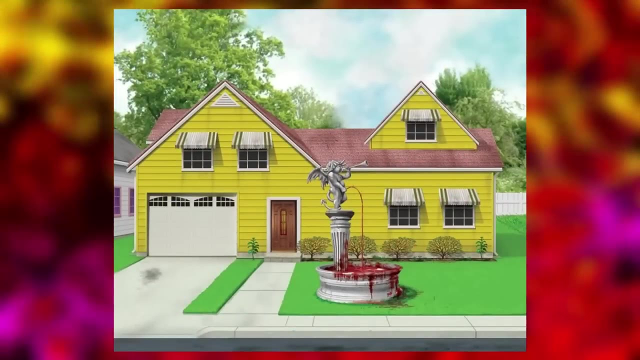 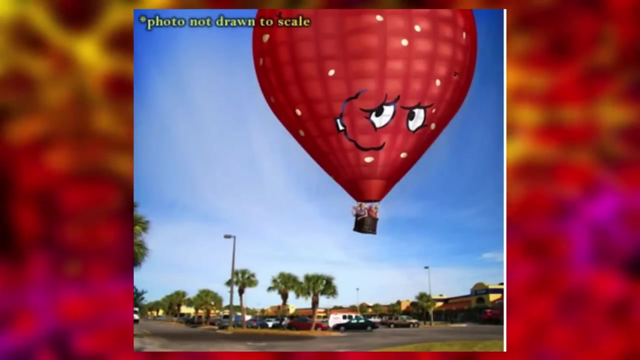 very outlandish items inspired by two popular IPs owned by the network: A Metalocalypse Blood Fountain, which I discussed more in the Metalocalypse Iceberg video, and, of course, the Aqua Teen Meatwad Hot Air Balloon. This balloon was listed on the Adult Swim Shop for. 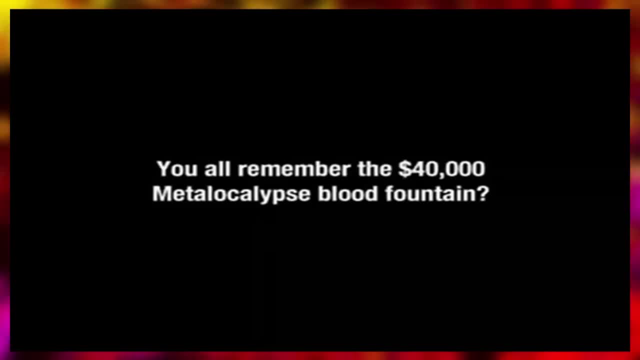 $70,000.. Sweet Captain Christ. And during the period of time when the balloon was available, nobody reportedly purchased it. There are also no photos of the finished balloon, because the product was intended to be built upon order. The same goes for the Metalocalypse Fountain. 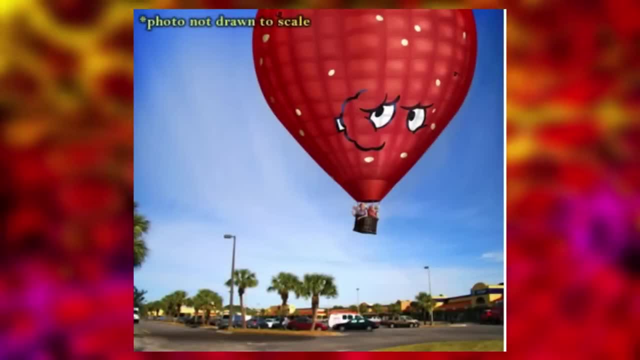 which nobody purchased as well. The product description for the balloon states the following: Let's assume that you're an Aqua Teen- Hunger Force fanatic, granted- who has amassed a ridiculous fortune because- why not? And wanted up a huge chunk of change financing a series of fantastic. 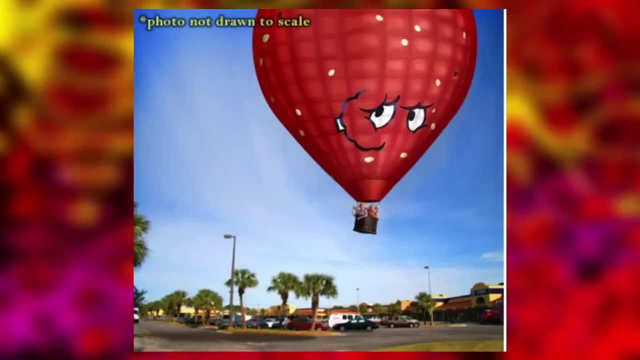 voyages, obviously. How exactly does one begin such an undertaking? What's the crucial part of this? Allow us to make a suggestion: Use a meager portion of your vast disposable wealth to purchase a big honkin' Meatwad Hot Air Balloon of your very own. 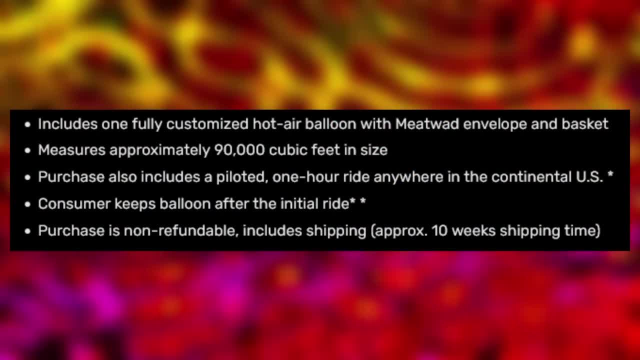 Includes one fully customized Hot Air Balloon with Meatwad envelope and basket Measures approximately 90,000 cubic feet in size. Purchase also includes a piloted one-hour ride anywhere in the continental US. Consumer keeps balloon after the initial ride. Purchase is not refundable. 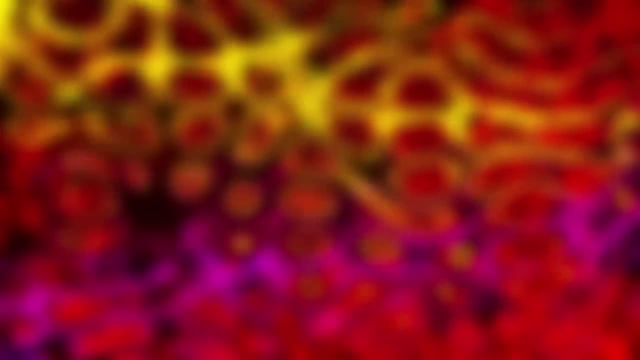 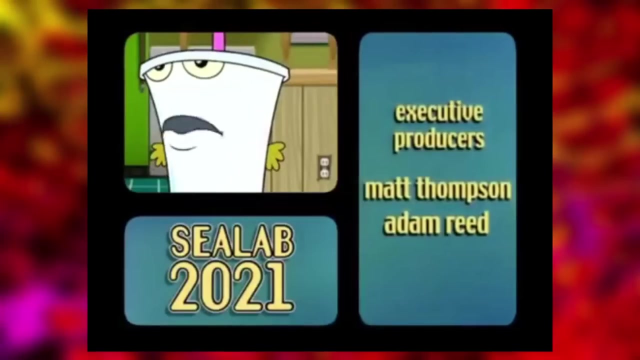 Includes shipping: approximately 10 weeks shipping time. The Sea Lab 2021: Cameos, Aqua. Teen characters have been seen in the classic Adult Swim series Sea Lab 2021, on a number of occasions, Like at the end of the Sea Lab. 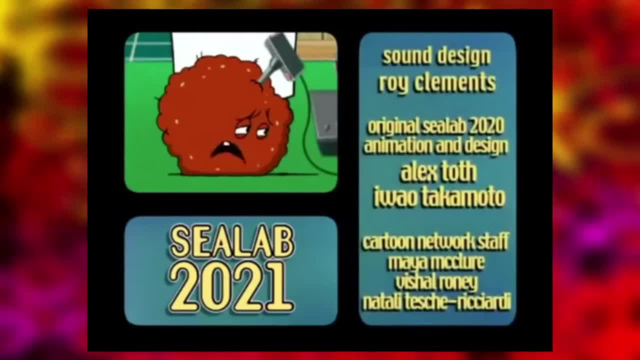 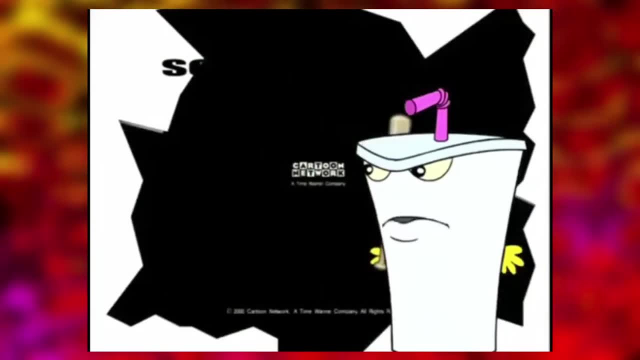 2021 episode: Murphy Murph and the Feng Shui Bunch. When Shake starts beating up Meatwad, the game console, the 7030 Productions logo, the William Street logo and the Cartoon Network logo, because he sucks at video games. The Aqua Teens are also seen in the episode Predator And Aqua. 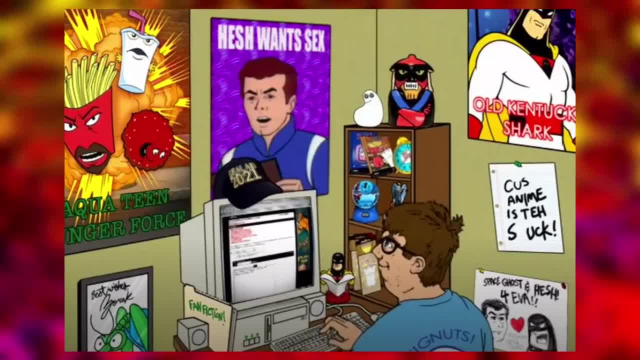 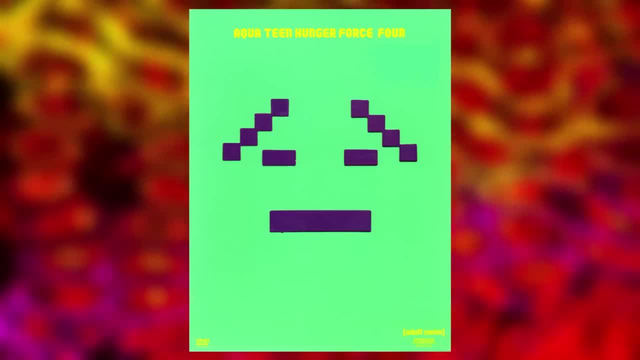 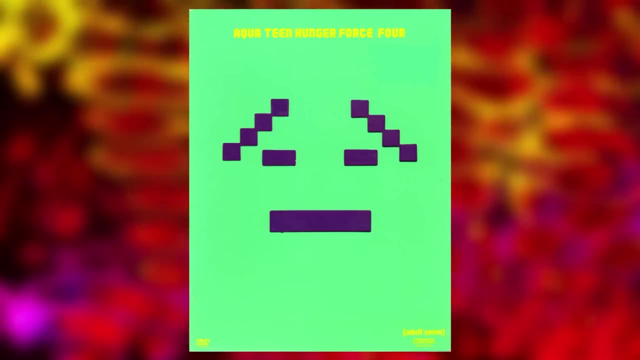 Teen. merchandise is visible at the end of the episode Dearly Beloved Seed. The Volume 4 Playlist. There is a feature on the Volume 4 DVD of Aqua Teen Hunger Force called Play All. Now it's common for DVDs or Blu-rays of TV shows to have a Play All feature, as it would allow for all episodes on 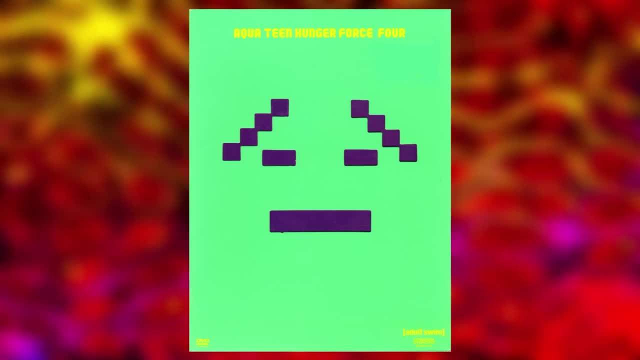 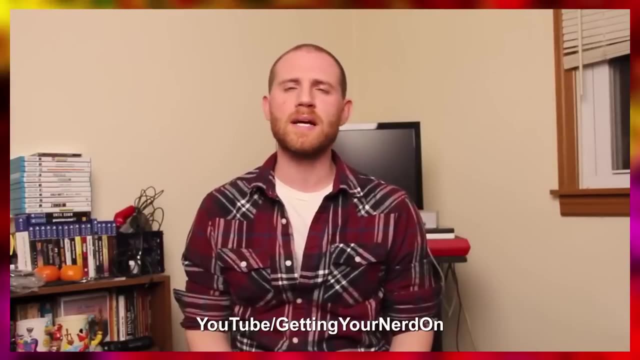 the disc to play back to back without any interruptions. However, Aqua Teen takes that concept and shoves it inside of an air fryer. YouTuber, Getting Your Nerd On- made a video explaining how the Play All feature on the Volume 4 DVD allows users to play every single episode. 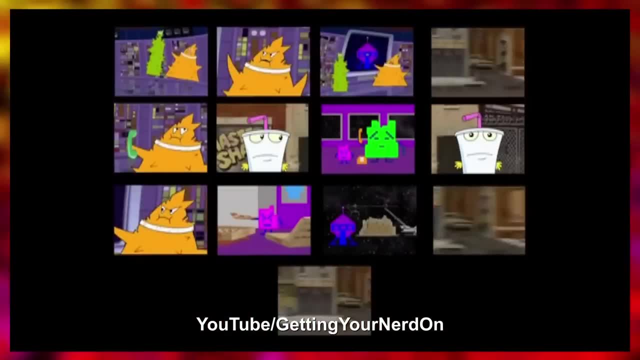 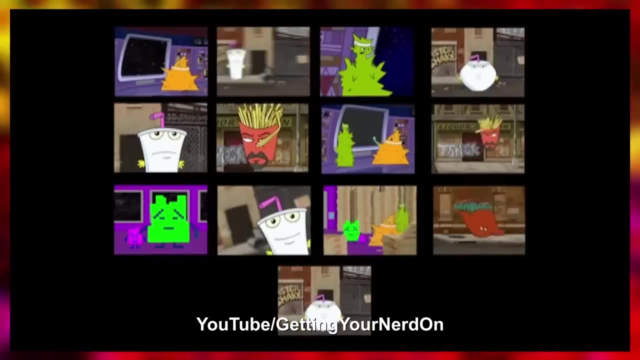 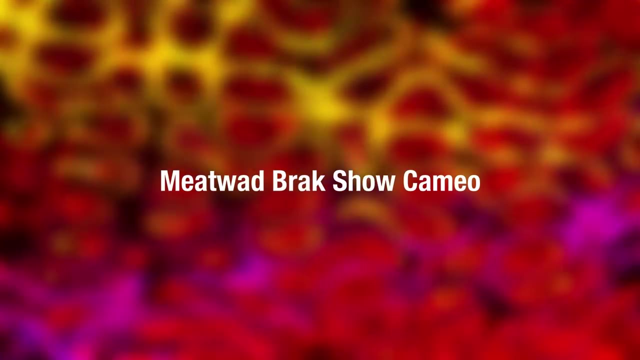 on the DVD all at once, Back to back. I mean every single episode on the disc plays on screen at the same time and it sounds exactly like how you would imagine it to sound. It sounds like being trapped inside of a crowded DMV. Meatwad Brack Show- Cameo In the Brack Show episode Brack Street- Men in the Band. 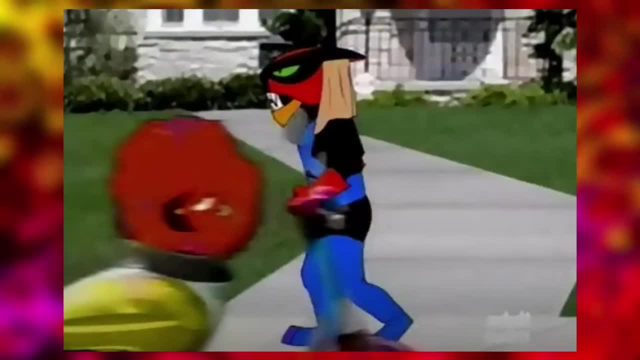 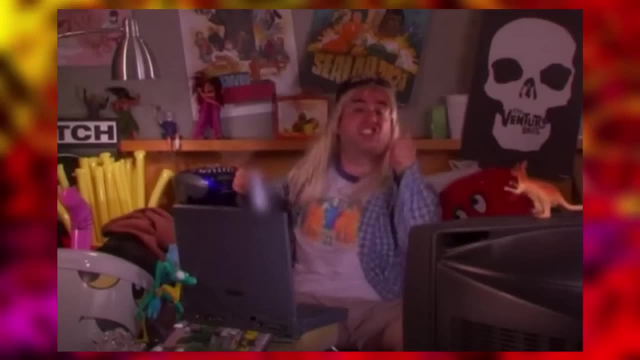 as Brack walks down the sidewalk rapping, there is a brief moment where you can clearly see Meatwad riding on a scooter. The Robot Chicken Cameos, Meatwad, Frylock and Shake are seen in the Robot Chicken episode. Plastic Buffet Shake is seen in 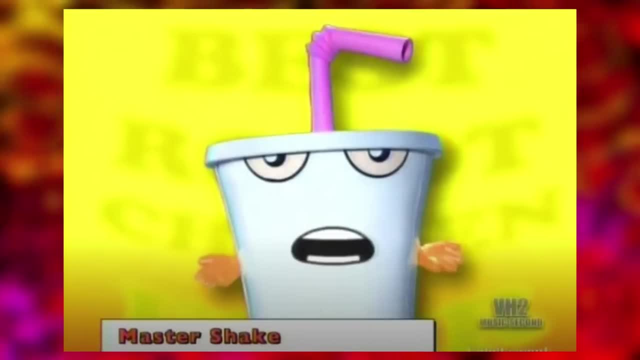 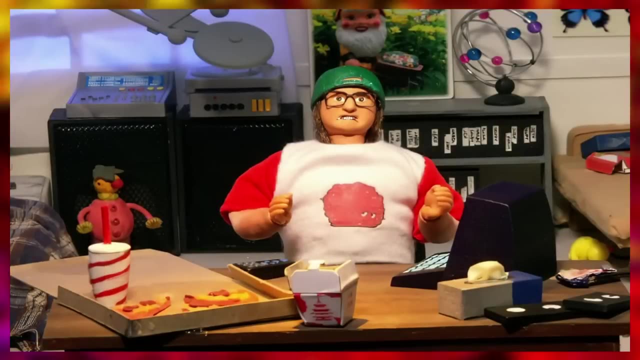 multiple episodes like Suck It 1987, and Immortal. In the episode Book of Corinne, the annoying fat Reddit moderator is seen wearing a Meatwad t-shirt. The Kid is also seen in the episode Werewolf vs Unicorn. The Meatwad t-shirt is also featured in the episodes in a DVD factory. 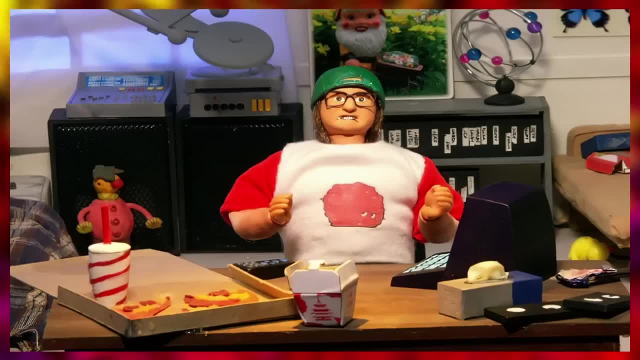 I love her President Who forbids it, and the Robot Chicken. lots of holidays, but don't worry, Christmas is still in there, so pull the stick out of your ass. Fox News Special. These are just the references and cameos that I could. 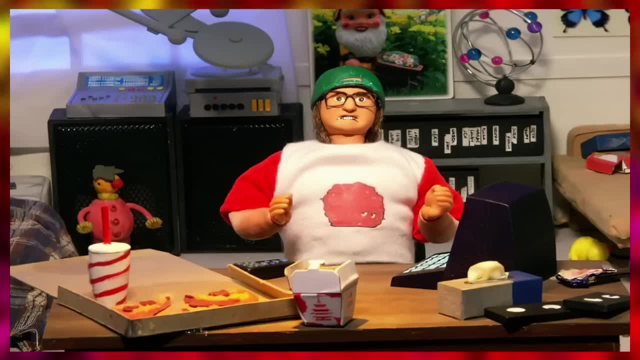 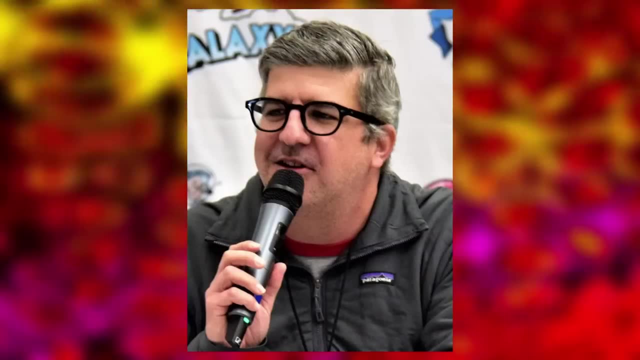 find I'm positive. there are tons of others, but I think you guys get the point. Dana Snyder Drunk Voice Message. This entry refers to the fact that Dana Snyder got the job of voicing Master Shake through an old college friend who went to high school with Dave Willis. Ronnie will. 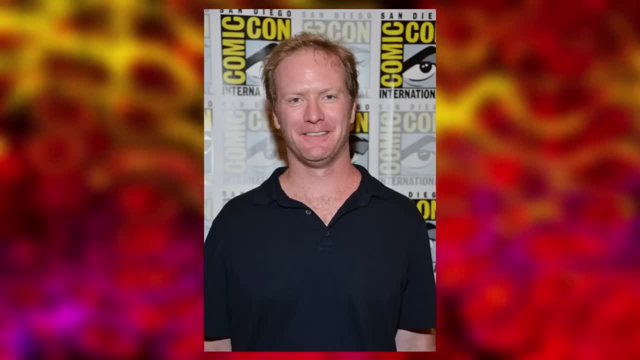 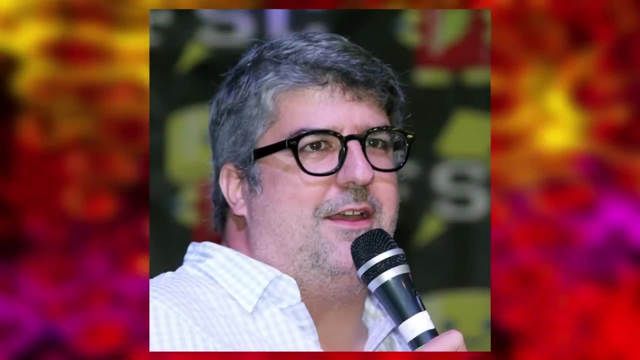 be talking more about this old friend later on in Layer 7.. But basically Dave was looking for voice actors and his friend recognized him as a voice actor. He was also looking for a voice actor who recommended Snyder. So Dana got drunk and left a very wild voice message on Dave Willis' answering. 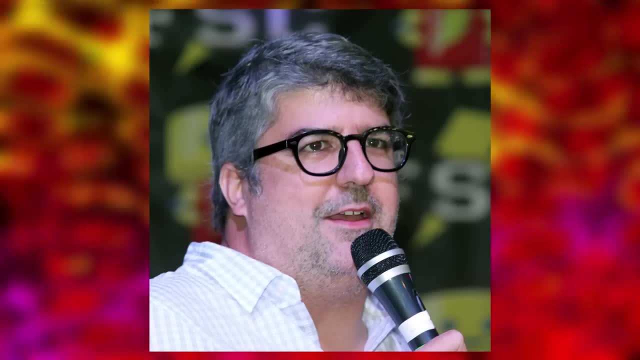 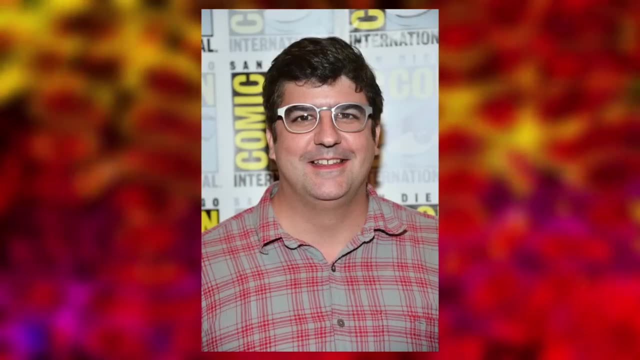 machine And Dave loved the messages but accidentally erased the recording and asked Dana to re-record himself, which he did, but this time sober. However, Willis wasn't super ecstatic on the second recording, so he asked Dana to try again and make it sound like the first drunk. 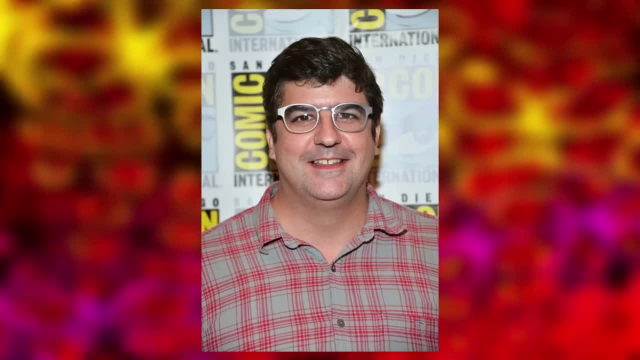 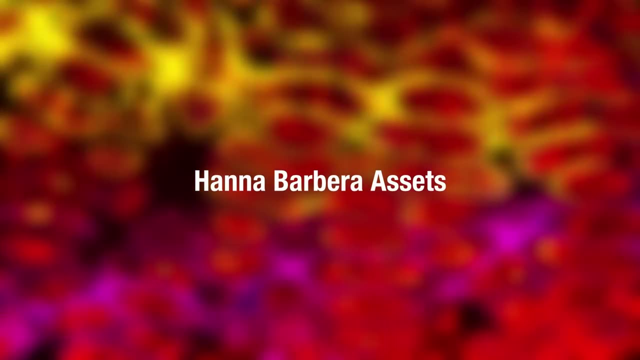 recording. And as to not disappoint Dave Snyder went out with some friends, got wasted and left another 3am message and was given the job of voicing Master Shake. So Dana got drunk and left a Hanna-Barbera Assets. Much of the backgrounds and features from the early episodes of Aqua Teen were assets. 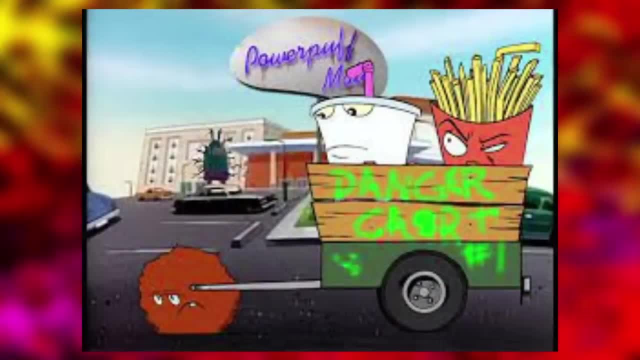 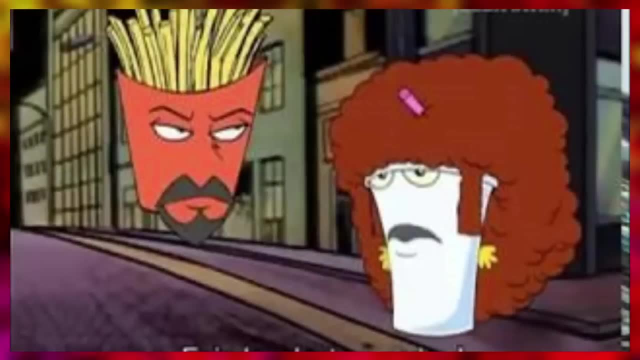 from Hanna-Barbera shows like Swat Cats, Johnny Quest and even the Powerpuff Girls, Some examples being Olgar's Space Ship, which was recycled and given to the Plutonians Downtown in the episode Rabot, the Powerpuff Mall, which was used in the pilot episode of 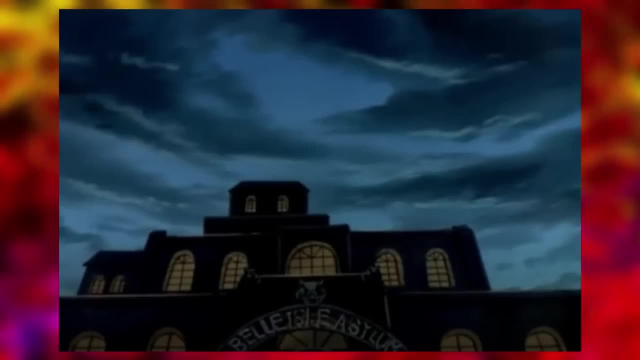 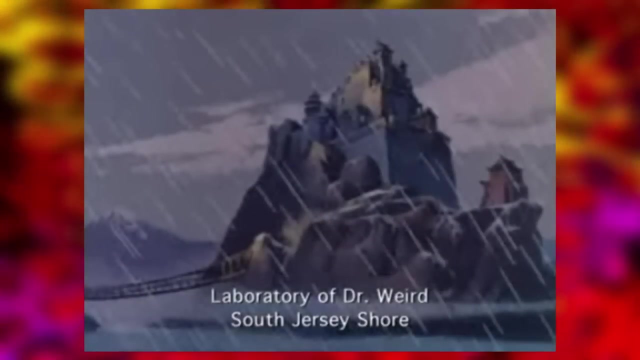 the Powerpuff Girls. the Belle Isle Asylum entrance scene, which was taken from the 1996 Johnny Quest series and the shot of Dr Weird's Castle was originally the Himalayan outpost from the Monster in the Monastery episode of the 1964 Johnny Quest series. 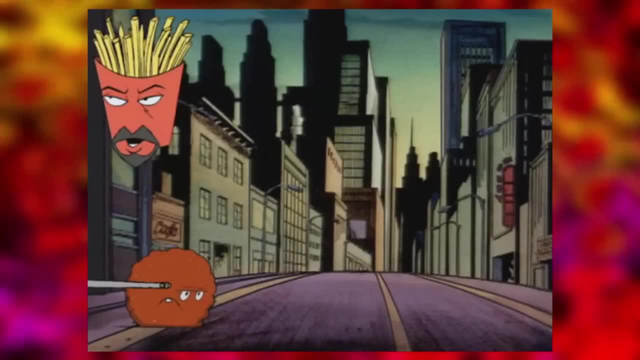 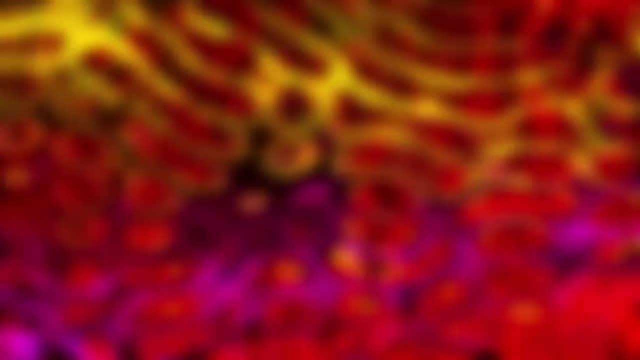 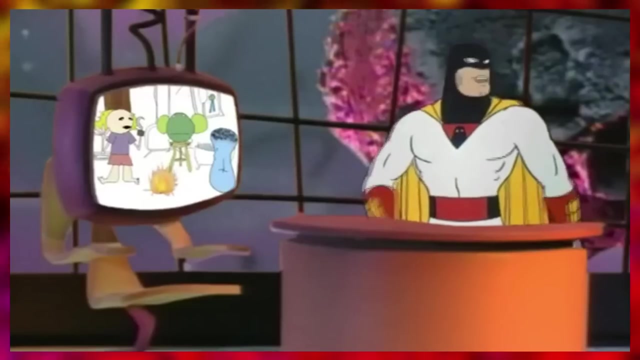 The reason why Aqua Teen used a lot of these assets in early episodes was simply because the network just didn't have a lot of money at the time but had complete access to the Hanna-Barbera library. 12 ounce mouse references In Aqua Teen. Hunger Force, colon movie film for theaters: Space Ghost before being demolished. 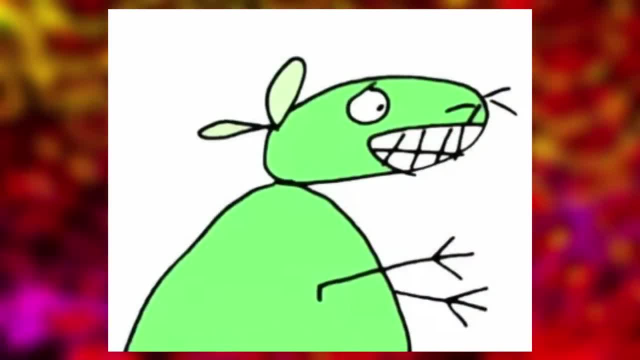 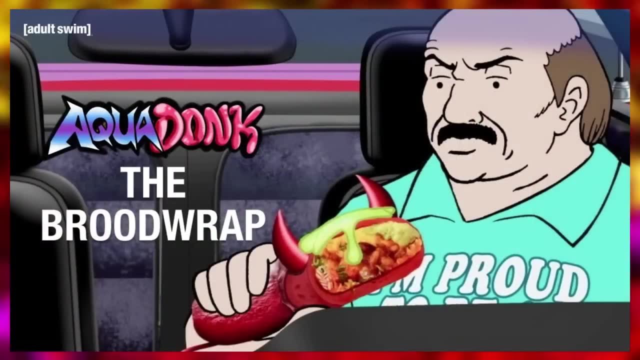 by a missile Is seen watching 12 ounce mouse, which is another Adult Swim original created by Matt Malero, And I guess it's worth mentioning that in the Aqua Donk episode, The Brood Rap Carl is seen listening to the song F Off, which is a song featured in 12 ounce mouse. 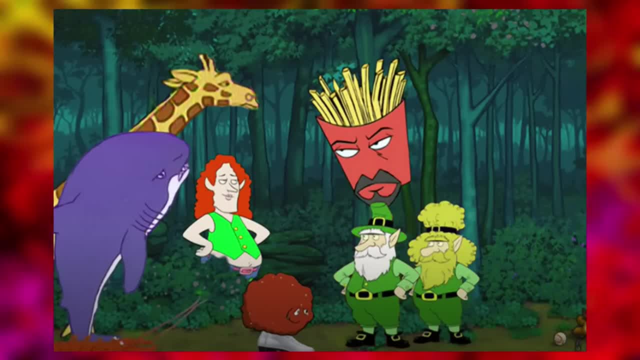 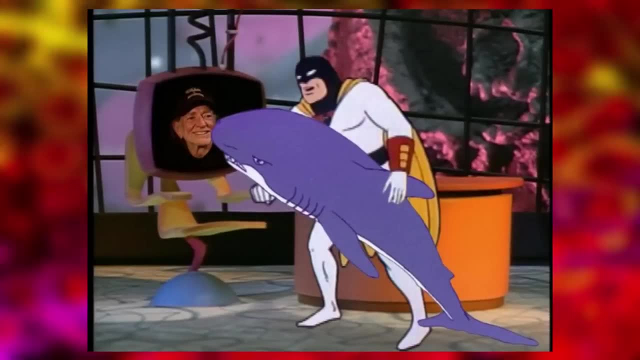 And also Shark makes an appearance in the episode Escape from Lepercopolis, which is a character in 12 ounce mouse, which is also another reused Hanna-Barbera asset. Have you ever heard of old Kentucky Shark? But before we start making assumptions, Matt Malero already put the Aqua Teen 12 ounce. 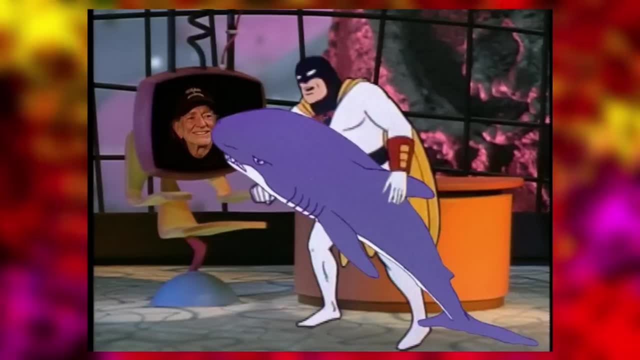 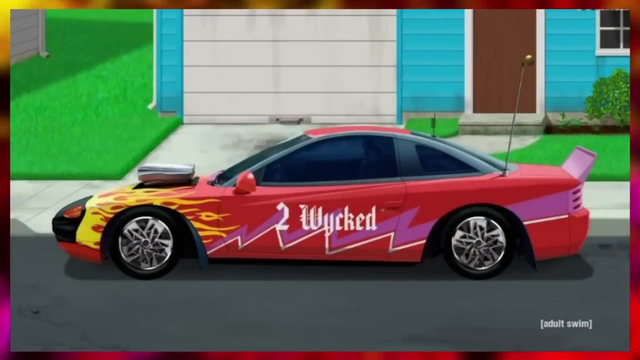 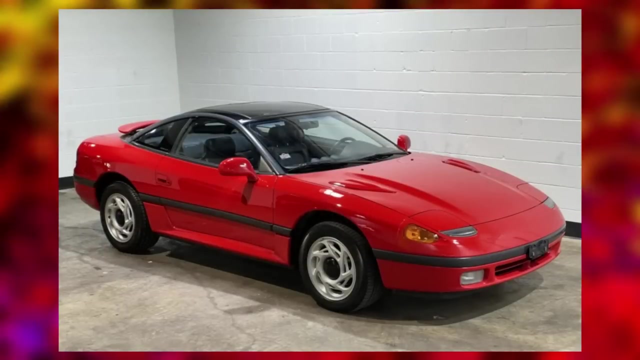 mouse universe theory to rest in his interview with Ronnie from Dancing is Forbidden- 2 Wicked Lore. Carl's beautiful car- 2 Wicked- believe it or not- was Matt Malero's real life car, which was a Dodge Stealth ES According to his Dancing is Forbidden interview. he took a photo of the car for the pilot episode. 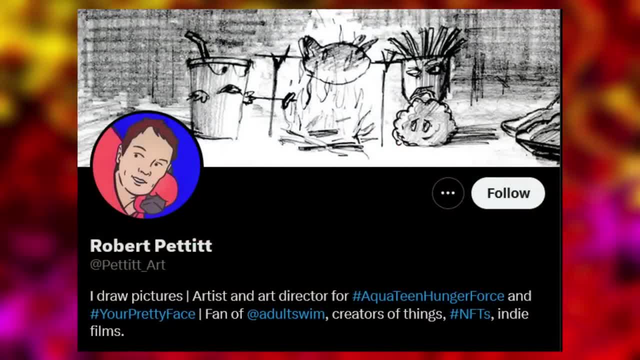 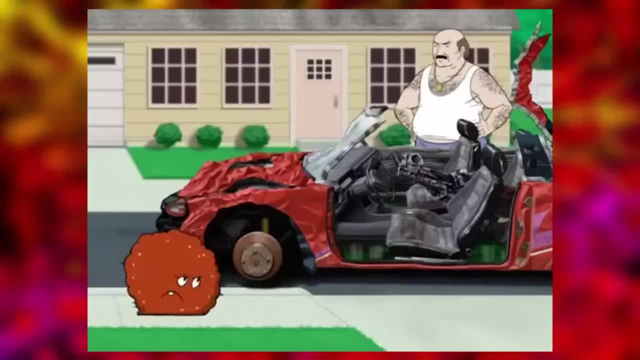 of Aqua Teen, and Bob Pettit, one of the artists for the series, drew the decals on it. He also revealed that the name 2 Wicked comes from a lynch mob song and that the episode Kidney Car was based on him donating his car to the Kidney Foundation. 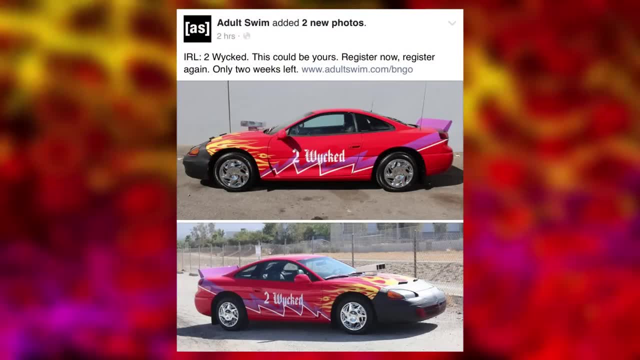 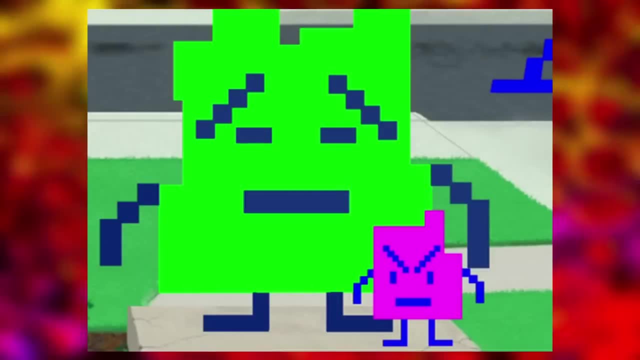 What a good guy. Oh, and Adult Swim gave away a replica of 2 Wicked back in 2015.. Ghosts of ET for the Atari 2600. The Moonanites were first conceived as the ghosts of the failed ET game for the Atari 2600. 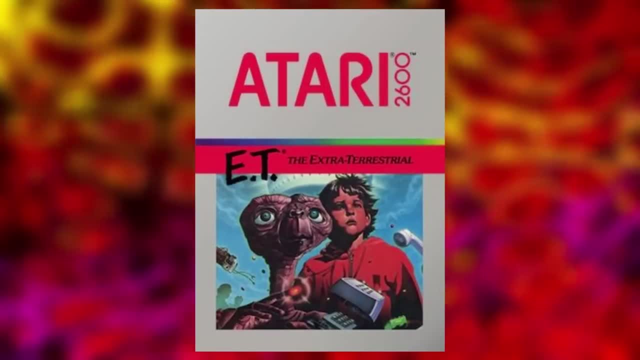 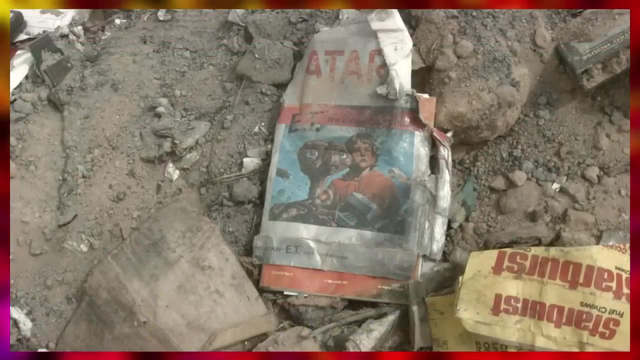 For context, Atari created a game based on the popular ET film. However, it was a financial disaster. All of the customer return copies were then buried, And buried in a desert in New Mexico, because what else is a gaming company supposed to? 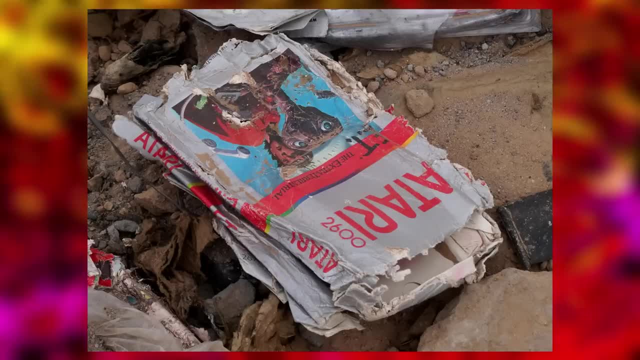 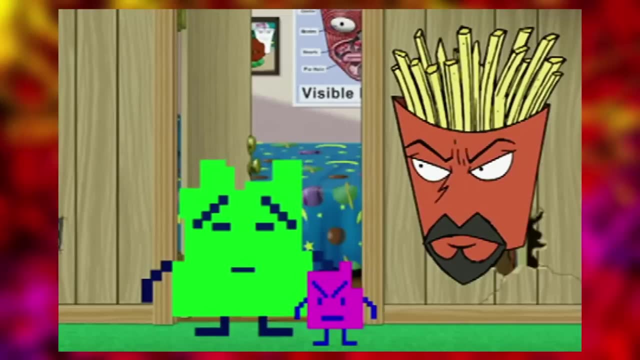 do when their product turns into a consumer's nightmare. Maybe Halo Infinite should be buried as well. Just a heads up, though: the creators didn't end up keeping the idea for the Moonanites being ghosts of the failed ET game. While we're on the topic of video games, I guess it's worth mentioning that the TV 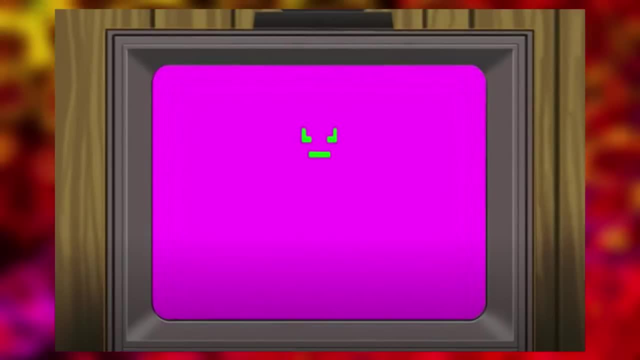 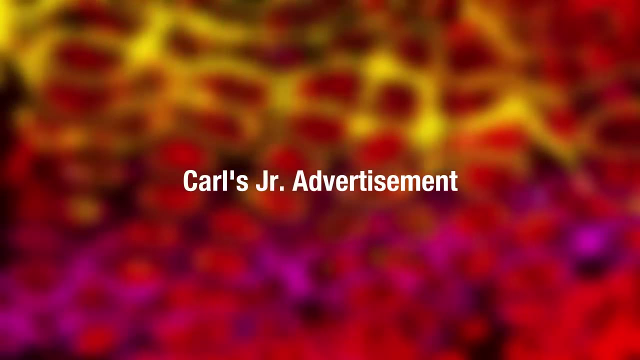 screen in the episode of Video Ouija flashes green and pink, which of course are Ignignak and Ur's colors. Carl's Jr Advertisement. You can't even make this up. Carl from Aqua Teen was featured in a Carl's Jr and Hardee's commercial, and it's exactly. 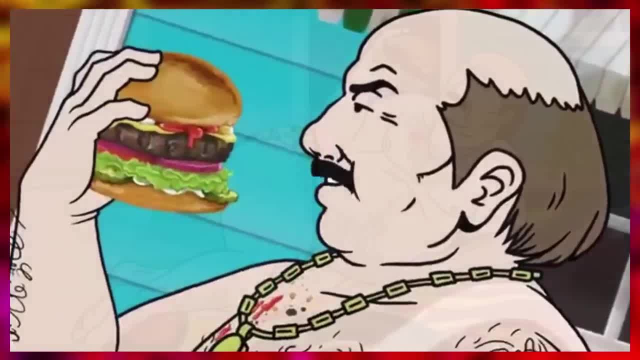 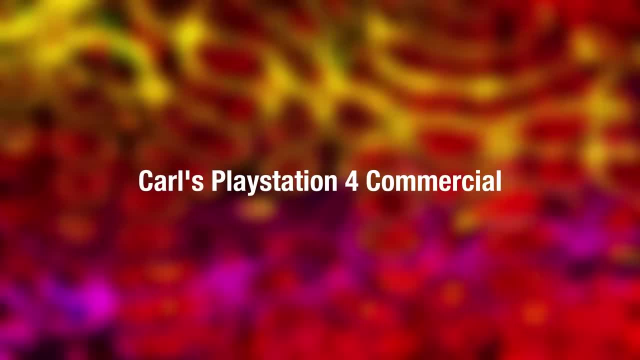 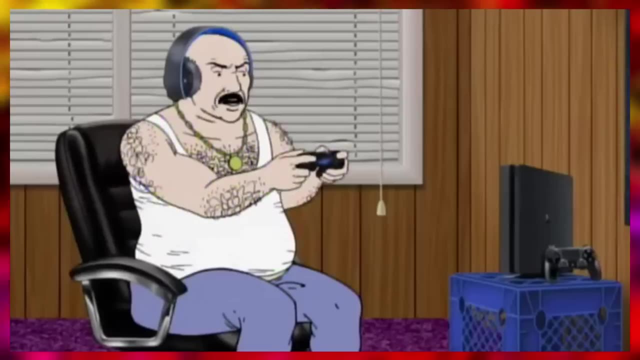 like what you would imagine: Half naked Carl cleaning off his car, getting all soapy with sauce and enjoying a nice tasty juicy burger. Hell yes, Carl's PlayStation 4 Commercial. Besides topless car wash burger commercials, Carl has also dabbled in the world of PlayStation. 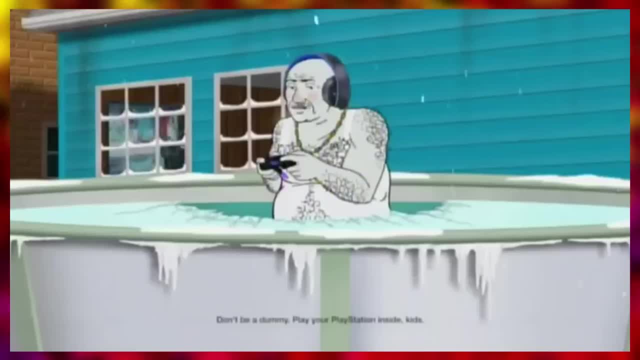 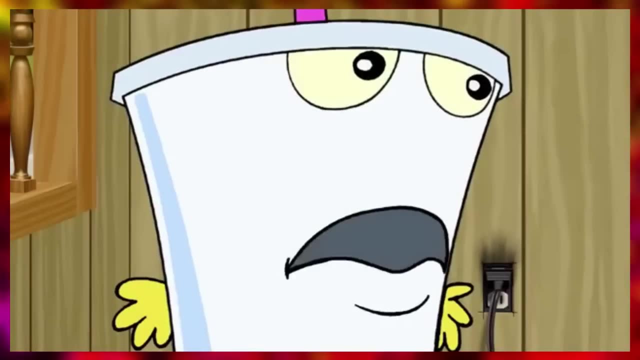 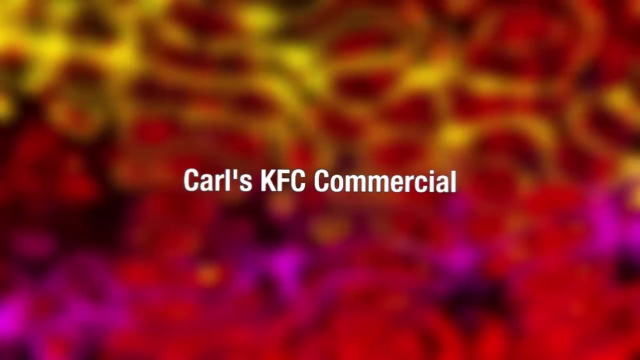 marketing. In January of 2017, Sony released a PS4 advertisement featuring Carl getting his hands dirty with some Call of Duty Infinite Warfare. Since we're talking about PlayStation, Carl, Meatwad, Shake and Frylock also appear in a PlayStation View commercial. 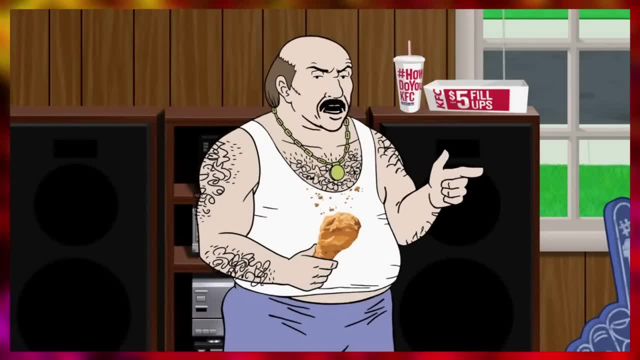 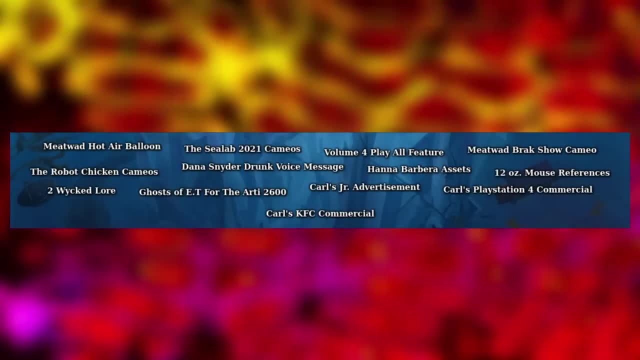 Carl's KFC Commercial Man. I'm starting to think that Carl is desperate for airtime. Once again, Carl is back on your TV screens, this time promoting KFC chicken. And that, my friends, was the fourth layer of the iceberg. 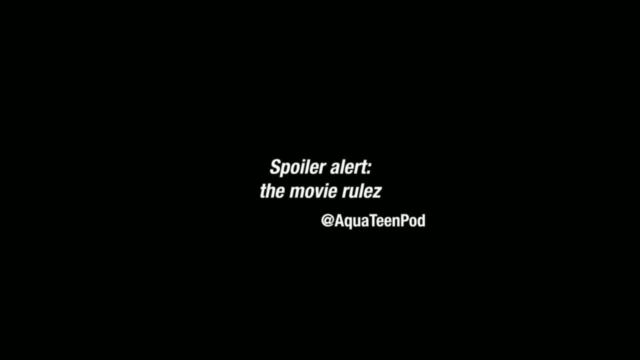 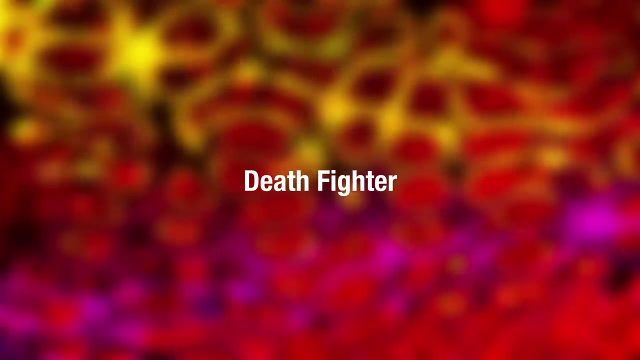 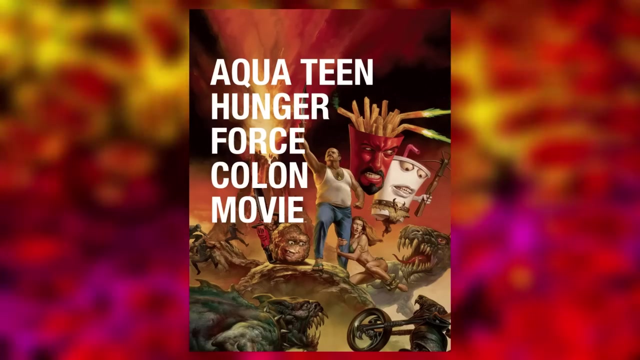 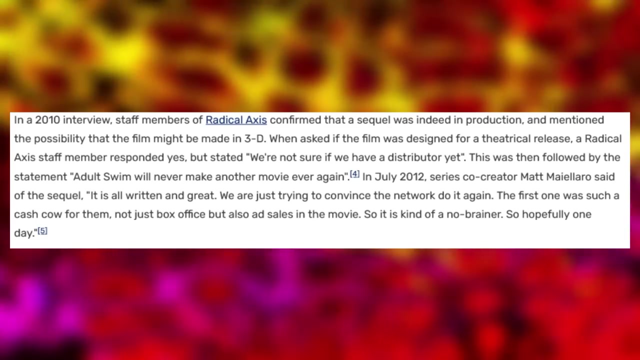 Death Fighter. So Death Fighter is a rumored sequel to Cullen movie film. For over a decade now. the proposed sequel had been mentioned a number of times in interviews and statements from Dave Willis, Matt Malero And even staff members from Radical Access. 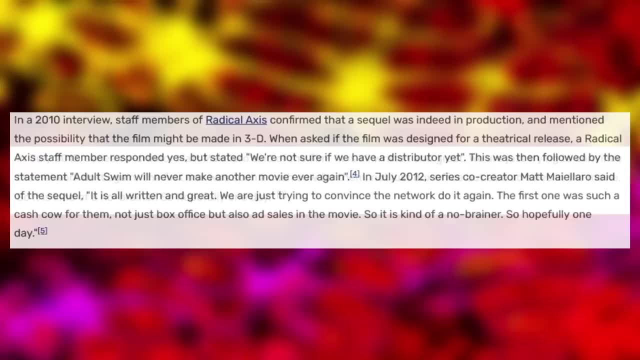 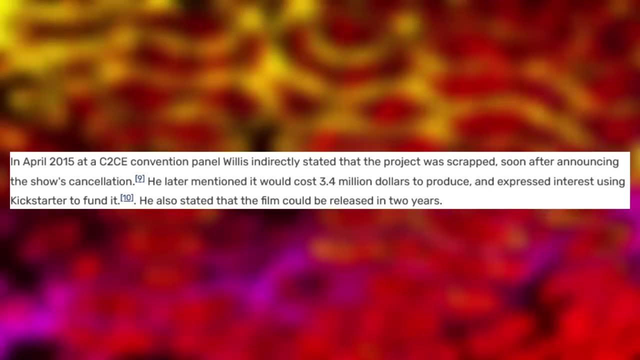 These statements regarding the film included script updates, potential release windows, the possibility of the film being in 3D, convincing the network to make another film, and Dave Willis even stating in a 2015 Reddit AMA that he would love to kickstart the project. and. 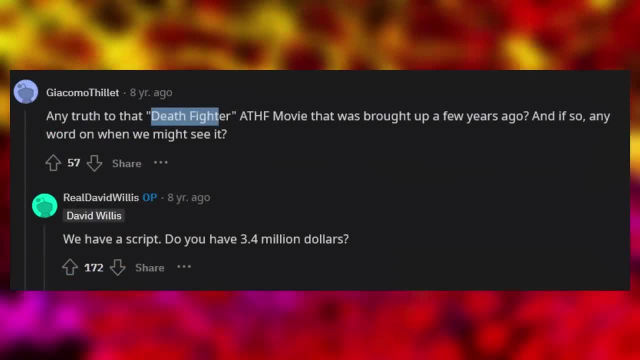 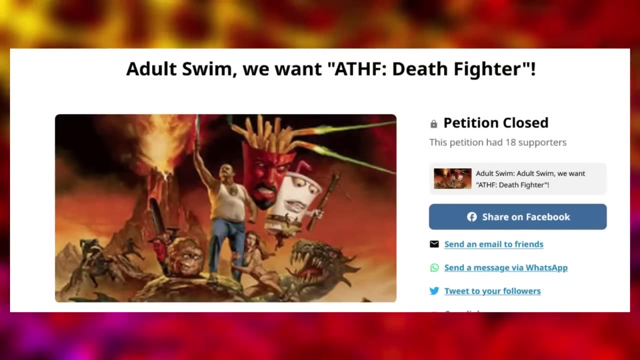 would just need a small loan of 3.4 million dollars. But ever since that 2015 AMA, we've heard zero updates regarding the project. There was a fan petition. It was initiated soon after the passing of C Martin Crocker, begging the network to either. 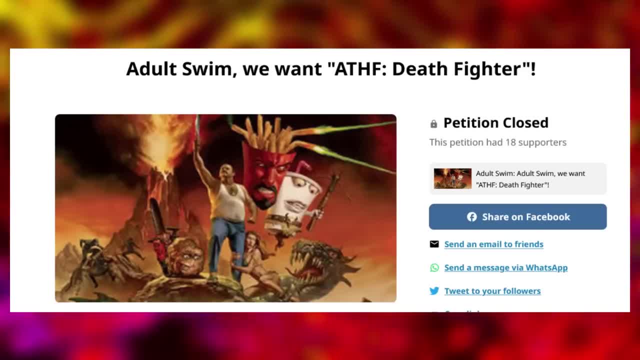 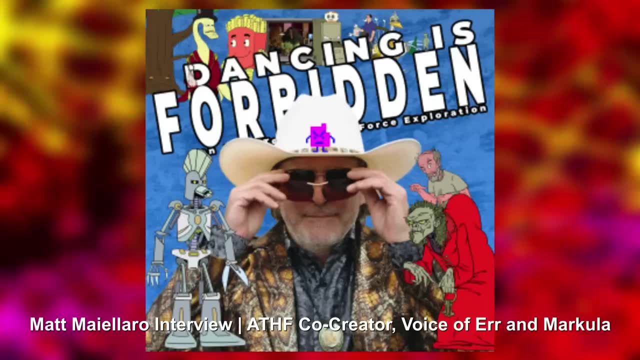 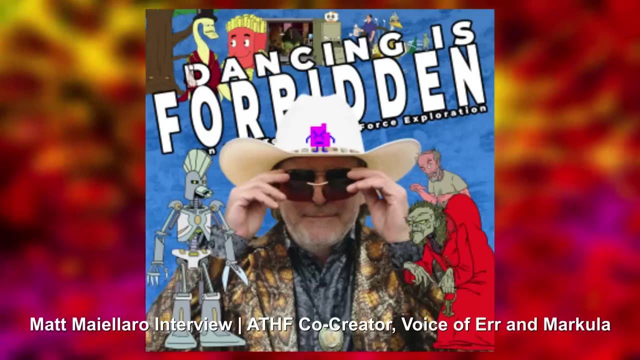 greenlight Death Fighter or just another Aqua Teen season, But the petition sadly passed away with only 18 supporters. However, on Matt's Dancing is Forbidden podcast episode. he was asked if he and Dave considered making the rumored Death Fighter movie when approached to make the new Aqua. 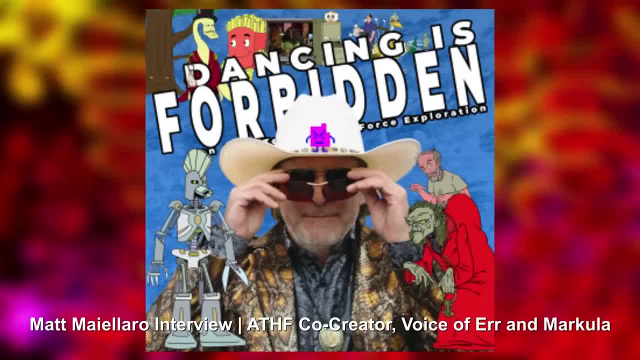 Teen movie, which we now know. as Plantasm And Malero said. We thought about it, But it's so good that we thought let's wait for a third one. That's what I'm saying. That's what I'm saying. 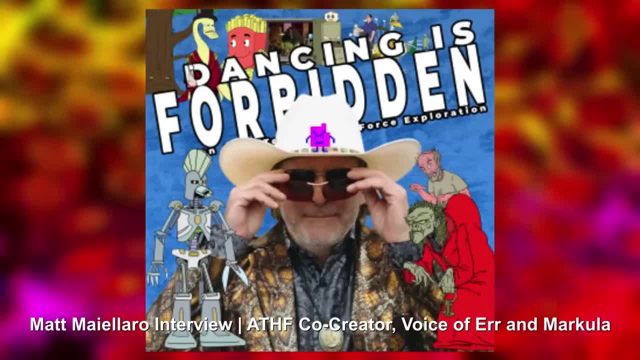 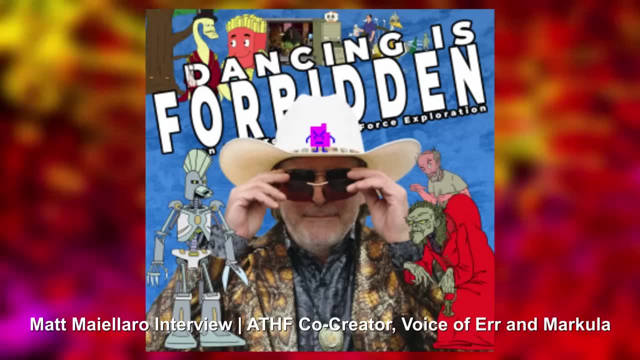 That's what I'm saying. Let's wait until we have more money to make it, because it requires a lot more intense animation and more big A-lister actors. While we're on the topic of Death Fighter, Aqua Teen artist Robert Pettit, who you should 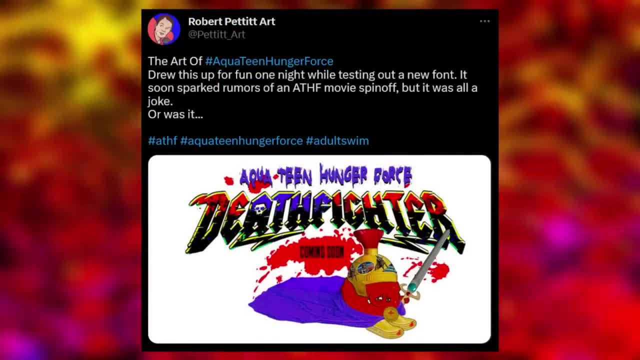 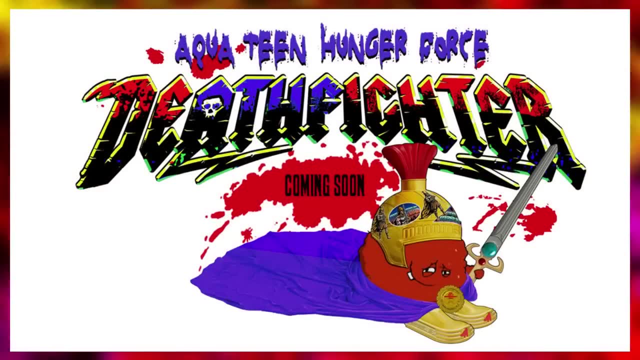 follow on Twitter recently posted this picture he created while testing out a brand new font And, according to him, because of this image, the Death Fighter rumors began to spark. But was it a joke? I don't know, son, I just don't know. 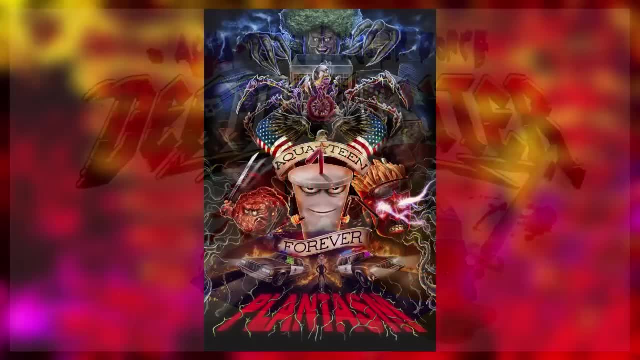 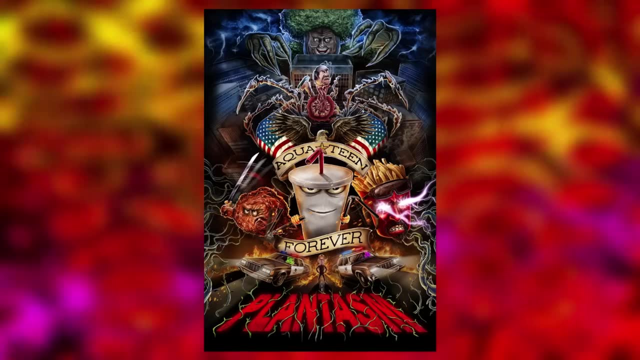 Go ask your mother. Although I am very happy with both Colton and Dave's decision to make the movie, I'm happy with both Colin and Plantasm and just very grateful in general that Aqua Teen now has two movies under its belt. I would do a lot of awful things just to see Matt and Dave bring Death Fighter to life. 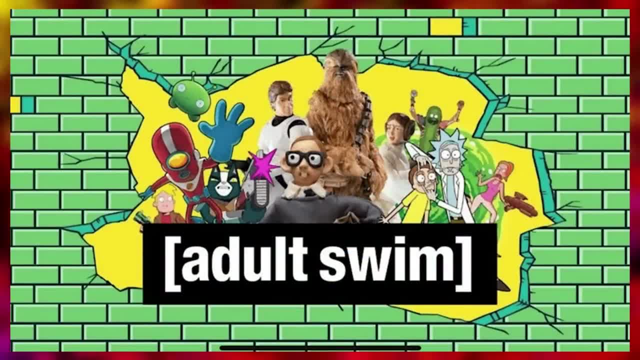 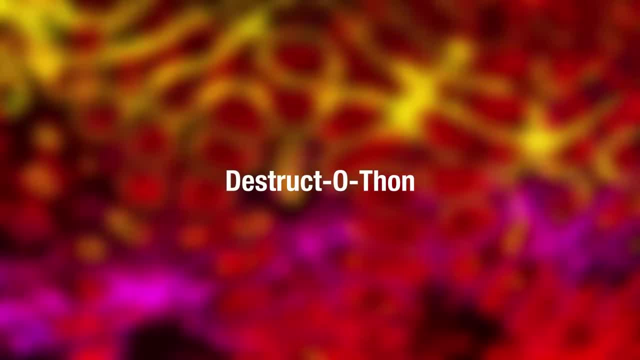 You know if it's real. So hey, Adult Swim. if the next season of Aqua Teen does very well, can you please give Dave and Matt more money? Destruct-A-Thon- Aqua Teen, Hunger Force. Destruct-A-Thon is a single player. action reflects mobile. 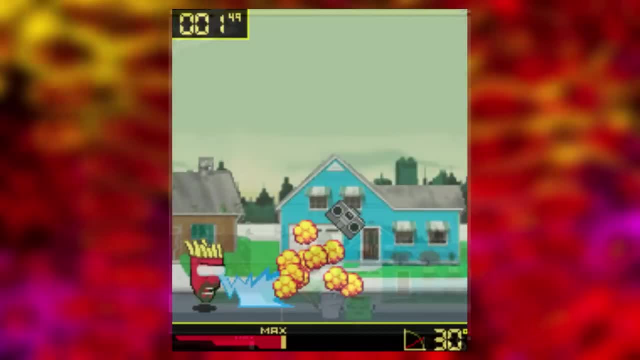 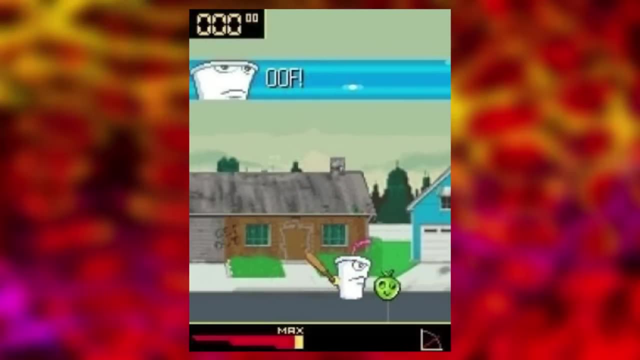 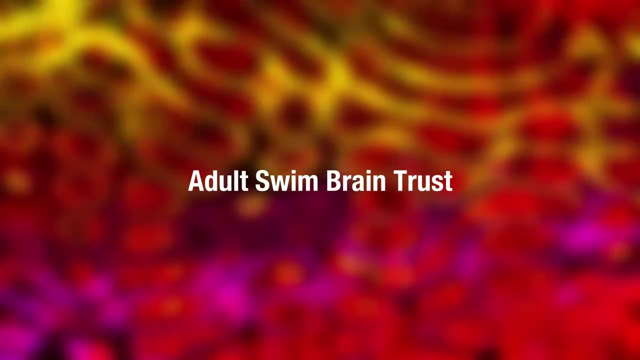 game released in 2004 and created and published by Glu Mobile. The goal of the game is to hit various items as far as possible across the level, to complete a number of challenges and unlocks while playing as either Shake, Meatwad or Frylock. 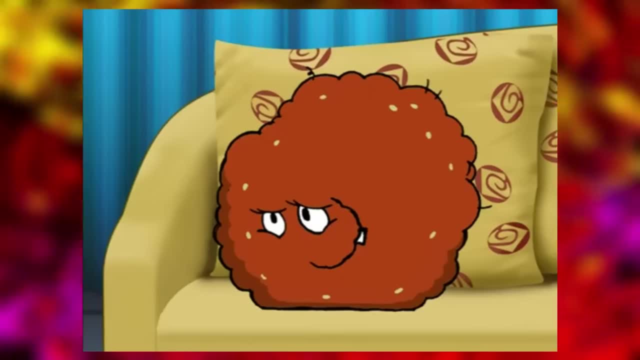 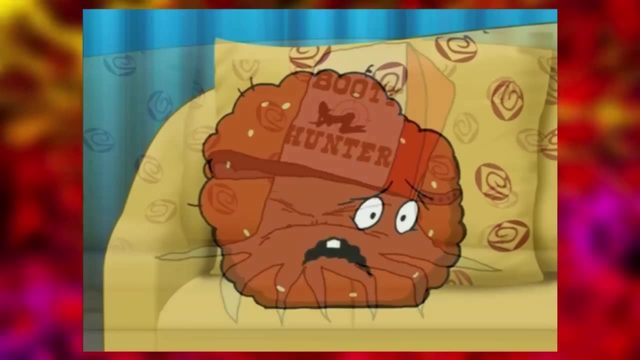 Adult Swim Braintrust. Adult Swim Braintrust, or the Anime Talk Show, was an animated special that aired on Adult Swim in November of 2004.. The special revolved around the unofficial pilot For Squidbillies. the special featured Space Ghost, who hosted a focus group discussion. 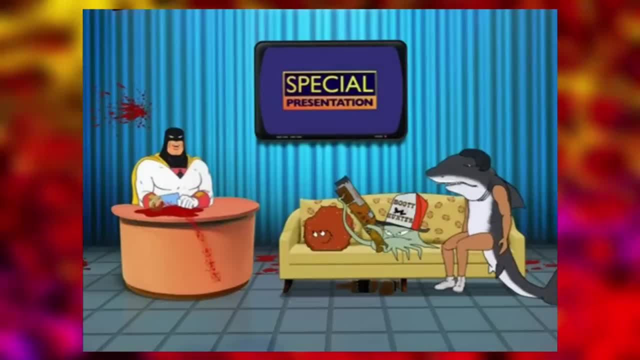 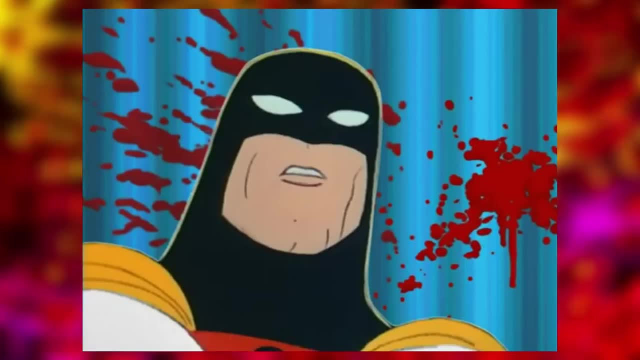 about the unofficial Squidbillies pilot with other characters like Early, Sharko, Zorak and Meatwad, along with the cybernetic Ghost of Christmas Past from the future who makes a cameo as a caller. And just a fun fact: the name Anime Talk Show comes from the fact that the special aired 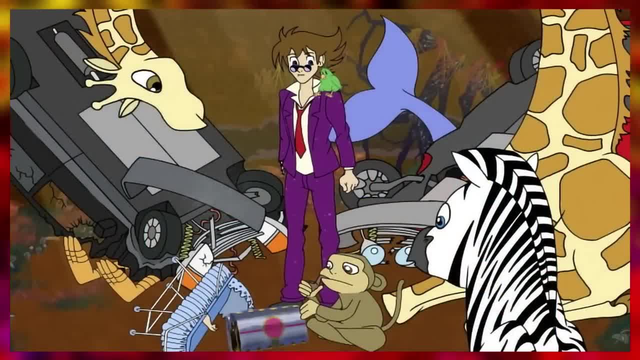 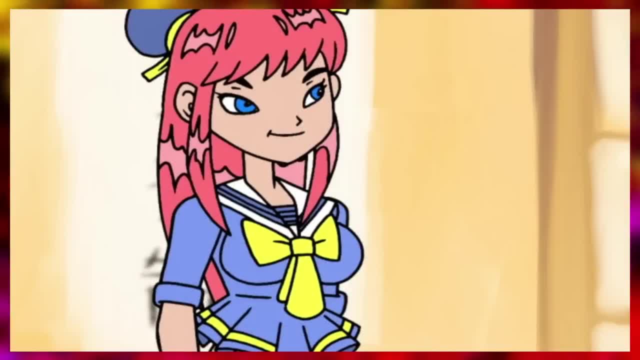 after the premiere of Perfect Hair Forever, which was another show created by Matt Malero along with Mike Lazo and Matt Harrigan, Which aired in place of what was supposed to have been the premiere of Squidbillies. And just another random fact, a lot of voice actors from Aqua Teen are featured in Perfect. 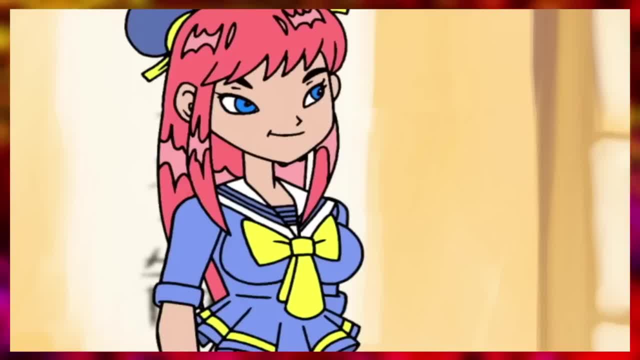 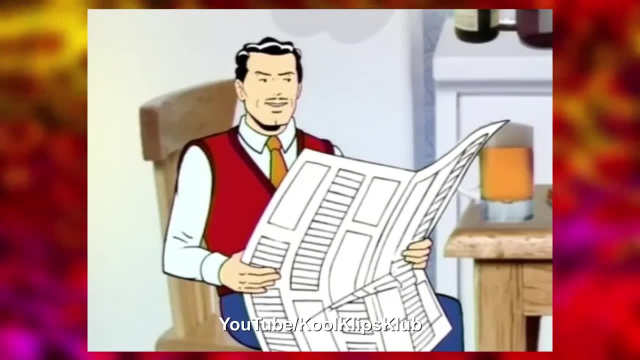 Hair Forever, like Dave Willis, George Lowe C, Martin Crocker and more Bashington's New Year's Eve. On New Year's Eve of 2003,, Adult Swim featured a load of bumpers about the Brack family hosting a New Year's Eve party with loads of special 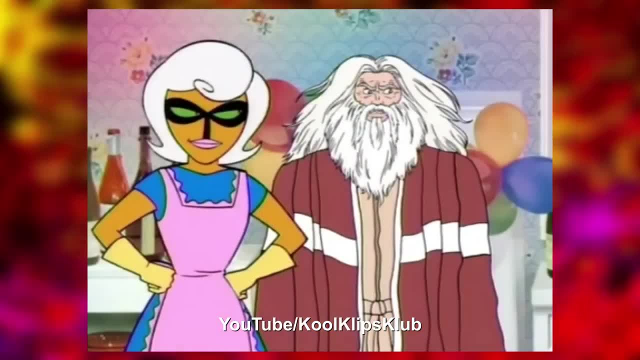 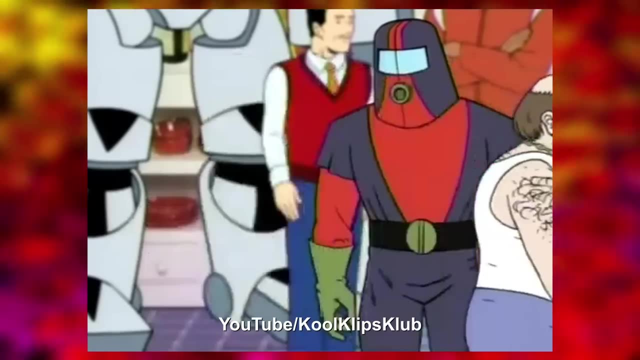 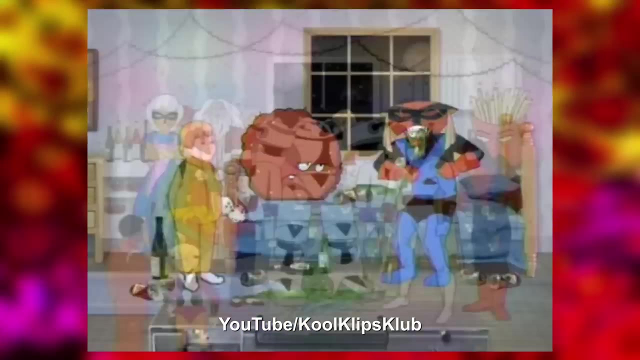 guests like the Aqua Teens Sea Lab 2021 characters, Harvey Birdman characters, Space Ghost, George, Lowe, Zorak and more. Some notable moments from these bumpers include Maltar convincing Carl to go hit on Debbie from Sea Lab, Frylock getting annoyed with Hesh, Meatwad and Brack getting drunk. and. 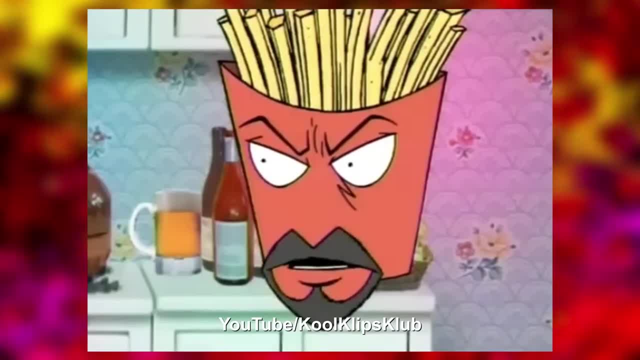 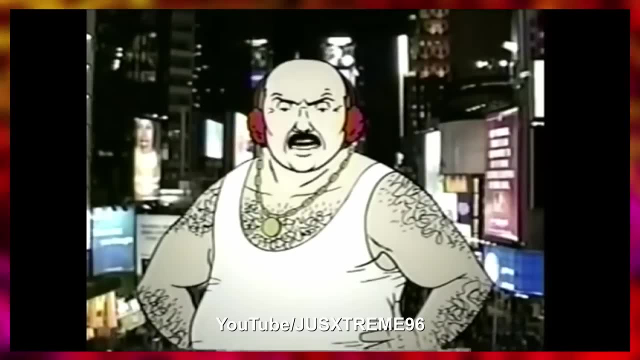 also learning about how Thunderclease was created by Frylock. Speaking of New Year's, the previous year saw Brack and Carl ring in 2023 together in Times Square, which was pretty hilarious to see as well, And on New Year's Eve, 2005,, Adult Swim teamed up with Widespread Panic to perform at the. 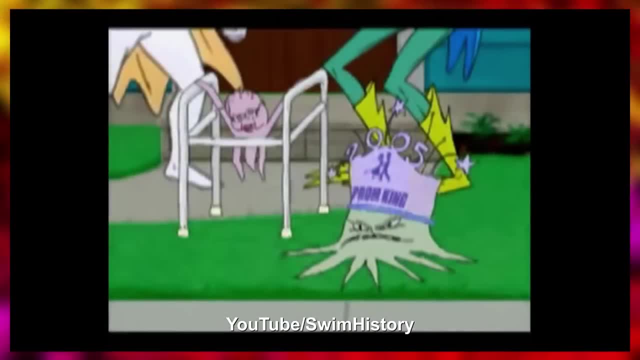 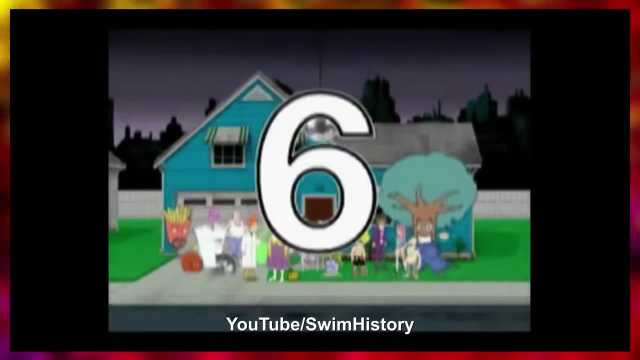 Phillips Arena in New York. In Atlanta, Georgia, the performance featured exclusive clips with Adult Swim characters from Aqua Teen, Hunger Force, Squidbillies, Space Ghost and more. bringing in the New Year. The Bashington and New Year's Eve Bash Bumpers can be found on YouTube via the channel names. 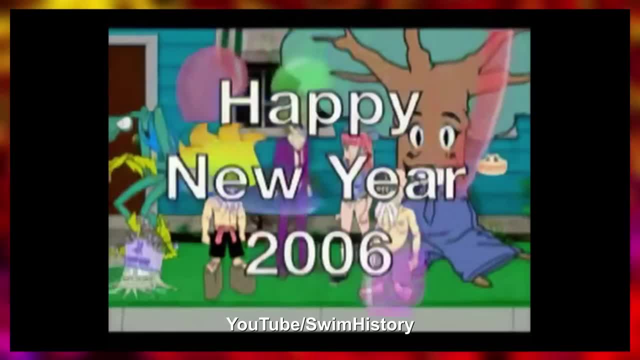 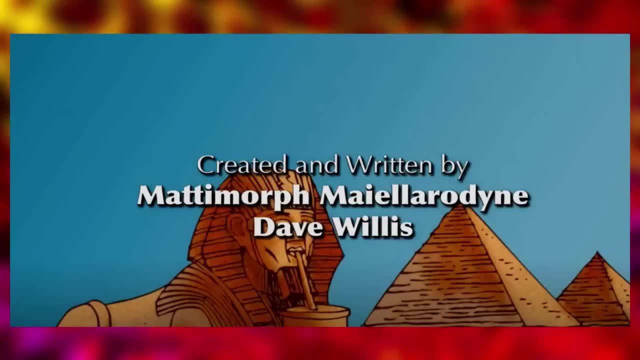 I displayed underneath the footage, as well as the New Year's Eve 2005 clips. Matt Malero Credit Gag. In the ending credits for some of the Season 7 episodes, Matt Malero's name is altered. In Rabot Redux, Matt is credited as Mattomorph Malerodyne. 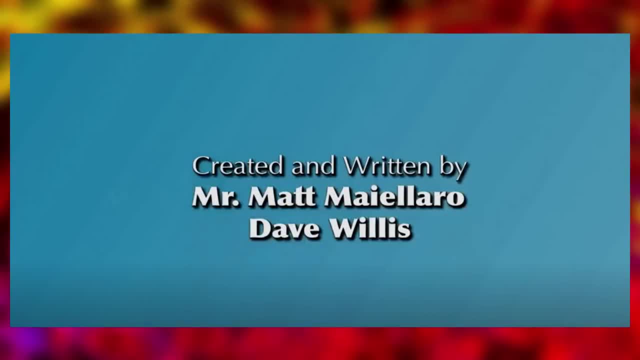 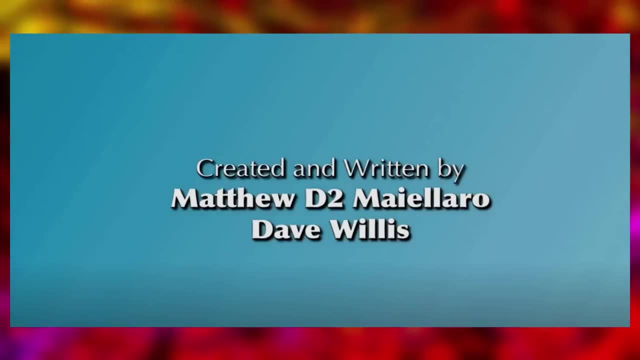 In the episode Eggball, his name is credited as Mr Matt Malero. In the episode Monster, he's credited as Matt Marrin County Malero. In Hands on a Hamburger: he's credited as Matthew D 2 Malero. 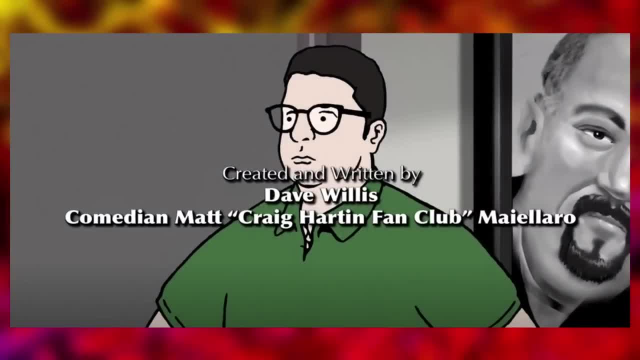 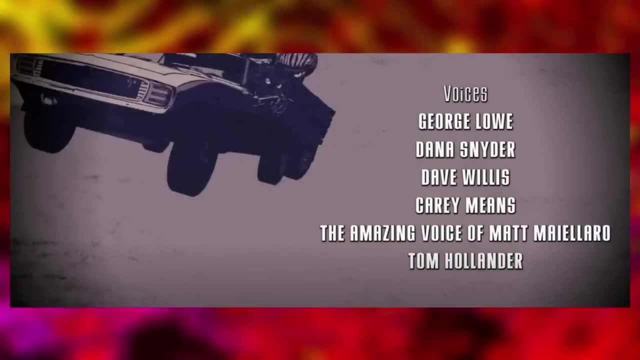 And in the episode 100, he's credited as comedian Matt Craig Harton Fan Club Malero, And in a lot of other episodes he's mostly credited as the amazing voice of Matt Malero. Oh and of course he was also credited as Malero in the ending credits of Brackisode. 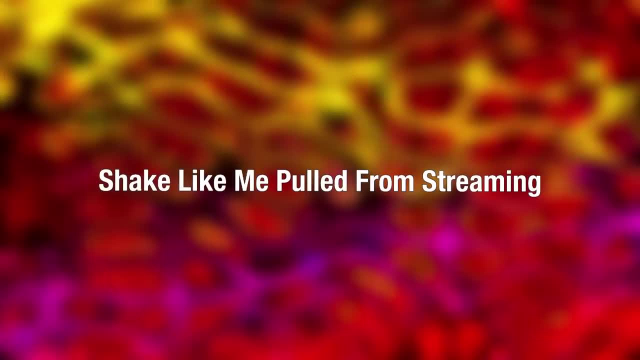 which is a word I can't say on YouTube anymore. Thank you for watching and I'll see you in the next episode. Shake Like Me pulled from streaming Way back towards the beginning of the video. I mentioned that the episode Shake Like Me. 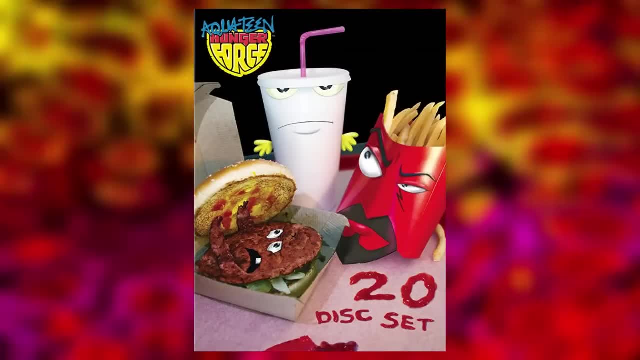 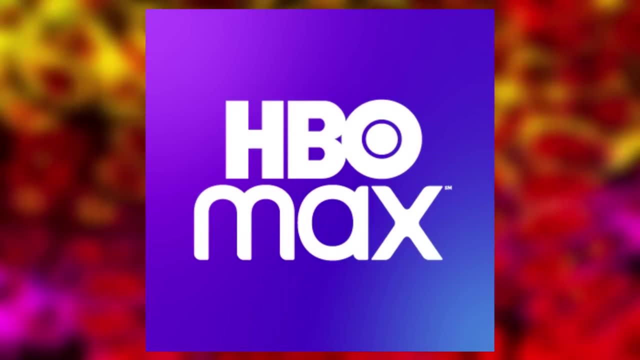 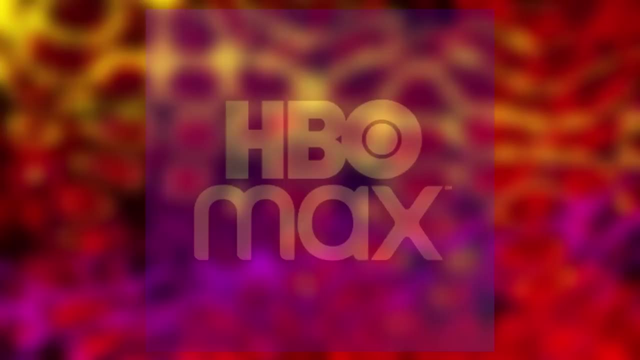 was the only episode officially released to not make the Baffler Meal box set cut. Well, besides not being included on the box set, HBO Max had also pulled the episode from its streaming platform as of June 2020.. However, the episode is still available on the Season 6 DVD and could also be found online. 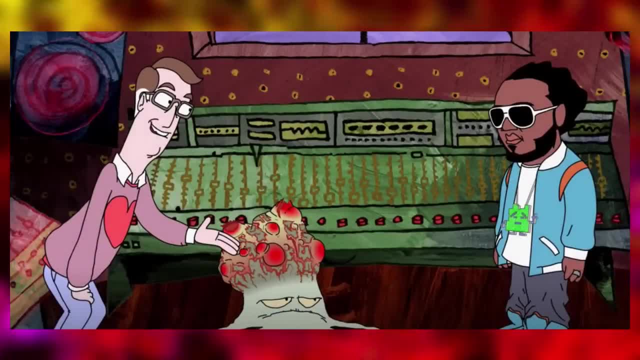 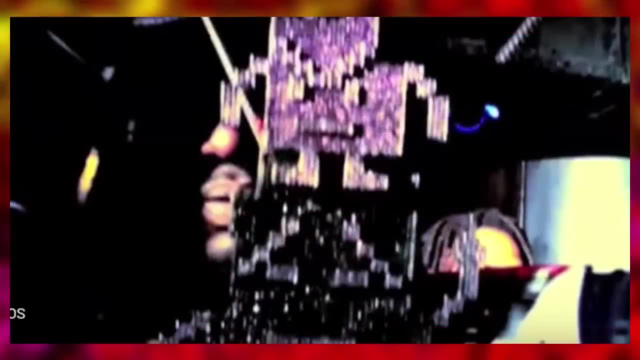 The Squidbillies, Moon and Egg Chains. In the Squidbillies episode, As best as I can, T-Pain is seen rocking some Moonanite ice. What's even crazier is that T-Pain has Ignignok and Err Chains in real life. 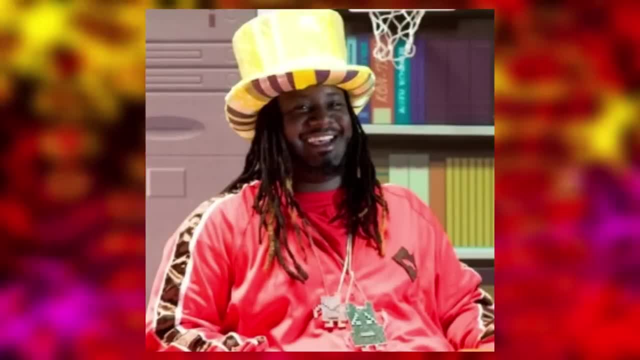 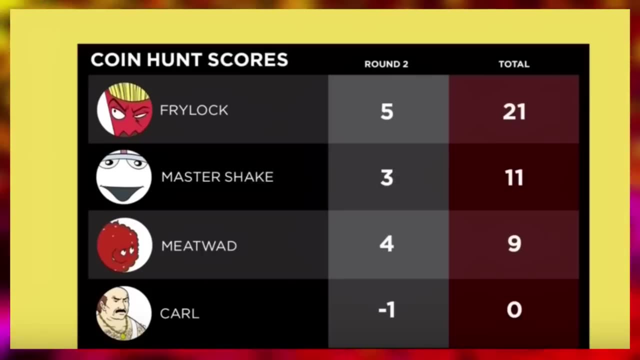 In fact, he is seen wearing those exact chains in the live action Aqua Teen episode, The Last One: Forever Endeavor, Coin Hunt 2015.. On April Fool's 2015,, Adult Swim had the main cast of Aqua Teen partake in a version. 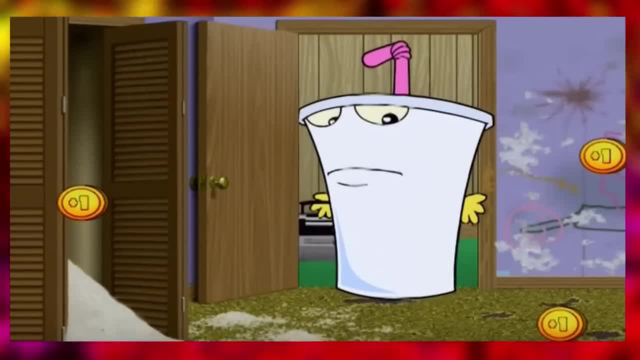 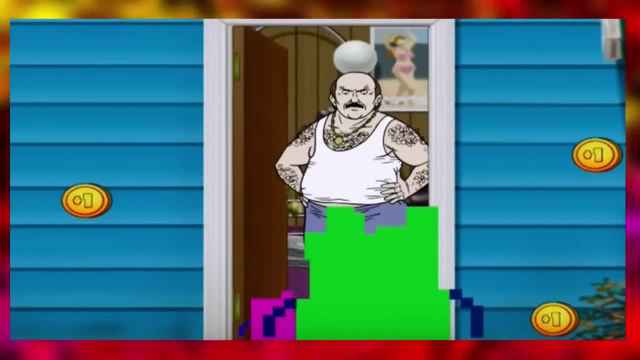 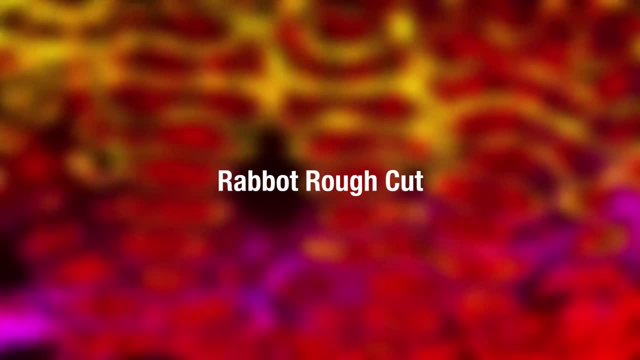 Aqua Teen. They also earned points by moving towards superimposed coins in a marathon of episodes, And by superimposed I mean the coins were on screen and they would not go away. Rabot- Rough Cut. There are three versions of the Aqua Teen pilot's Rabot. 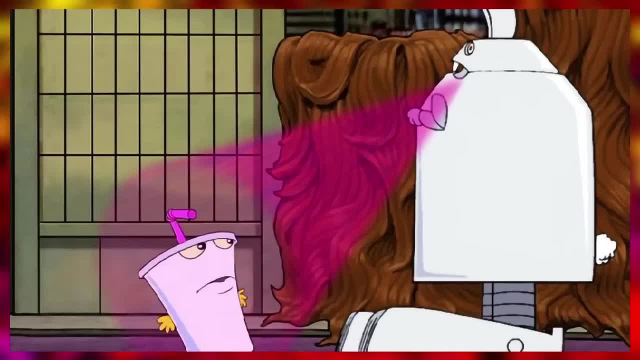 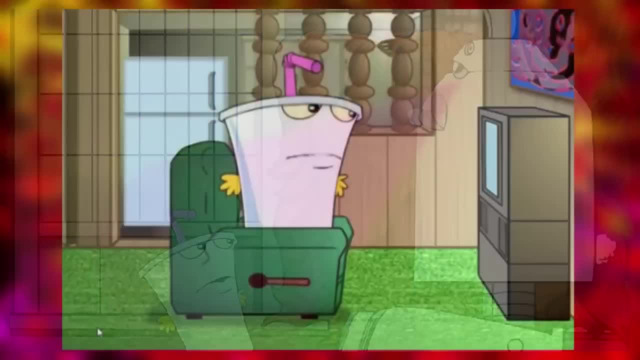 The final version, the stealth pilot that premiered prior to Adult Swim and the Rough Cut, which I want to briefly discuss, because there are a lot of notable differences between the Rough Cut and the official version. I mean, for starters, the inside living room of the Aqua Teen's house is shown in this. 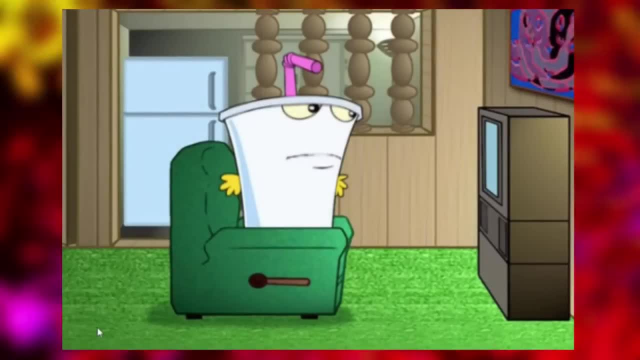 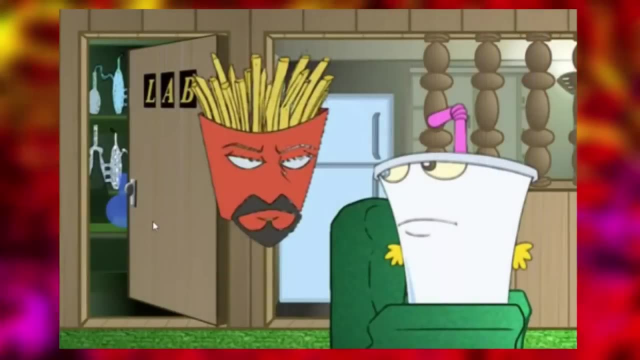 Rough Cut version. Quite a number of scenes take place here, but those scenes in the living room altogether were removed from the stealth and final cuts. The living room in general just looks pretty wild in terms of its animation Like. the layout is pretty identical to the current living room we know now, but the textures 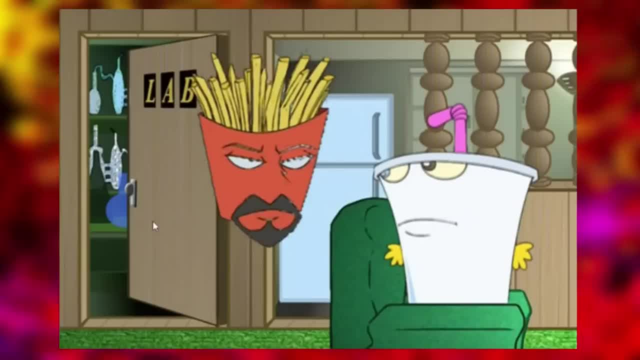 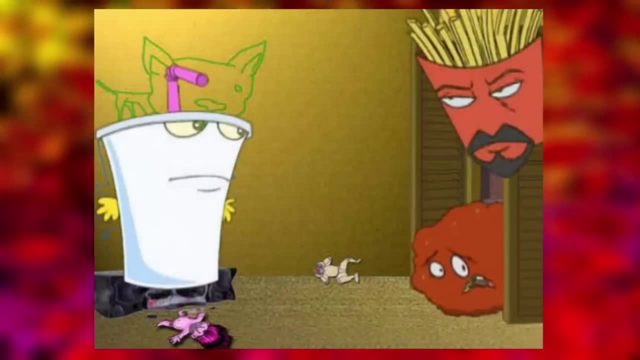 were very wacky. There's even a door that leads to a laboratory. Shake also had a reoccurring catchphrase. Originally, blank is forbidden was going to be his catchphrase, but from my understanding the creators realized how redundant that saying was in the Rough Cut so they just kept the 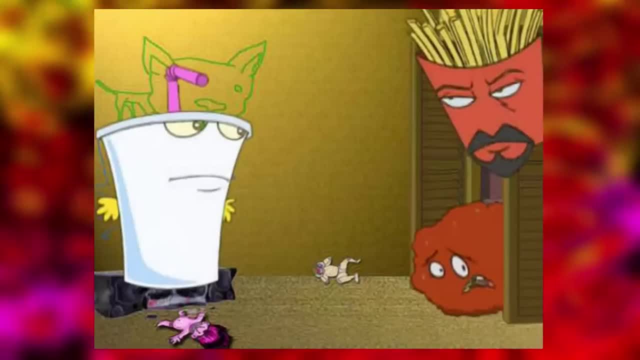 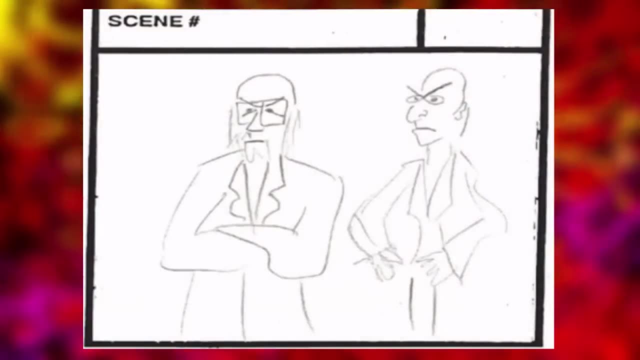 dancing is forbidden. statement in the final cut. I don't know why they did that. They also included that line in the outro credits song and just dropped the catchphrase idea altogether. The cold opening was much longer than the final cut and also wasn't quite finished. 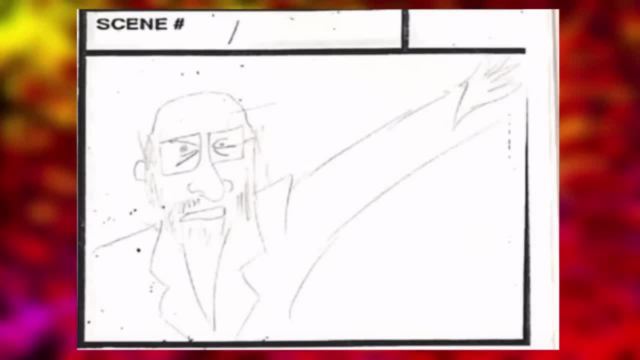 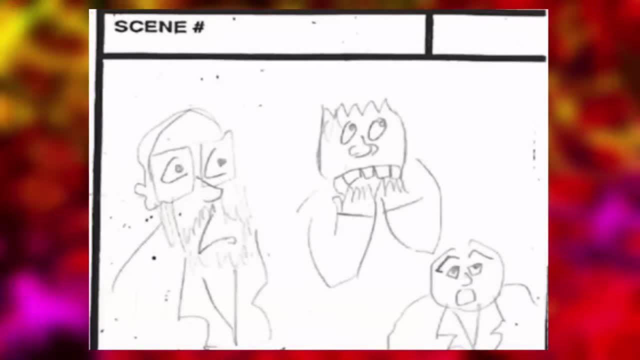 Like the scene mostly showed early storyboard designs of Dr Weird and Steve, because they were not animated yet, There were also some other random scientists in the storyboard sketches as well, Hence why Dr Weird's opening line was GENTLEMEN, because there was more than one person in. 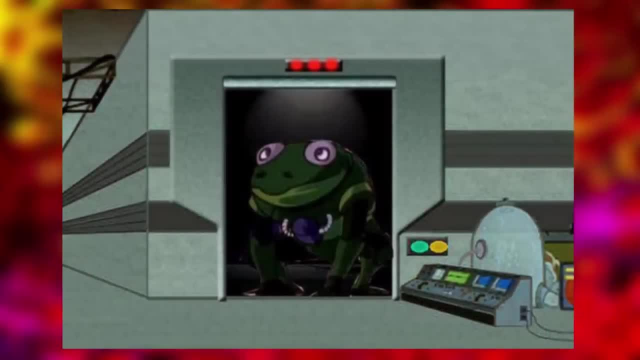 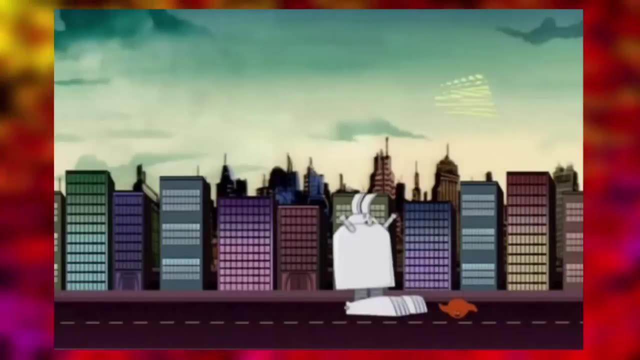 the room. A mechanical frog makes an appearance right after the Rabot escapes, and I believe the mechanical frog is also in this scene. It was also in the stealth pilot but was completely thrown out in the final cut. At one point Frylock tries to attack the Rabot but completely misses. and that's not even. 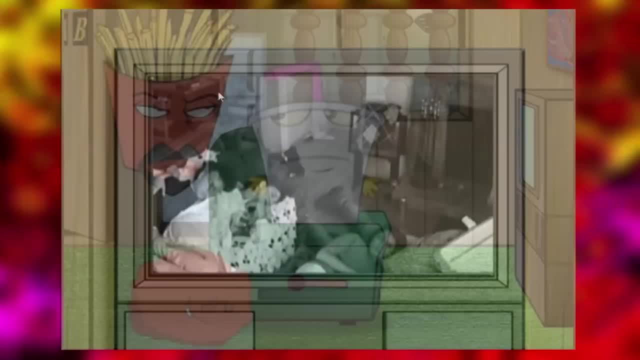 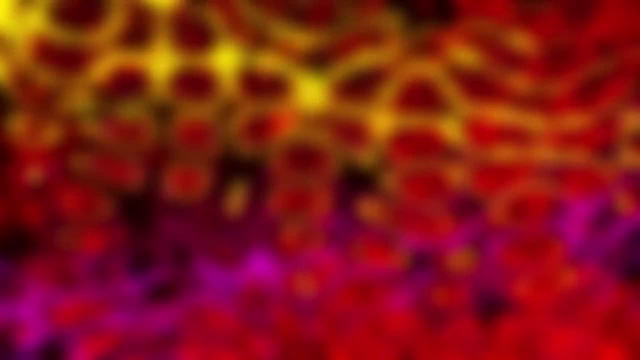 scratching the surface. There are dozens of other differences between the rough and final cuts. so if you want to see the director's cut, then grab a copy of the volume 1 DVD or the Baffler Meal box set, Napkin Lad. 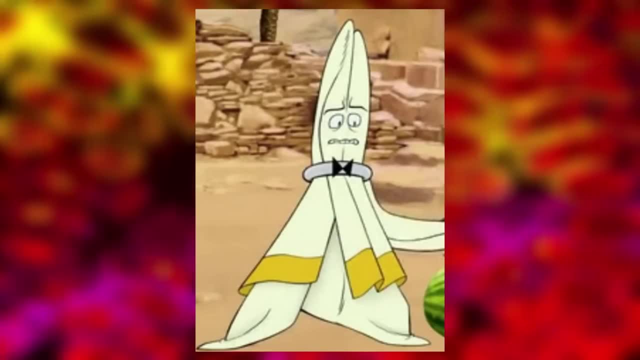 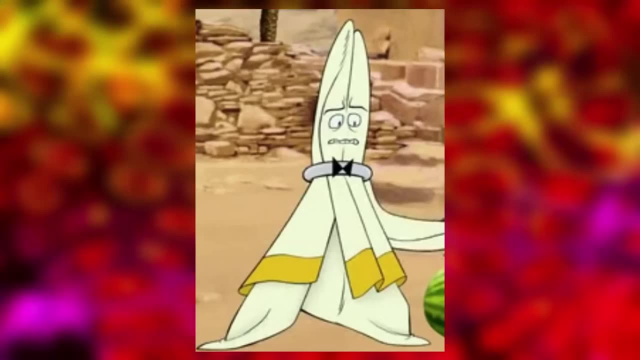 Napkin Lad originated as an idea for the Space Ghost Coast to Coast episode Baffler Meal. He would have been killed off by the end of the episode from having water poured into him. Todd Hansen, a writer for The Onion and the voices of Dan Halen on Squidbillies, the wwwyzzerddcom. 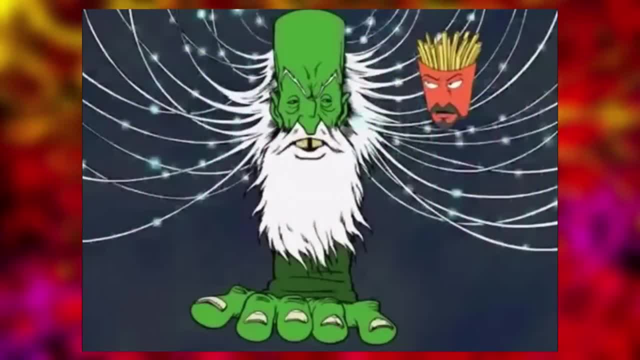 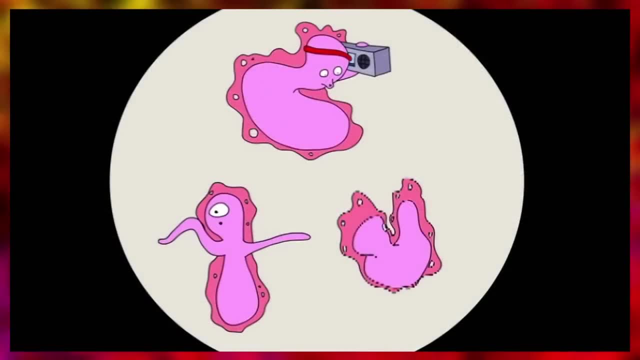 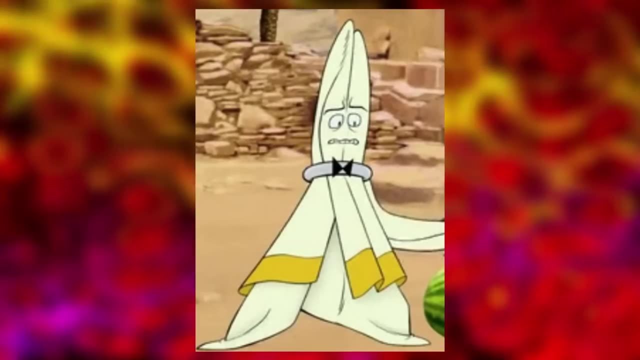 oh wait, my sincerest apologies, it's pronounced w-w-w-w-wizard, and a hypno-germ pitched the character during the development of Baffler Meal. However, the character and concept was ultimately scrapped. Eventually, Napkin Lad did end up seeing the light of day in the Aqua Teen episode Last. 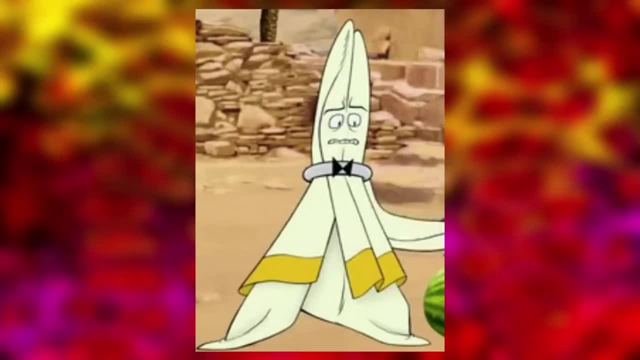 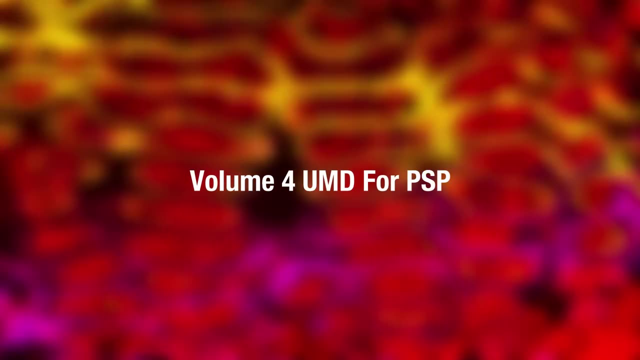 Dance for Napkin Lad, Where the character appears as a spy and was even voiced by his creator, Tom Hansen. Volume 4, UMD for PSP. So a UMD or a Universal Media Disc is a discontinued optical disc medium developed. 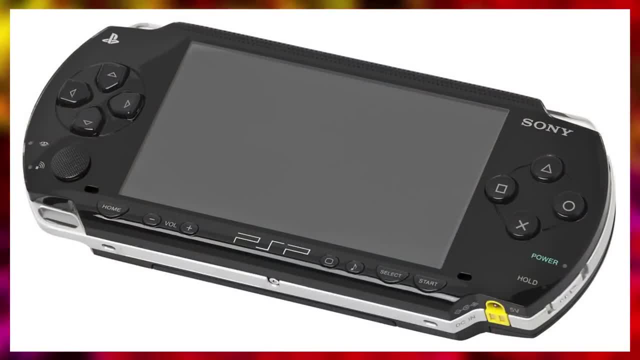 by Sony for the PlayStation Portable, or PSP. The disc was able to hold up to 1.8 gigabytes of data and was capable of storing video games, music and films. Now, what I'm about to talk about, I didn't even know about, because I never owned a PlayStation. 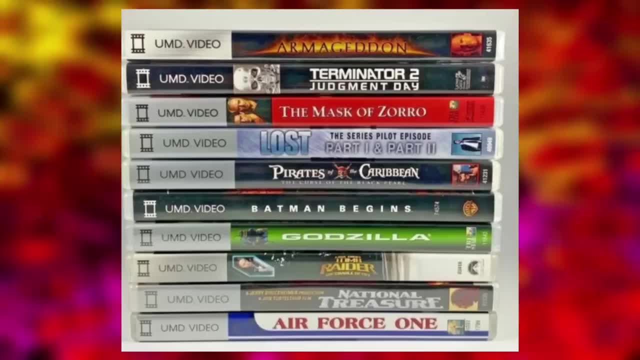 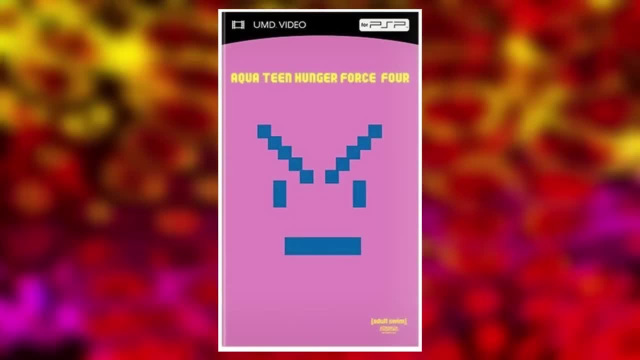 handheld in my entire life, But apparently companies used to put seasons of TV shows and movies on these UMD discs for PSP users, and one of those shows was Aqua Teen, specifically Volume 4.. What's pretty cool about this Volume 4 UMD disc is that the cover art depicts Ur, whereas 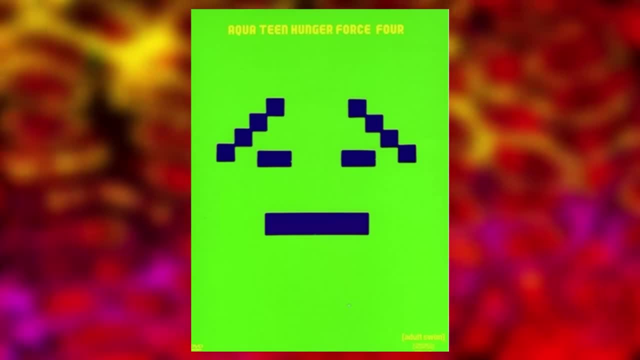 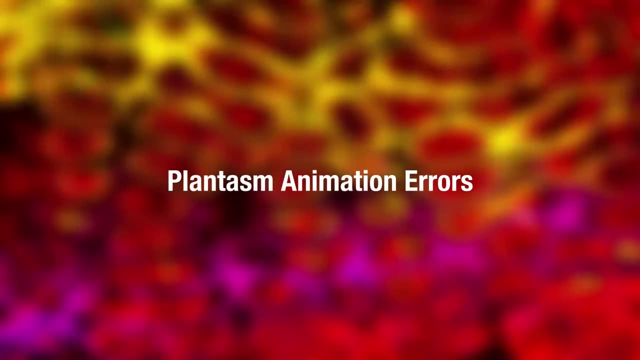 for the regular DVD of Volume 4, the cover depicts a Gnick Gnock. It's kind of strange to me how the previous three Aqua Teen volumes were never released for the PSP, though. Oh well. Plantasm: Animation Errors. Dave Willis, during an early screening of Plantasm, spoke about an animation error inside. 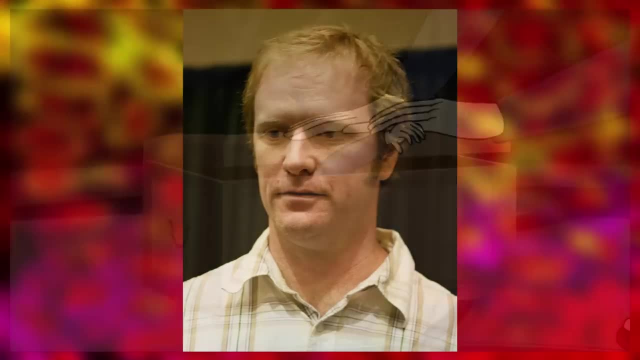 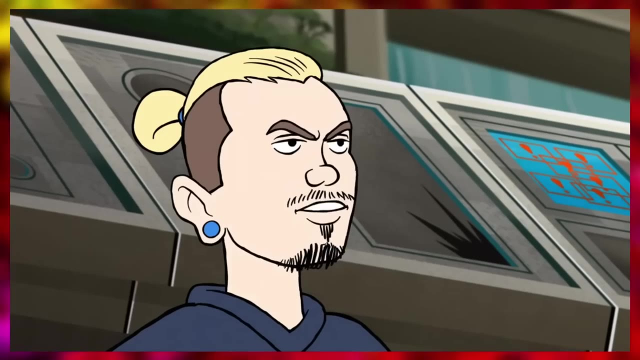 of the film and that the team were too late to fix the problem. That issue in particular is that Neil's mouth doesn't move when he says the line: get me fitted into my tuxedo after being blasted out of the box by Frylock. 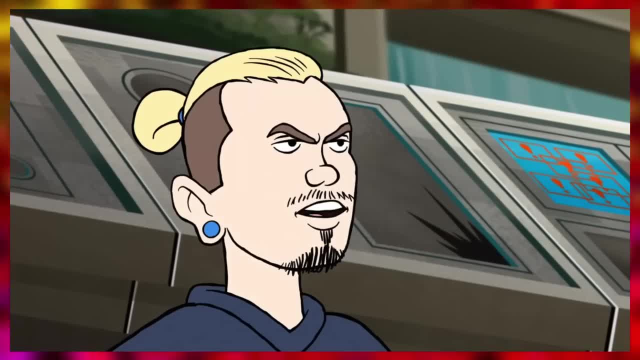 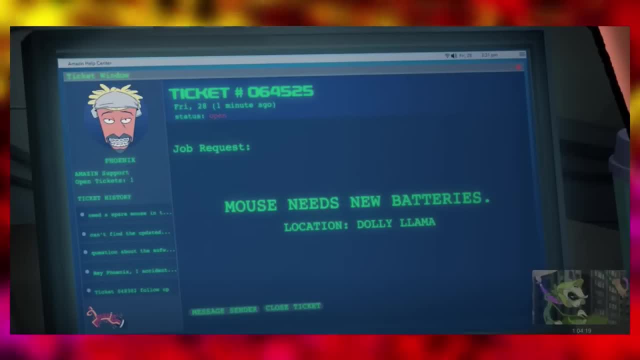 While we're on the topic of errors, I found another part in Plantasm that I think is an error- but maybe it's not- and that's when Frylock receives a ticket on his computer for new batteries and the location says Dalai Lama. 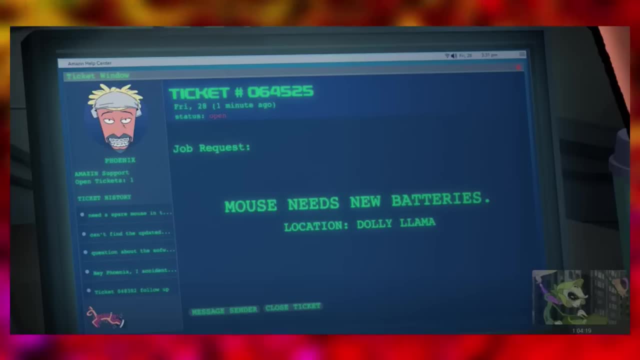 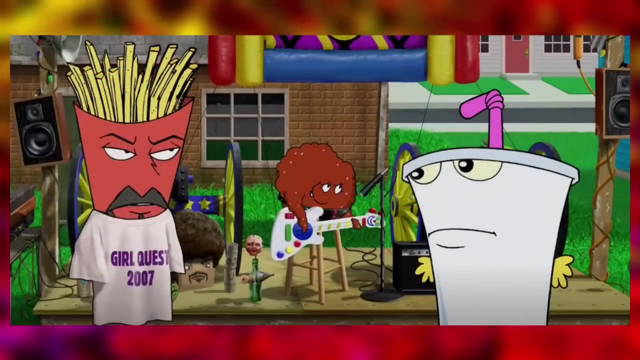 Despite the ship being called the Lama Dali, as to not upset Neil's best friend, which is the Dalai Lama. However, this might not be an error, because something similar like this happened back in colon movie film at Meatwad's concert. 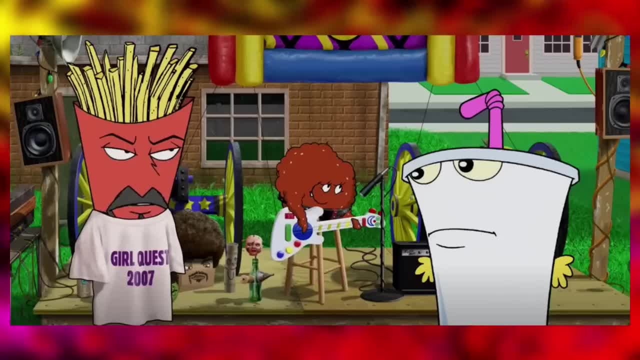 Frylock is seen at the concert wearing a t-shirt that says Girl Quest 2007,, but he refers to it as Girl Quest 2005.. So this might just be a gag, it might not. I really couldn't tell you though. 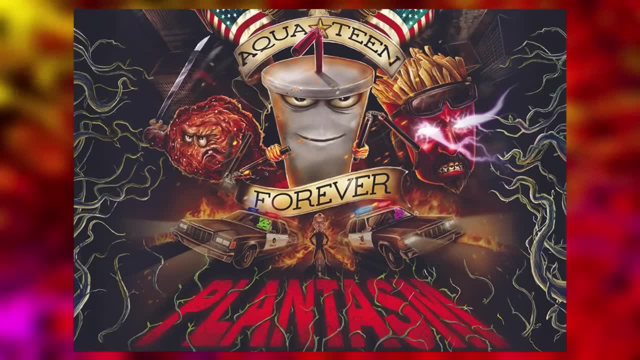 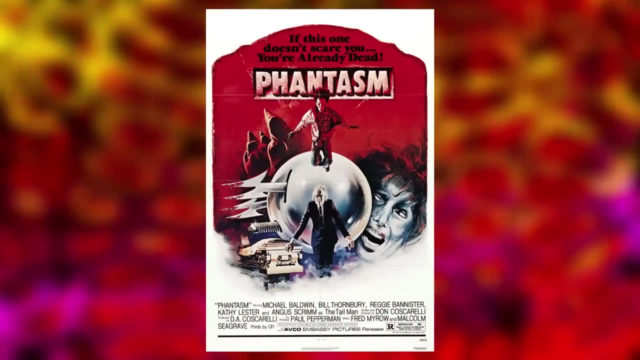 Tantasm, Plantasm. the title of the new Aqua Teen movie is a reference to one of Matt Malera's favorite movies, Phantasm. But did you know that this isn't the first time Phantasm had been referenced in Aqua Teen? 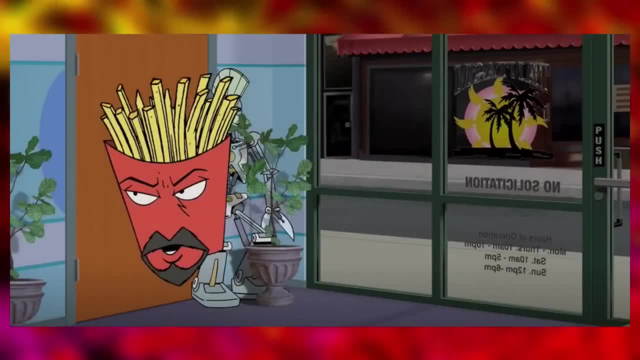 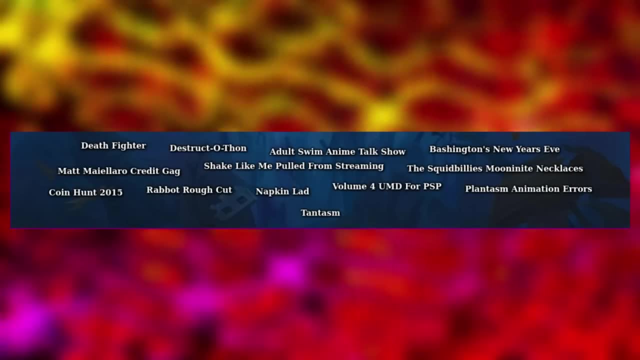 Back in colon movie film, the name of the tanning salon that Shake goes to was called Tantasm and if you take a look at the logo on the door you could see the sentinel sphere built into the Tantasm logo. But anyways, that, my friends, was the fifth layer of the iceberg. 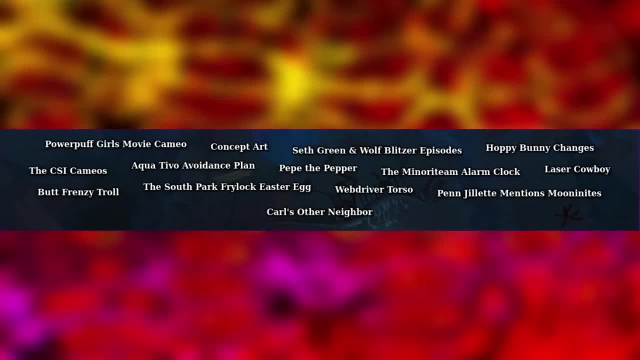 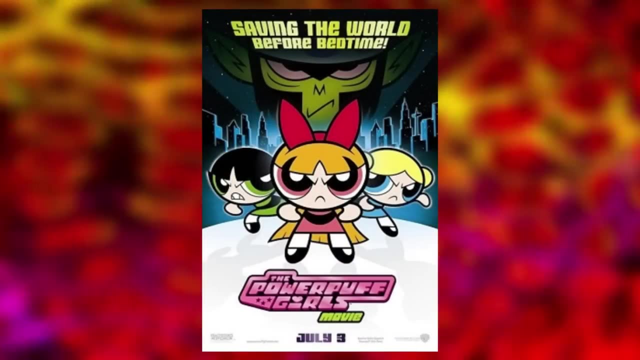 You get your hotdog. Yeah, I ordered a hotdog Through the mail. Powerpuff Girls Movie Cameo. In the 2002 Powerpuff Girls movie, Shake, Frylock and Meatwad are seen on a monitor in the background. 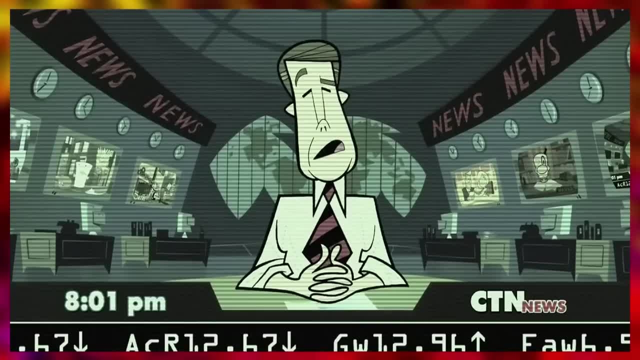 of the newsroom, which means that it's possible that Aqua Teen and the Powerpuff Girls exist in the same universe. This isn't the only Powerpuff Aqua Teen connection, though. Meatwad is seen using a Powerpuff Girls themed parachute in colon movie film. 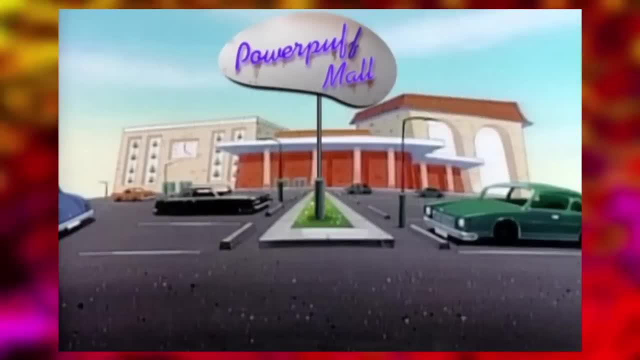 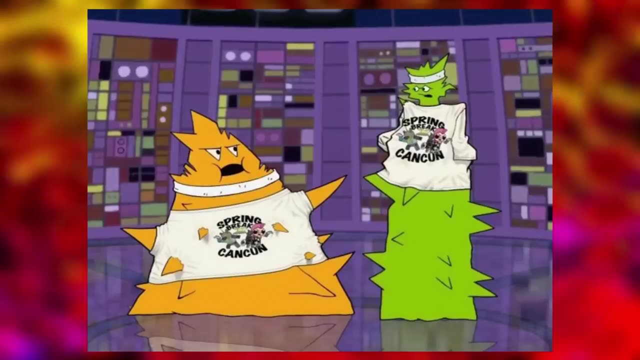 Hell. even the first version of the Powerpuff mall seen in the early seasons of Aqua Teen was used for the pilot episode of the Powerpuff Girls, and it's even called Powerpuff Girls, And the Plutonians are seen wearing t-shirts with a Powerpuff Girl looking design. 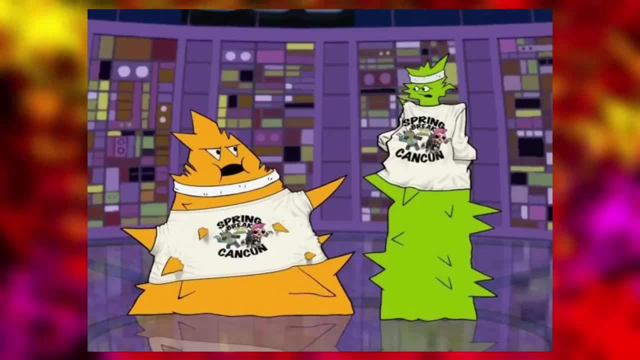 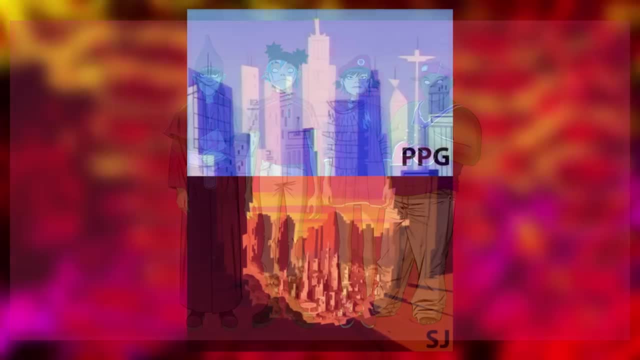 So if Aqua, Teen and Powerpuff Girls do exist in the same universe, that also means that Samurai Jack and the band Gorillaz also exist in the same universe. There is an episode of Samurai Jack where Jack walks through a destroyed city and passes. 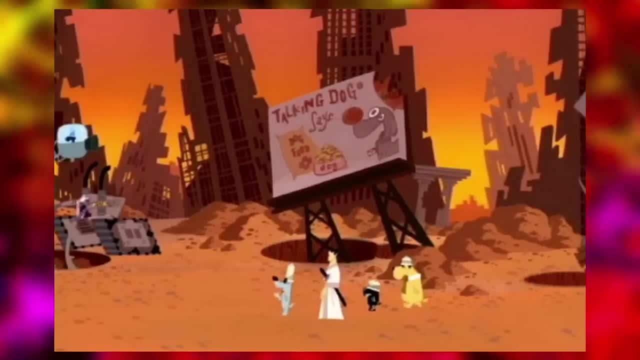 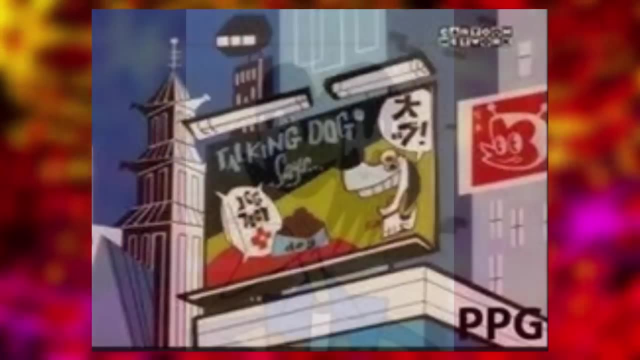 by a dog food billboard. If you've seen Powerpuff Girls before, then, you already know that the same exact billboard was featured in the series. As for the Gorillaz Ace from the Green Gang, Green Gang replaced Murdock during the Now. 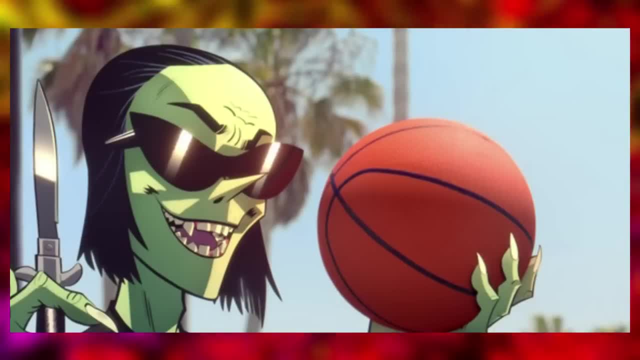 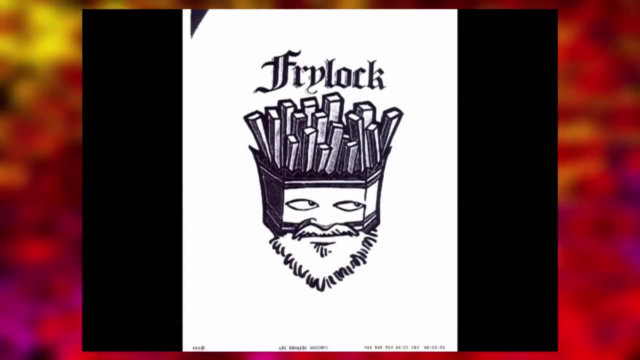 Now album cycle. It's pretty cool to see how all of these properties are linked together: Concept Art. So credit to Ronnie for hooking me up with a folder containing tons of concept art for Aqua Teen Hunger Force, Like this design created by Ben Prisk. 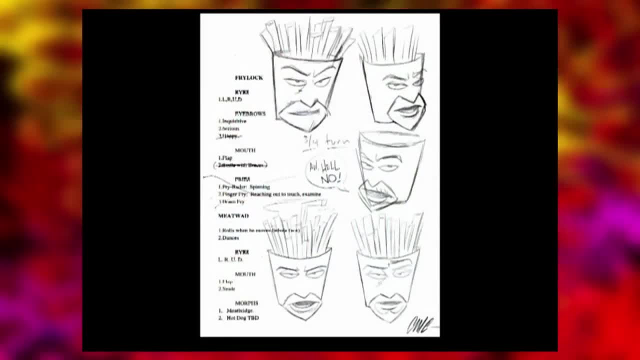 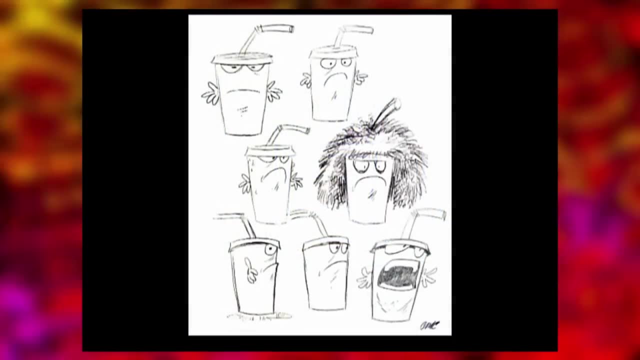 Look at those colors. These designs showcase early versions and concepts of the Aqua Teens, Like there's artwork of Meatwad turning into Jerry from Tom and Jerry And Master Shake with legs and arms, And also Frylock walking upside down using his fries as legs. 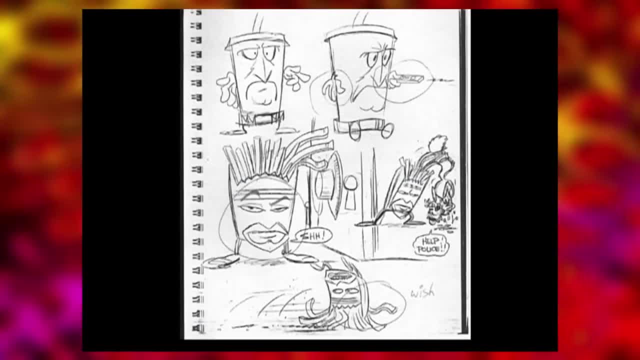 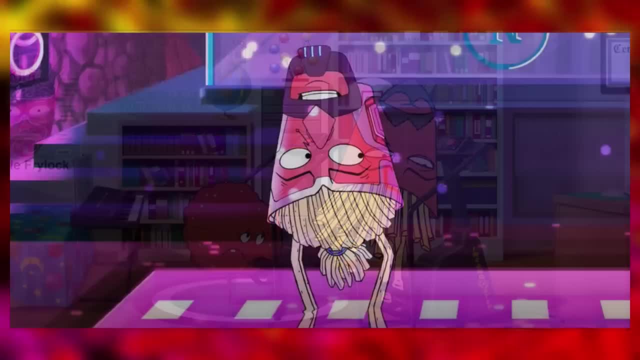 And while that aspect never made it into the final Frylock design, Frylock is seen upside down using his fries as legs on the Stairmaster machine in the episode Chick Magnet and also in the dancing scene from Plantasm. It's cool to see failed concepts and ideas get reworked. 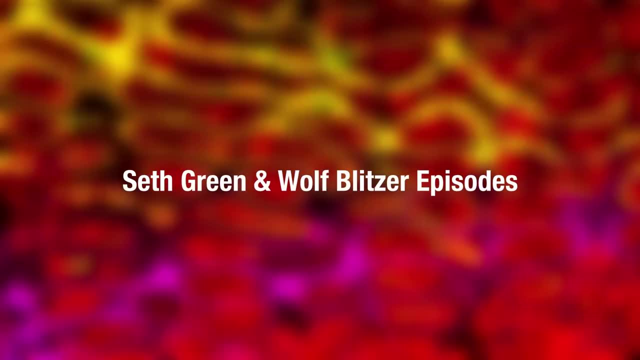 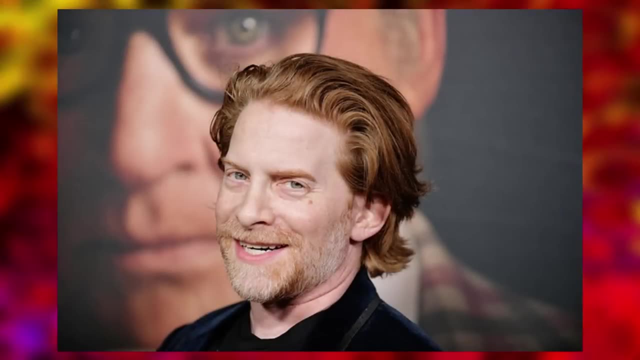 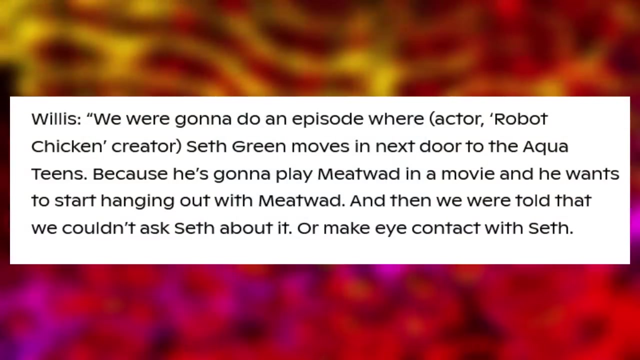 Or reused Seth Green and Wolf Blitzer episodes. According to a waborg interview, David Matt wanted to make two episodes featuring Seth Green and Wolf Blitzer. The Seth Green episode would have featured Seth moving in next door to the Aqua Teens because he was going to play Meatwad in a movie and he wanted to start hanging out with 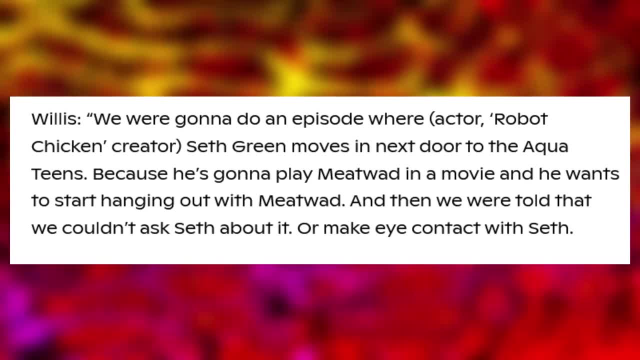 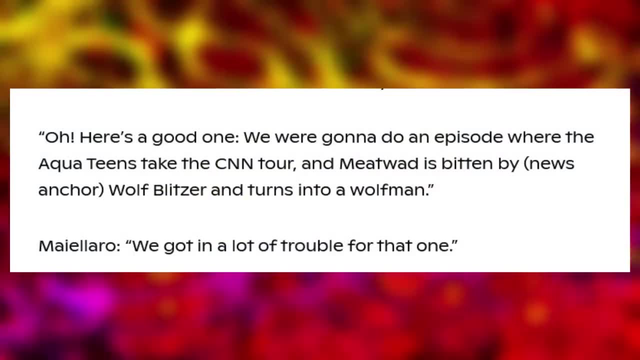 him, But apparently the creators were told that they couldn't ask Seth about it or even make eye contact with him. Seth Green was in an episode of Aqua Teen, though for like a brief second. In regards to the Wolf Blitzer episode. the Aqua Teens were going to take a tour of Seth's. 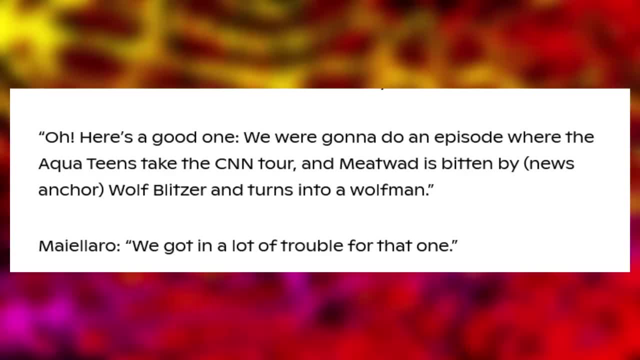 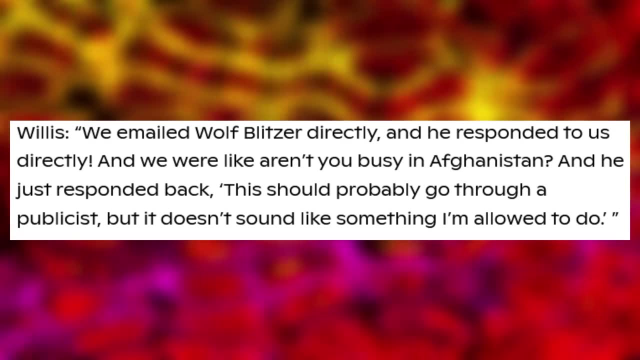 channel and Meatwad was going to be bitten by news anchor Wolf Blitzer and turn into a Wolfman. But according to Dave, they emailed Wolf directly about this. They asked if he was busy in Afghanistan and Wolf replied with: This should probably go through a publicist, but it doesn't sound like something I'm 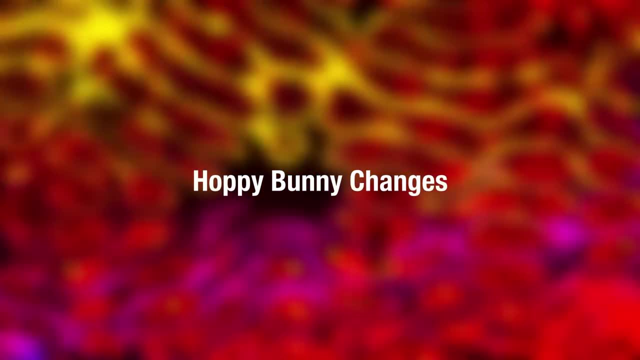 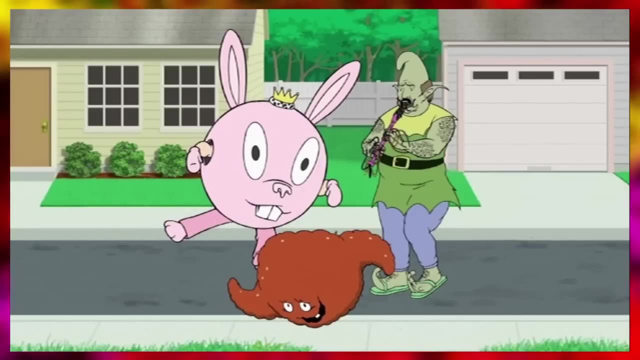 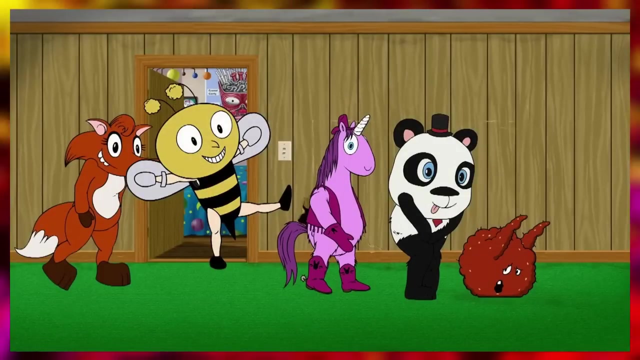 allowed to do Hoppy Bunny changes. According to the Volume 6 DVD commentary, this episode radically changed throughout the development process. At one point, Carl was supposed to summon rats with his recorder And later, down the road, Frylock and Hoppy Bunny were supposed to form an intimate relationship. 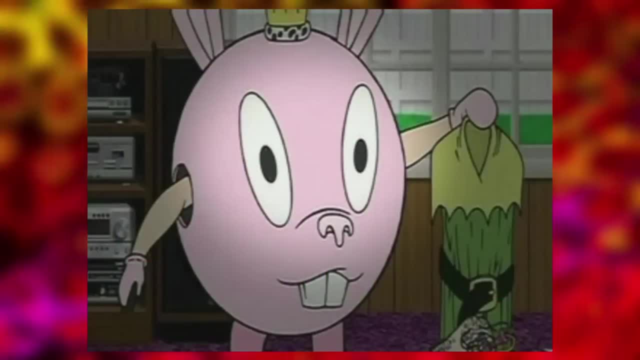 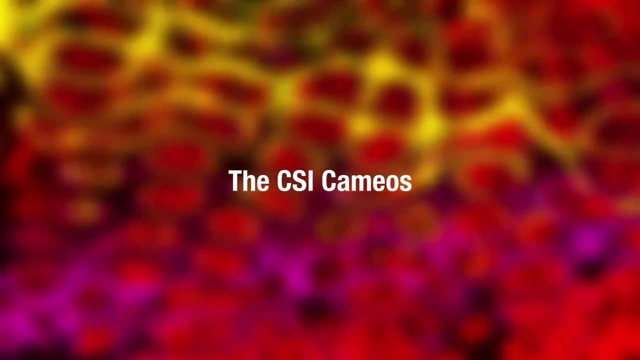 and Carl would become a griffin and slaughter everyone. And Hoppy Bunny was also originally named King Furry. Wow, that's a lot of changes. The CSI Cameos In the CSI episode Formalities, the Aqua Teen episode Video Ouija can be seen playing on. 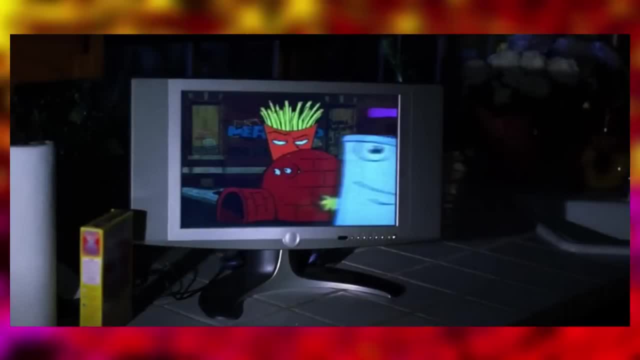 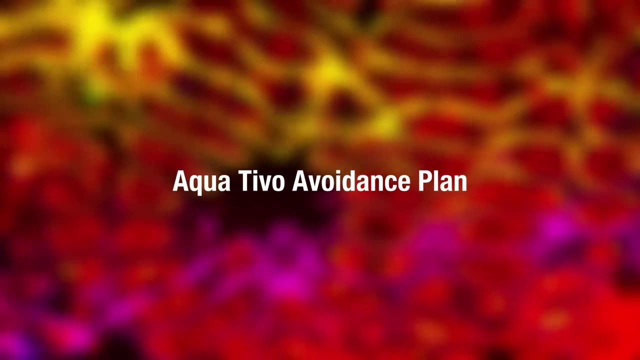 the television set in the hotel room And the Aqua Teen opening is also seen in the CSI episode Spark of Life, Aqua Tevo Avoidance Plan. So Aqua Teen Season 10 was originally going to be called Aqua Tevo Avoidance Plan. but 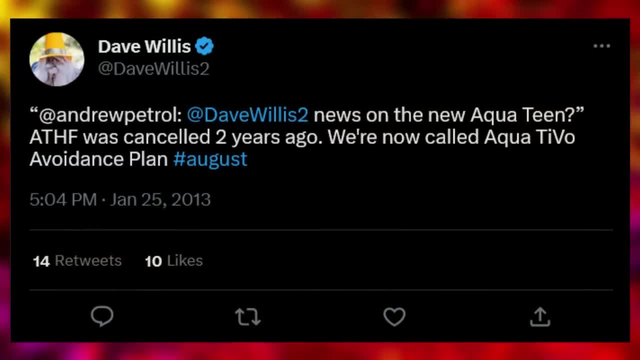 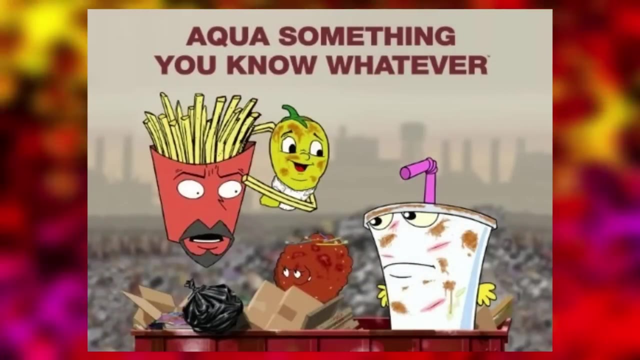 was renamed to Aqua TV Show Show. There's no exact reason on why the title was changed, but my guess is that the creators probably changed it as to not start any trouble with the Tevo Company Pepe the Pepper. When Season 9 of Aqua Teen was first being promoted, outlets like IGN announced that. 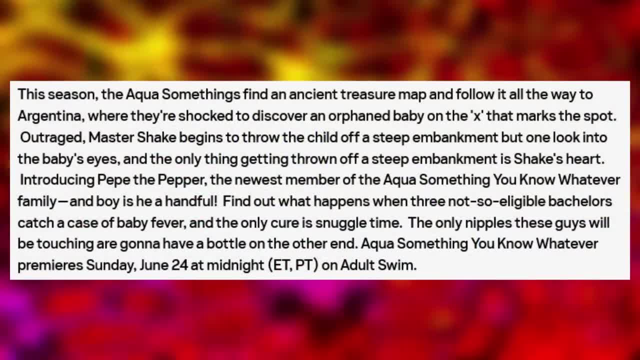 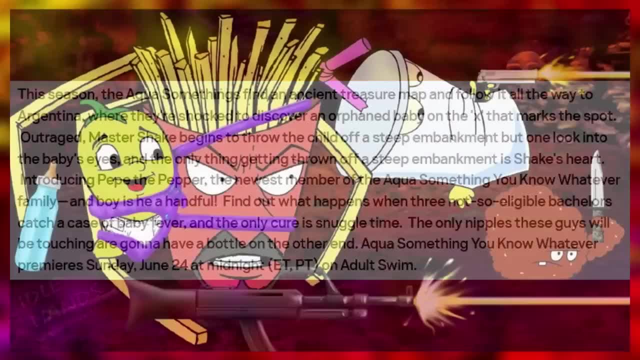 Shaq, Frylock and Meatwad would find an ancient treasure. Follow it all the way to Argentina and find an orphaned baby on the X that marks the spot. That baby was Pepe the Pepper. The creators announced that the Aqua Teens would bring Pepe home and raise him for the 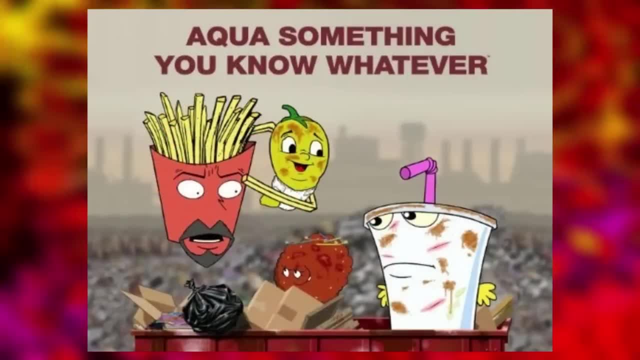 entirety of the season. However, that never happened. Pepe the Pepper was a gag character. He had never been seen or mentioned at any point in the series. He was only featured in the season's promotional material, The Minora Team Alarm Clock. 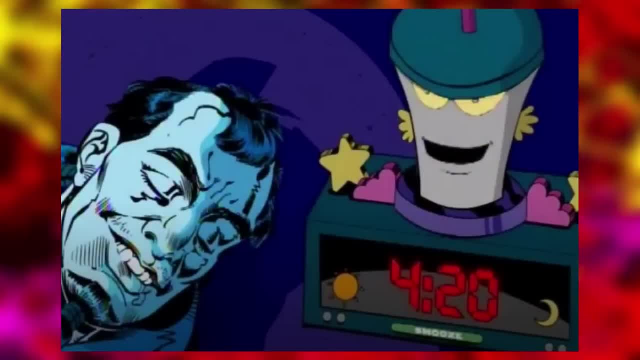 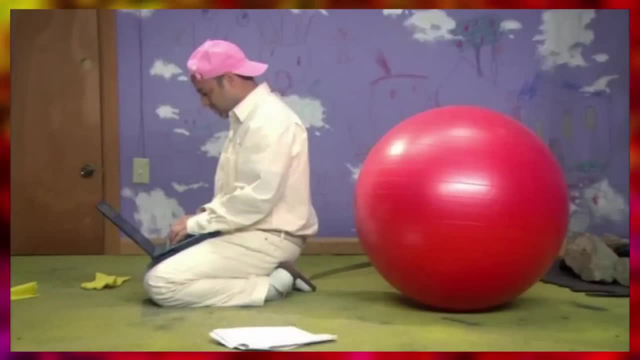 There is a Master Shake Alarm Clock in the Adult Swim series Minora Team, specifically the episode Tremendous Class Laser Cowboy. Laser Cowboy, according to Matt Malero, was a live-action feature for digital that Matt wanted to create back in either 2014 or 2015.. 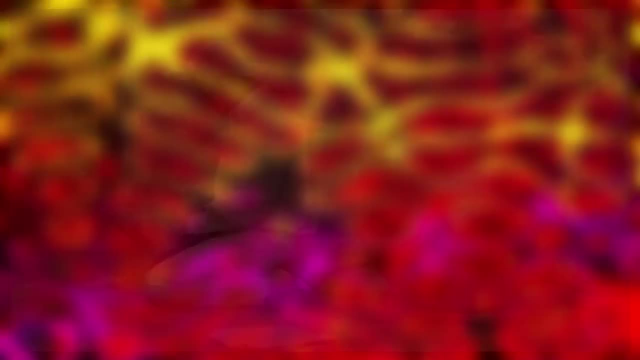 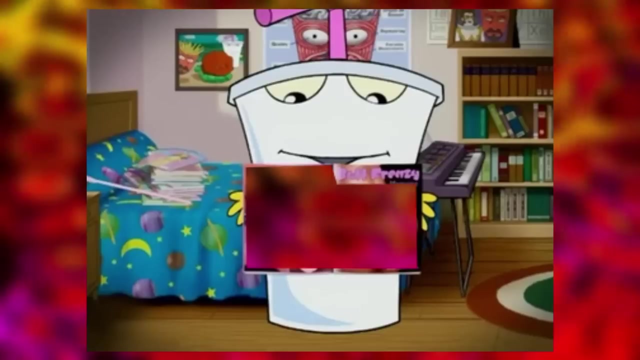 However, the idea never got pushed through. Butt Frenzy Troll. So Butt Frenzy is a naughty magazine that's featured in episodes like The Meat Zone, Dirt Foot and Green Ripper Gutters. And, believe it or not, the butts featured in the magazine are the butts of the writers. 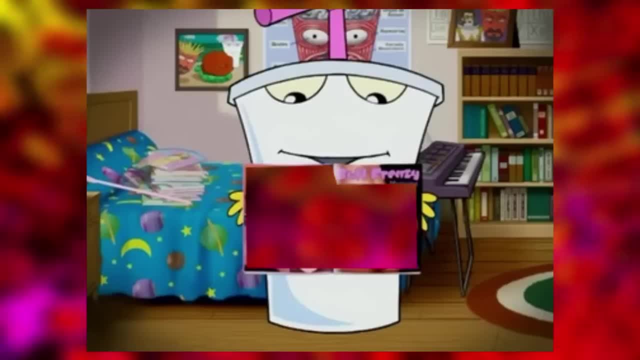 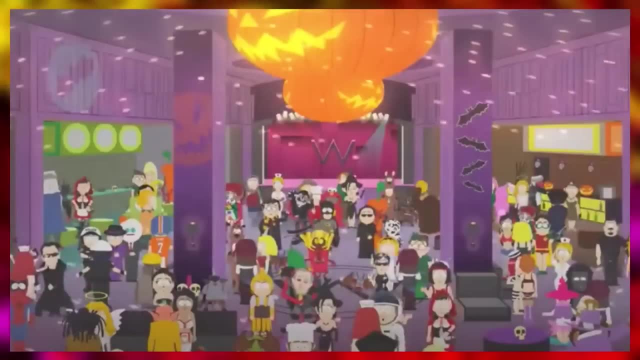 of the show. The reason behind this gag was so the writers could moon everyone who watched the series The South Park Frylock Easter Egg. In the South Park episode Hell on Earth 2006,, someone is seen dressed up as Frylock at Satan's. 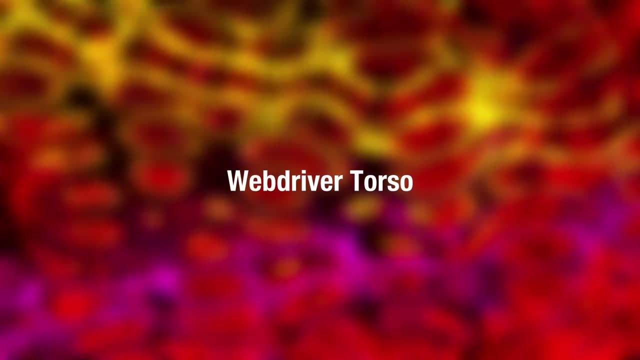 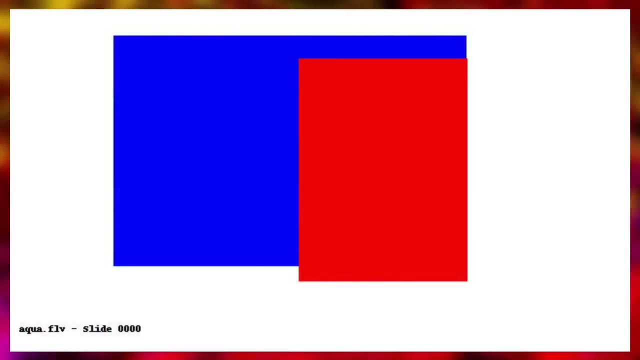 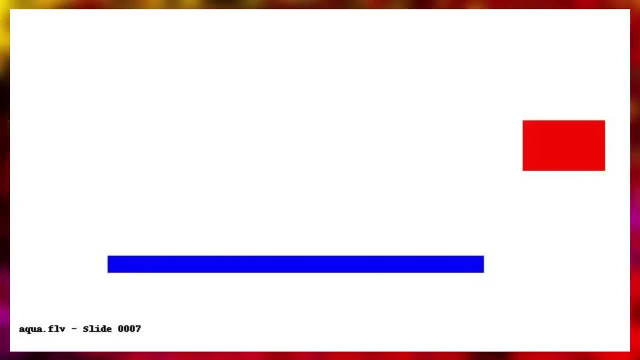 party. Webdriver Torso. Webdriver Torso is a YouTube automated performance testing channel that blew up in popularity around 2014.. The videos featured on the channel are slideshows showing two colored rectangles. Most of the videos are 11 seconds long, but there are videos on the channel that are also 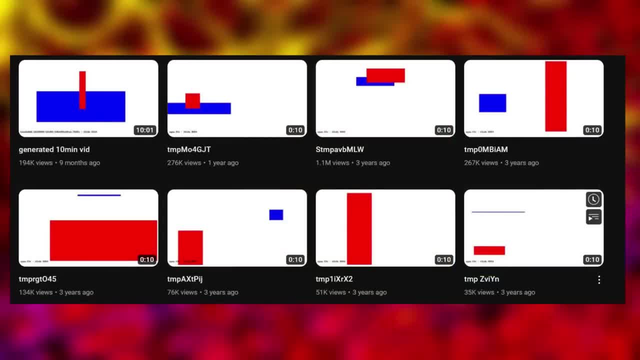 1 minute, 5 minutes or even 25 minutes long. Prior to the channel being confirmed by Google and YouTube as a performance testing channel, it was heavily speculated that the channel was created by extraterrestrial life trying to contact humans construction plans, and some have even speculated that the channel 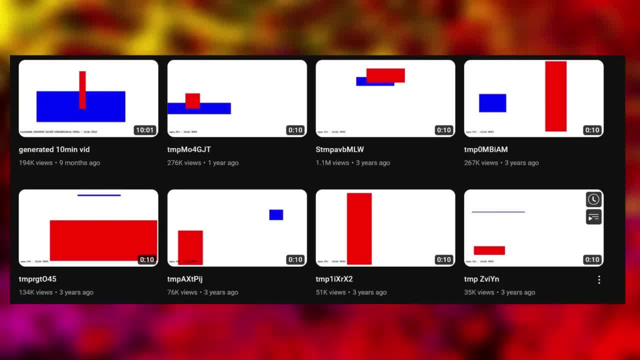 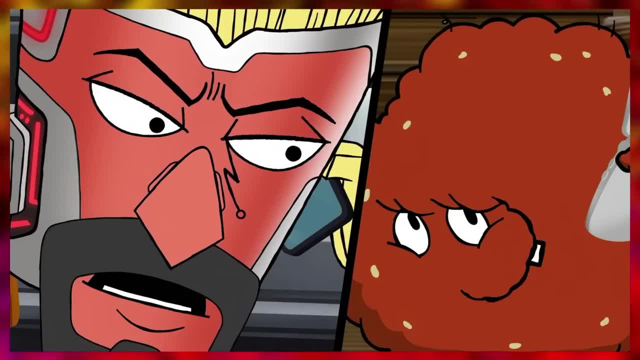 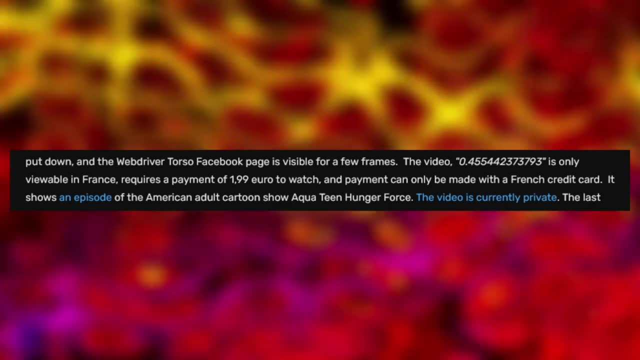 was a Cicada 3301 recruitment program. So how the hell is Aqua Teen Hunger Force involved with Webdriver Torso? Well, one Webdriver Torso video, only viewable in France by the name 0.455442373793, features. 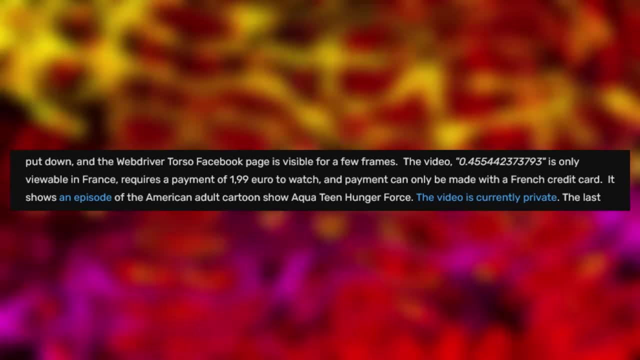 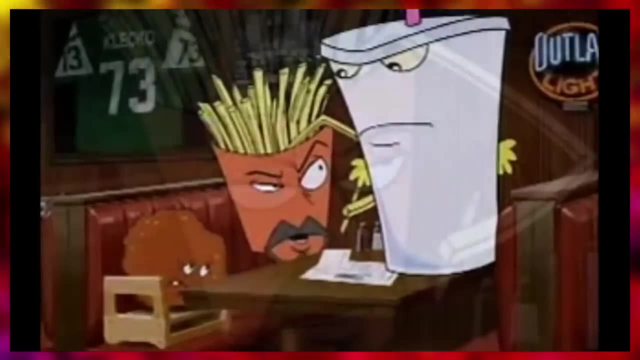 an episode of Aqua Teen Hunger Force, specifically the episode Super Trivia. Prior to the video's privatization, the video costed a payment of €199 to watch and could only be bought using a French credit card, And the episode was the Spanish version. 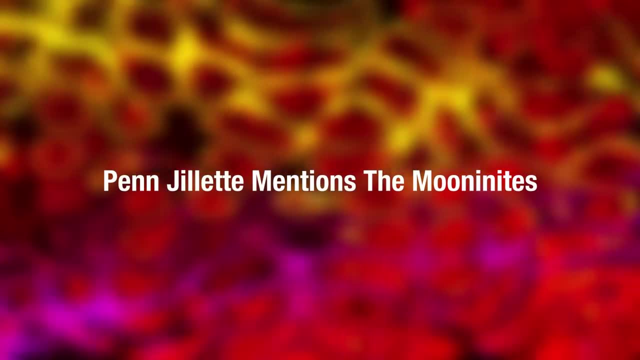 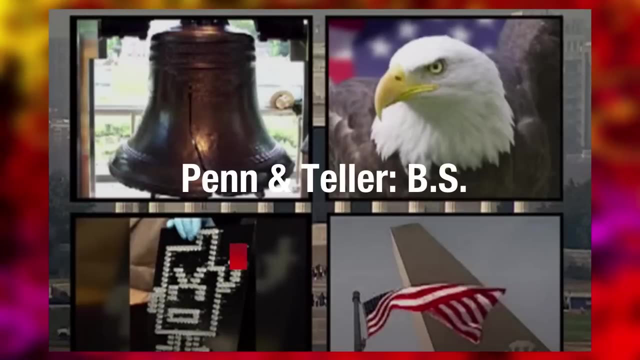 It's like dub, because why not? Penn Jillette mentions the Muna-Nights. Magician Penn Jillette mentioned the Muna-Nights in the Penn & Teller bull**** episode Mount Rushmore- Underrated series, by the way, go check it out. 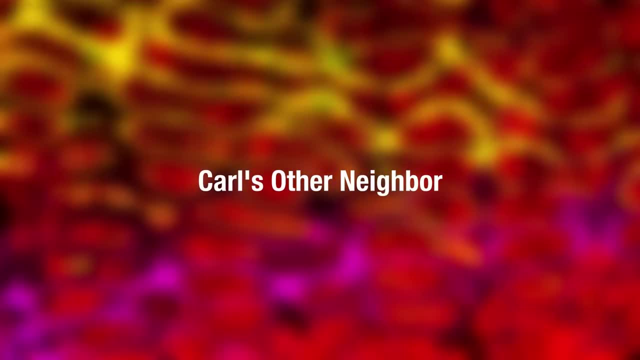 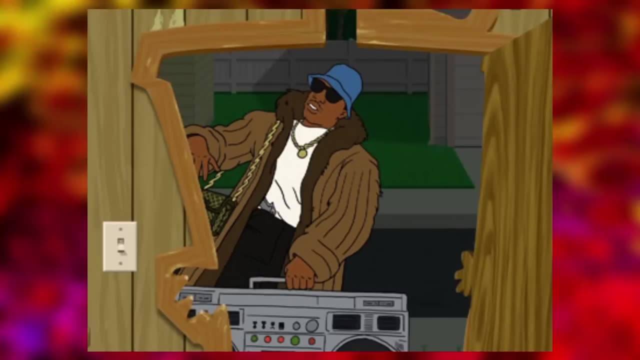 Carl's Other Neighbor. At one point there was an idea for Carl to have another next door neighbor, and that next door neighbor was potentially going to be Schoolie D. Obviously, the extra neighbor idea never went through, and that's possibly because the creators- the creators- felt that having an extra neighbor would have complicated things to an extent. 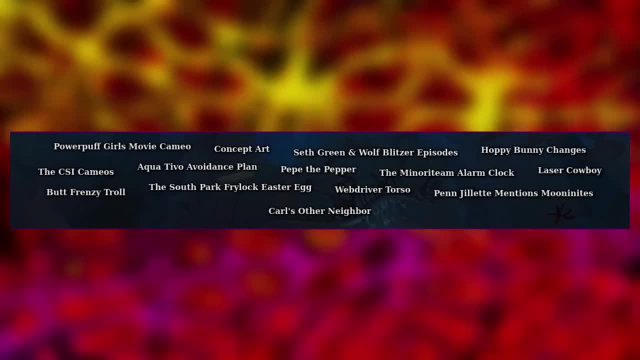 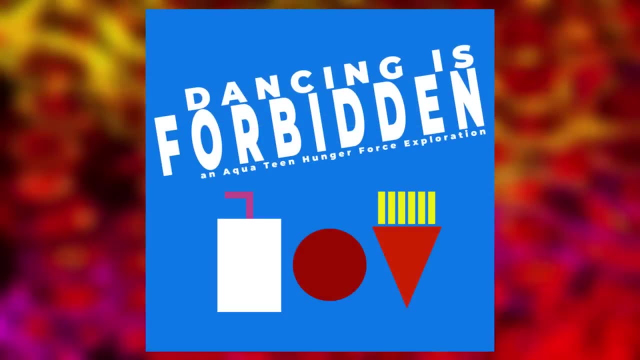 And that, my friends, was the sixth layer of the iceberg Yoo-hoo running crew. Ronnie, here from Dancing is Forbidden- a podcast all about Aqua Teen Hunger Force, Thanks to the absolute unit, the number one cool guy, Zero Omens, for letting me get myself. 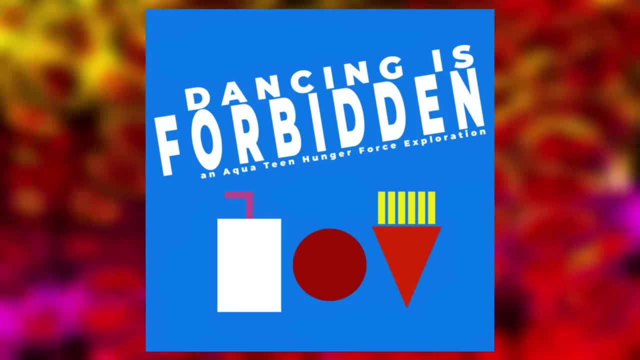 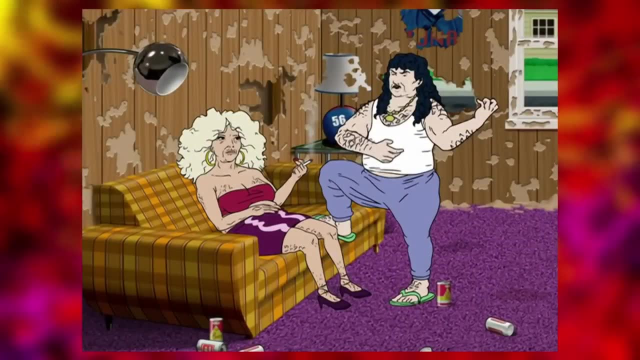 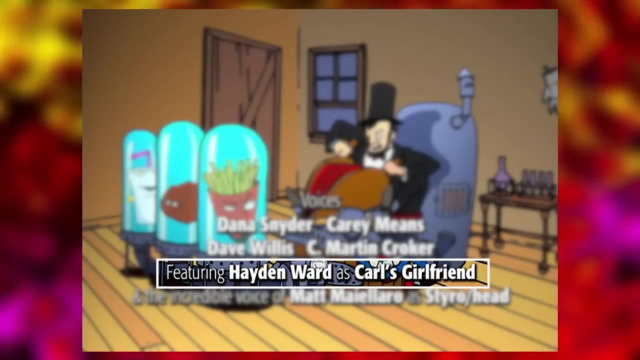 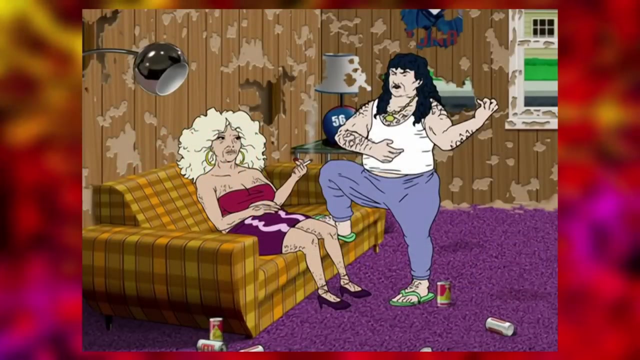 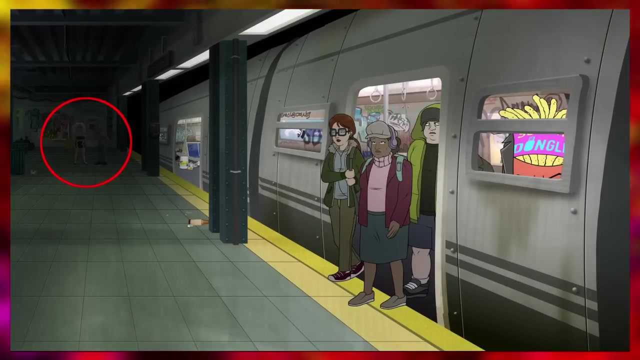 all over this filthy iceberg. Let's jump in and talk some teens. Recently in 2022's Plantasm. However, this iceberg entry isn't about the character of Carl's girlfriend, but rather her voice actress, Hayden Ward. What if I told you, without Hayden, Aqua Teen likely wouldn't exist? Do you believe me? Well, maybe I can convince you. Hayden Ward grew up in Conyers, Georgia. While I'm sure that Hayden did lots of cool stuff while growing up there, she did one thing that is particularly of interest to us. 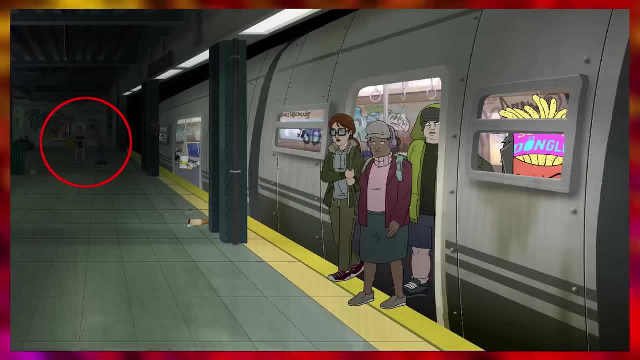 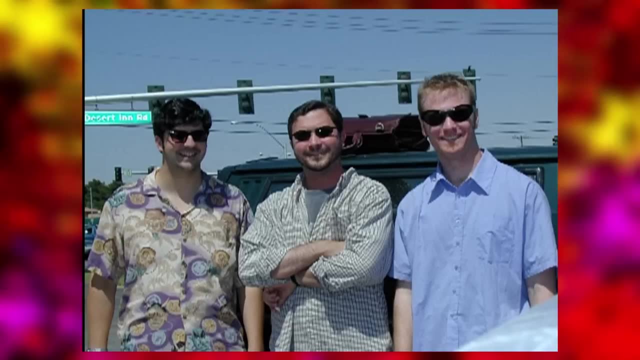 In high school, Hayden dated Aqua Teen co-creator Dave Willis. While Hayden and Dave didn't last as a couple, they did remain friends. So let's jump ahead a little bit. Let's jump to the year 2000.. 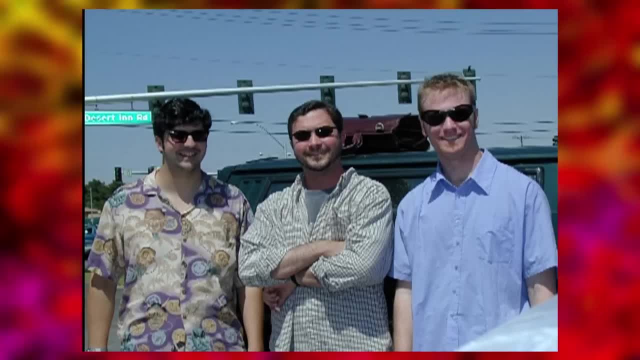 Hayden is living in New York City where she gets a call from her buddy, Dave. Now, usually when you get a call from somebody you knew in high school, it's to sign you up for some MLM thing, but that's not the case here. 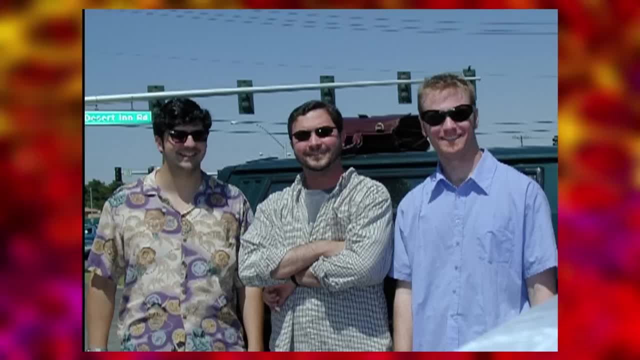 Dave tells Hayden that he's putting together his own TV show about talking fast food products and he's wondering if Hayden has any suggestions for the lead milkshake character. Luckily, Hayden knows a guy. See, Hayden's sister, Ashley Ward, went to Webster University where she met a dude named Dana Snyder. 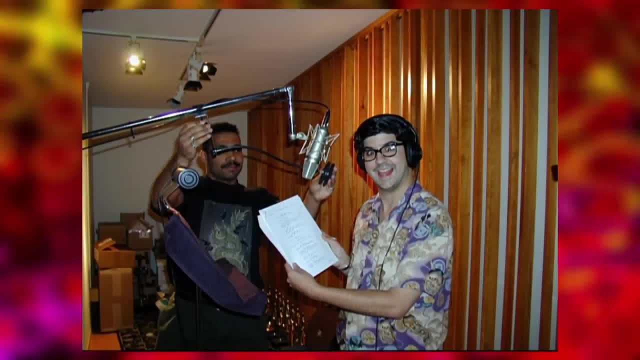 Ashley introduced Dana to Hayden and Hayden then suggested Dana to Dave for the role of Master Shake. And by the way, a side note on Ashley, she goes on to appear in Aqua Teen in the season three episode Robo-Sitter, as Sheila. 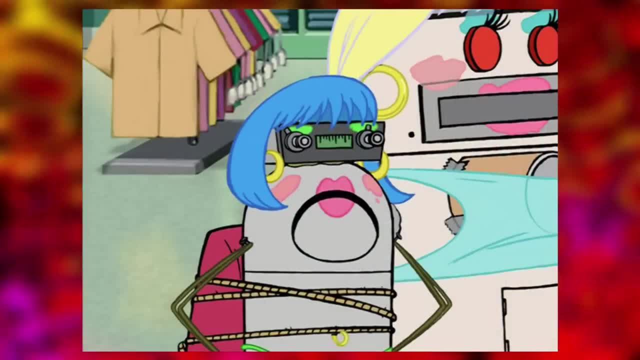 However, Hayden's influence on Aqua Teen does not end there. Remember how I said she was living in New York City. While there she was working at the UCB Theater, Hayden shared ticket booth duties with a guy by the name of Chris. 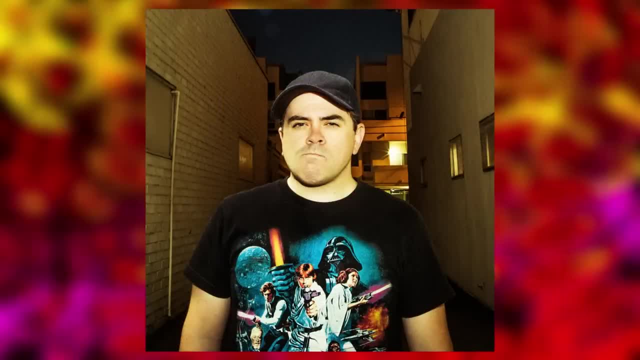 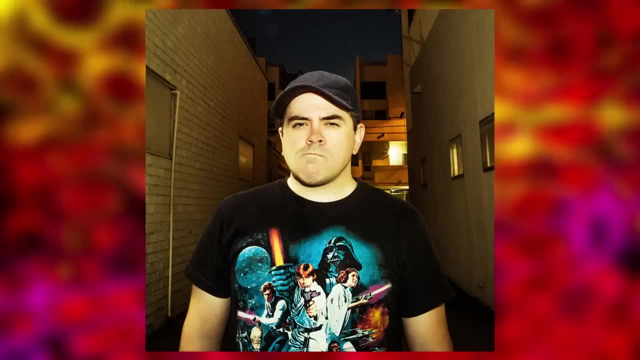 Chris Ward, also known as MC Chris, And despite sharing the same last name, the two are not related, Believe me. I asked At some point in early 2000,. Dave Willis- he heads up to New York City. He had to go check on some C-Lab 2021 production stuff for Adult Swim. 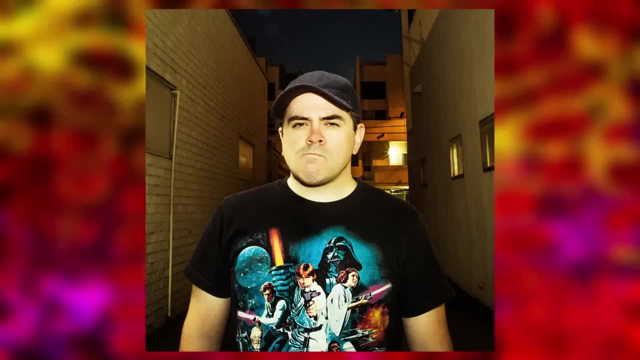 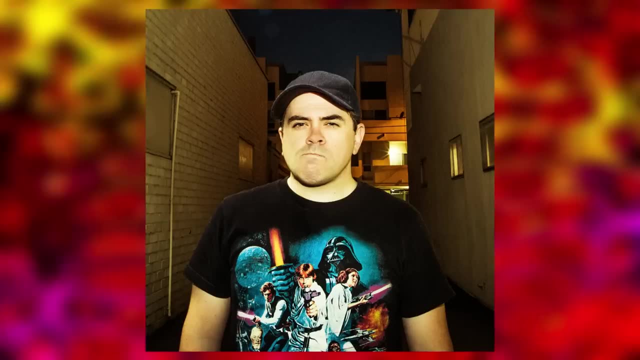 And while there he meets up with his friend Hayden and she brings along her buddy, Chris Ward. Chris goes on to impress Dave with both his drinking and humor skills And Dave tells Chris, man, you got to come on down to Georgia to work on my Aqua Teen show. 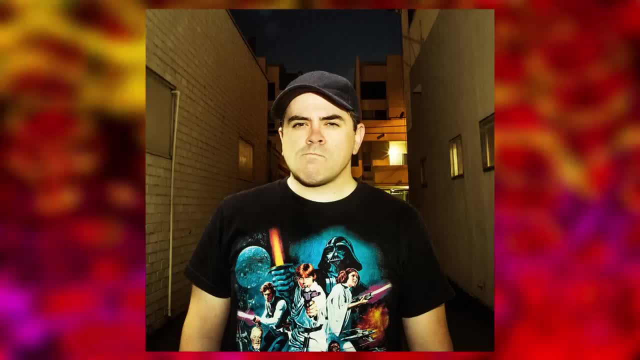 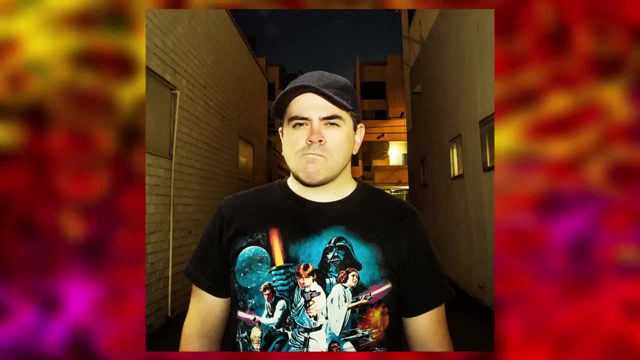 Chris. Chris says, no, I'm not going to do that. I want to stay in New York. So Dave sets Chris up with his C-Lab 2021 gig And, as you know, Chris eventually does come down to Georgia to not only be the voice of. 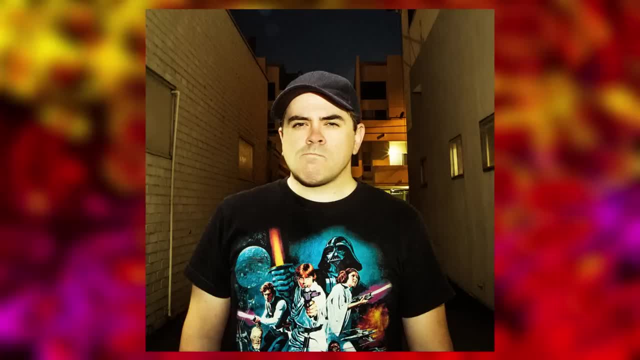 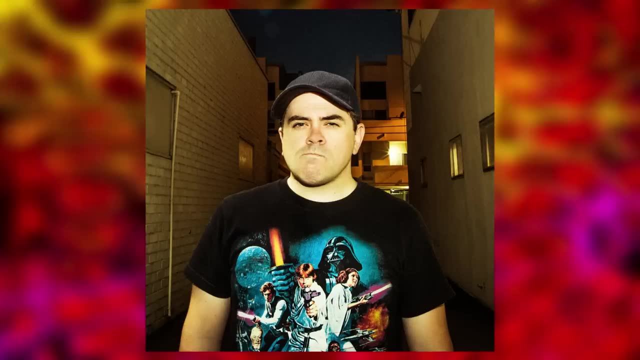 MC Peepance on Aqua Teen, but also a production assistant on the show. So that is Hayden Ward's influence on Aqua Teen. Not only is she the first English speaking female voice on the show, but she brought on some of the show's biggest talents. 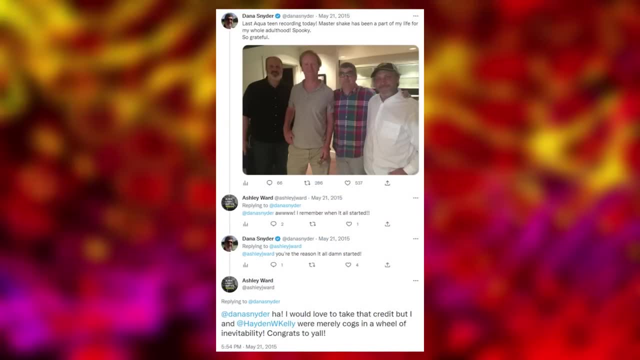 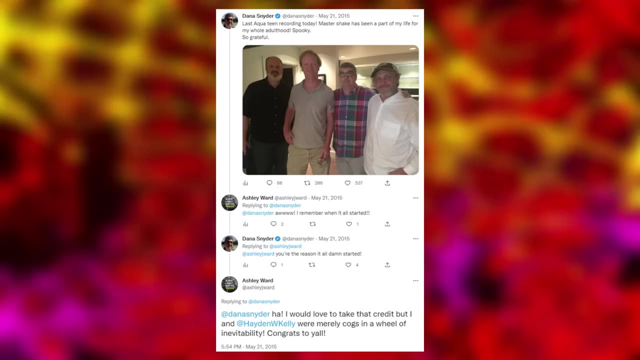 And I don't really think it's a controversial opinion to think that without her, this show probably wouldn't have been as successful as it was. So thanks, Queen, because I don't even want to imagine an Aqua Teen without Master Shake and MC Peepance. 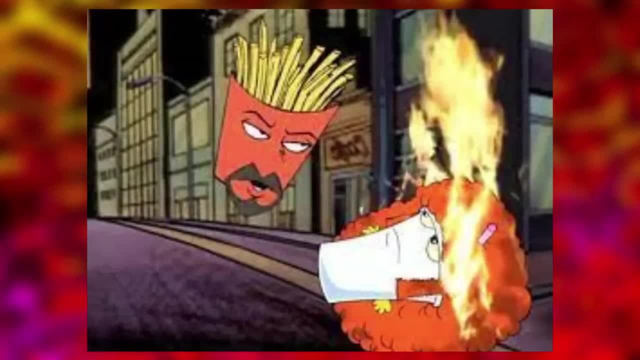 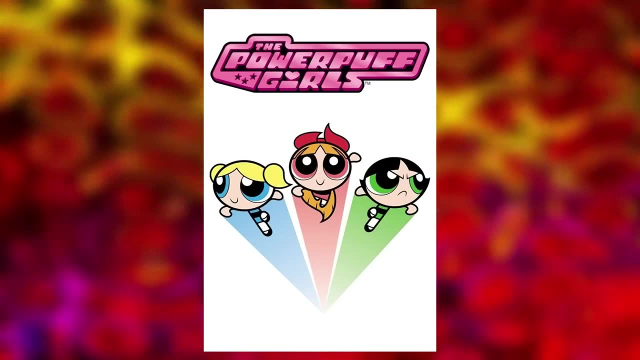 The Ring. While Aqua Teen has been featured in dramas like The Sopranos and Breaking Bad, as well as cartoons like C-Lab 2021, Brac Show and Powerpuff Girls, did you know that Aqua Teen Hunger Force was featured in horror film The Ring? 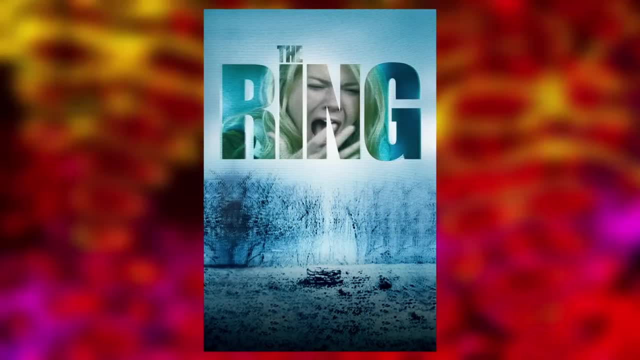 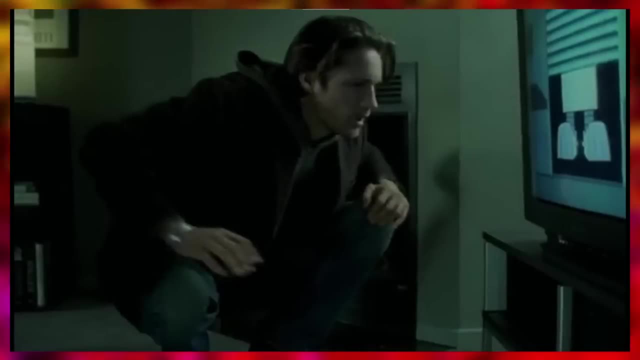 It was a deleted scene, unfortunately, but we do see the boy in the film watching the episode, Rabot, And not only is Aqua Teen heavily featured in that clip, but you also hear the audio from it as well. Both Matt Malero and Dave Willis loved the idea of a haunted videotape. 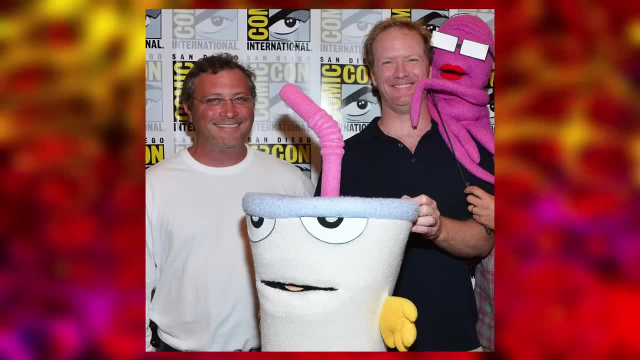 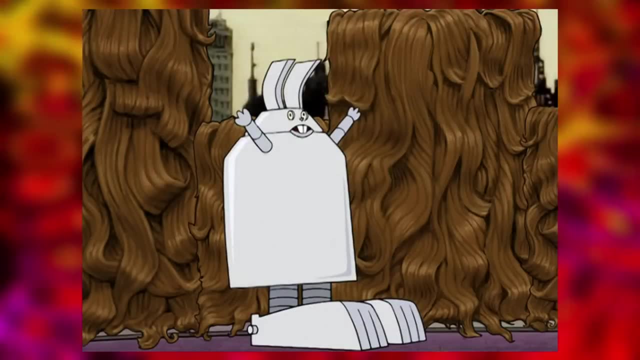 as in, they loved how dumb the idea was and they constantly made fun of it. Space Ghost in Rabot. Since we're talking about how Rabot was almost in The Ring, let's talk about how Space Ghost was almost in Rabot. 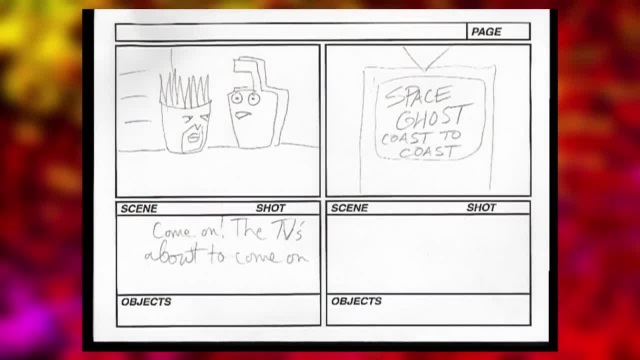 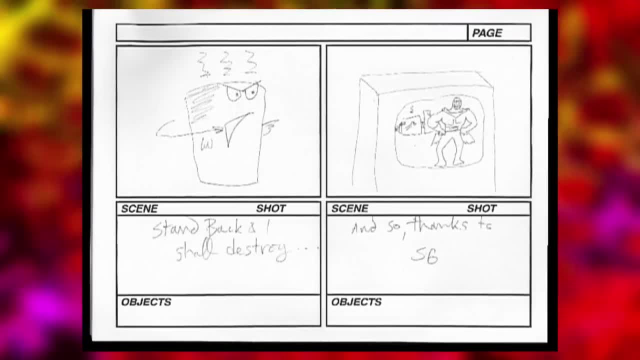 On the Volume 2 DVD, we get a ton of concept art, behind the scenes photos and even some storylines. We also get some storyboards, which is interesting because Aqua Teen ultimately wasn't storyboarded, but it looks like they tried to do it when creating this first episode of the show. 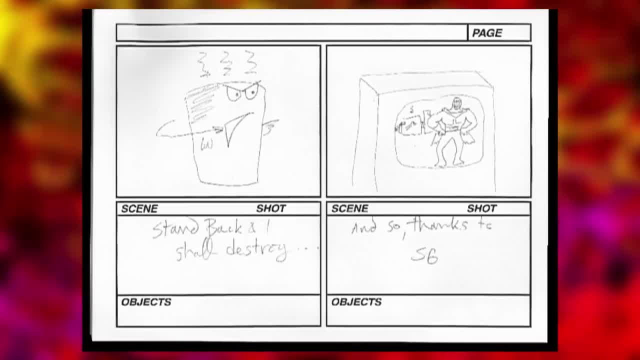 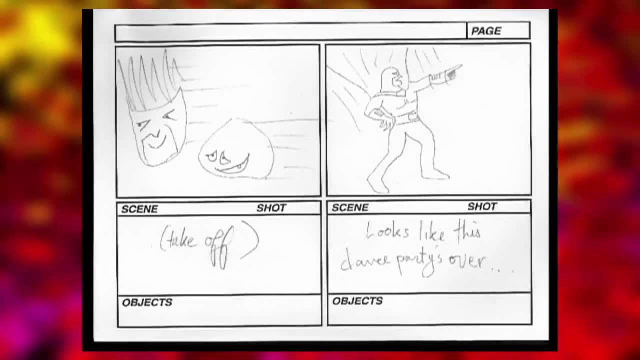 Space Ghost is actually featured several times throughout the storyboard art. First, the Aqua Teens are supposed to watch Space Ghost on TV and secondly, Space Ghost is supposed to show up and defeat the Rabot himself, which is obviously a big turn from where that episode ultimately went. 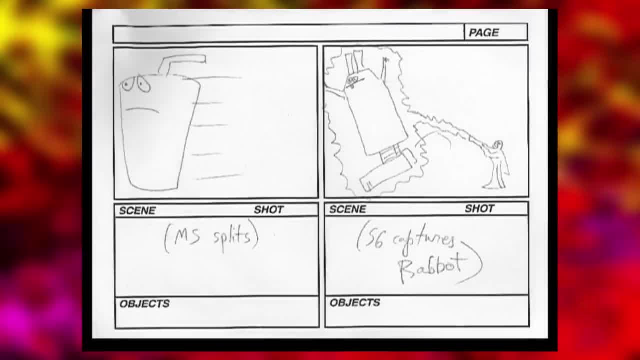 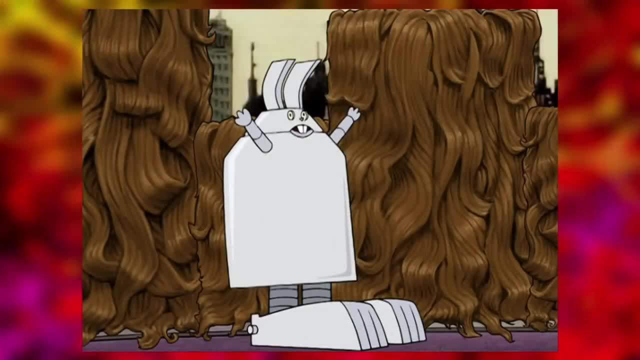 and is such a different tone from what the show ended up being that I am just glad they did not do this, because the point of that episode is that they don't defeat the Rabot. It's still downtown, wreaking havoc while the Aqua Teens are in the pool kind of ignoring it. 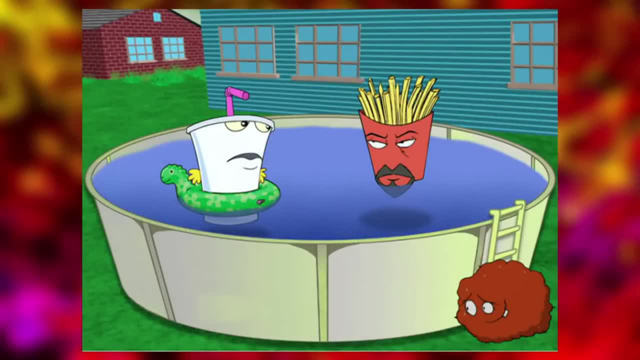 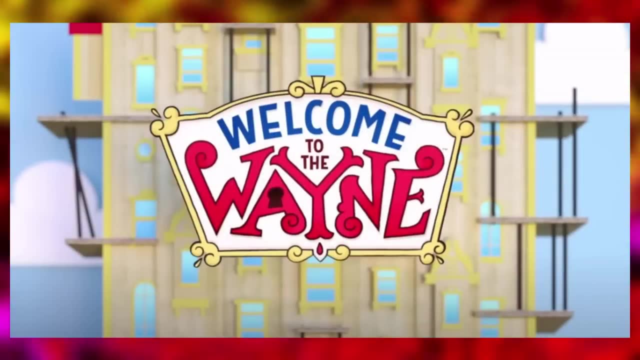 And, as you know, that is the tone that the show successfully took, but still, I think this is a fun piece of Aqua Teen trivia. Welcome to the Wayne- Welcome to the Wayne was a cartoon on Nickelodeon that ran from 2017 to 2019.. 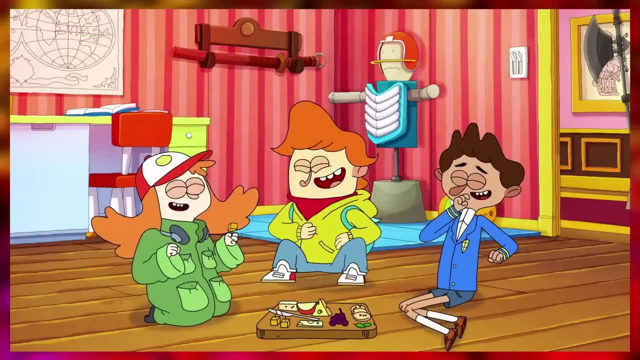 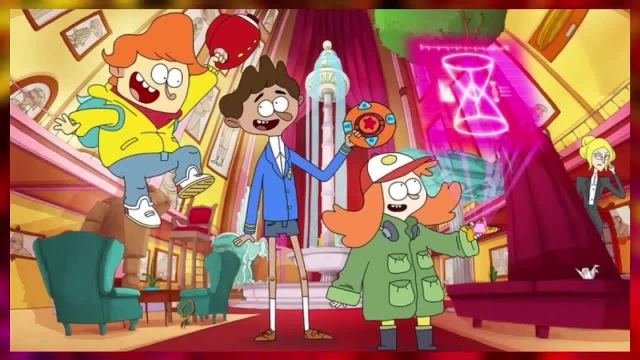 The cartoon follows the adventures of 10-year-olds Ansi Molina and Ollie Timbers as they explore their apartment building and get mixed up in the craziness of the strange tenants that reside inside the Wayne- And I know you're thinking now. 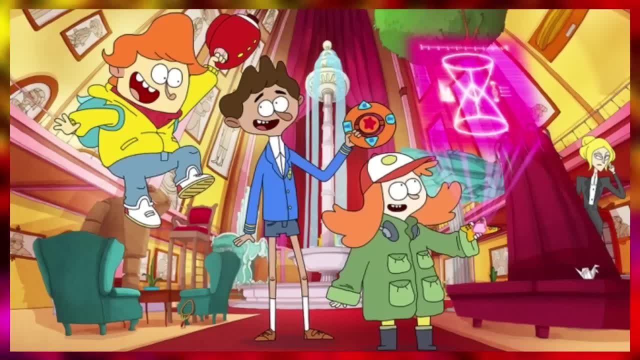 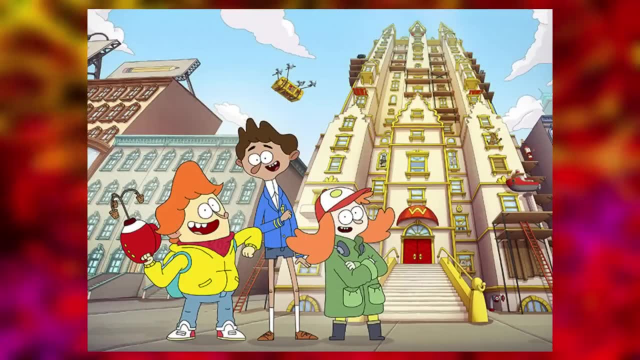 okay, Ronnie, cool. why are you telling me about this other show? This is an Aqua Teen iceberg. Why did Zero Omens let you on here? Slow down there. I'll tell you why you care about this. because Aqua Teen crew Dave Willis, Carrie Means and Dana Snyder. 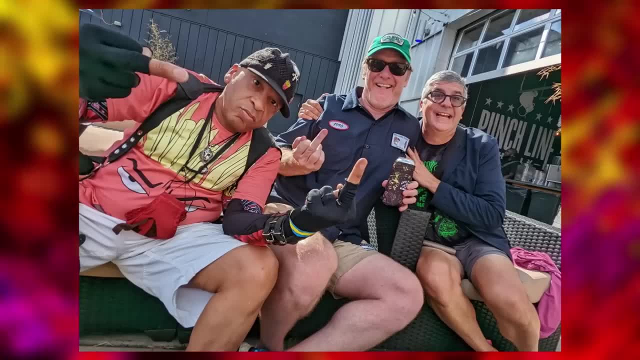 all play major supporting characters on the show across many episodes, So that's right. they didn't just play one character one time. they play many characters that show up multiple times throughout the show's short run. Some of them even show up in the same episode together. 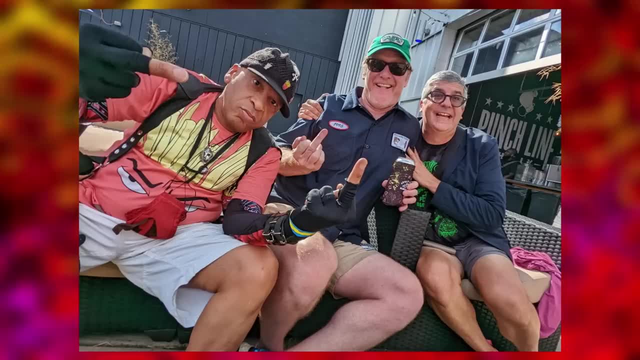 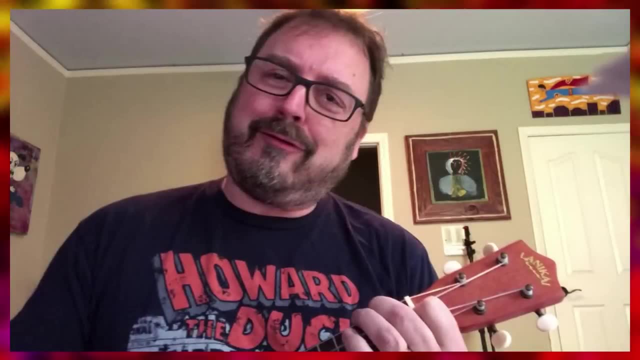 so you might see Dana Snyder and Dave Willis trading some lines in an episode, And worth noting that Matt Melero, as well as Oglethorpe voice actor Andy Merrill, who you know also voices Brak- both those guys show up a couple times on the show as well. 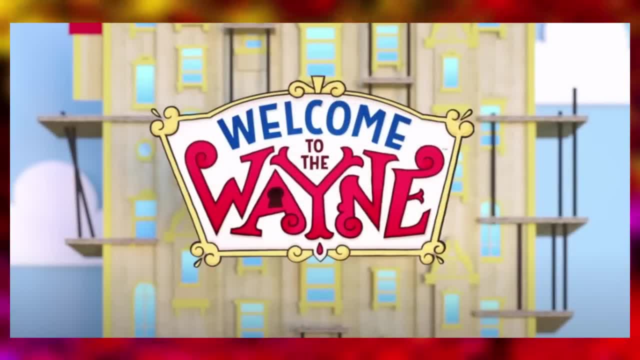 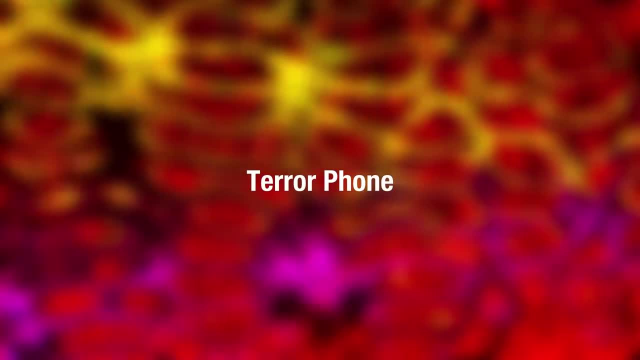 So if you're ever sitting around, you want to hear these guys' voices, but you don't want to watch Aqua Teen for some weird reason, Turn on. Welcome to the Wayne Terror phone. Terror Phone Trilogy is a series of horror short films spread across the final three Aqua Teen DVDs. 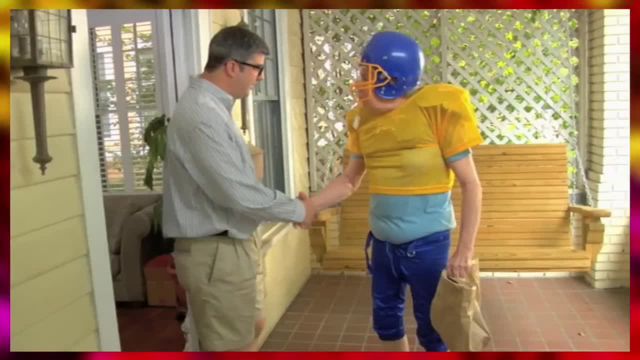 These are cool because they're live action and you get to see a lot of the cast and crew from Aqua Teen in them. All three shorts are absolutely incredible and interlinked, but I'll just describe the first one to you. Dana Snyder plays a man who receives a telephone from a high school football. 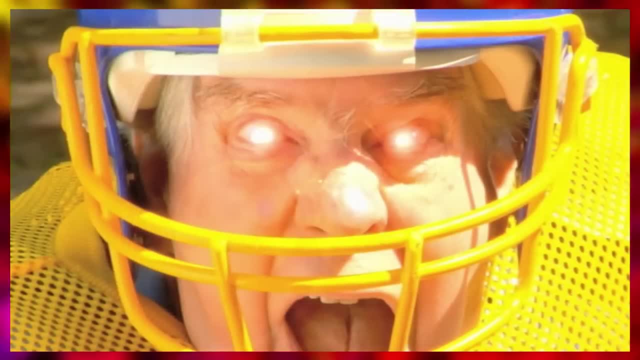 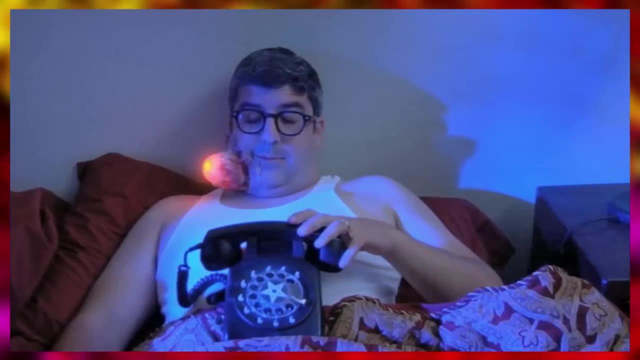 player, who's played by Don Kennedy, an old man who you might recognize from Assisted Living, Dracula or Vegetable Man. The phone ends up being haunted and tries to kill Dana's character, until Dana breaks the fourth wall complaining about how he doesn't like the script it makes. 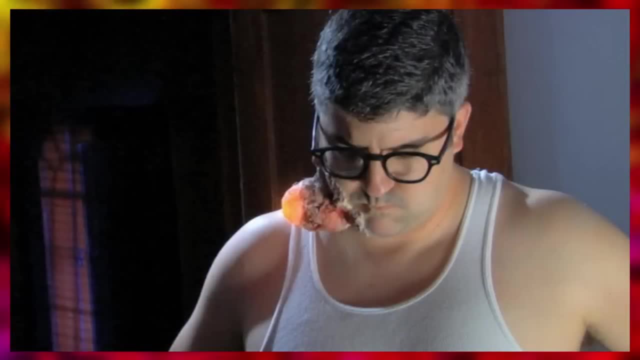 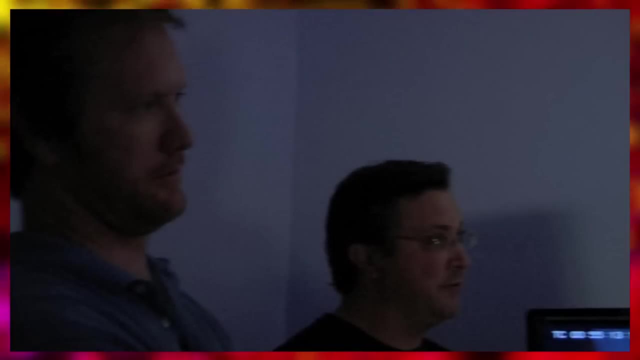 no sense, and particularly he doesn't like a line about having to give himself a butthole massage. The camera then pans to the other side of the room where we see Dave Willis and Matt Malero. There's some back and forth and eventually they bring Carrie Means in to replace Dana's character. 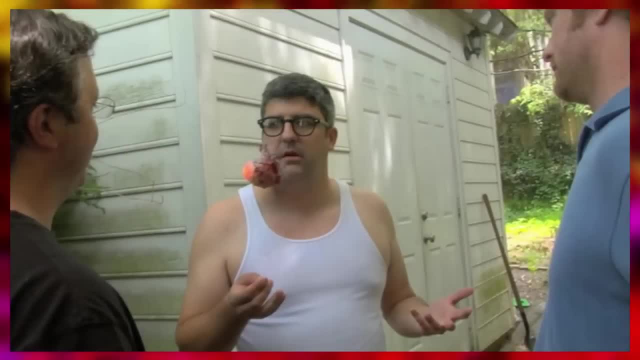 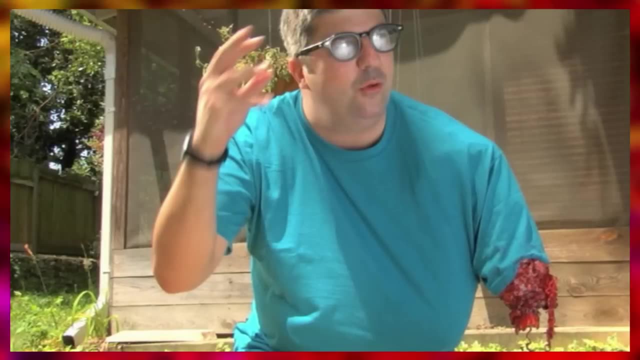 but Carrie can't quite get the lines right, so they fire him. They have to bring Dana back promising that he won't have to say the butthole massage line anymore, only for them to poorly and obviously overdub him saying that he's going to give himself a butthole massage. So that's only a part of it. There's way. 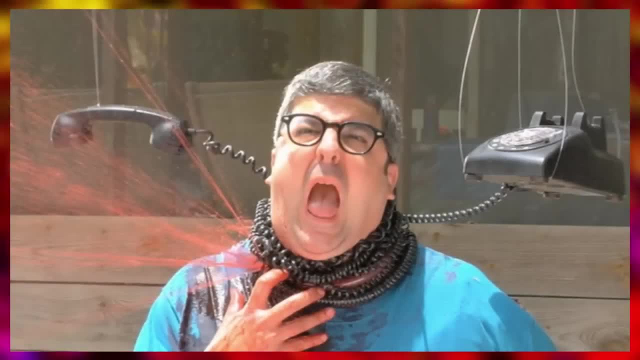 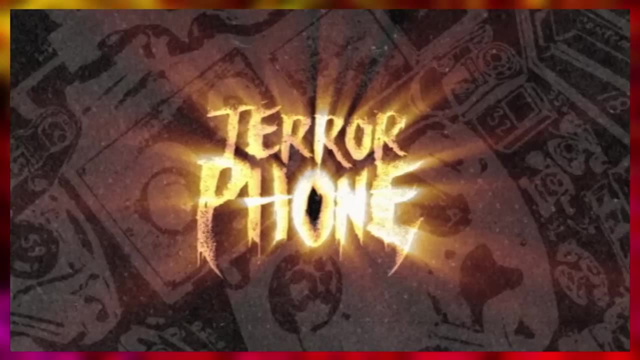 more to even just that first. short than that, They are very funny. There's some of my favorite things that the Aqua Teen crew have done, and I think it's just criminal that they never got to do a sketch series like this, because just seeing all these guys on camera playing around together, 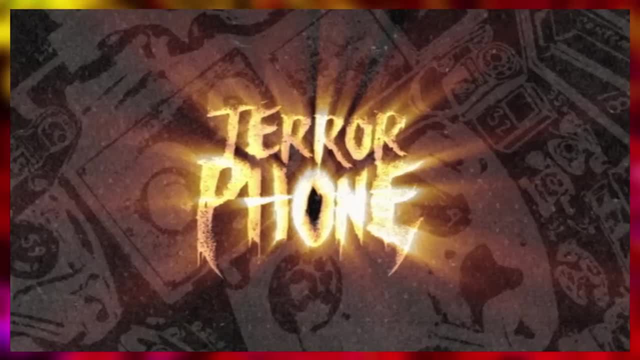 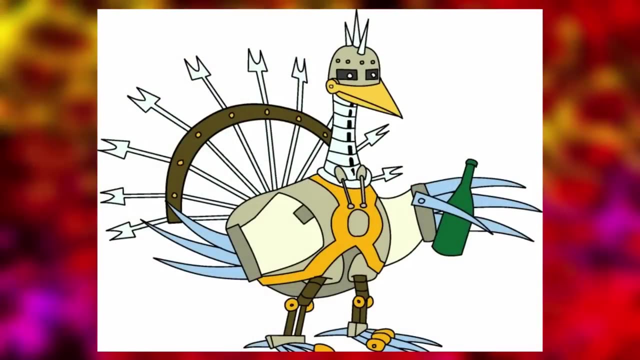 very fun. Check it out. If you don't have the DVDs, you could find them on YouTube. Golden Cyber: In Season 2's, The Dressing Turkatron shows up at the Aqua Teen's house to wreak havoc on their Thanksgiving. Very quickly, the teens figure out that the Turkatron seems to be the cybernetic. 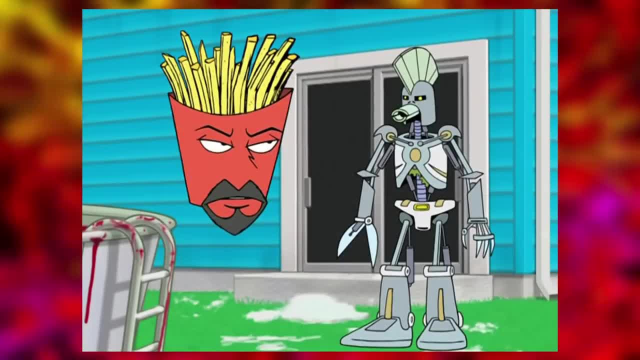 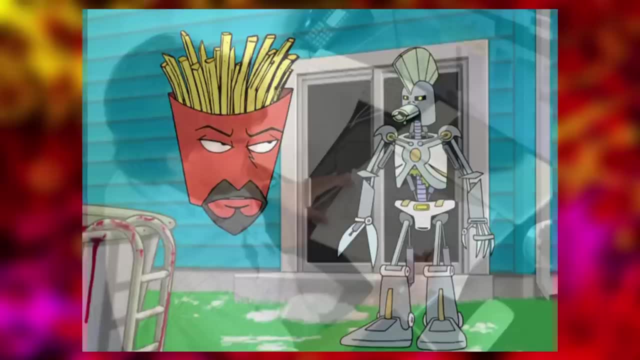 ghost of Christmas past from the future. and when confronted about this, Turkatron confirms the theory. Because Turkatron goes on long-winded stories, just like Cybernetic Ghost, we get a host of new images drawn by Ben Prisk to accompany these stories. When Turkatron reveals he is a 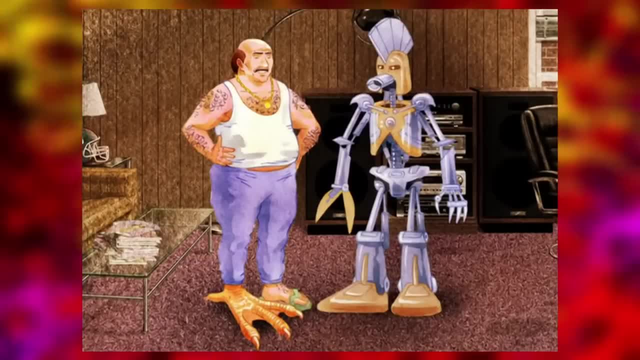 cybernetic ghost. we see a slide of Cybernetic Ghost standing next to Carl and, for whatever reason, the cybernetic ghost has a ton of gold trim on his armor like way more than he actually does in that episode. As a kid, I always thought this was awesome and spoiler alert. as an adult, 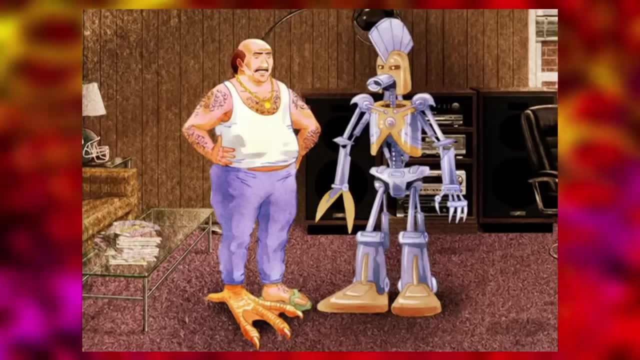 I still do. I think it looks great and I always wondered why. Was this supposed to have some sort of significance? Was this supposed to have some sort of meaning? Did Matt and Dave intend for this? So I reached out to artist Ben Prisk and asked him myself. Ben had this to say: 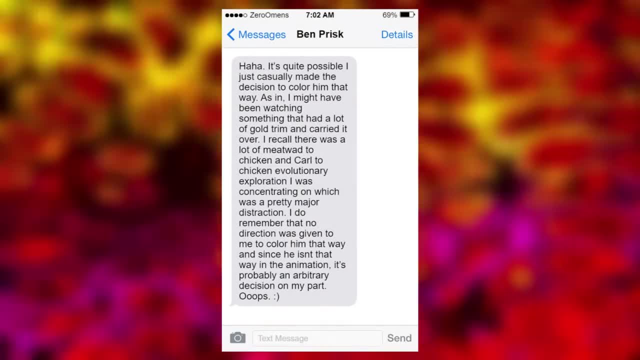 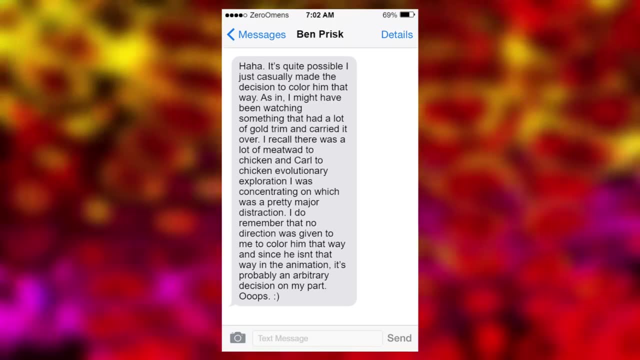 It's quite possible. I just casually made the decision to color him that way, As in I might have been watching something that had a lot of gold trim and carried it over. I recall there was a lot of meatwad to chicken and Carl to chicken. evolutionary exploration- I. 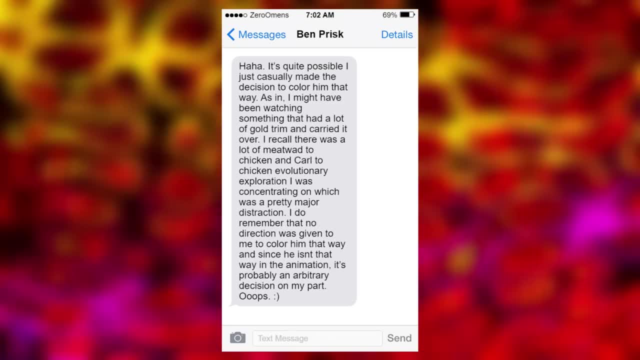 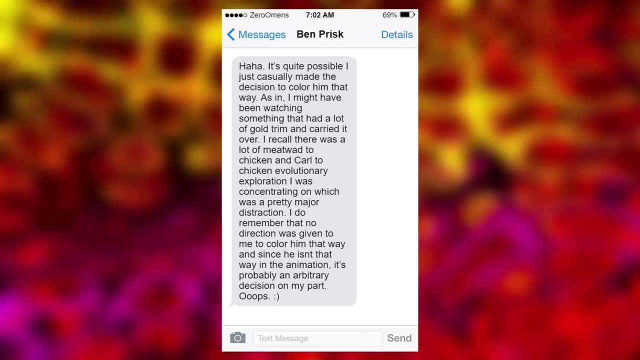 was concentrating on, which was a pretty major distraction. I do remember that no direction was given to me to color him that way and since he isn't that way in the animation, it's probably an arbitrary decision on my part. Oops, So there you have it from the man himself, some artistic. 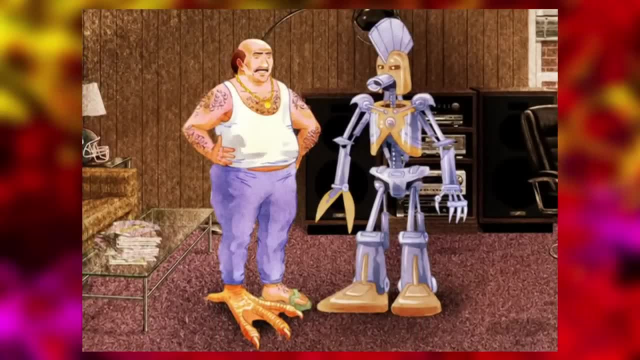 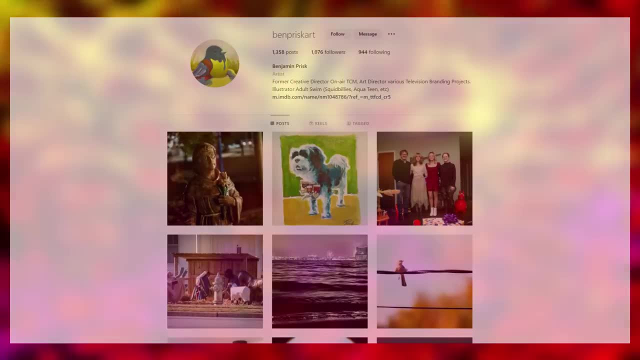 liberty taken and guess what? I think it paid off. I think it looks awesome. you can find Ben over on Instagram at Ben Prisk Art. he's got all sorts of cool stuff up there. check him out. Biff Pocoroba. Biff Pocoroba was a Major League Baseball player. 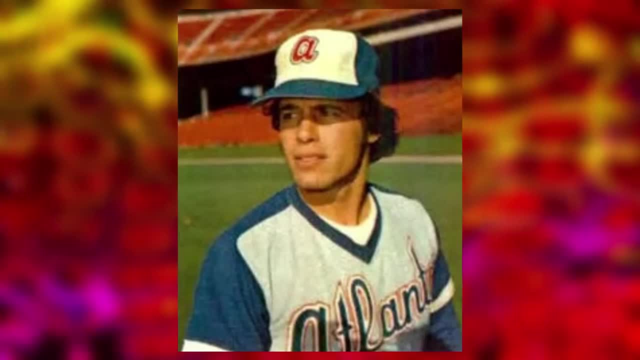 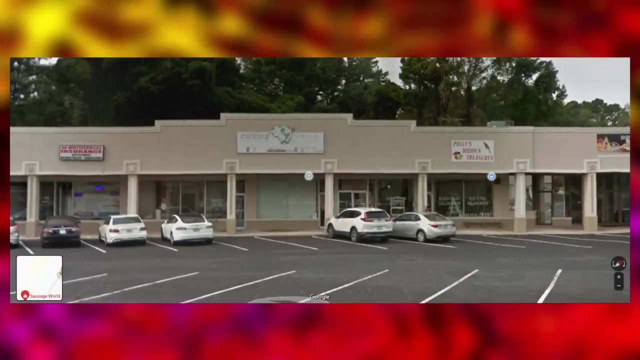 catching for the Atlanta Braves for 10 seasons, from 1975 to 1984.. After retiring, Biff operated a specialty meat business called Sausage World. That Sausage World fact not very important for you, but I wanted to say it anyways, because, wow, what a title on that one. Let me give you some. 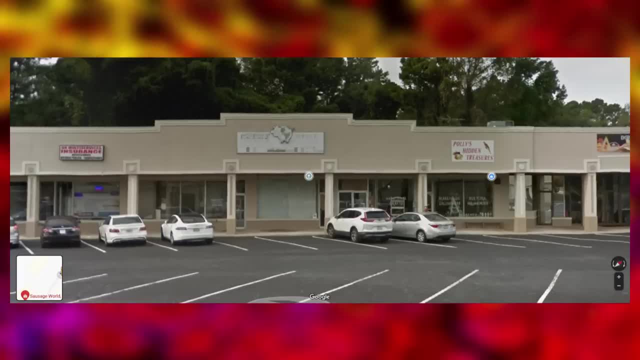 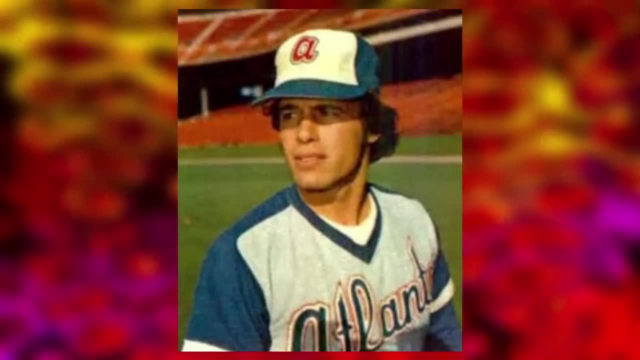 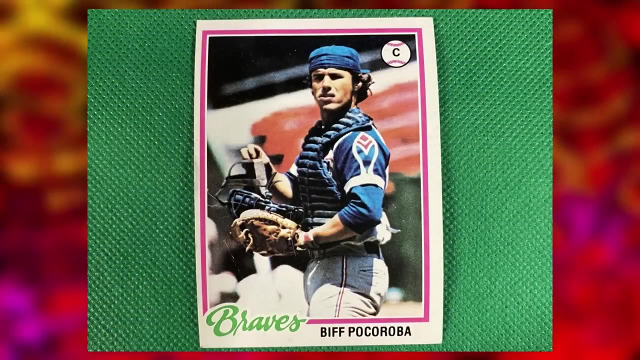 hints that you could answer. Biff Pocoroba. to Which player did Ted Turner purportedly try to trade for the San Diego Chicken? Biff Pocoroba. What baseball card does J Wade Edwards, Aqua Teen Hunger Force producer, carry in his wallet? Biff Pocoroba And our final trivia. 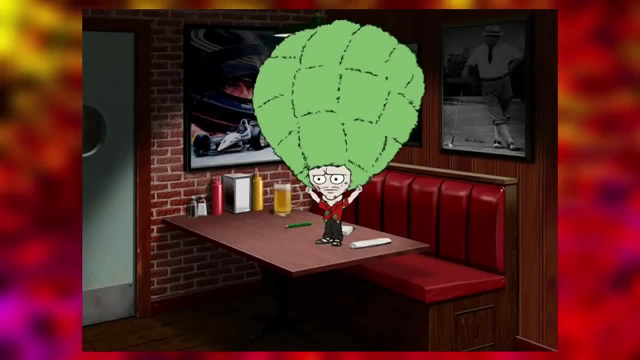 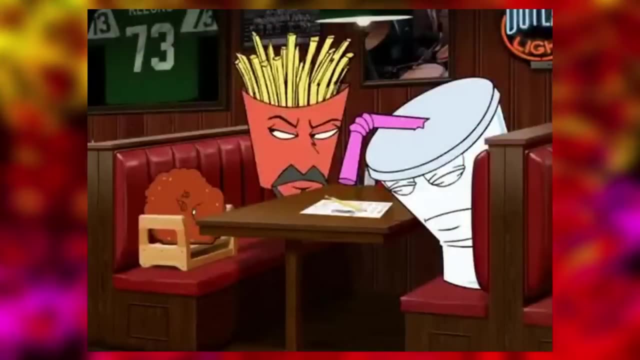 question which baseball player absolutely ruins the entire premise of Aqua Teen episode? Super Trivia: Biff Pocoroba. In Super Trivia, Frylock really wants to beat Wayne the Mainbrain by winning a trivia night and getting some bar bucks of his very own. and to accomplish this 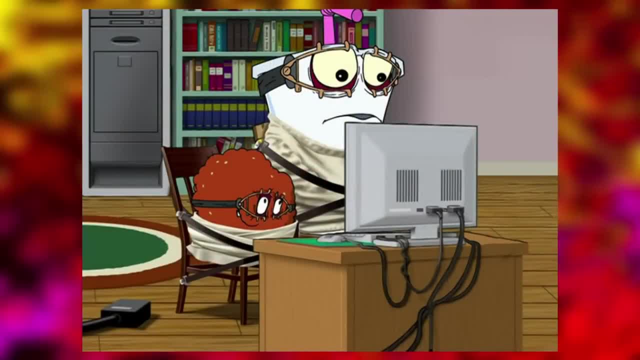 he ties up master shake and meatwad and forces them to watch all of the world's knowledge over the course of a week. but unfortunately, frylock, he forgot to put sports on the dvd. so what does he do? he brings carl to answer the sports questions. well, at the end of the night. in that 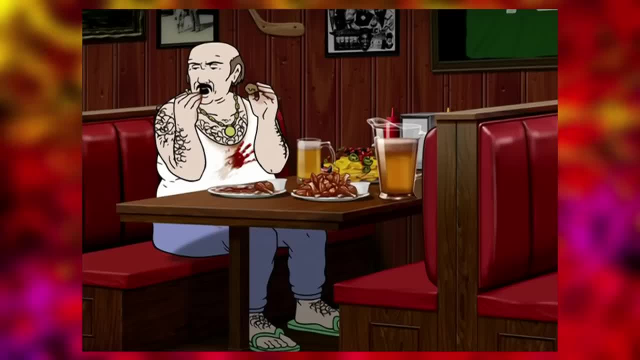 episode it's revealed: oh well, there were no sports questions. they brought carl for nothing. except, there are many points in that episode when we can see the answer sheet, and at one point we do see biff poka roba on there, which completely ruins the whole idea that there were no sports questions. 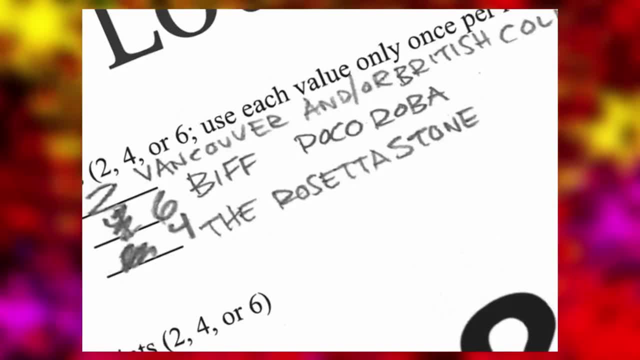 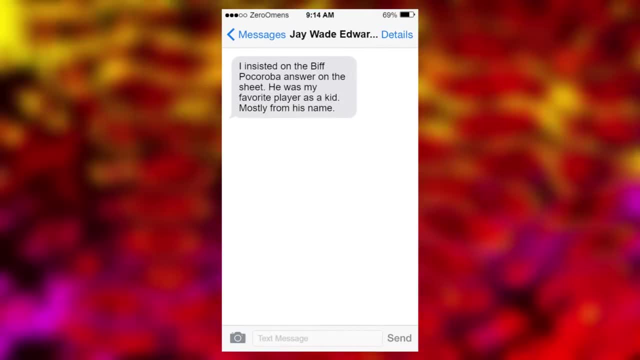 because we can clearly see that there were. when i asked jay wade edwards about this because i had heard that he helped create this trivia sheet, jay mentioned that he insisted on the biff poka roba answer on the sheet, as biff was one of jay's favorite players as a kid, mostly from his name. 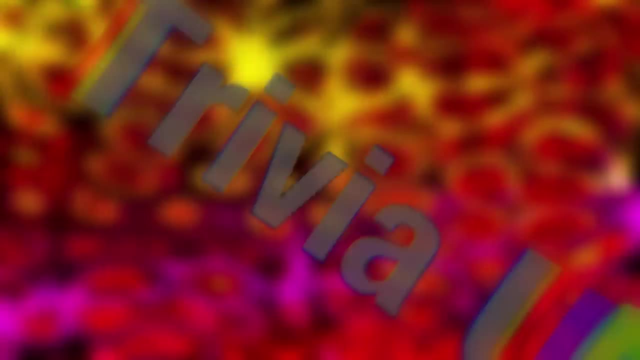 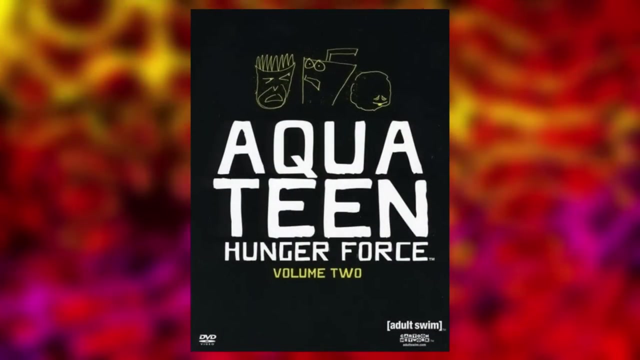 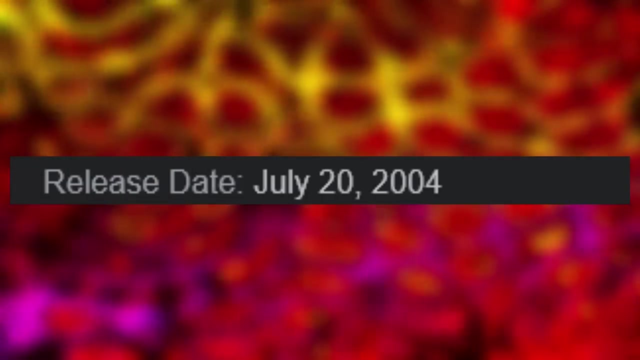 and you know what, jay, i can't blame you. ultimate golden trivia unit patrol squad. since we're talking about super trivia, let's talk about this little gem from the super trivia dvd commentary. now, the volume 2 dvd came out july 20th 2004, so we know that the commentary was recorded at some point before then in the 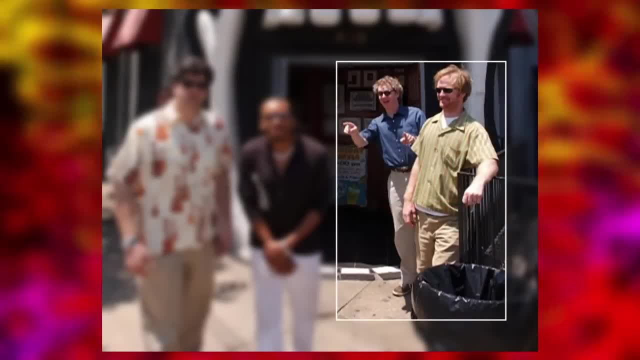 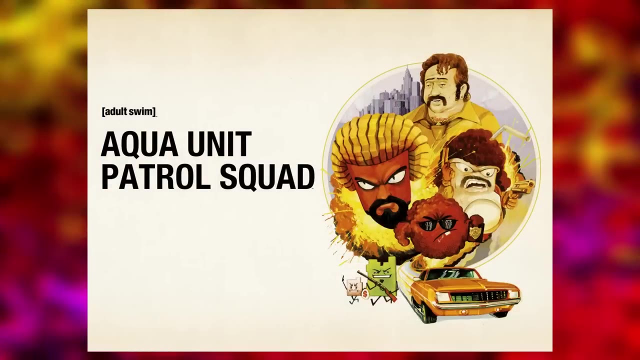 commentary, dave willis reveals that he and jay wade edwards did trivia under the name ultimate golden trivia unit patrol squad at one point. now, if that name sounds somewhat familiar, that's because the show later rebranded as aqua unit patrol squad one in 2011. so at least six years before the show rebranded dave, he had this idea. 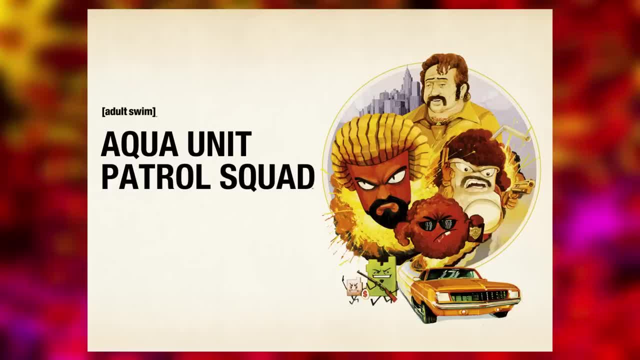 swimming around in his head. eventually it got out. actually, on the commentary, dave alludes to it being a short film idea as well. i wonder what that short film would have been. i guess i should ask him one of these days. total recal computer. in the end of the day, jay wade edwards said that he and jay wade 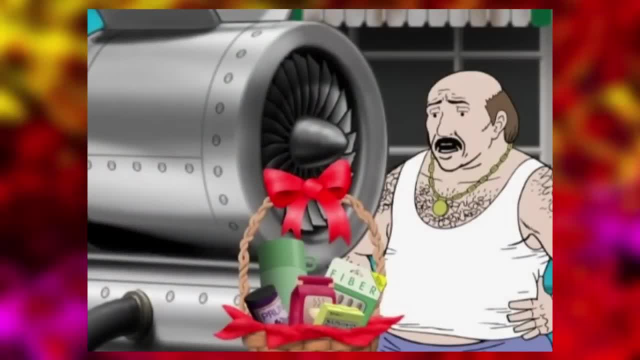 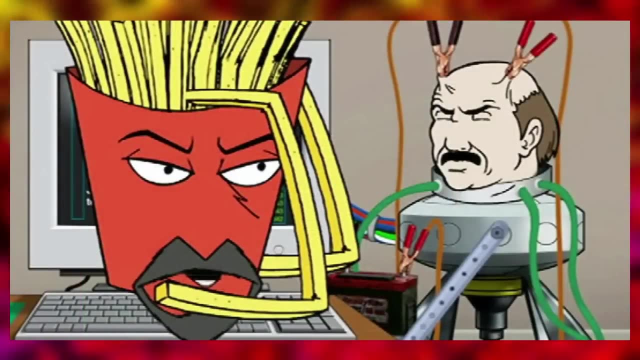 actually had a conversation about the super trivia unit in the first episode of the episode, total recal frilock accidentally killed carl with his super toilet. at one point frilock connects carl's detached head to frilock's computer where carl's brain waves can be read. meet wad comments on how? 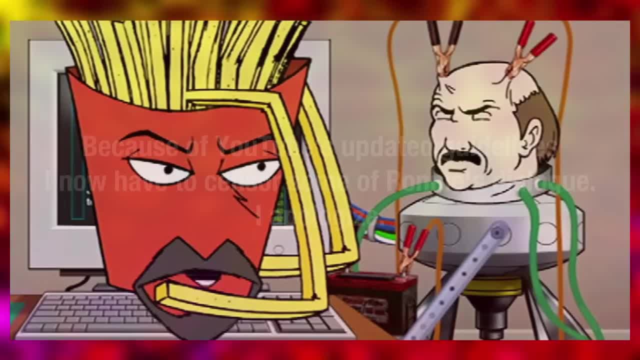 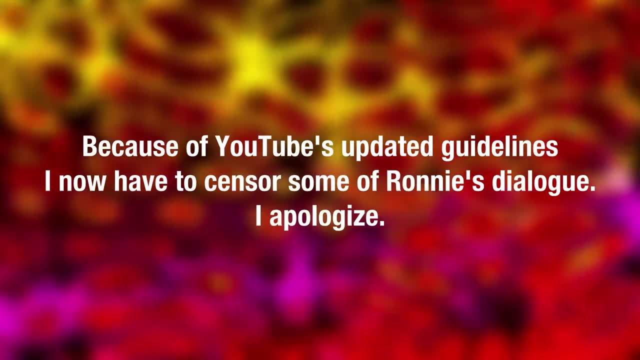 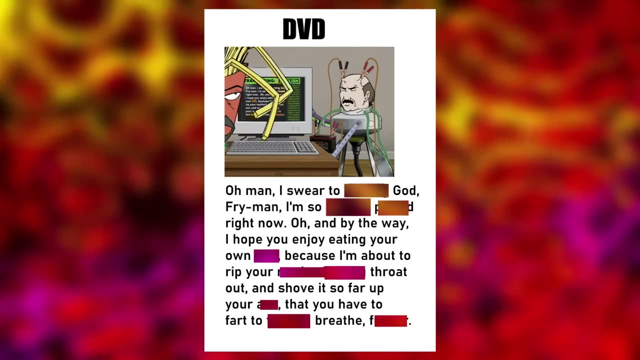 carl is dropping f-bombs, and he's correct. while you can never see the entire screen at once, you can pause at several times and figure out what carl is saying. i'll read you the uncensored text. oh man, i swear to god, fry man, i'm so right now. oh and, by the way, i'm so sorry, i'm so sorry, i'm so. 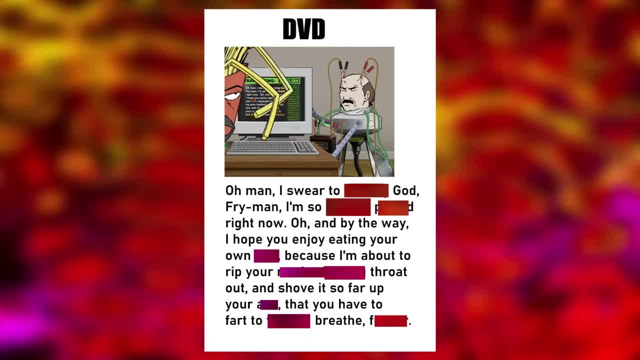 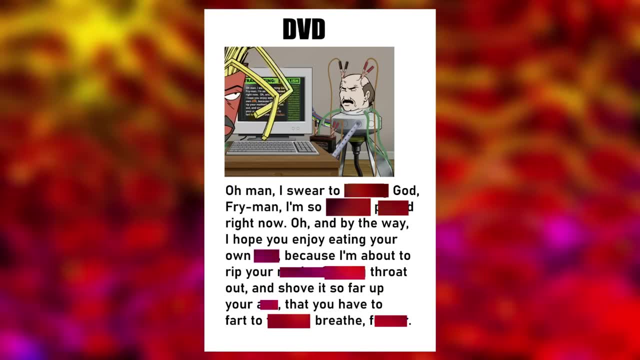 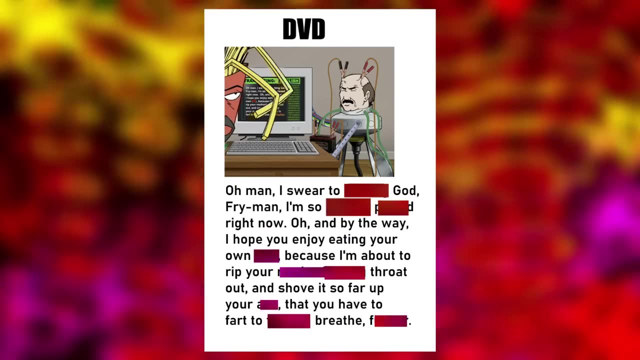 i hope you enjoy eating your own, because i'm about to rip your throat out and shove it so far up your that you have to fart to breathe. as a 10 year old kid, i have fond memories of sitting there for at least three minutes trying to pause my dvd player with a laggy remote, until i finally did it. 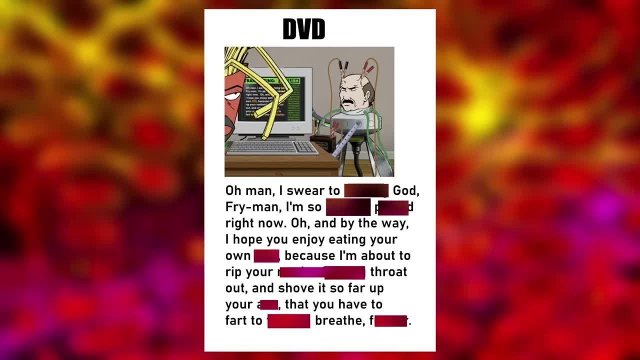 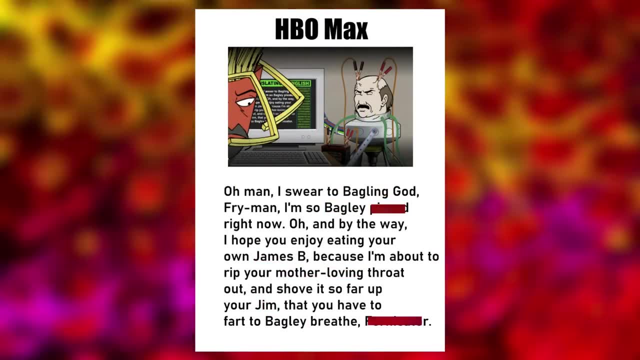 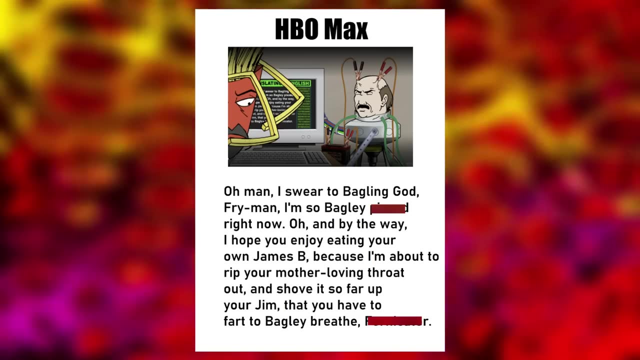 and i got to see the f-bombs. it was probably one of the top 10 moments of my life, easily. however, if you're a 10 year old kid now sitting on hbo max, you're gonna have a different experience. hbo max actually replaced the original text with edited text. the edited text reads: oh man, i swear. 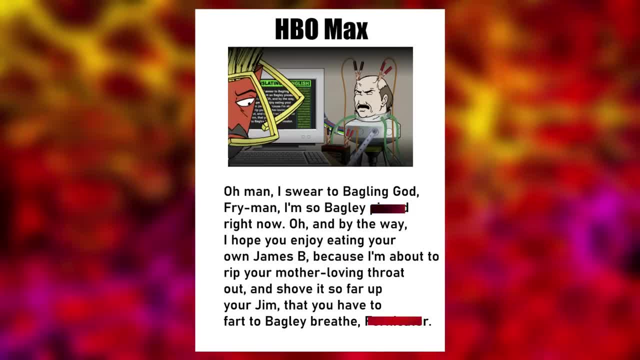 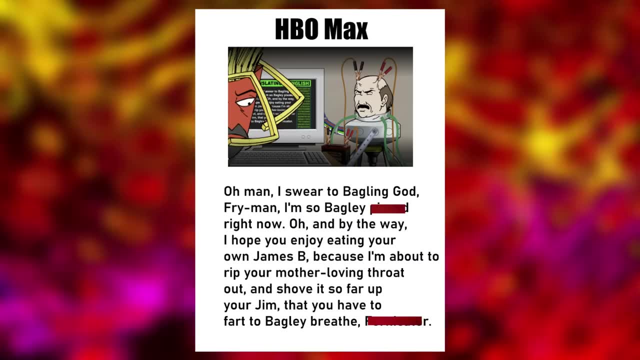 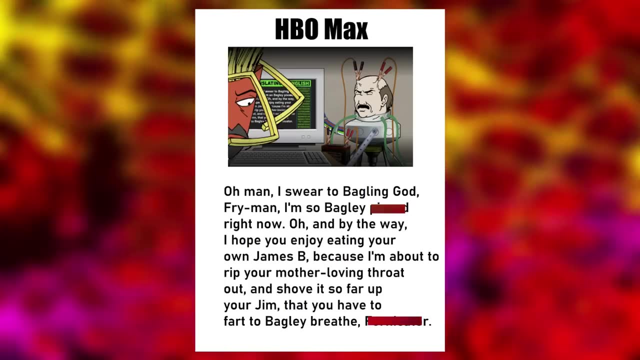 to bagling. god fry man, i'm so bagly right now. oh and, by the way, i hope you enjoy eating your own, james b, because i'm about to rip your mother loving throat out and shove it so far up your gym that you have to fart to bagly breathe. so yes, they replaced the text on the screen with 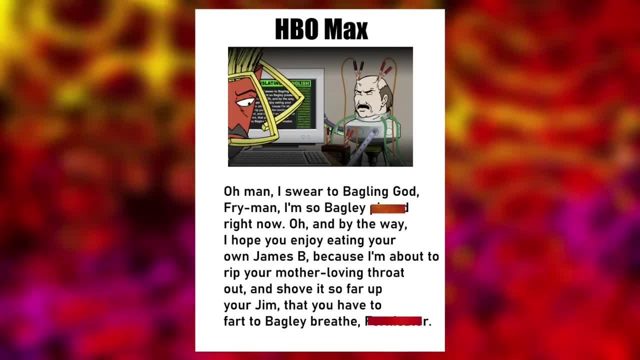 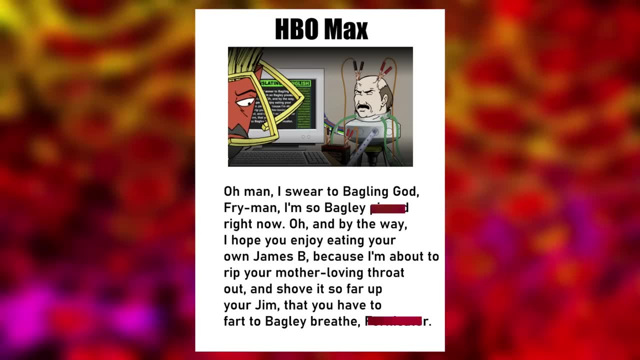 what i just read, which is so strange because you see it for like half a second and you have to pause it and and compile it together to try and figure out what's even being said. so i'm shocked that they went through and replaced this. i wondered. 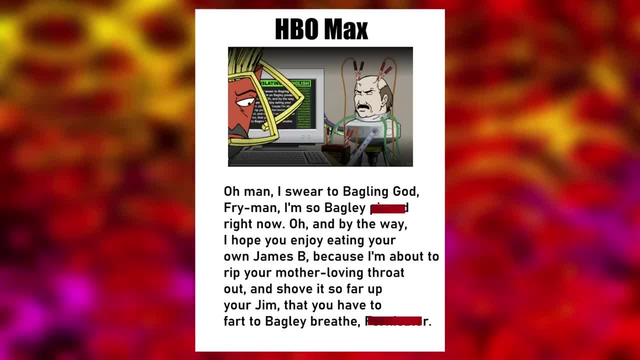 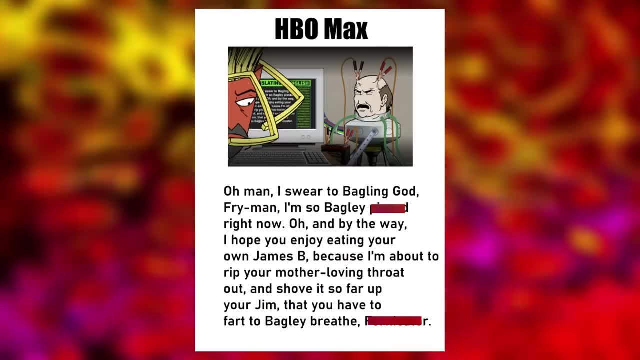 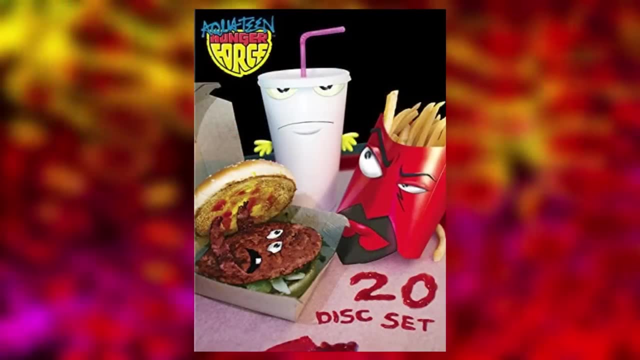 who wrote the new text- and i asked dave willis about this- he actually didn't even know that the text was changed, let alone who wrote the new copy. our last bit regarding this computer text change is: i checked the baffler meal disc and it is the uncensored version with the swear words, so you can. 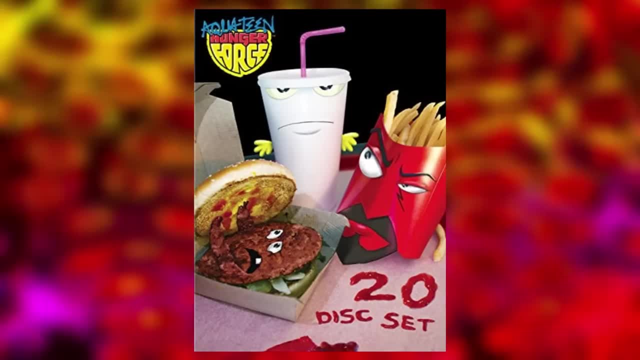 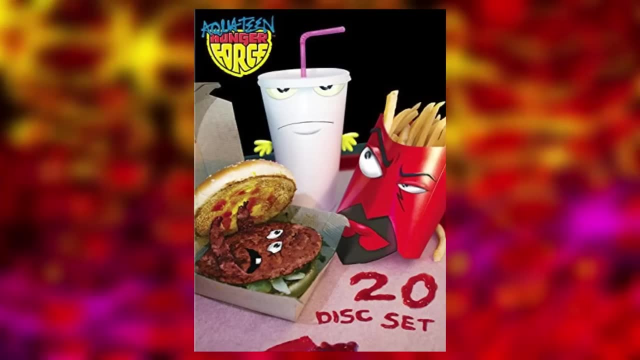 see it in the video and, yes, it has been super well hidden from the fans and i'll just give it a high five. this is the only one that comes out of the original version and it's a really interesting thing because, like i said, it's the only one that comes out of the original man youtube. 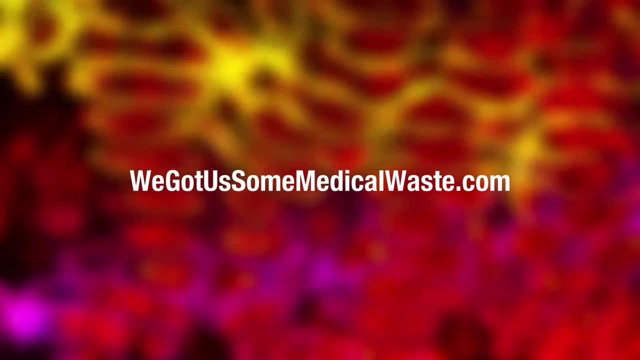 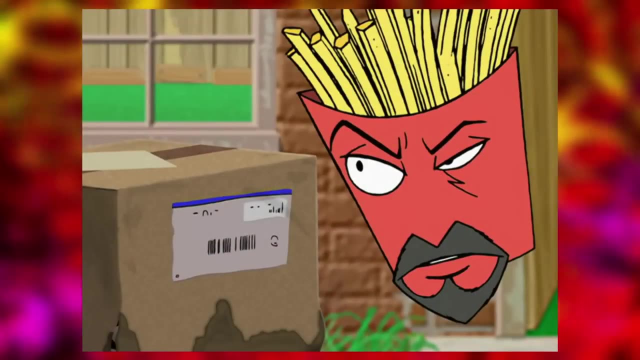 one, but it is a really interesting thing not to be confused with the original version, because the one on the back- that's the one that came out- was the one on the back of one of the videos. started out as a review of the original version that came out in 2022, but it's interesting because 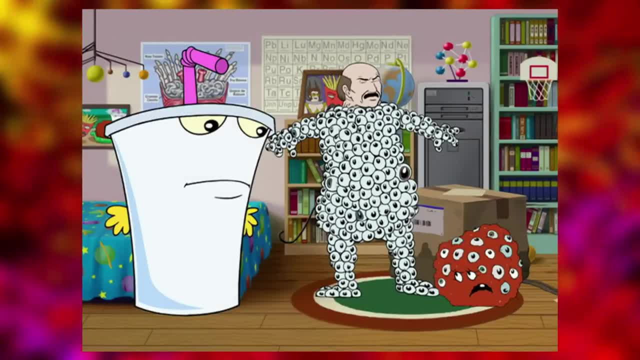 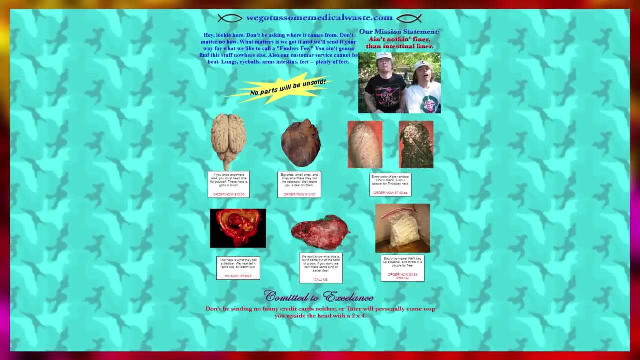 site. unfortunately, nothing happens. Someone bought the domain in 2018, and it's now inactive. However, from 2003 to 2018, this was a different story. Adult Swim originally bought the domain and an entire fake organ marketplace was set up. The page had a blue- camo background. 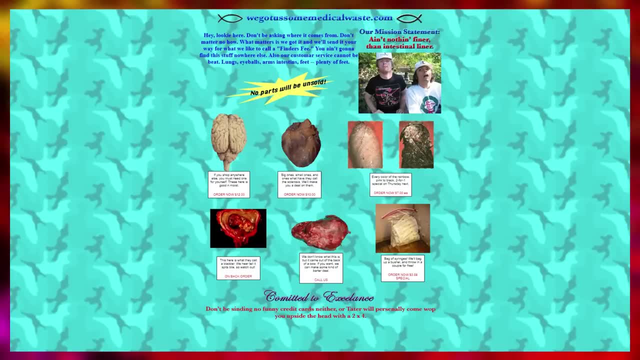 Jesus Fish, encompassing the site name and a picture of Dave Willis and production assistant Nick Nkatanawat making silly faces. And of course, there were lots of pictures of organs, fake descriptions, fake prices, the works, But beyond that, almost every element of the page. 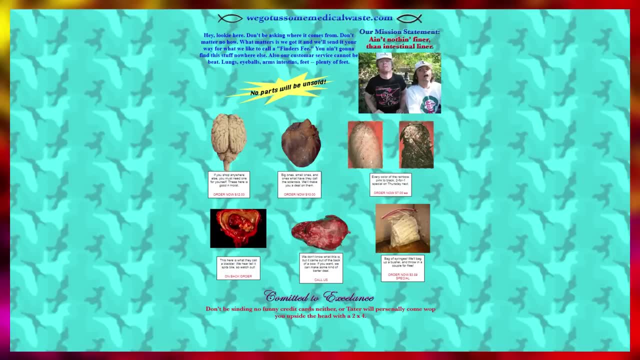 had an alternate text that you could see by inspecting the page elements. So, for example, on the photo of Dave and Nick it said owners and proprietors, with proprietors spelt wrong. Then it says: I done do this fancy newfangled web stuff. She done all the order, taking and sending. 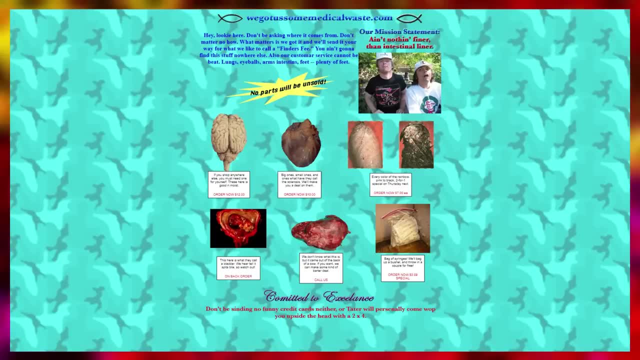 So you can see it was all kind of written in a southern kind of tone- Remember Aquatine made in the south- and the entire website is that way. Luckily you can still find this page on Wayback Machine because a lot of work was put into it, So I'm glad you can still. 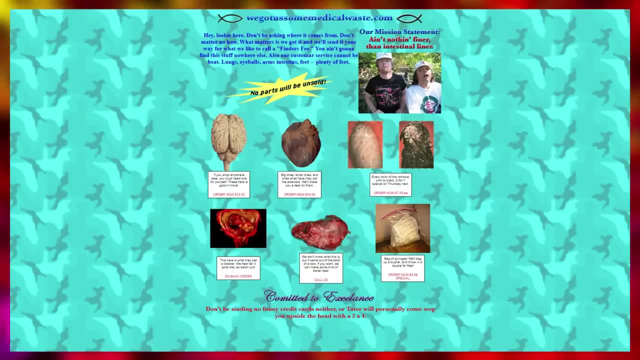 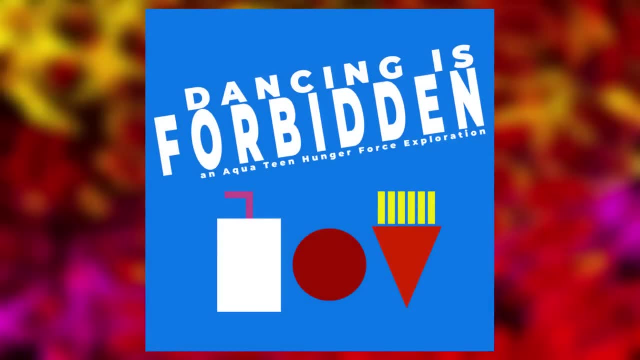 see it. Unfortunately, though, it doesn't work. You can't buy any organs on it, So please let me know down in the comments below where I should do all my future organ shopping. All right, that's it for me. Thanks so much to Zero Omens for letting me come on here and talk. 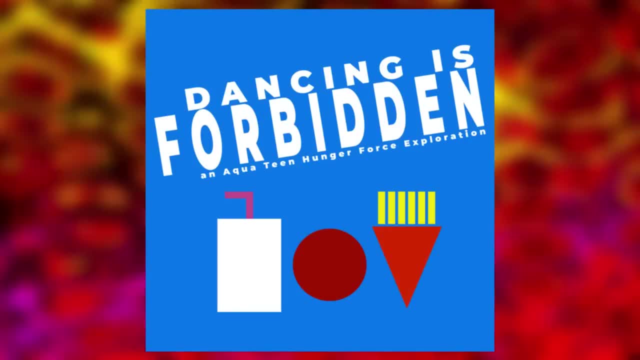 teens with you. And in case you're wondering: yes, Zero, Omens, he's a nice guy, not all the time. Only did he let me partake in this video, but he also taught me three new skateboard tricks for free. How about that? Again? my podcast is called. Dancing is Forbidden. You can find it at: 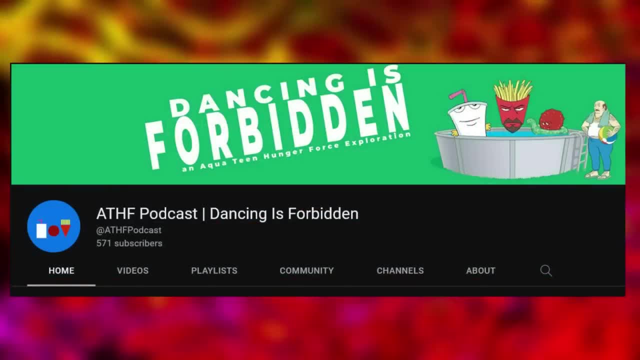 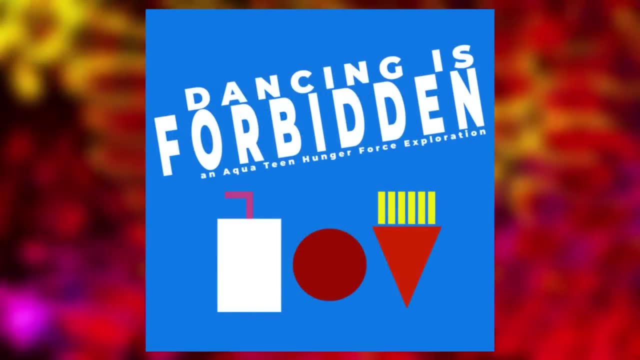 dancingisforbiddencom. Otherwise, it's on Apple Podcasts, Spotify, YouTube- anywhere you could find podcasts. It's there Every Monday. we're either diving through an episode of Aquatine, trying to find all the facts we possibly can about it, or I'm interviewing people from the show. 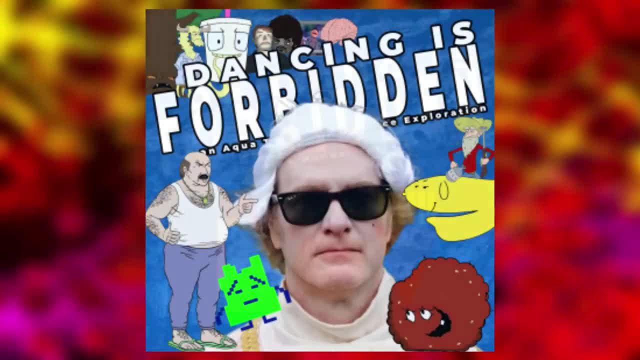 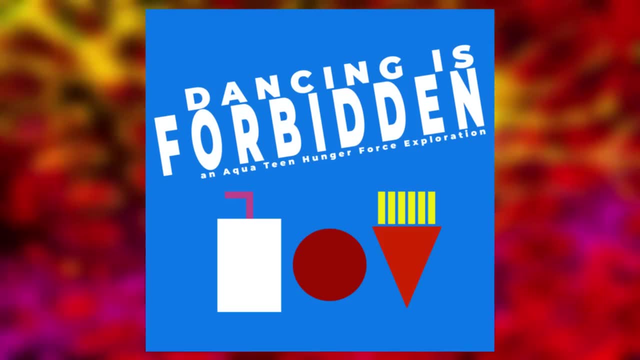 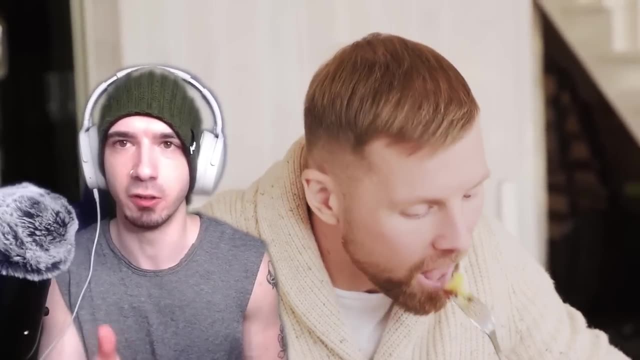 If you're watching this video this far, I suspect you might like it. Hope to see you there. In the meantime, prepare yourself, brace yourself for the seventh level of the iceberg. Hey, what's up? I'm back again. Just wanted to pop in one more time to let you guys know. 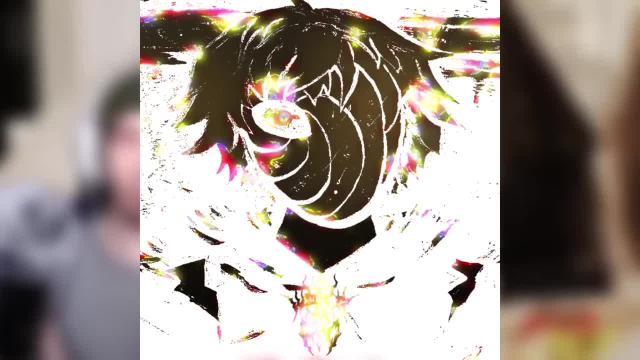 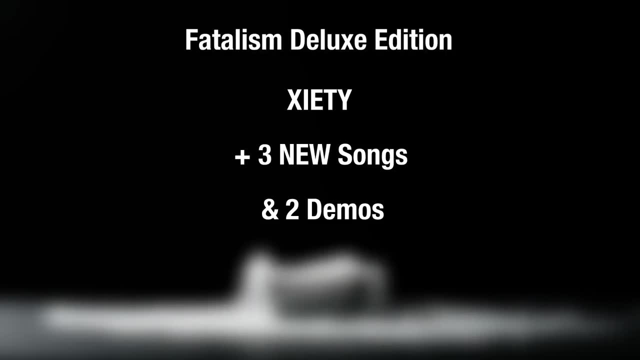 that my band Water On Red is putting out a deluxe edition of our album Fatalism on March 20th. The deluxe edition will include our single Anxiety, plus three brand new tracks and two demos, for a total of 19 songs. The standard edition of our album is called Fatalism and it's going to be. 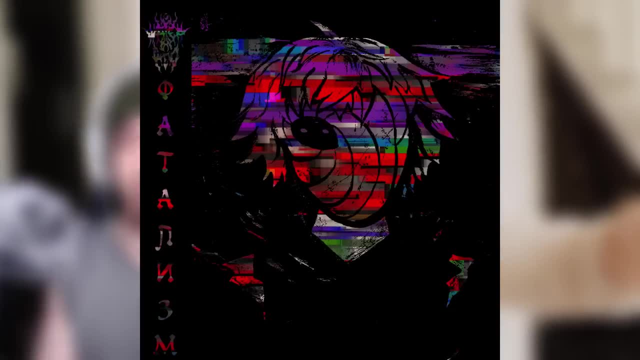 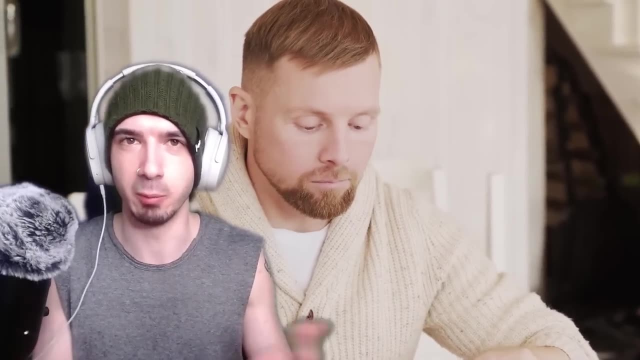 out on Spotify, Apple Music, Deezer and more. if you want to check it out, You can even check out the tracks on our YouTube page. No pressure, though, And if you don't vibe with our music, then no worries at all. Thank you for letting me plug my band, But without further ado. 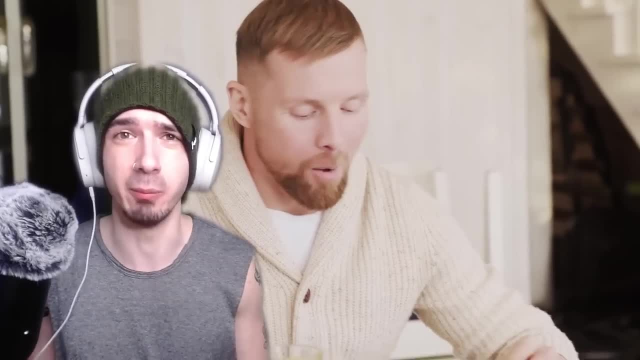 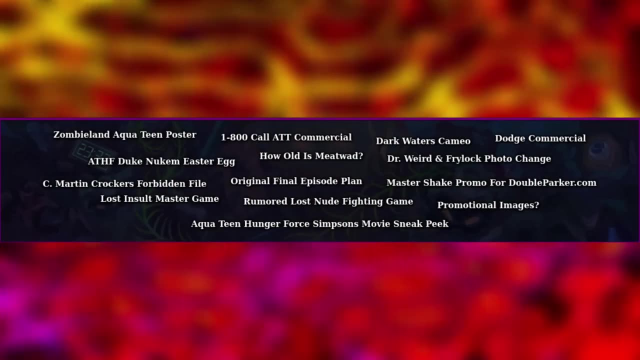 no more interruptions from here on out. It's time to get weird baby. Let's dive back into the rest of the iceberg. If anyone calls, we're off to the vet to get someone spayed, neutered and maybe, just maybe, if he's lucky- put to sleep. 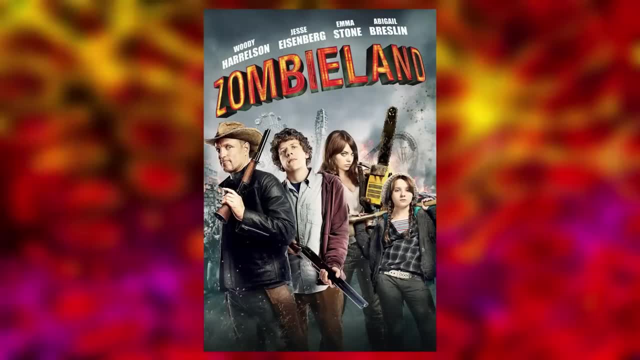 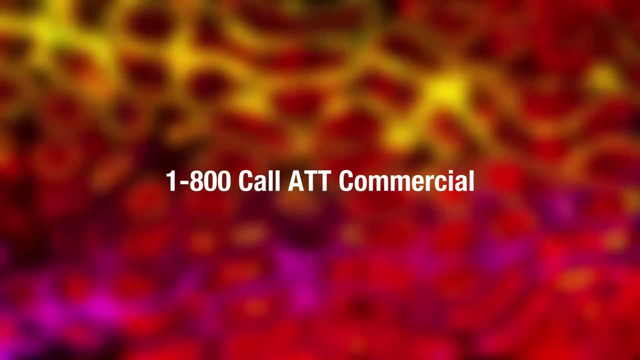 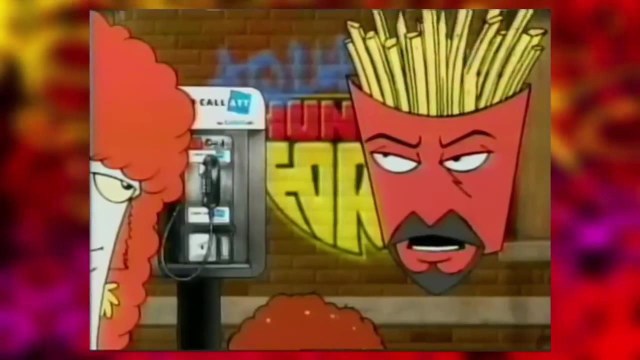 Zombieland Aquatine Poster. In the 2009 film Zombieland, an Aquatine Hunger Force poster can be seen by the door of Columbus's apartment 1-800-CALL-ATT-COMMERCIAL. In either 2001 or 2002, the Aquatines were featured on a. 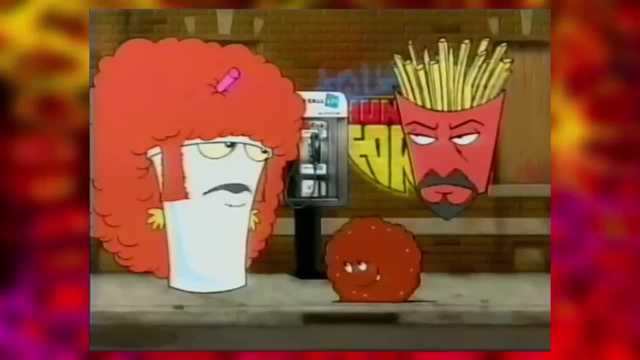 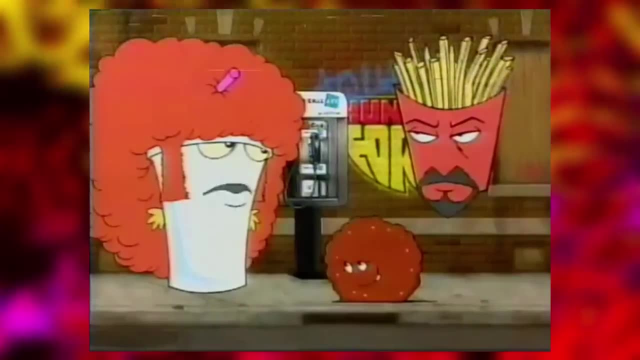 1-800-CALL-ATT-COMMERCIAL. In the advertisement, Shake is seen rocking some orange hair. Now, this hairstyle should look very familiar to a lot of you guys, and that's because it resembles comedian Carrot Top's hair, who was also featured on a Call-ATT commercial too. Oh yeah, and Shake. 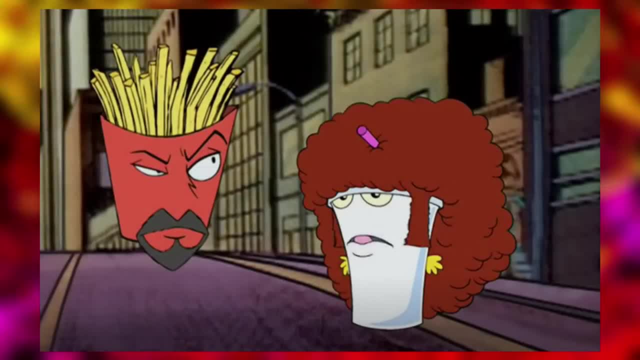 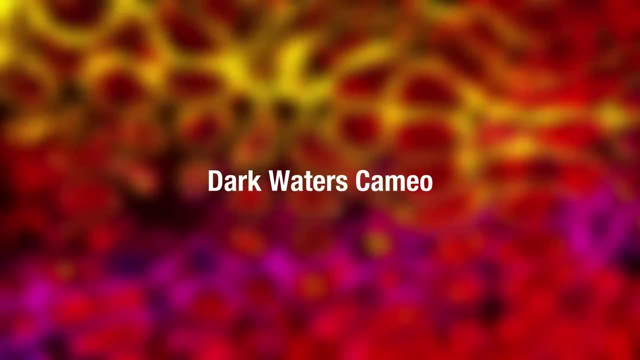 also had the exact same hairstyle in the episode, Rabot, except the shade of his hair in the episode was brown and not orange. Dark Waters Cameo. In the 2019 film Dark Waters, Mark Ruffalo's character is seen feeding his baby in the year. 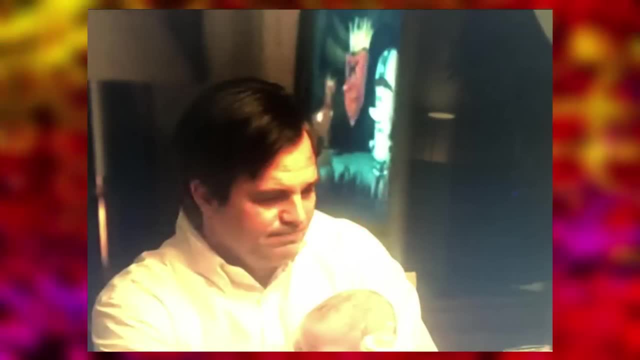 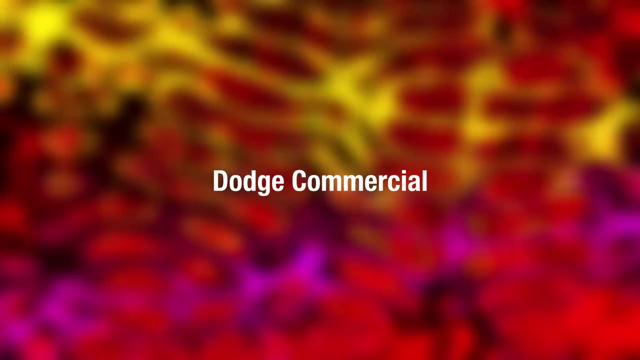 1998.. However, the cartoon playing behind him is a bit different. It's a bit different from the Aquatine Hunger Force, specifically episode 100, which came out in 2010.. Dodge Commercial. There is an old Dodge advertisement featuring two construction. 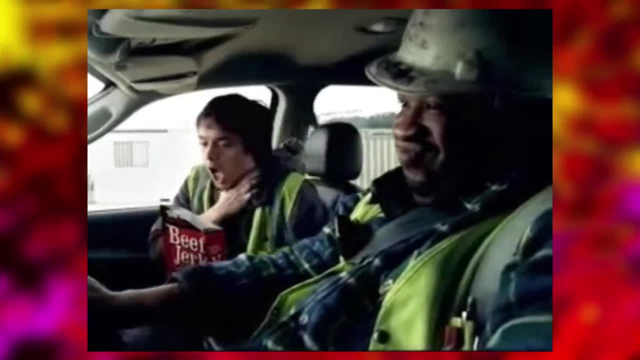 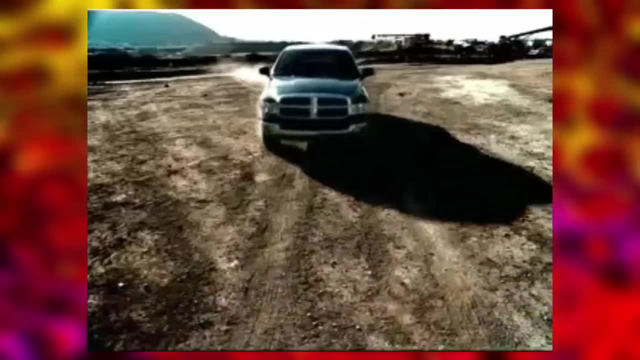 workers sitting inside of a brand new Dodge Ram. The passenger in the vehicle begins to choke on a piece of beef jerky and, instead of the driver performing the Heimlich maneuver, he takes a more responsible approach to helping his friend. The driver speeds down a dirt road as fast as lightning. 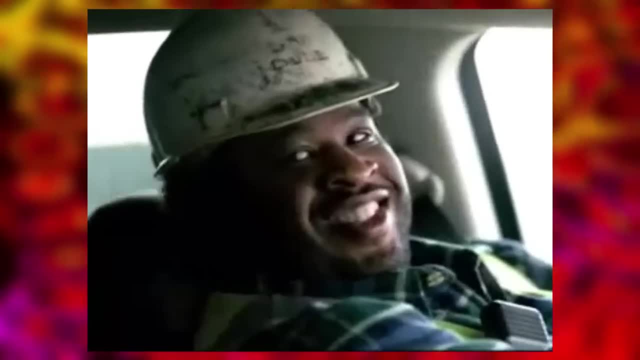 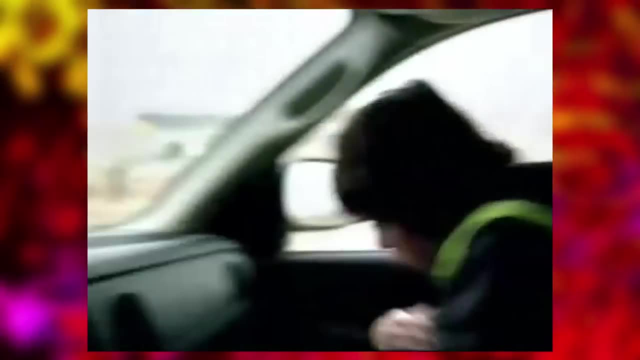 before stomping on the brakes, which results in the throat jerky from the passenger to be spat back up onto the windshield. The passenger lived to see another day and oh look, what's this? Is that Meatwad? What's he doing there? What's going on here? So some of you guys mentioned this commercial. 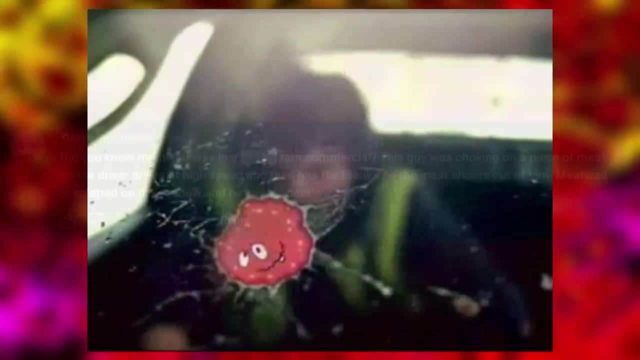 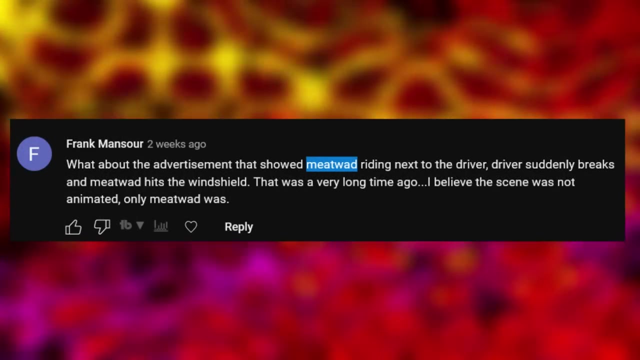 to me in the comments of my last Aquatine Iceberg video and I'll be totally honest, I don't remember seeing this ad growing up. This was a very interesting discovery for me. Shout out to all the comments on screen who told me about this commercial. Aquatine Hunger Force, Duke Nukem. 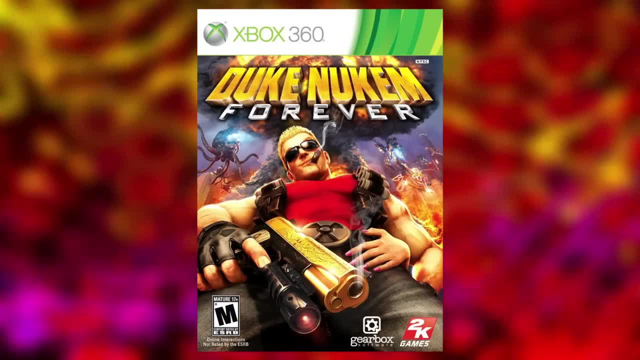 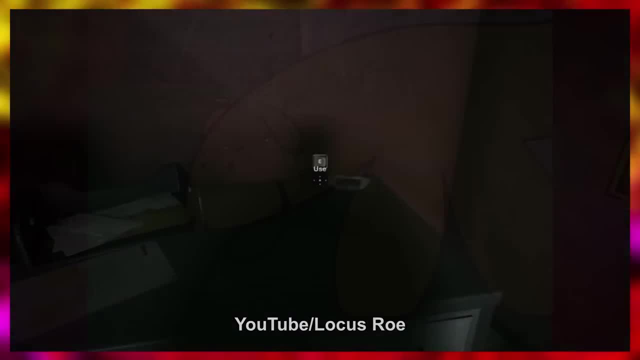 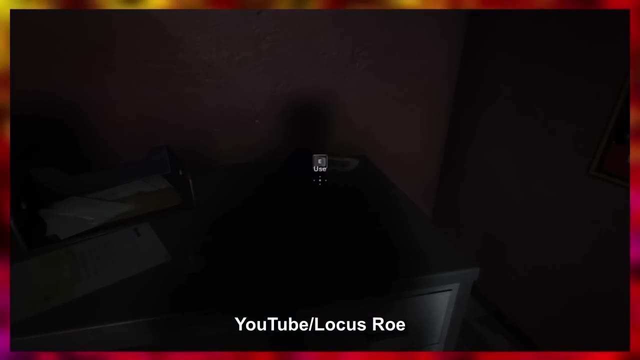 Easter Egg. There is an Aquatine Easter Egg in Duke Nukem Forever. If you listen to the message on the phone in the employee's office of the strip club, you'll hear a voice message that says: tonight, you, which is straight up, hand bananas. catchphrase. How old is Meatwad, So how? 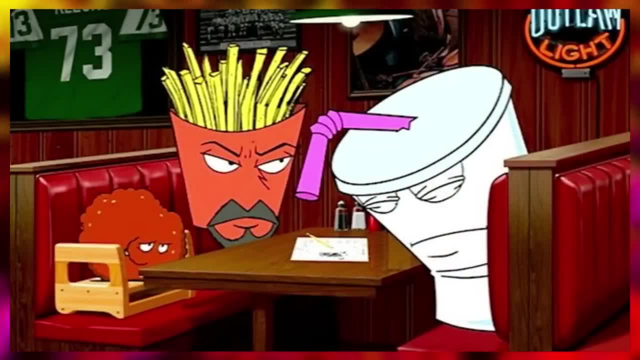 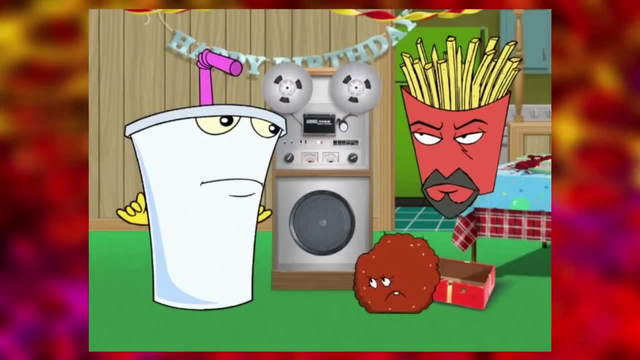 old is Meatwad Welp? nobody really knows. In the episode Super Trivia, Frylock tells Meatwad that he's not old enough to drink alcohol. In the episode Spirit Journey- Formation Anniversary- Meatwad states that he's 55.. In the episode Two and a Half, Star Wars at a Five or Pink Man, Meatwad says that he's 37. 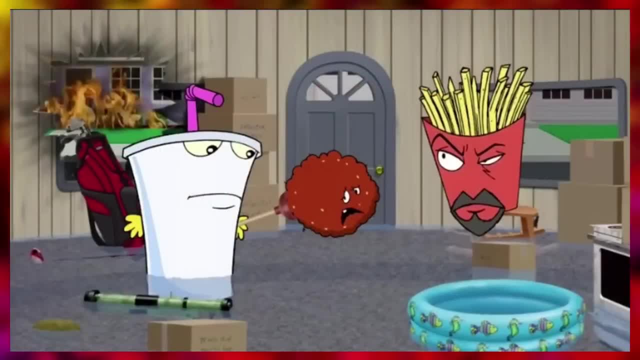 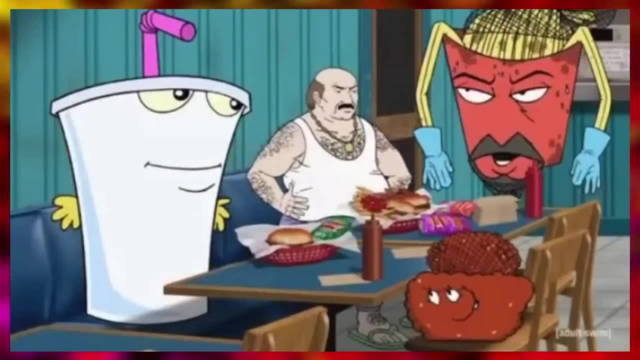 years old. In the episode Rabbah Redux, Meatwad states that he'll be 37 in July. In the episode Knapsack, Frylock says that Meatwad is 6.. And in the episode Working Stiffs, Frylock mentions that. 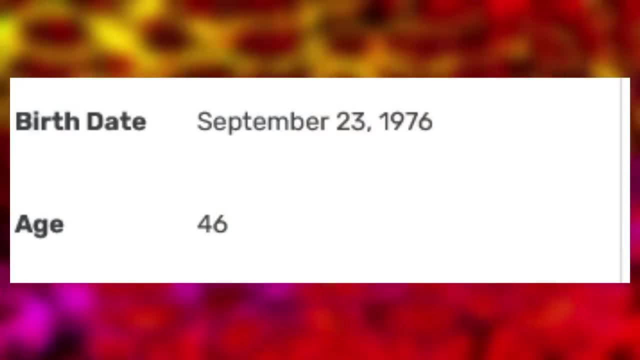 Meatwad has the mind of a 10-year-old And according to the Aquatine Wiki, Meatwad is 46. But if I had to make an educated guess, I'd say Meatwad is like 68 years old. 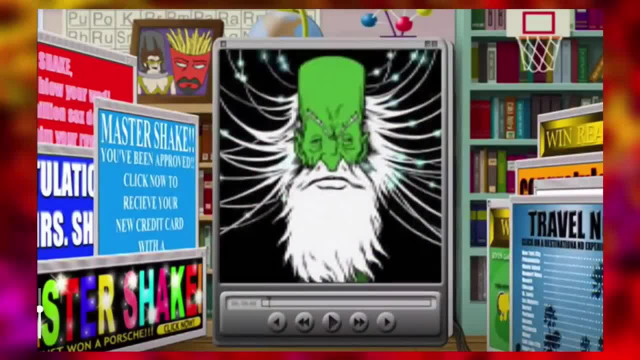 Dr Weird and Frylock photo change. So in the first three seasons of Aquatine there is a photo of a young Dr Weird standing beside Frylock on top of the bookshelf in Frylock's room. However, the photo only makes 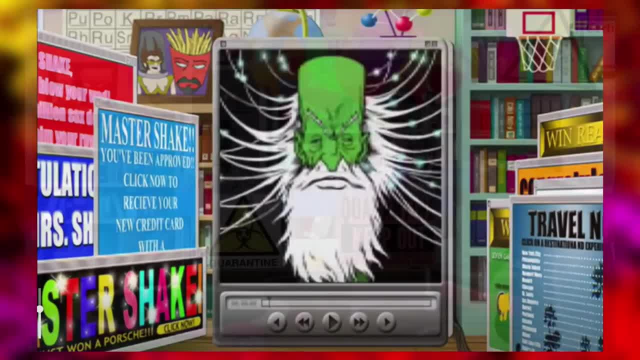 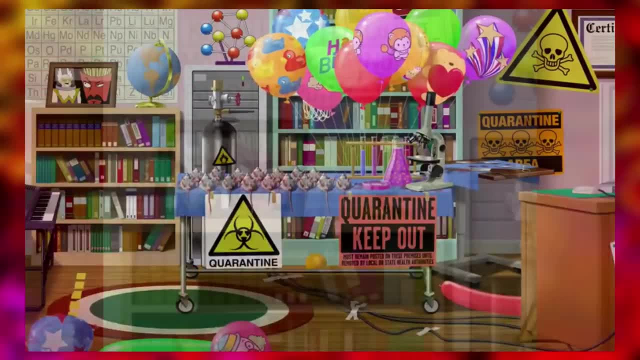 an appearance or two in season four before disappearing completely until the season six episode Dirt Inflatable Fuhrer. However, in that episode the photo is updated to show an older or I guess, modern Dr Weird standing next to Frylock. The updated photo makes another. 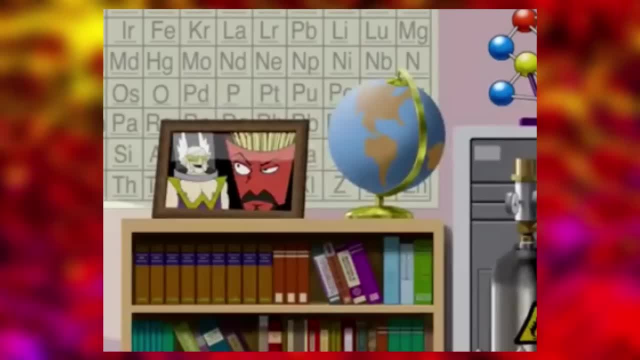 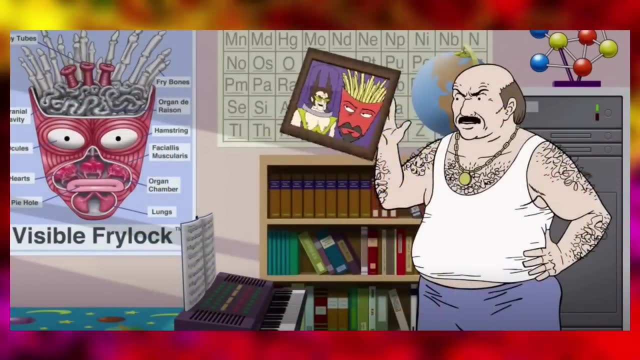 appearance in the episode Piranha Germs, before vanishing again until its final, final appearance in the episode Hospice. However, the version of the photo shown in that episode is the original. And just a quick disclaimer. I might be missing an episode or two, so please. 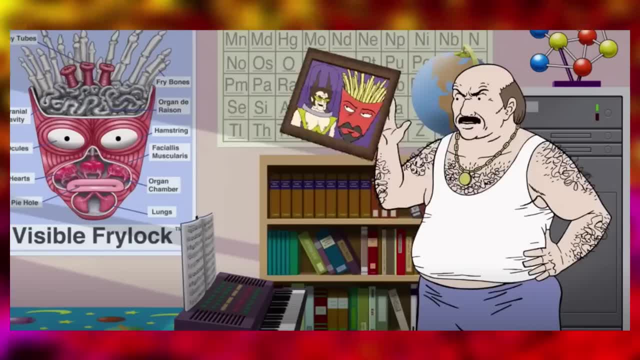 forgive me, I quickly skimmed through all 11 seasons the other day just to see which episodes featured the photo change. So what's up with the photos disappearing and being updated? What's going on with that? Well, I might have an explanation as to why the photo only appears. 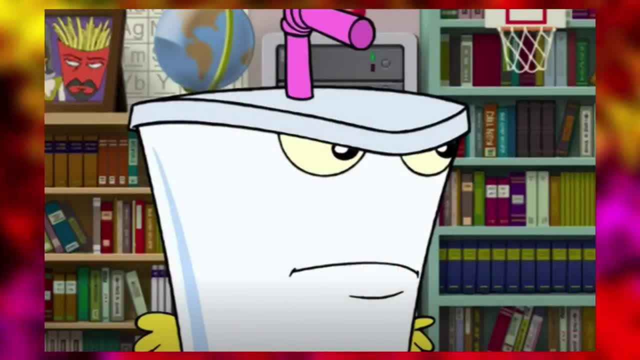 in like two episodes of season four before completely vanishing. So during production of Coal and Movie Film, all of the assets for the show are completely gone. So I'm not sure if that's the case, But the photo had to be recreated and those assets were also used for the series going. 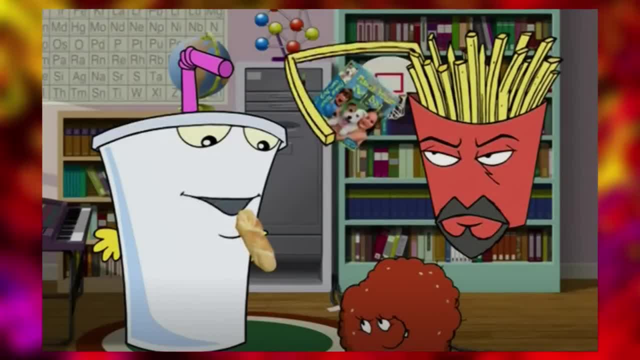 forward, And while developing the movie, the creators were also working on the series at the exact same time, So it's very possible that the episodes in season four featuring the photo were created before the updated assets were instated, But that doesn't really explain why there is a 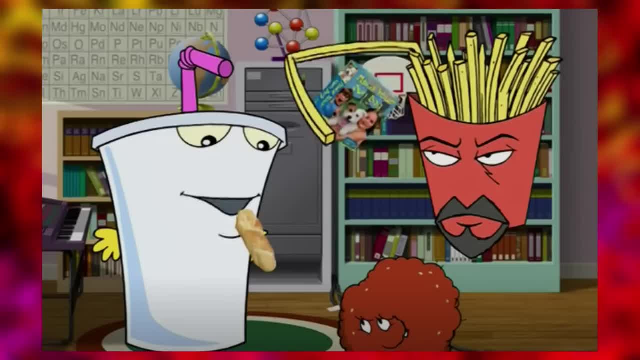 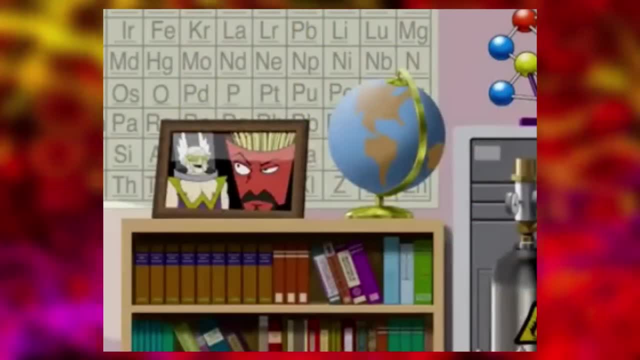 newer Dr Weird and Frylock photo in a couple of later episodes in the series, Unless of course the newer photo exists because Frylock and Dr Weird met face to face in Coal and somehow during their crazy family reunion. And if that's the case, then that's a rare moment of continuity. But I doubt it because if that were, 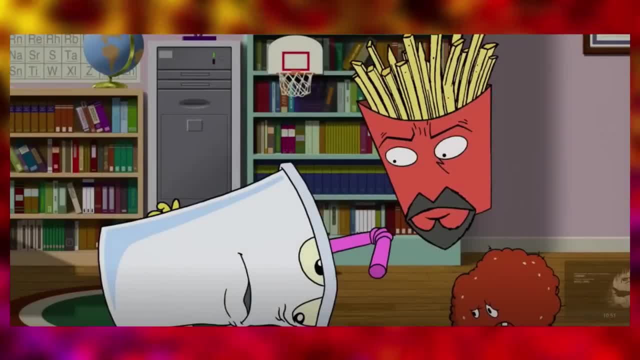 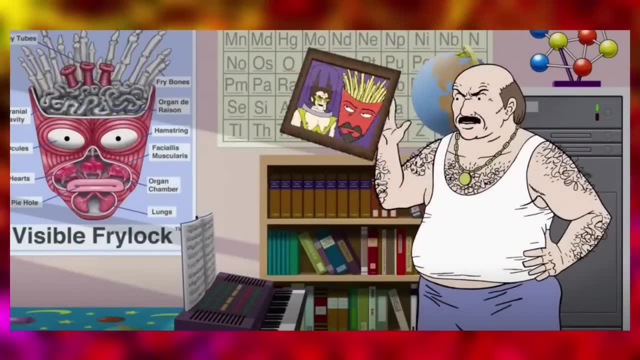 the case, the newer photo would be in the background of every episode post Coal and Movie Film. But then why is the original photo seen in Hospice? Where's the new photo? It just doesn't make any sense. So I've come to some conclusions. Either there's a real purpose behind this photo change, or Matt, or 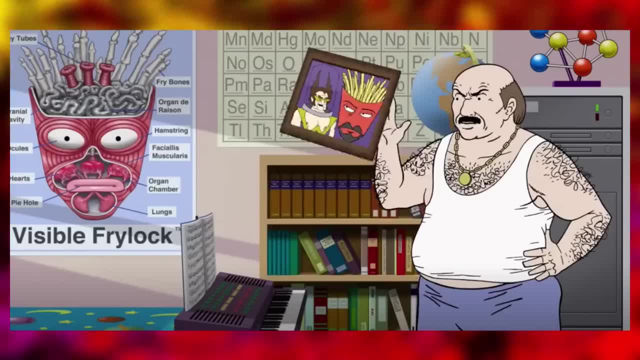 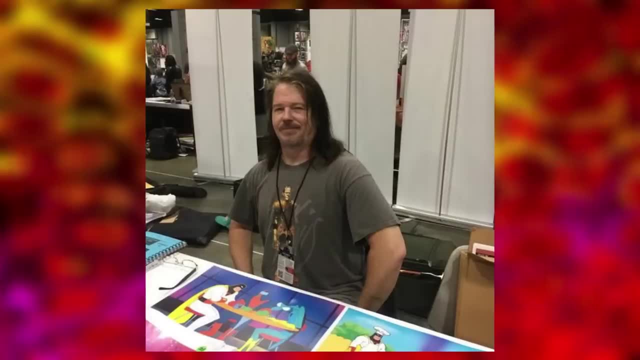 Dave or someone did this to mess with the fans And, if you want my two cents, we're probably being debated Clay Martin Crocker's Forbidden File. So I talked about this entry in my Adult Swim Iceberg before, but it doesn't hurt to talk about it again. Clay Martin Crocker could sound like a familiar name. 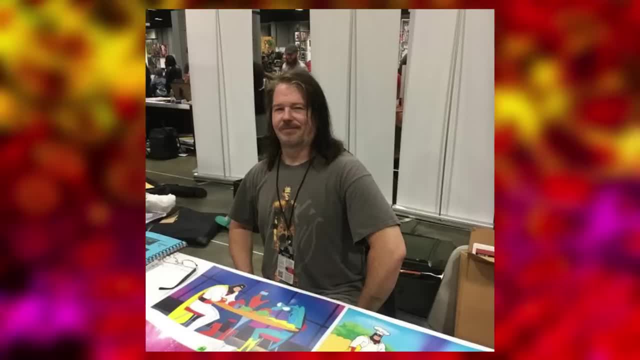 to all of you, And that's because he was the voice of Dr Weird and Steve on Aqua Teen. He was an animator for the series as well. He also voiced Multar on Toonami back in the late 90s and also. 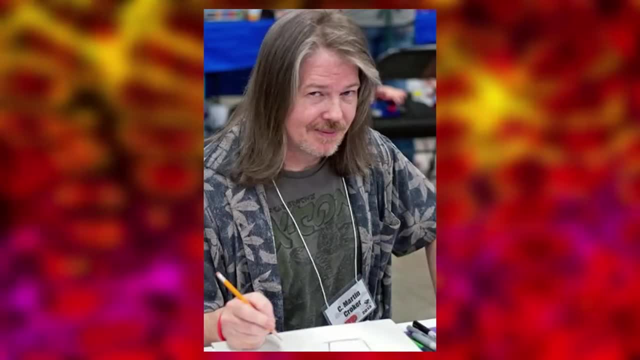 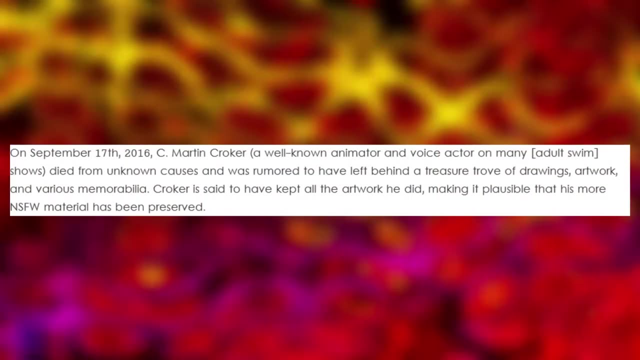 Zorak on Coast to Coast and The Brack Show. Now, sadly, Crocker passed away back in 2016 at the age of 54. But there is a rumor that Crocker left behind a treasure trove of Dr Weird and Frylock. 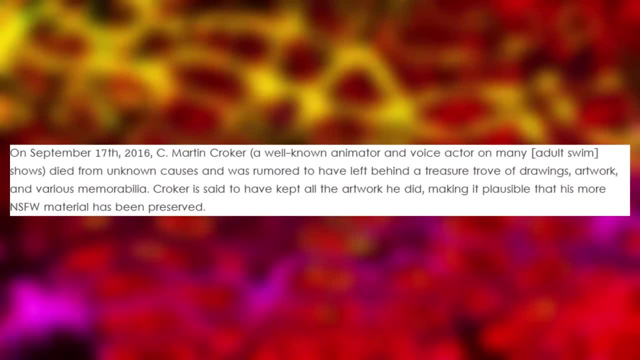 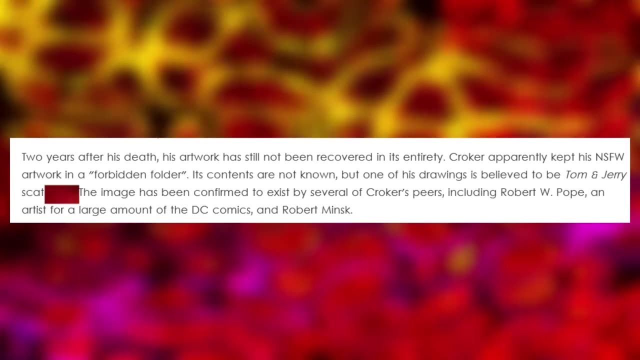 drawings, artwork and various memorabilia. It's said that Crocker kept all of the artwork he created, making it plausible that his more NSFW material has been preserved. Yes, you heard me correctly: His dirty, dirty, naughty, naughty sketches. Two years after Crocker's passing. 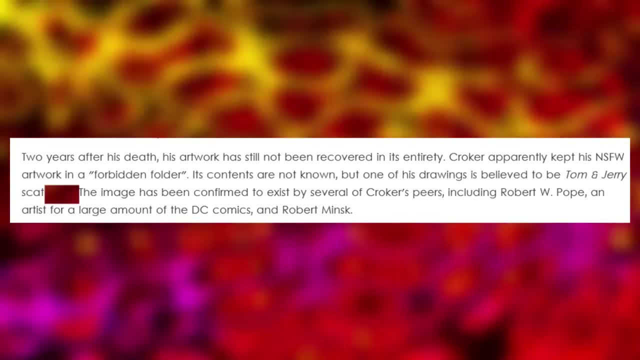 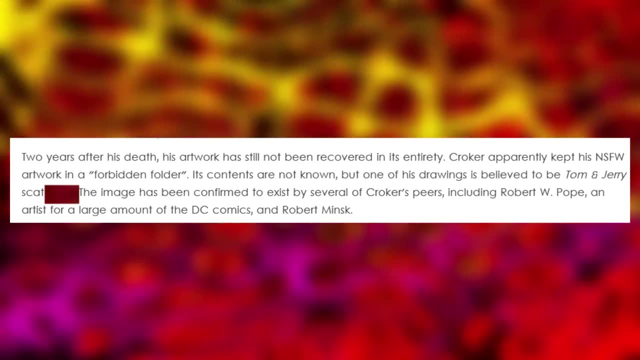 so around 2018, Crocker's work has still not been recovered in its entirety. Apparently, he kept his NSFW artwork in a forbidden folder. Its contents are not known, but one of his drawings is believed to be Tom and Jerry's. 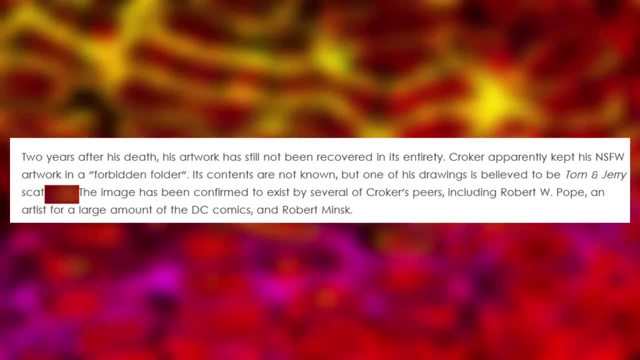 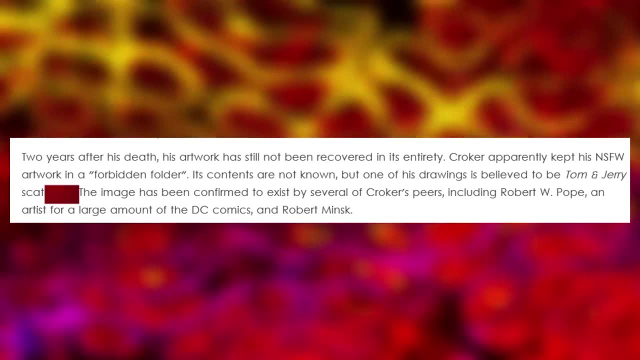 followed by a word that rhymes with corn. The image has been confirmed to exist by several of Crocker's peers, including Robert W Pope, an artist for a large amount of the DC Comics, and Robert Minsk. Preservation efforts for the forbidden file was led by Crocker's sister. 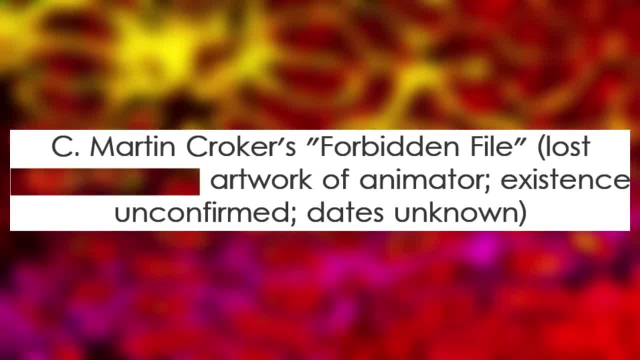 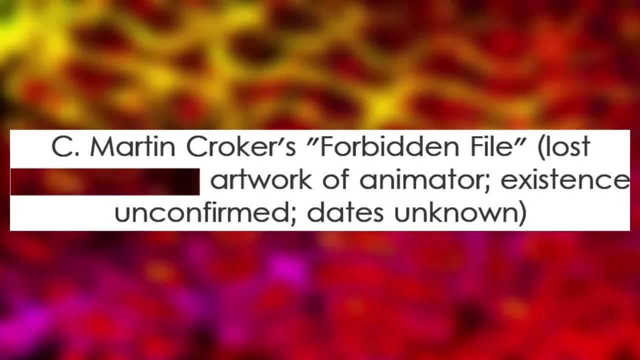 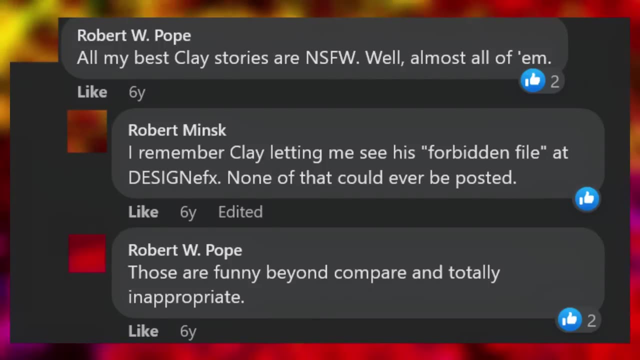 Julia Thornton. Now, all of this information is coming from LostMediaWikicom, but I do want to state that this file isn't really lost. media Crocker's forbidden file is just a rumor and its existence is a mystery. However, Robert Pope, who I mentioned before, had acknowledged the existence of the file. 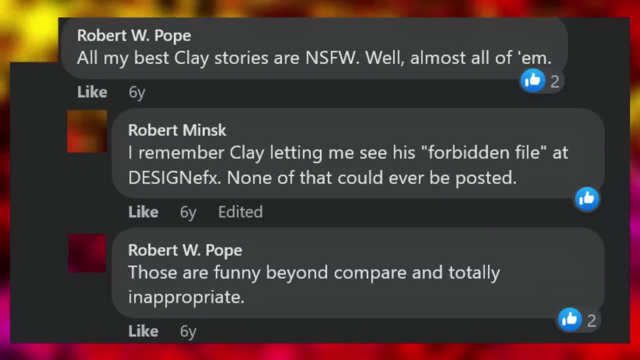 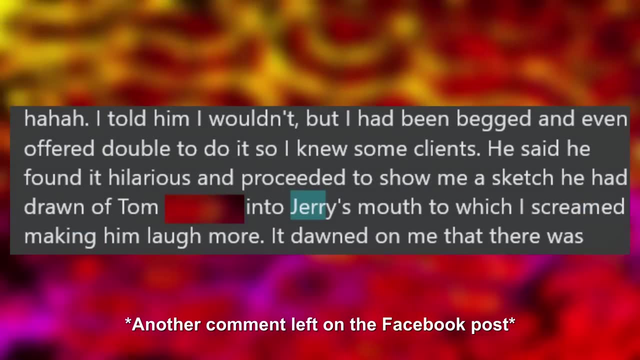 in a Facebook comments section from a couple years ago about a post asking for funny Crocker stories. So from my perspective it seems like the file is likely to be real, but nobody has fully uncovered it just yet. It sounds to me like Crocker had just shown his close friends. 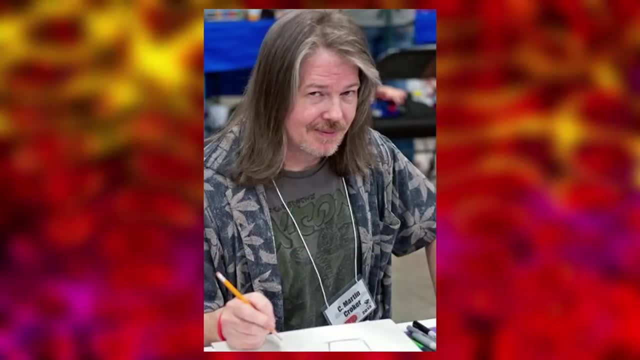 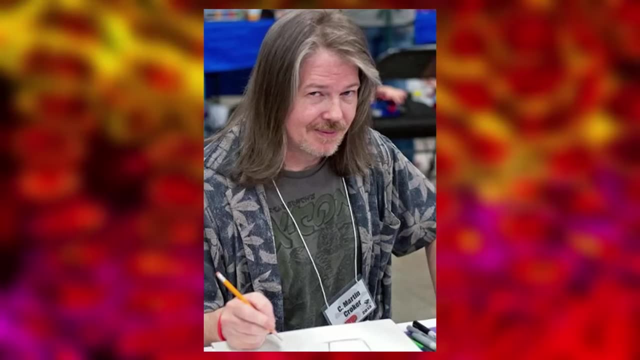 bits and pieces of his dirty art stored in this forbidden file, but kept its location hidden. So allegedly somewhere on this planet there is a folder with a ton of dirty, crazy art, and lord have mercy. if it's real, we need to find. 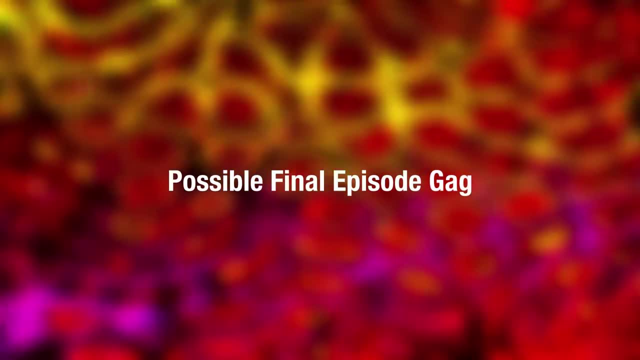 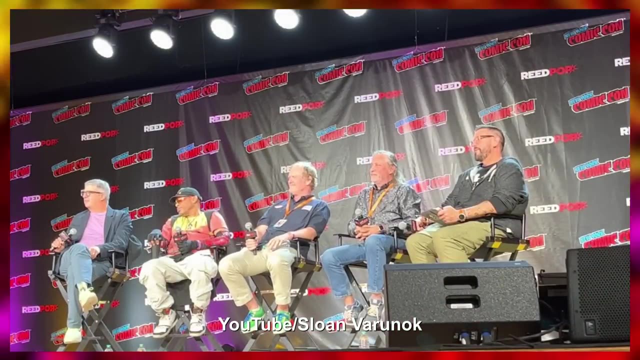 it Possible Final Episode Gag. An Aqua Teen fan at the Plantasm premiere at New York Comic Con 2022 asked the Aqua Teen cast why they decided to troll the audience by marketing the last one, forever and ever, as the final episode, before silently airing the greatest story ever told. 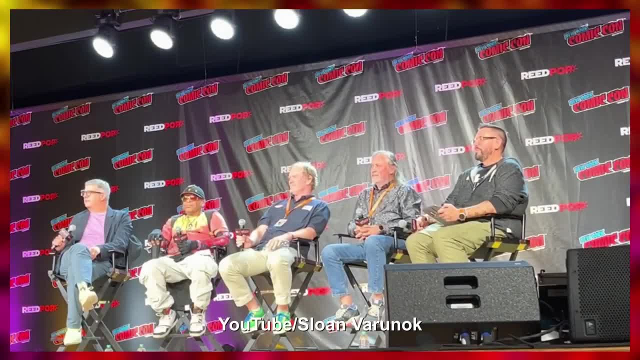 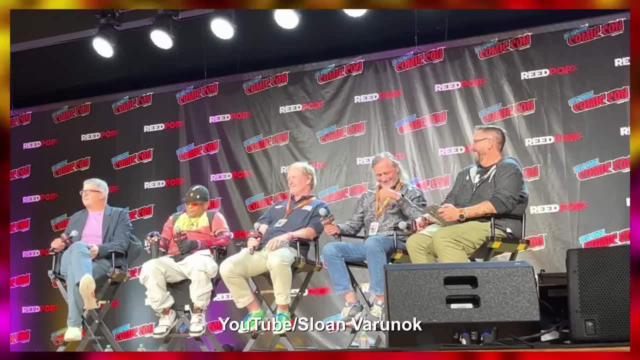 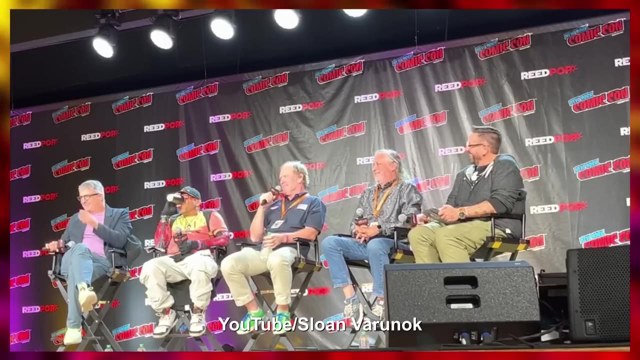 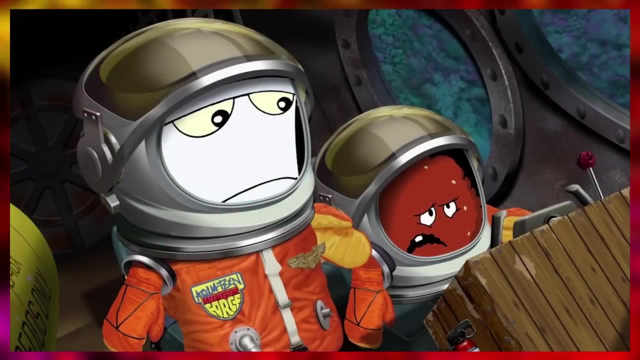 without any promotion, And Dave Willis responded with: It's possible that Dave was joking here, but maybe he was serious. Either way, that would have been hilarious if Adult Swim continued to air new episodes of Aqua Teen after the greatest story ever told for like a couple more weeks, just to really screw with people. 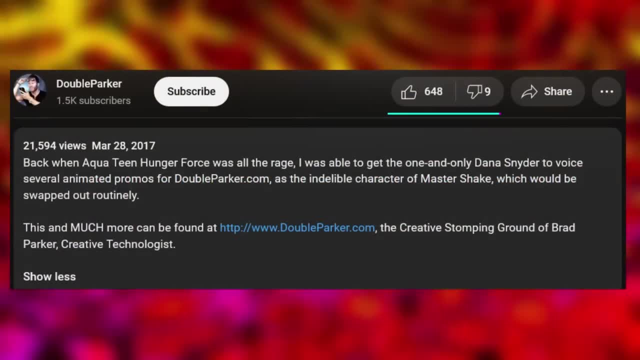 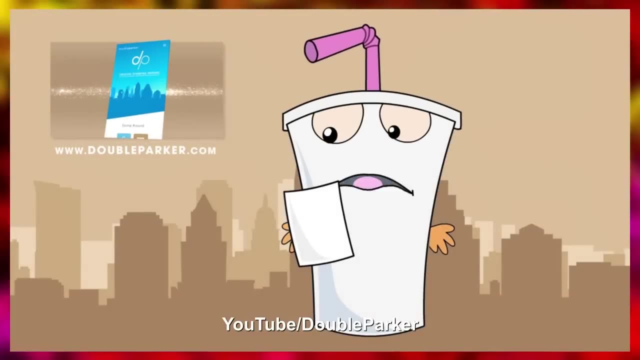 Master Shake Promo for DoubleParkercom. Double Parker is a recreational project run by a man named Brad Parker and according to him, he managed to get Dana Snyder to voice several animated promos for his website as Master Shake, And on screen is one of them uploaded to: 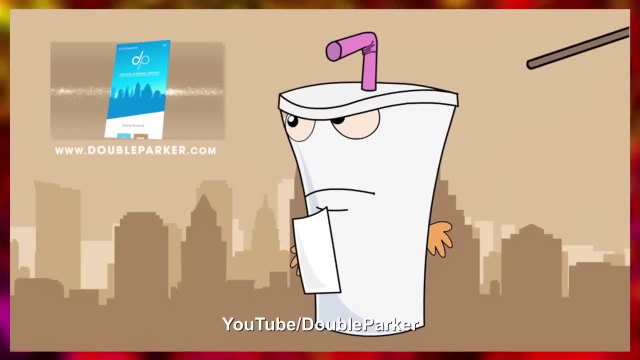 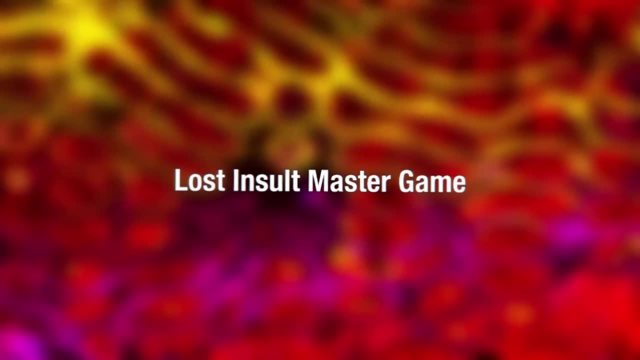 YouTube. Although you could easily tell that this Master Shake is an imposter because the real Shake doesn't know how to read, I am not reading this. It sucks Lost, Insult Master Shake. But this is not an Insult Master game. 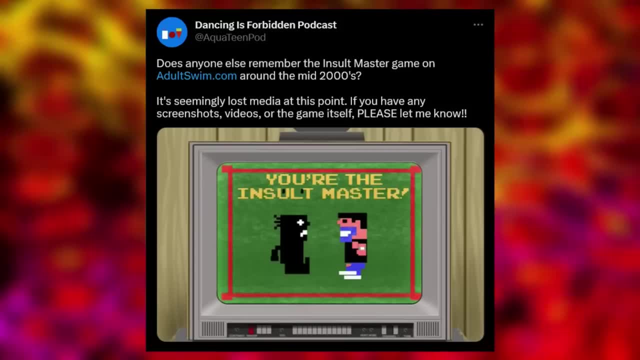 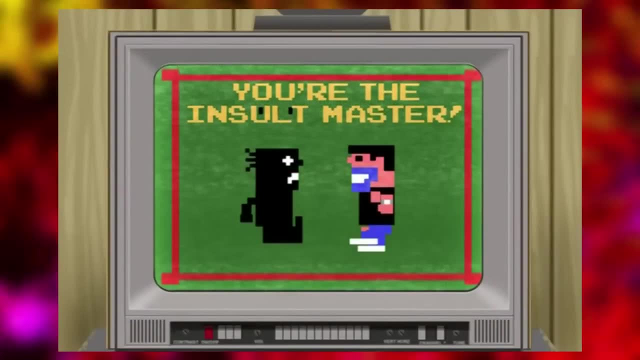 So Ronnie tweeted a couple weeks ago about an old Adult Swim Aqua Teen game called Insult Master, which was based on the Insult Master that we see Mithwaad playing in the episode video WeeGee, And apparently it's a piece of lost media. so I'm mentioning this in my video because I want. 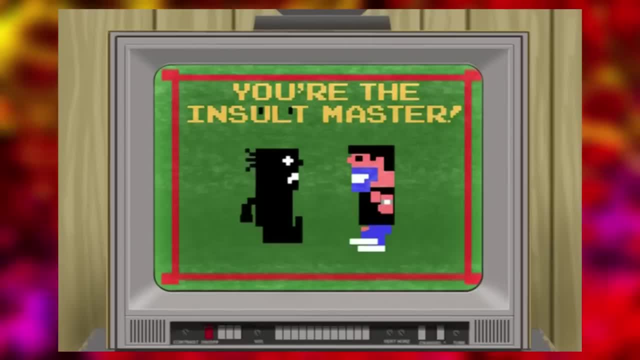 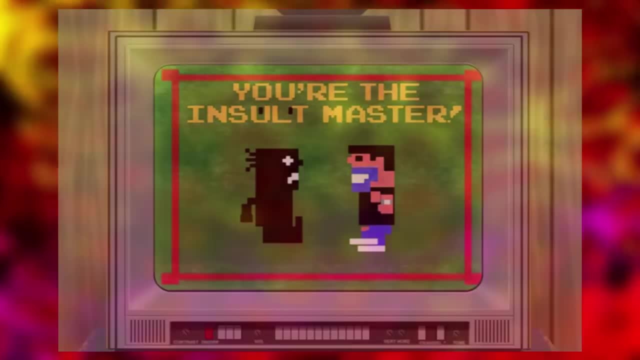 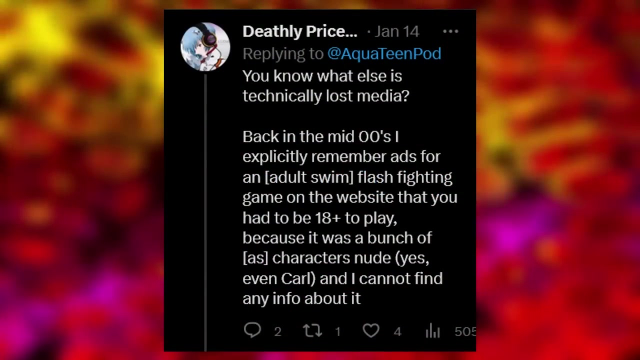 to bring awareness to this lost game. If anyone watching this has any screenshots, videos or has even managed to archive the game itself, then please let us know in the comments. Rumored Lost Nude Funnel Comment. According to Twitter user Deathly underscore Price in the comments of Ronnie's tweet regarding the Lost Insults Master Game. 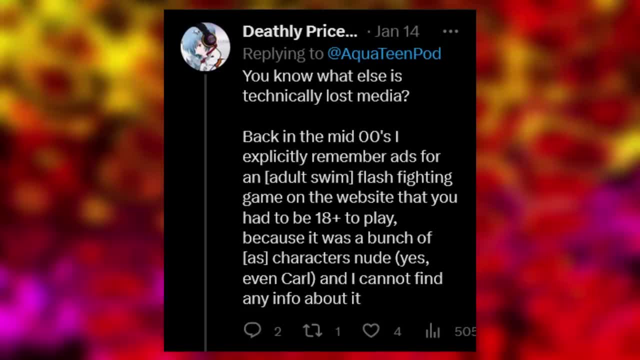 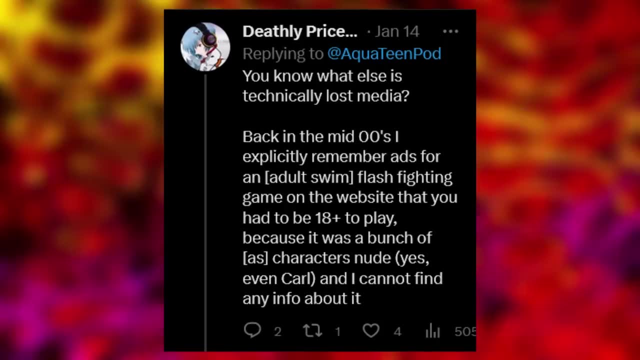 they explain that they explicitly remember ads for an old Adult Swim flash fighting game on the website that users had to be 18 plus to play because it featured a bunch of Adult Swim characters nude, and that included Carl. So if anybody has any information on this rumored Lost Nude fighting game, then drop it in the comments as well. 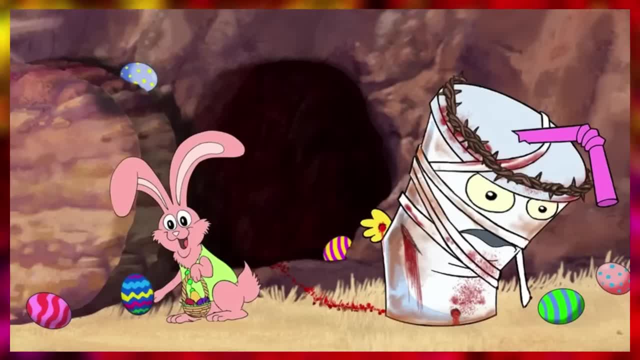 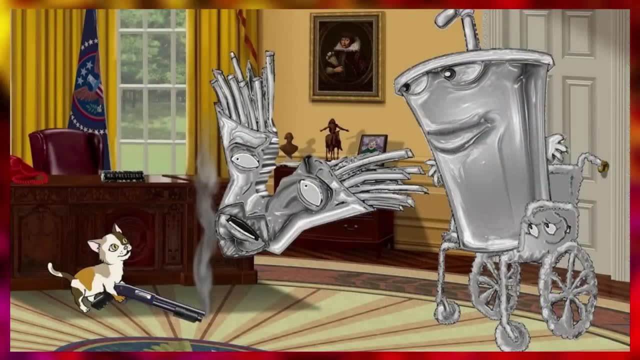 Promotional images. Yeah, I'm not entirely sure what these images are or where they came from. I wouldn't be surprised if they were just promotional images created to confuse people, because that isn't a new concept or anything for the Aqua Team creators. 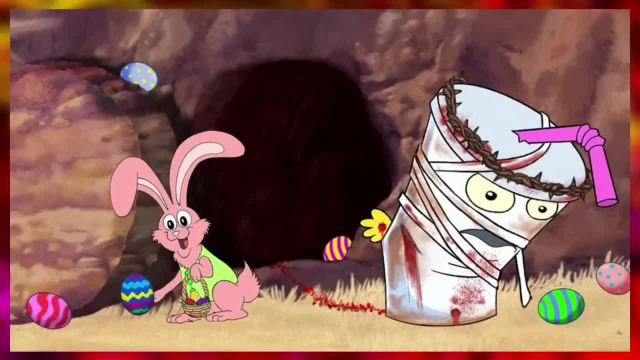 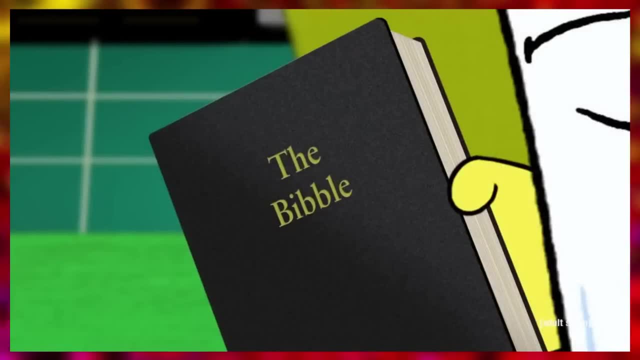 But the first image we have here is Shake, dressed up as Jesus crawling out of a cave, a reference to the story of Jesus being resurrected on Easter from the Bibble. Wait, is it from the Bibble? I mean Bible. I mean, yeah, Bibble. 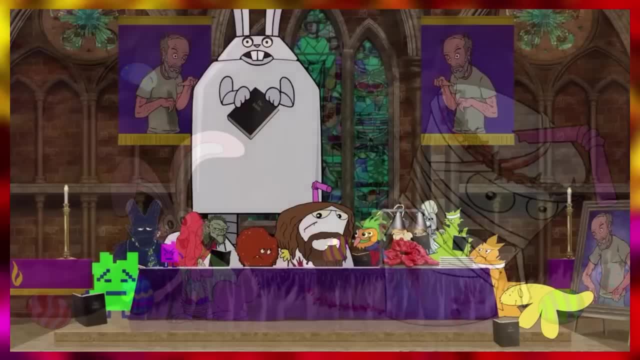 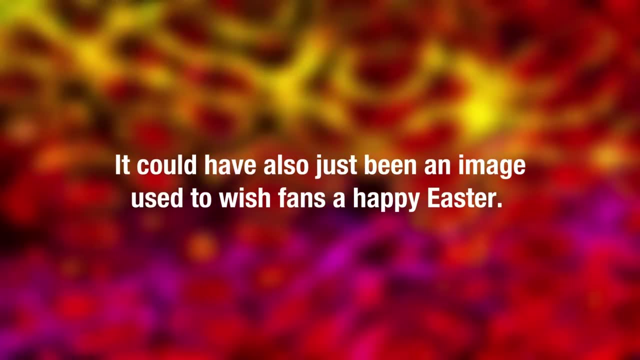 I don't know, I didn't read it. And outside of the cave is the Easter Bunny. Was this like a promotional image for the last episode of Season 11 or something? Because Shake is depicted in The Greatest Story Ever Told and then he dies. 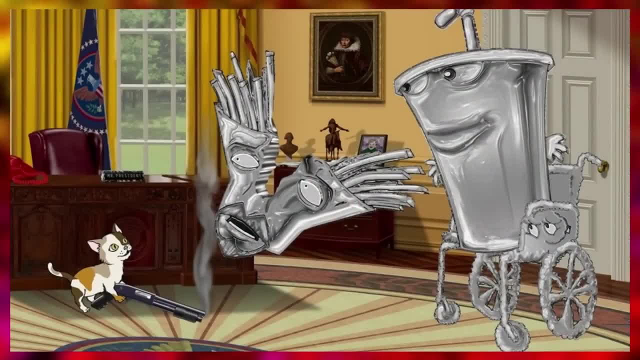 So maybe this image is him being resurrected. And let's take a look at this image. This is even more confusing. It's Shake Frylock and Meatwad- made out of metal, I think, and a cat blasting Frylock. I hate putting these two images so far down on the chart. 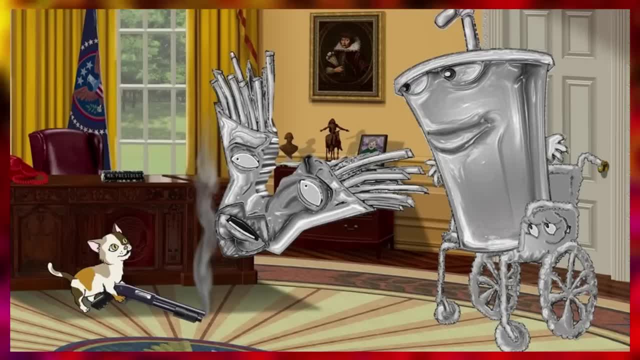 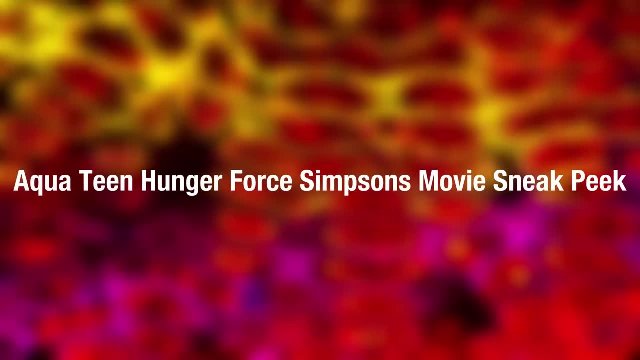 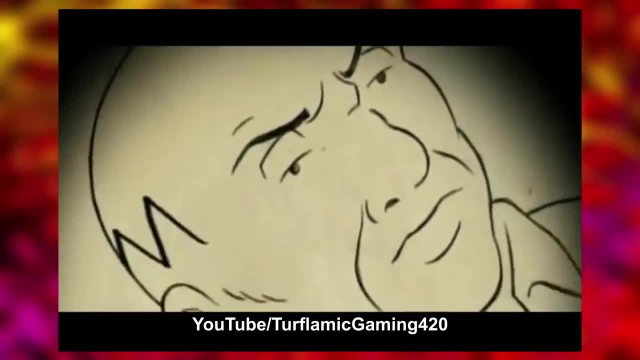 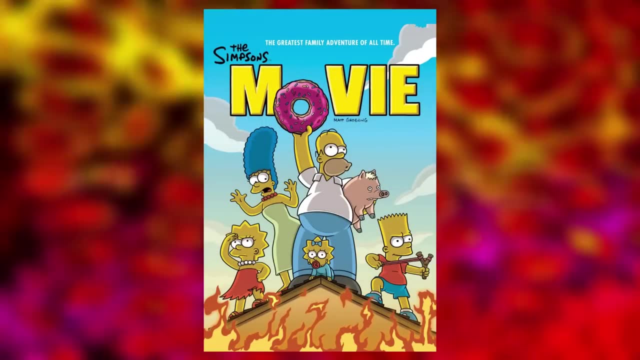 For my research, sometime between Friday July 20th 2007, and Wednesday July 25th 2007,, Adult Swim aired a Simpsons movie advertisement with a twist. The twist was that, instead of this being a regular Simpsons movie promo, 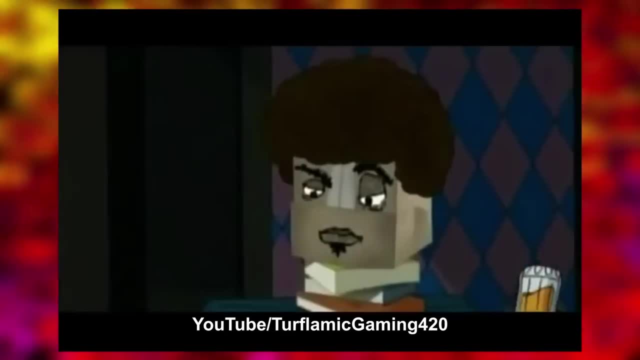 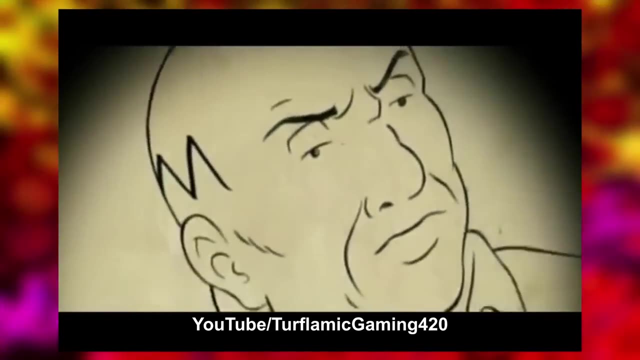 it featured Aqua Team, Hunger Force characters redesigned as Simpsons characters: Carl was Homer, Meatwad was Marge, Frylock was Lisa, Shake was Bart, Ezekiel, Jesus Ezekiel was Maggie, Dr Weird and Steve were Mr Burns and Smithers. 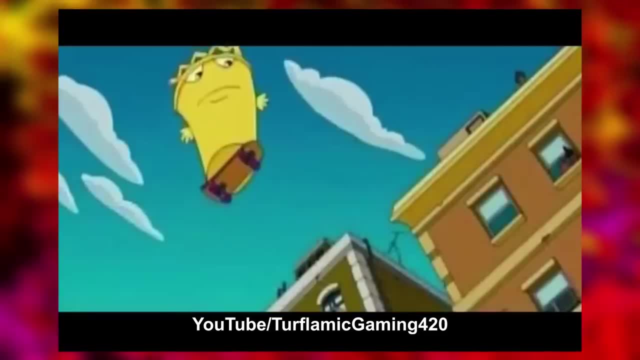 Bingo was Krusty Oog was Barney Happy Time. Harry Emory was Lenny Foxy Brown was Carl Little Brittle or MCP Pants was Grandpa Emery was Apu Oglethorpe was Chief Wiggum. 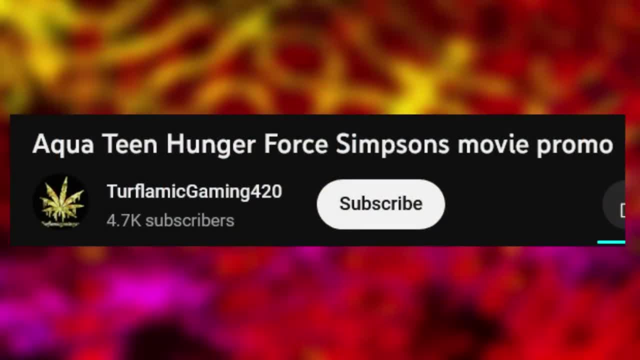 And there's so many others, I'm going to refrain from showing you guys the full trailer, but search up Turf Blame It Gaming 420's channel on YouTube if you want to see this wild piece of history in full. Now, at the end of the advertisement. 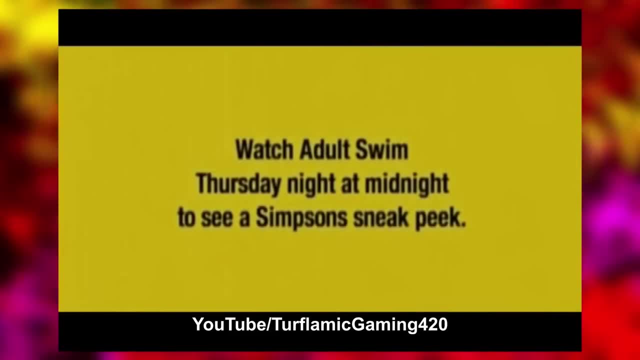 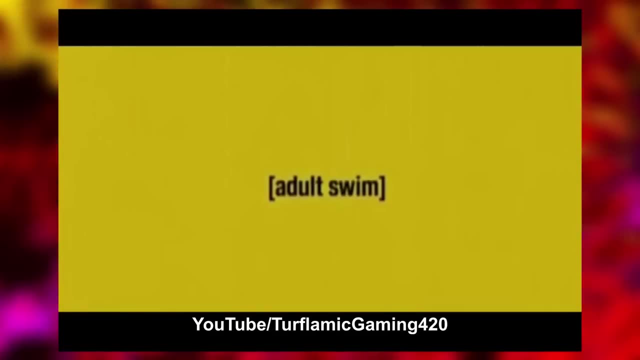 viewers were told to watch Adult Swim on Thursday night, the 26th, to see a sneak peek of the new Simpsons movie. However, nobody has any footage from that night. I've seen comments online from viewers claiming that there wasn't really a sneak peek. 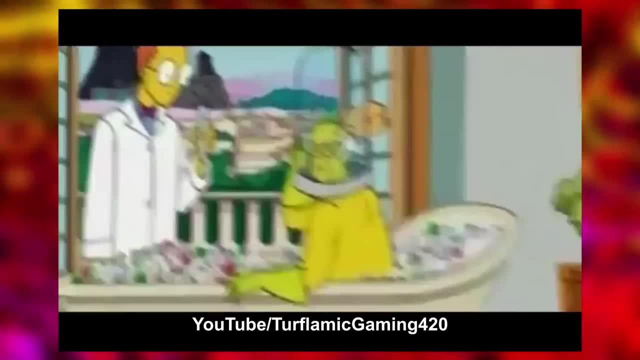 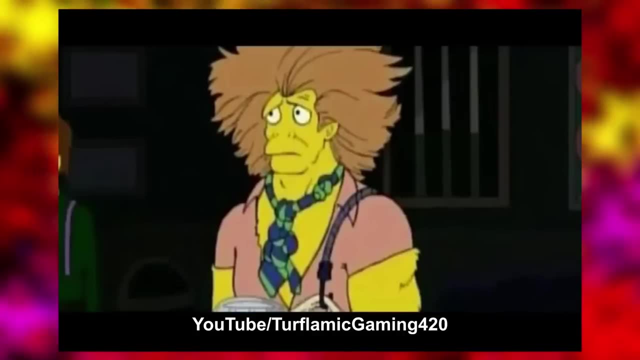 but just a showing of the official Simpsons movie trailer. I've seen comments from people swearing on their own mother's graves that they saw a legitimate Simpsons sneak peek from that night, but don't remember which clip they showed. And I've mostly seen people confirm. 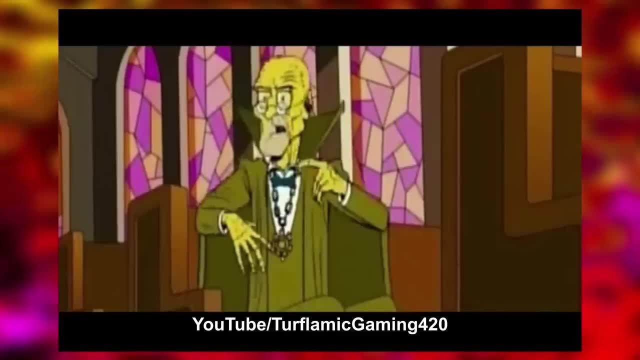 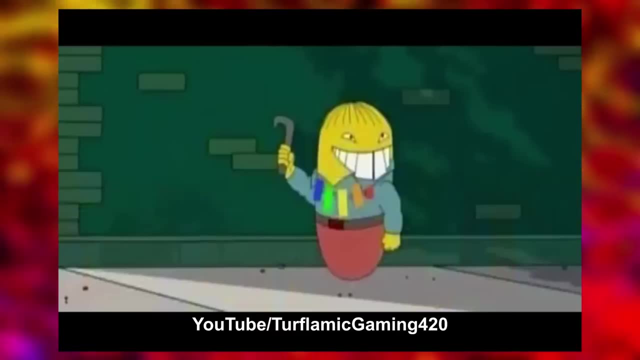 that they had no idea about this trailer's existence or anything. I might have also seen a comment or two from people claiming that they showed a clip from the film with the redesigned Aqua Teen characters, but I honestly doubt that. To be honest, I think this was just a one-off promo for the Simpsons movie. 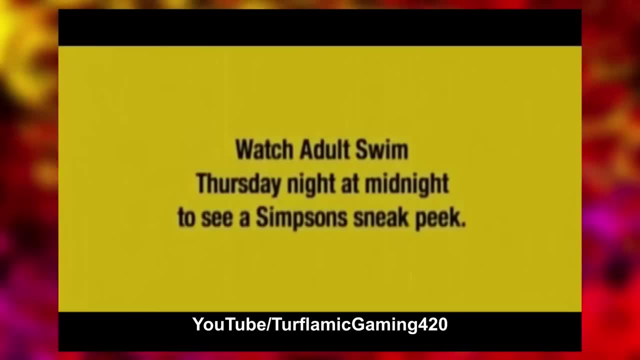 and that was it. So, um, I leave it to you guys. I don't really know if this is considered lost media. I mean maybe, But if you guys know anything about the Simpsons sneak peek or you have footage from that Thursday night over a decade ago or something, 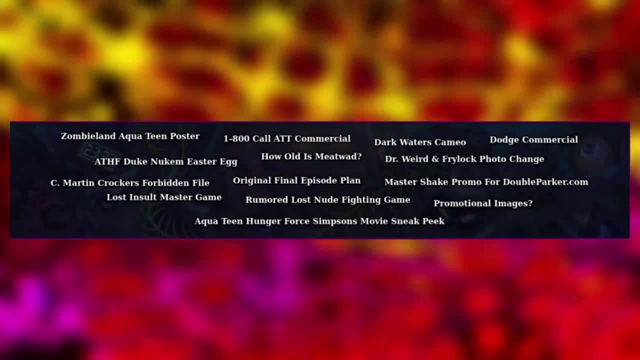 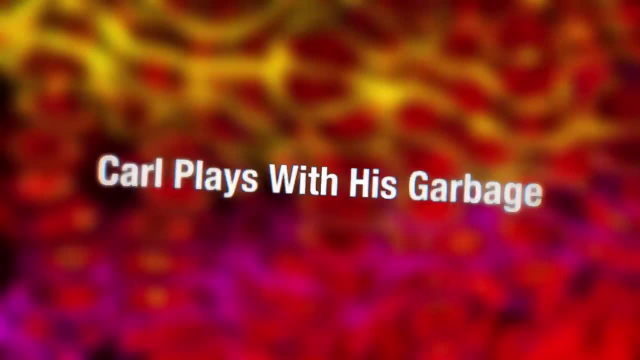 then let me know in the comments. But that, my friends, was the eighth layer of the iceberg. Dude, they're moonin' us Impossible, We are the moonin' knights. Carl plays with his garbage. A Reddit user named FryTheFly posted a theory on r slash fan theories. 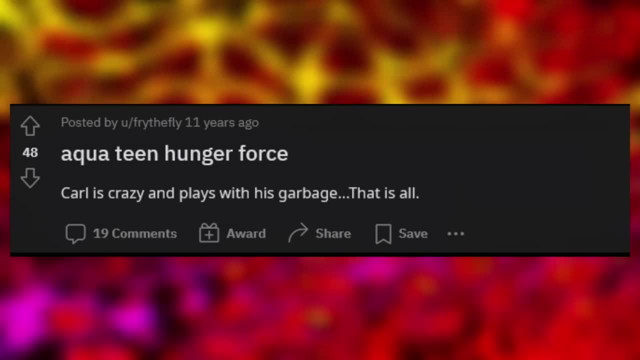 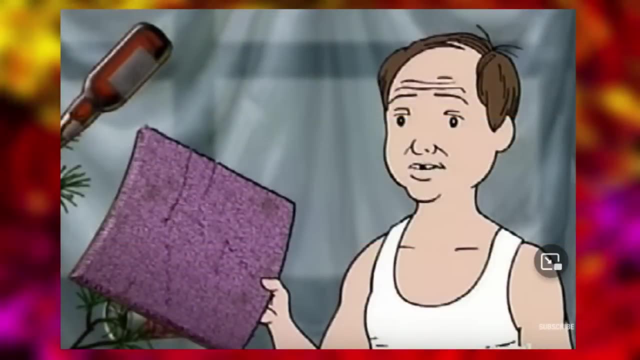 that reads: Carl is crazy and plays with his garbage. That is all. And in the comments section I saw a user trying to make sense of the whole idea by stating that when Carl was a kid he was forced to eat carpet because he was so poor. 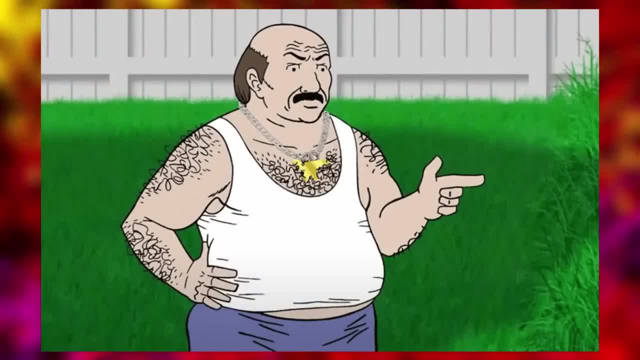 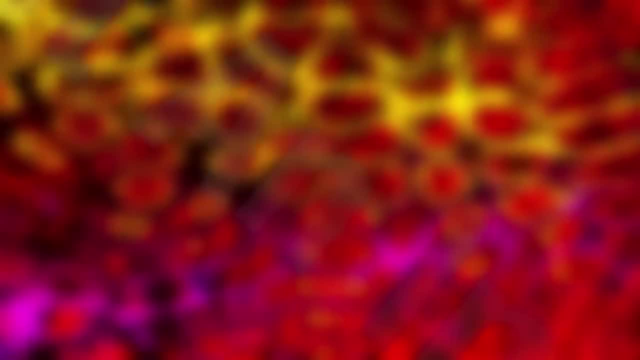 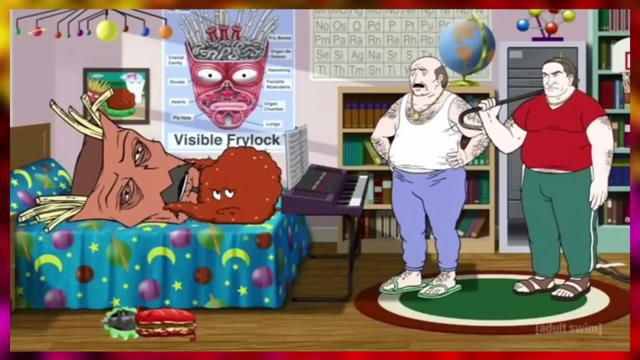 So playing with trash was more affordable than buying real toys at a store. Basically, everything that happens in Aqua Teen is just from Carl's imagination and he just acts it out using garbage. Death is just an inconvenience. This entry just means that death isn't really a terrible tragedy in the Aqua Teen universe. 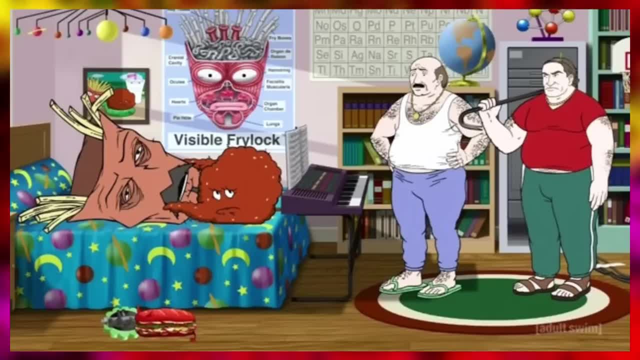 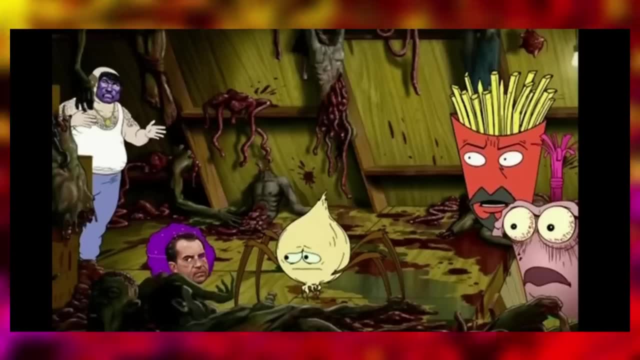 But rather a giant inconvenience and a huge pain. One minute, Shaker, Carl or whoever faces a truly grotesque death, only for them to be reanimated to life in the next episode. and the cycle repeats. So either Neil Peart is still out there. 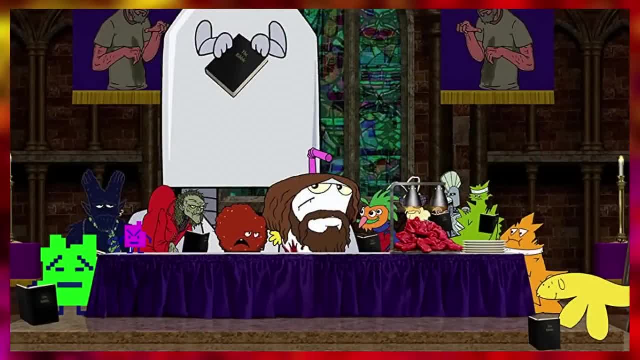 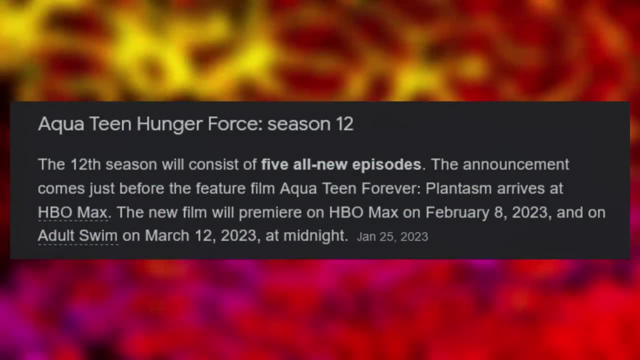 resurrecting characters with his drum solo of life, or characters are just trapped in hell for a few business days before having the opportunity to go back. Either way, death is temporary. Just ask Adult Swim Circuit Attack According to both the Aqua Teen season. 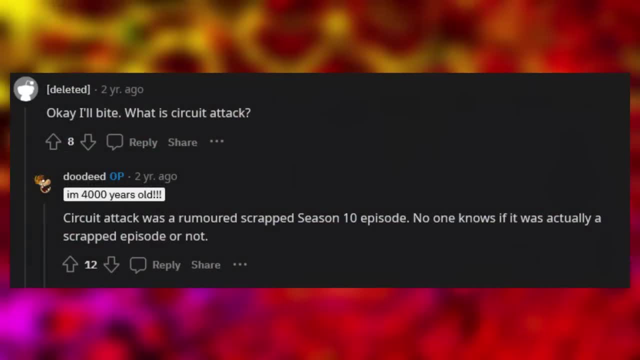 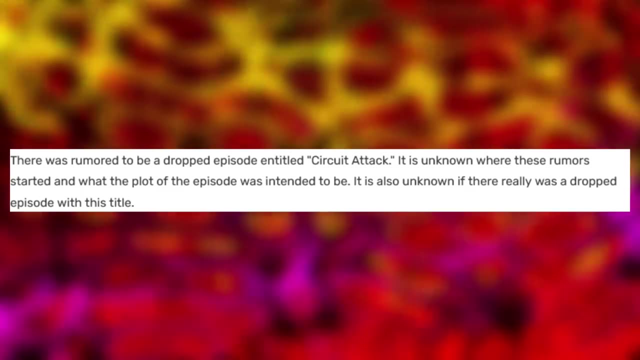 and this comment from Reddit. Circuit Attack is a rumored scrapped episode, But nobody on this godforsaken planet knows where this rumor started. I mentioned Circuit Attack in my last Aqua Teen iceberg because it was an entry on one of the charts that I used to create mine. 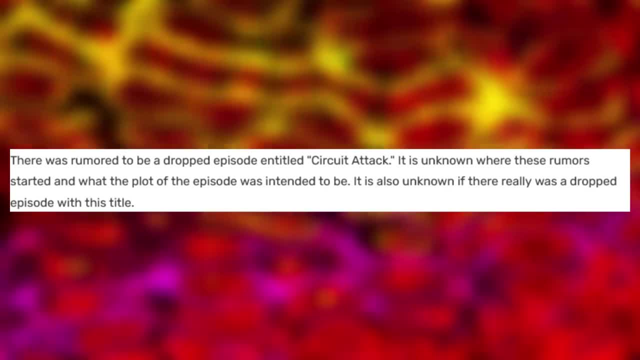 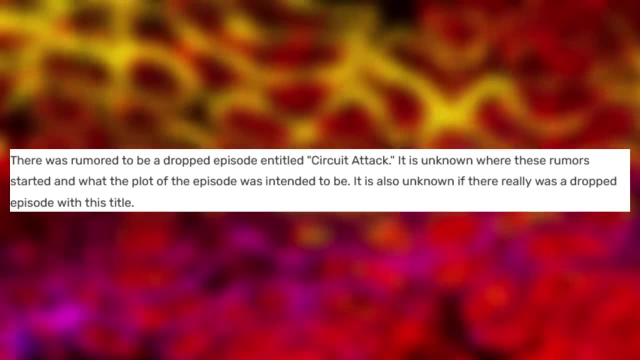 And since working on this updated video, one of my main goals was to figure out if this episode was real or not, And, thanks to Ronnie, we now have somewhat of an answer as to where Circuit Attack might have stemmed from. I asked Ronnie if he could ask Matt Malero about the Circuit Attack. 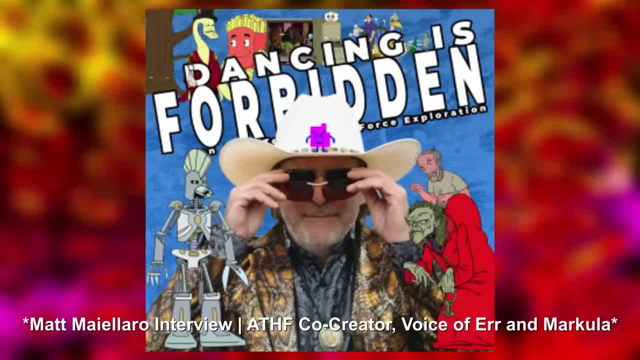 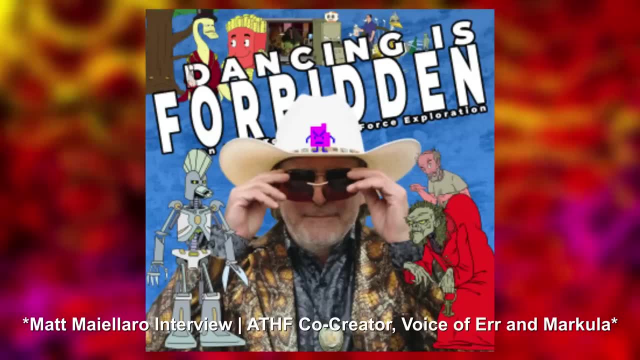 and here's what Matt had to say about it. Okay, so I have a question for you about two rumored scrapped episodes. There is the rumored episode Circuit Attack. Does that ring any bells? No, it doesn't. What's it about? I've never heard of Circuit Attack. 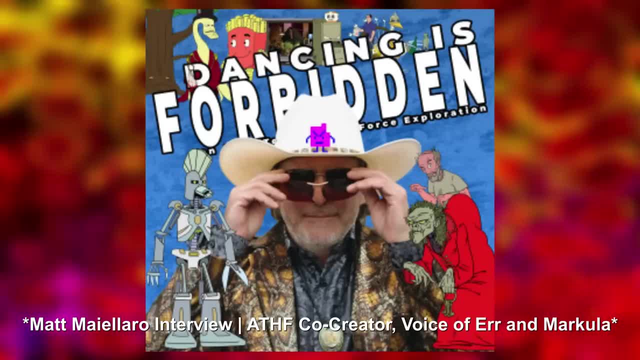 I don't know about Circuit Attack. All I've seen is it's rumored that someone just gave a name. Obviously, I didn't really expect it to be true, but I wanted to ask you about that. Yeah, I don't know anything about that one. 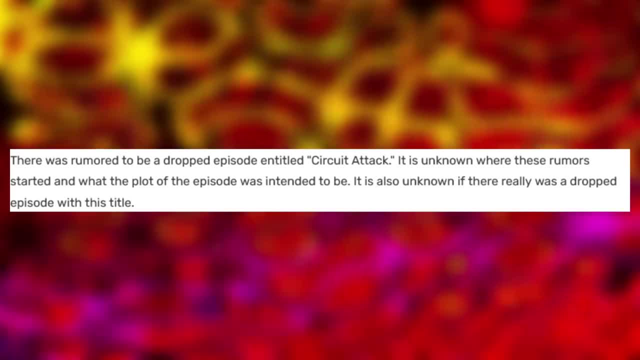 So yeah, Matt has never heard of Circuit Attack before. It's most likely a rumor. It's most likely a rumor. It's most likely that this rumor was started by someone looking to get attention, Unless Dave knows anything, but I doubt it. I truly think this Circuit Attack rumor is complete. BS. Space Ghost totally died in Aqua Teen, Hunger Force, colon movie film for theaters. I mean, we all saw it. Space Ghost blew up in colon movie film and is never going to come back ever. 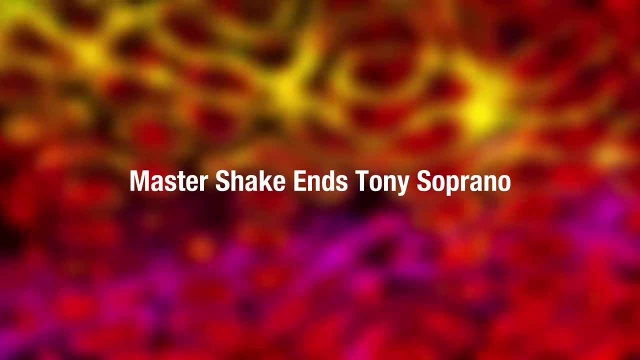 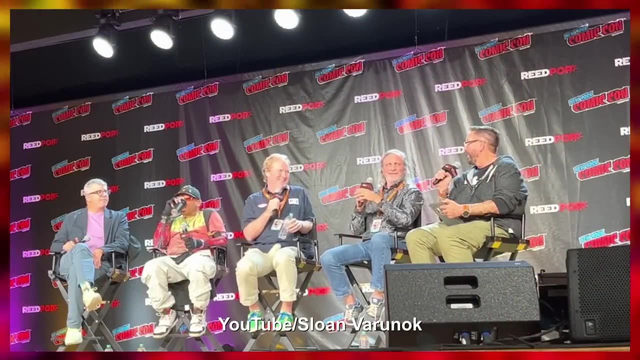 Hashtag continuity: Master Shake ends Tony Soprano, An Aqua Teen fan, at the Plantas and movie premiere at New York Comic Con 2022, asked the cast what they thought of the Aqua Teen cameo in The Sopranos. 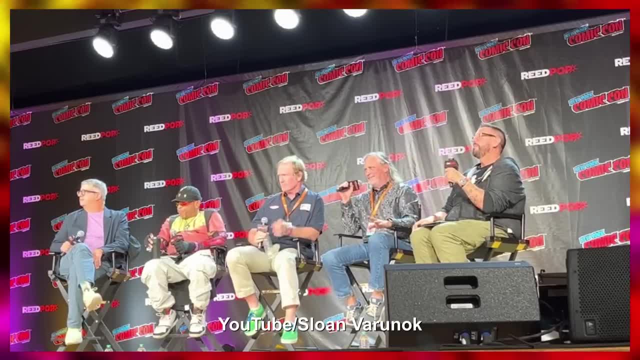 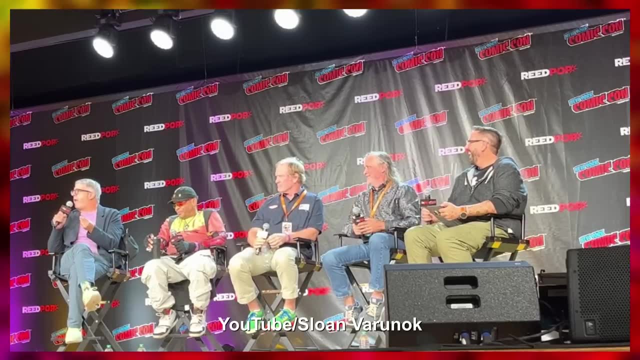 And Dana Snyder responded jokingly with how Master Shake was going to kill Tony Soprano in the final episode. You know already The Sopranos is a top tier series, but I would have lost my mind if Shake stood behind Tony before the cut to black. 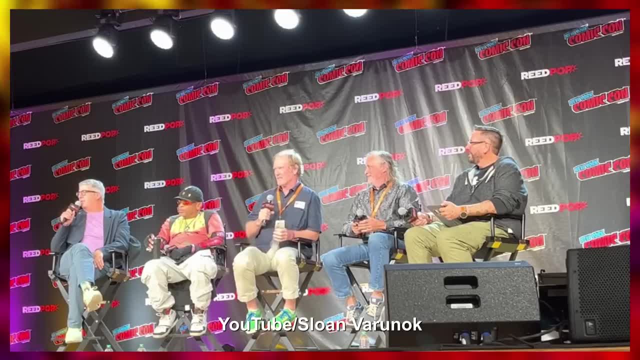 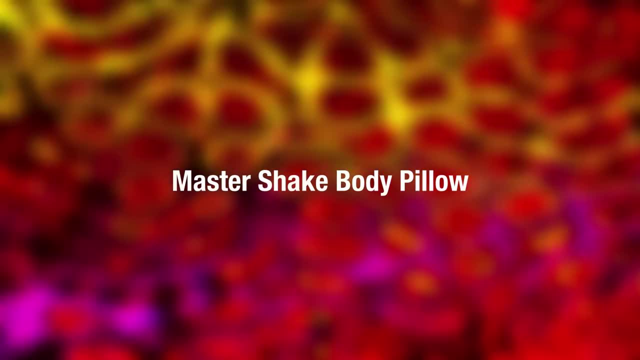 Well, and also Master Shake killed him in the last episode, but they didn't want to pay for new animation. That's what actually happened. Master Shake body pillow. I posted on Twitter that I was looking for some more entries for this iceberg and Twitter user The Masked Ink YZ. 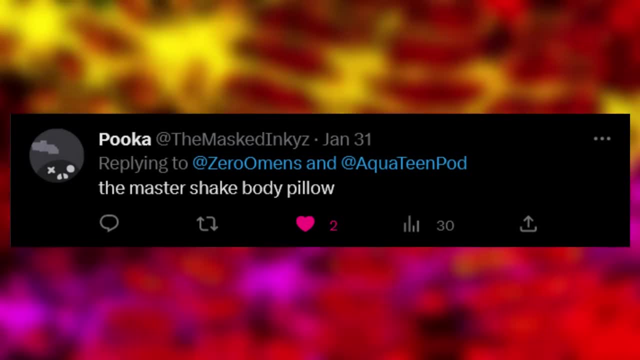 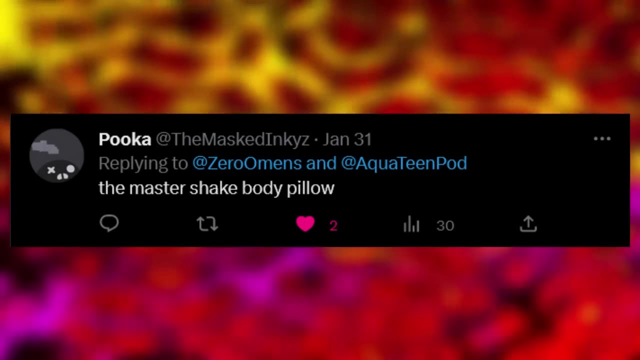 or The Masked Inky Z mentioned the Master Shake body pillow And I've never heard of this, So I Googled it, and I don't know if I was in the right neighborhood. when I Googled this entry, I found a thread from 2020 on Twitter. 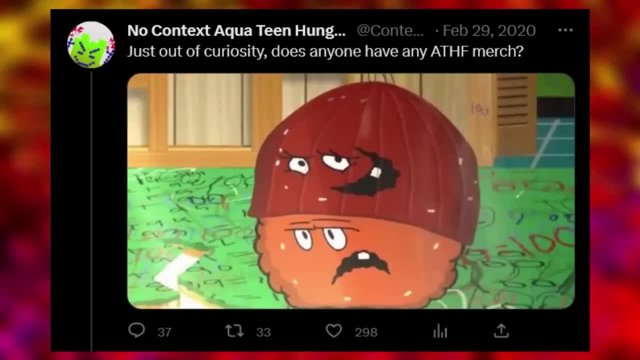 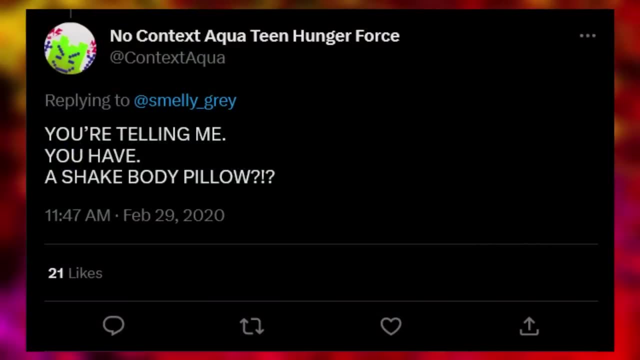 where Context Aqua asked if anyone had any Aqua Teen merchandise and user Smelly underscore Gray stated that they had a Master Shake body pillow. However, the pick of the pillow was deleted by the user, So I had to do some detective work to find this Master Shake Dakimakura. 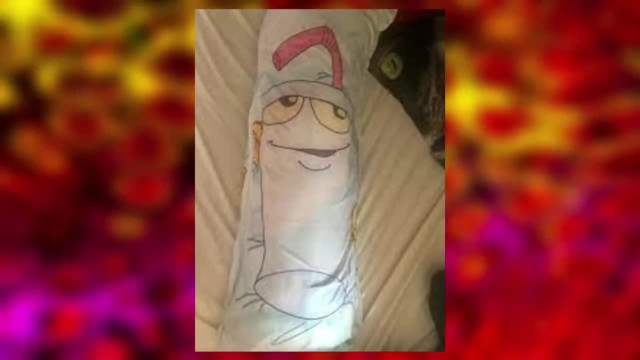 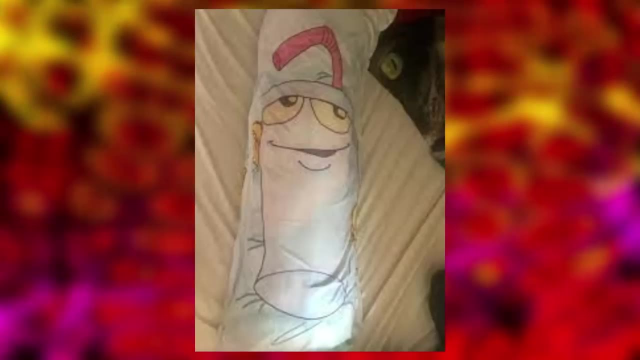 Now I'm not entirely sure if this is the same pillow that Smelly underscore Gray posted and owns, but I found this image on Google and it's the only image that I could find of a Master Shake body pillow. I even reversed image, searched the photo and nothing popped up. 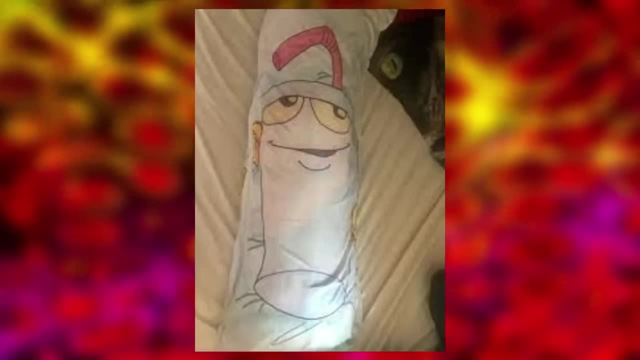 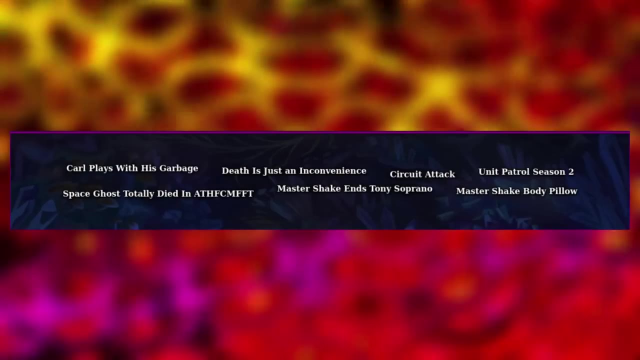 So I have some questions. Number one, where did this pillow come from? I mean, was it custom made? And number two, is this your pillow Smelly? But that's my question. This, my friends, was the final layer of the iceberg. 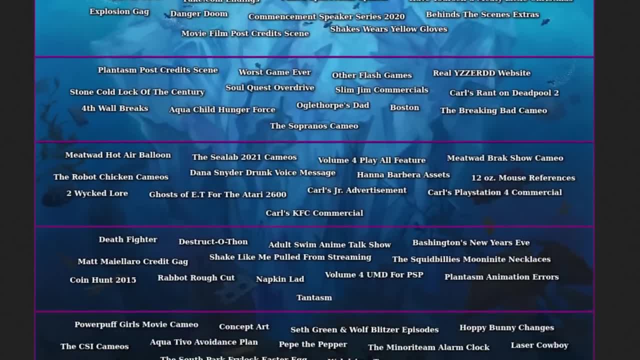 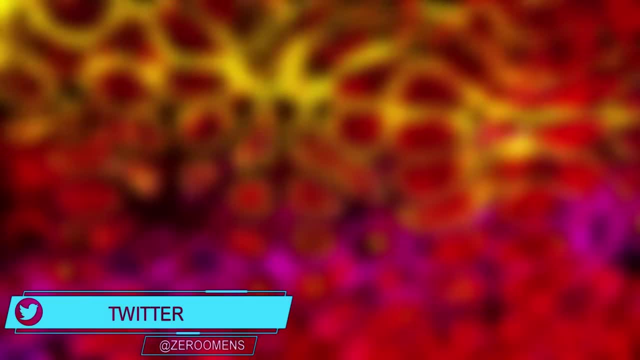 I'm going to go take a nap. Truly, they were an Aqua Teen hunger force. There you have it, my friends: A deep dive into the world of Aqua Teen hunger force. This video has been in development since October of 2022. 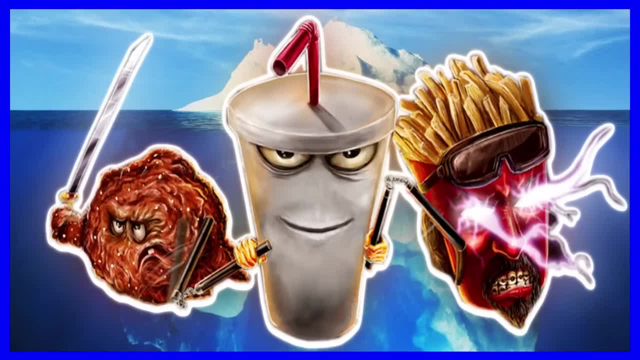 And boy oh howdy, golly, gee balls. Does it feel amazing to finally release this monster of a project to you guys? I've been hyping up this video for months, So hopefully it was well worth the wait for all of you. 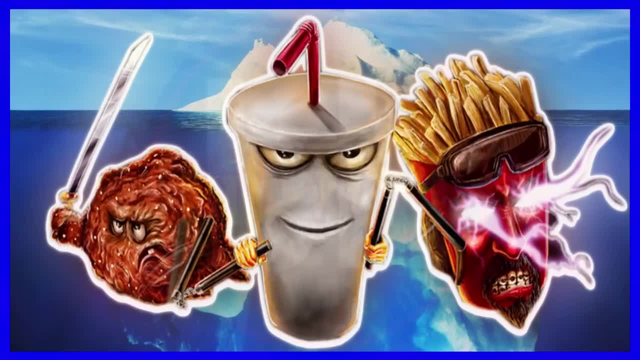 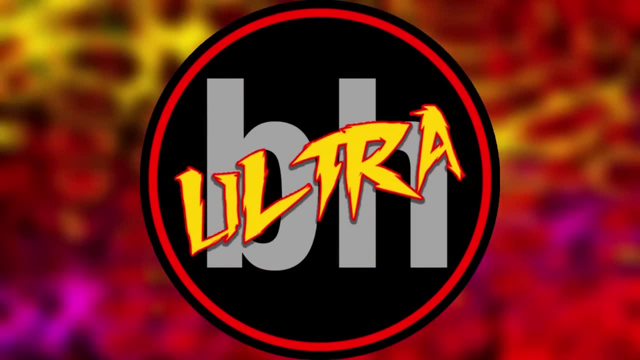 So thank you guys for being very patient with me while I worked on this project. Special thanks again to BHUltra for partaking in this video, narrating a layer and even adding some extra details to some entries as well. If you enjoy long form content and live streams, then you'll definitely love his content, as 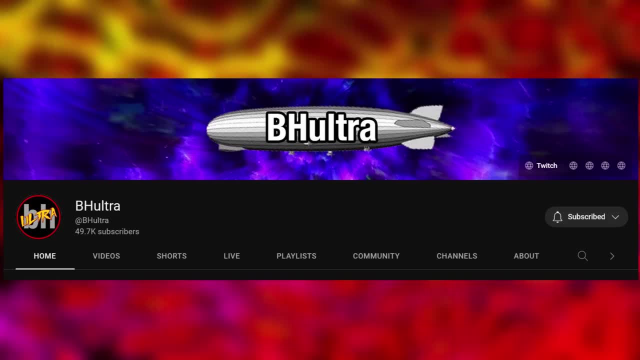 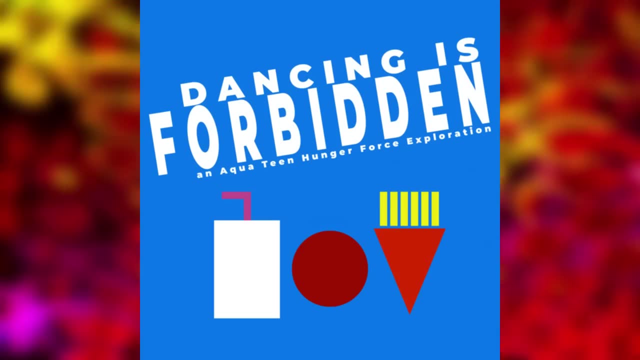 well, Their channel will be in the description below. And, of course, special thanks to Ronnie from the Dancing is Forbidden podcast for helping out a ton with this project. He narrated a layer, Introduced me to a bunch of new information that I had never heard of before. 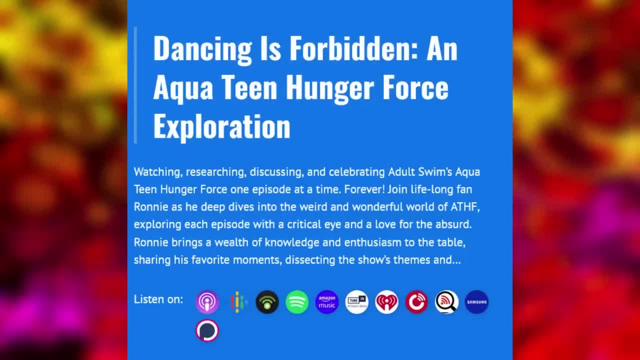 And he was very kind enough to answer a lot of my questions regarding some entries as well. And yes, the rumors are true. by the way, he is a very nice guy behind the scenes And I highly recommend checking out his podcast. Dancing is Forbidden, especially if you are. 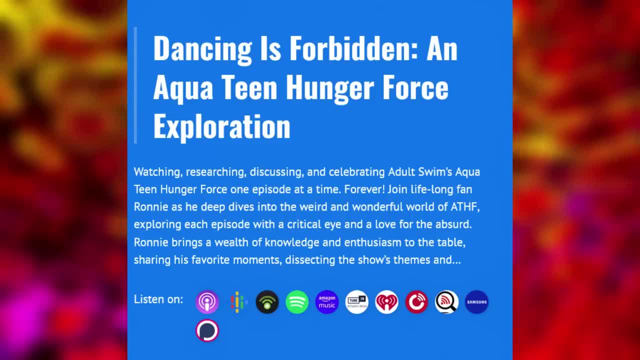 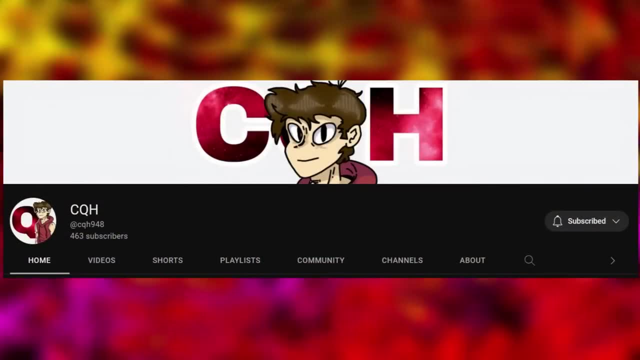 a hardcore Aqua Teen fan. You can listen to it on Apple Music, Spotify and much more. All links in the bio below. Big thanks to my homie Q for making a brief cameo in the middle of layer two. Really appreciate it, man.